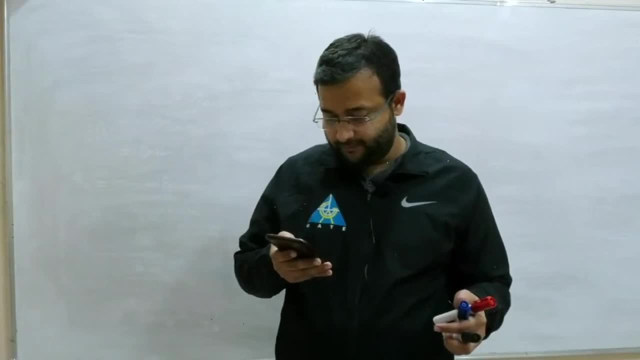 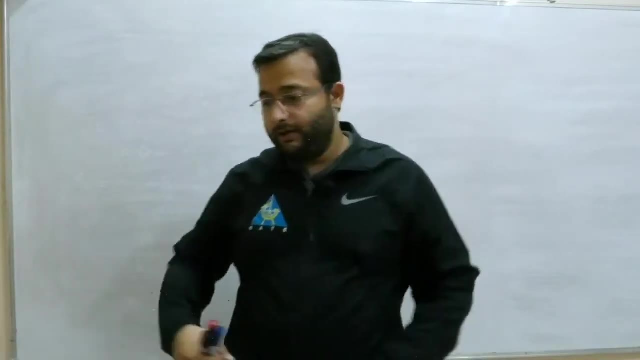 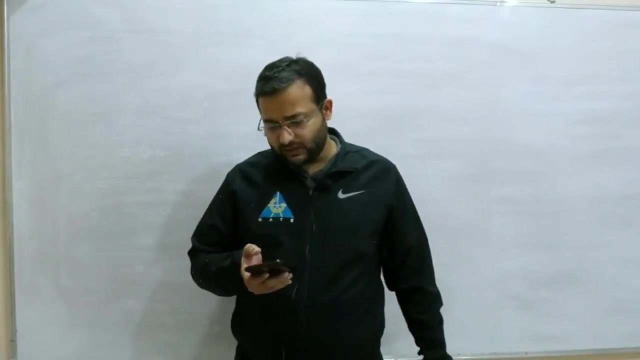 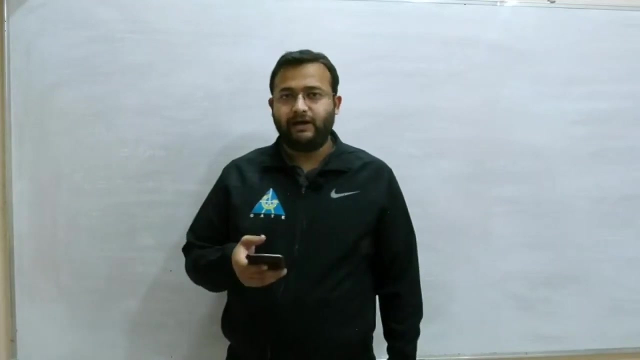 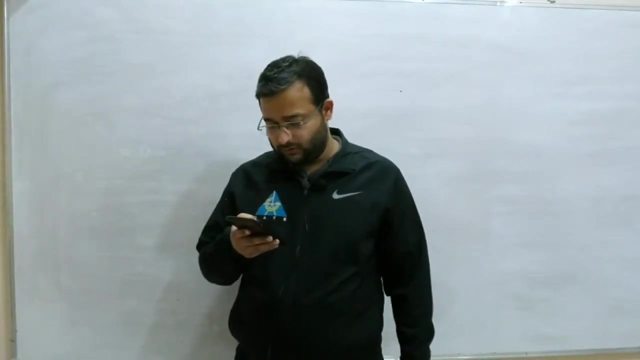 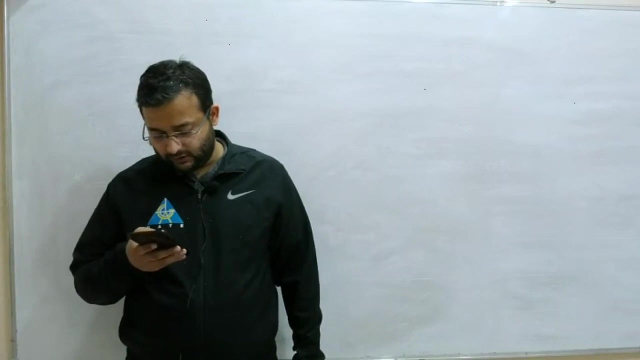 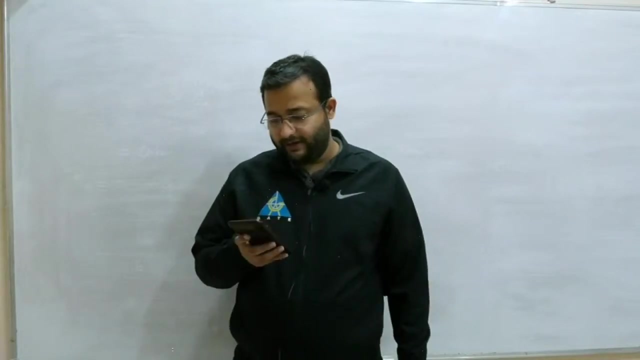 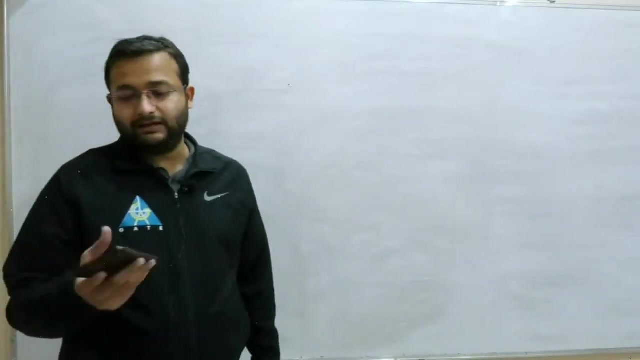 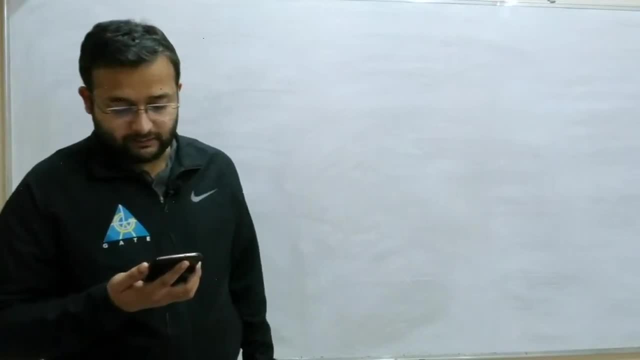 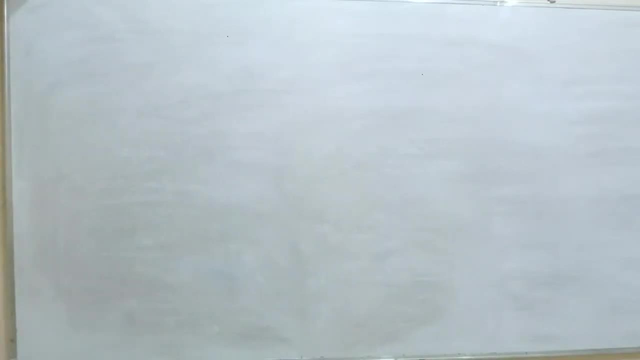 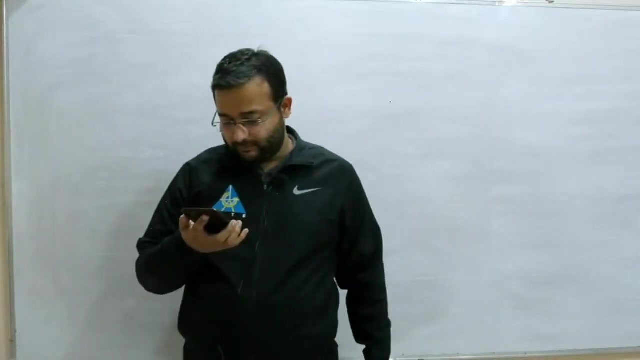 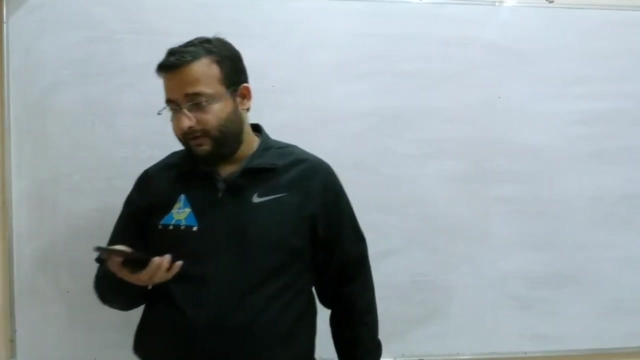 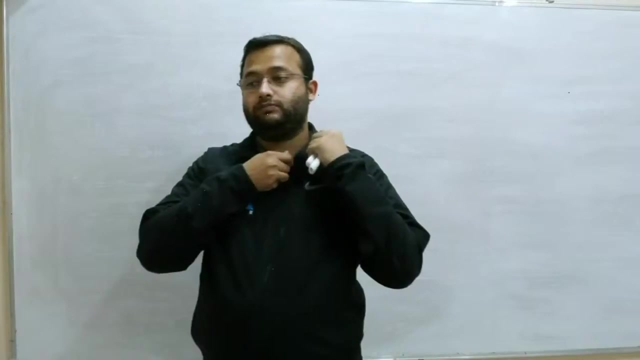 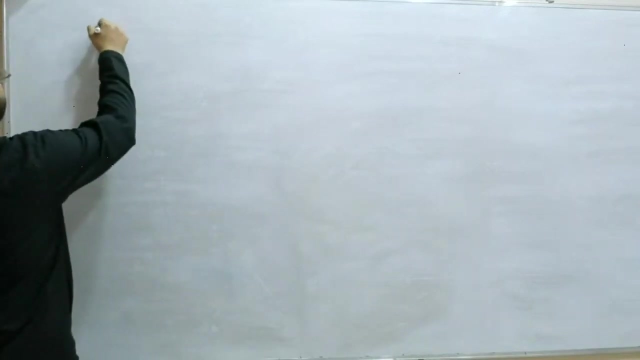 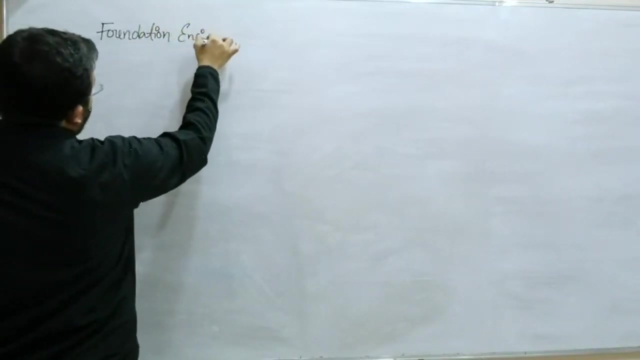 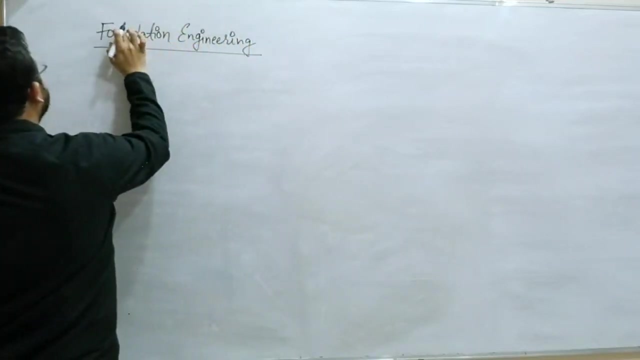 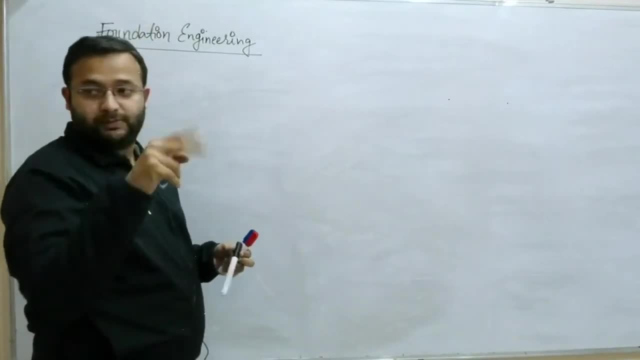 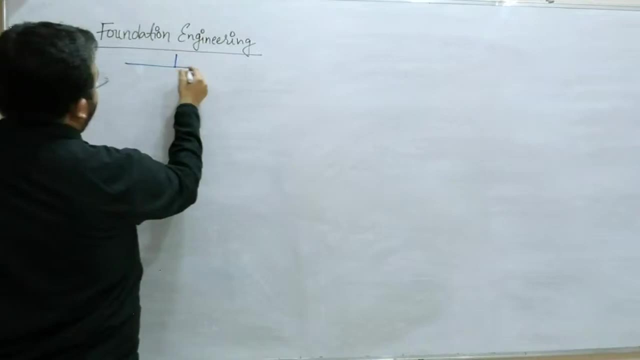 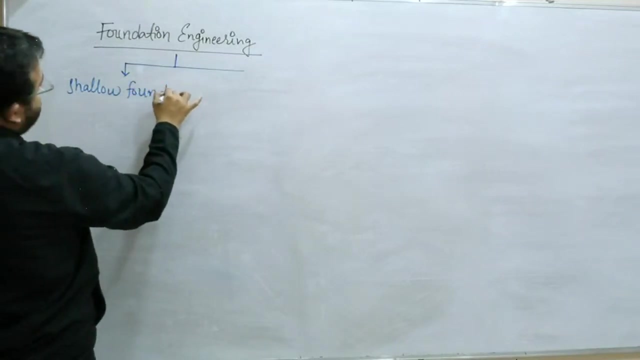 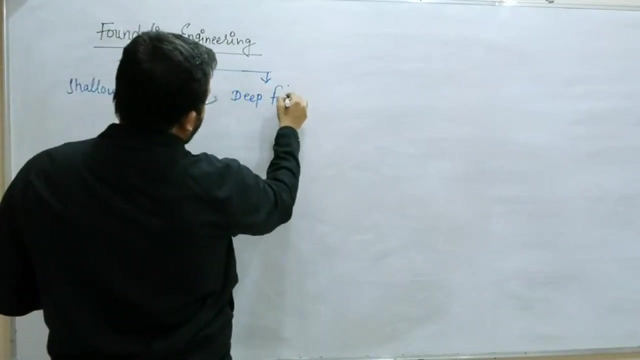 In engineering we are going to have two main chapters. one is shallow foundation and the other is deep foundation. I have two types of foundations. one is shallow foundation and the other is deep foundation. This can be shallow foundation and this can be deep foundation. 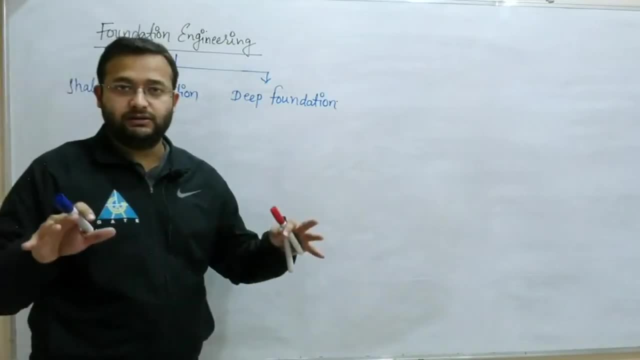 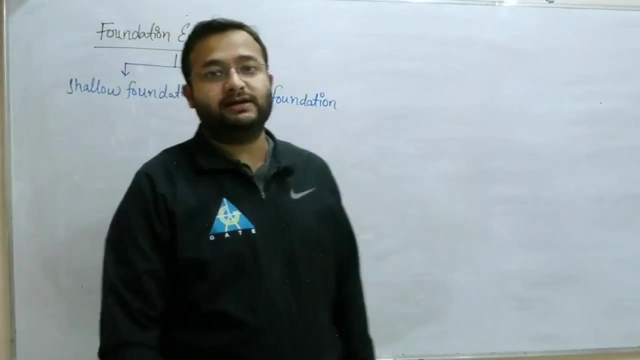 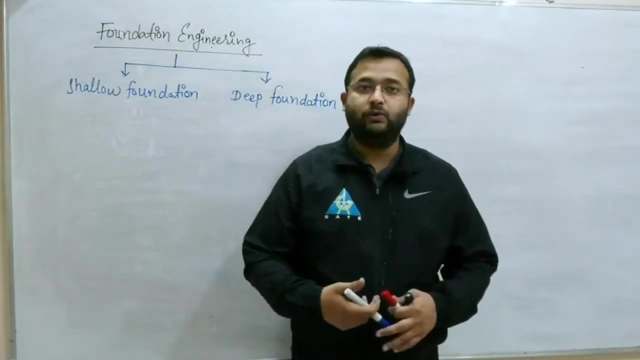 And here I have two different chapters If we talk about shallow foundation or deep foundation. I want to clear one thing: that in foundation engineering we don't learn to design foundation. You don't think that I will teach you design here that how much depth of thickness of footing you have to keep, how much area of steel reinforcement you have to provide. 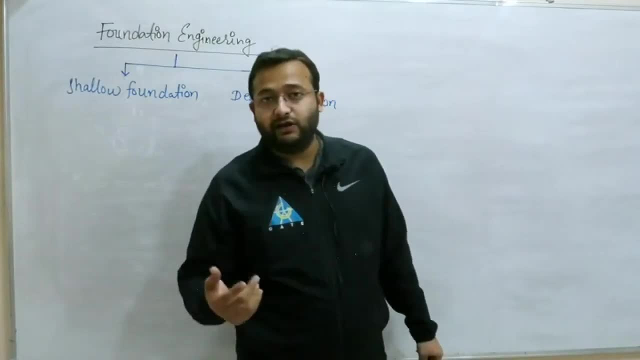 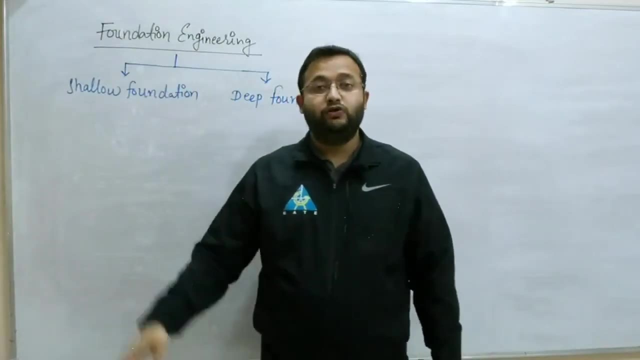 what will be the plan area of your footing? how many load signs there will be on it? We are not going to talk about all that here. That is the part of structural design. That is the part of structural designing. So what will we talk about in foundation engineering? 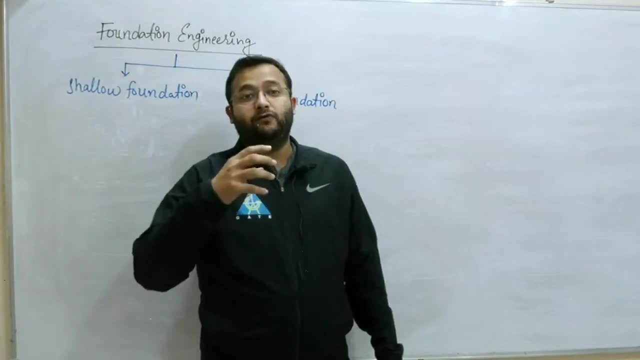 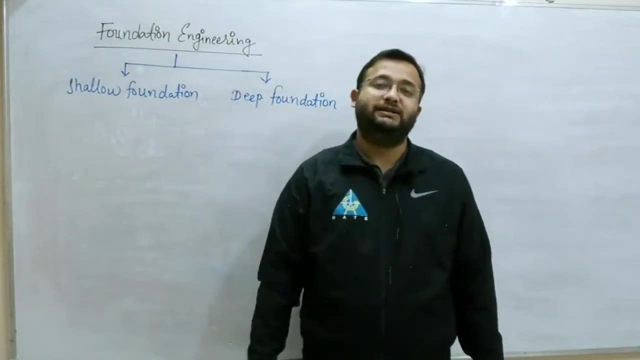 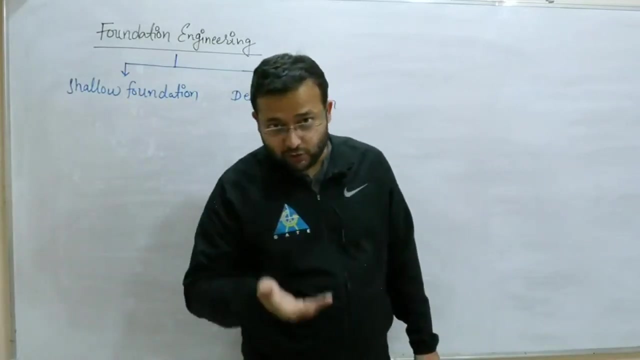 In foundation engineering, we will talk about the bearing capacity of the soil which is present under the base of your footing. What I am saying is that in foundation engineering, we will talk about the bearing capacity of the soil which is placed on the footing if you have shallow footing. 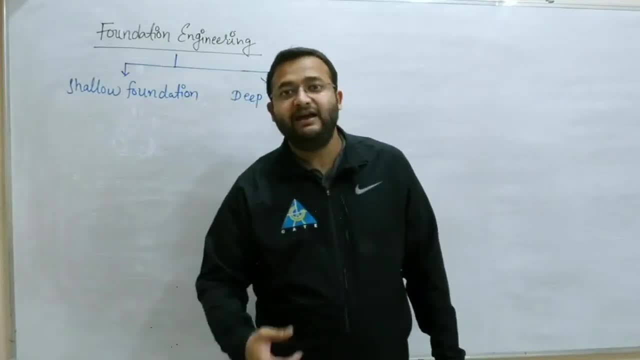 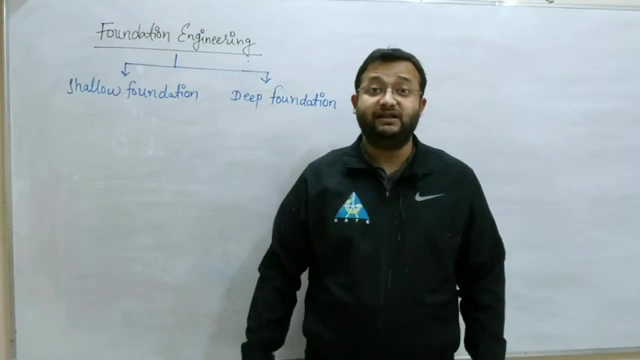 What is the bearing capacity of that soil? Can that soil take the pressure of this footing or not? We will talk about that In deep foundation. we will also talk about the capacity of soil capacity. How much maximum load can be applied on the pile so that the soil is not shear? 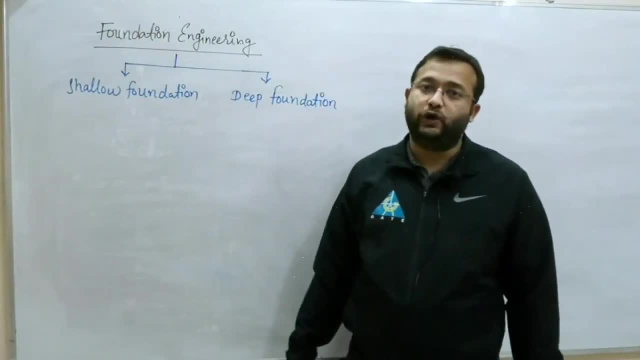 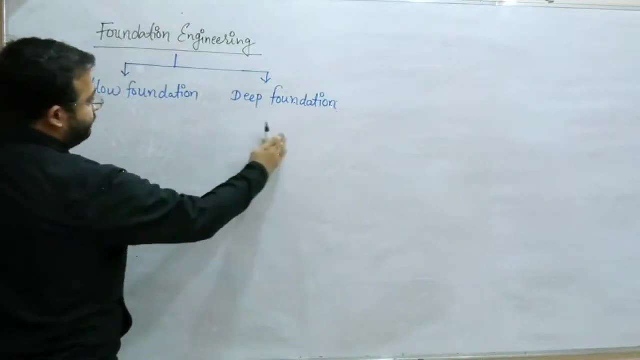 So we will learn all those things here related to soil. Okay, So if I talk about shallow foundation, then you will understand at a very good level that what is the meaning of shallow foundation and what is the meaning of deep foundation. Even then, I will write once that such foundation, whose width is more or equal. 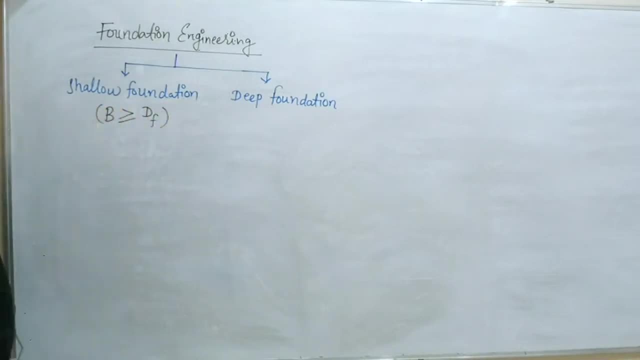 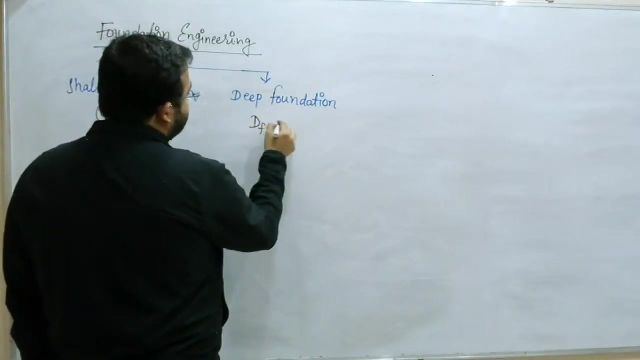 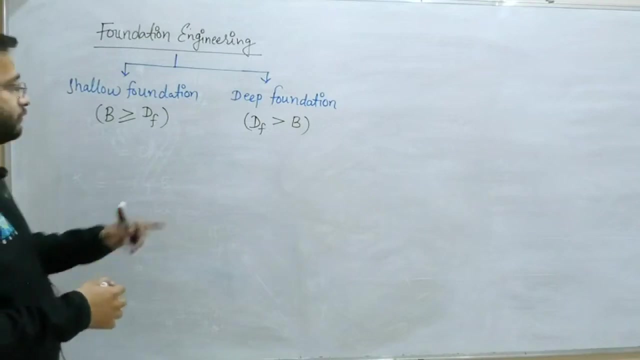 depth of footing, we will call it shallow foundation. And what is the meaning of deep foundation? Such foundation, whose depth of foundation is more width of foundation, we will call it deep foundation. So in deep foundation we will talk about pile foundation and in shallow foundation we will discuss about different types of footings. 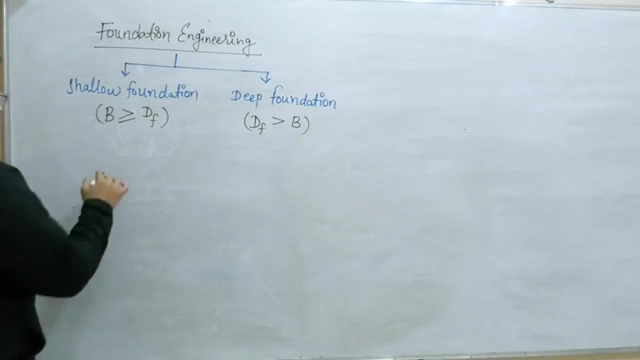 Let me clear one thing: What will be the meaning of depth of footing When I say that I have a ground surface here, then I dig a hole here. What do I do here? I do excavation work. So what did I do? 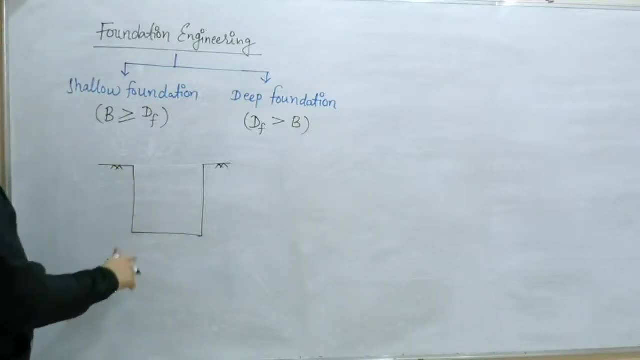 I dug a hole here. I dug a hole here. So the depth of the hole I dug, this is my depth of footing. This is my depth of footing. Some people do not understand that depth of footing means this thing. We are going to provide such footing right. 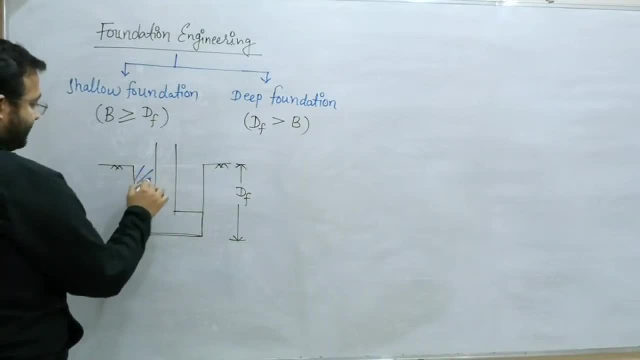 Brother, we will provide such footing. and what will we do here? First of all, we will fill the soil. Let's do this First of all. we make a hole, make a trench, put RCC in it, take the column out and fill the remaining portion with the soil. 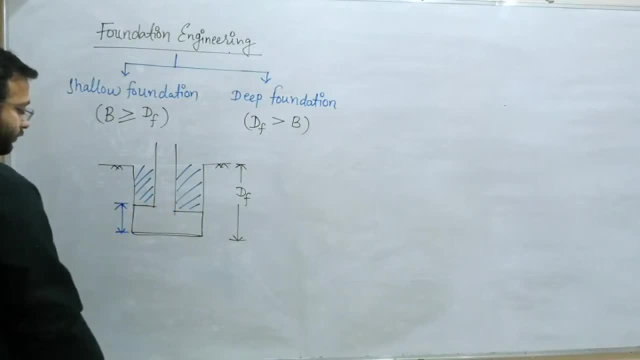 So some people do not understand that depth of footing means I am talking about thickness of footing- Wrong, I am not talking about this. I am talking about the whole depth of the hole. The depth of the hole you have dug, that is your depth of footing. 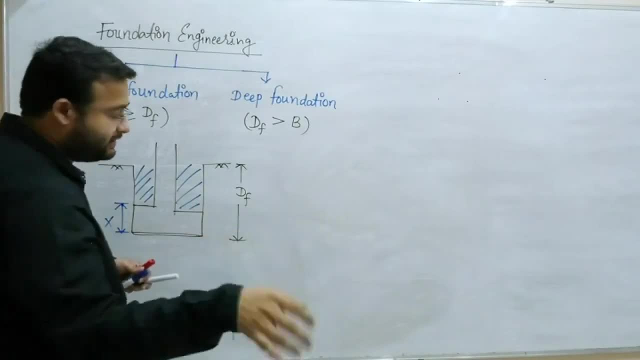 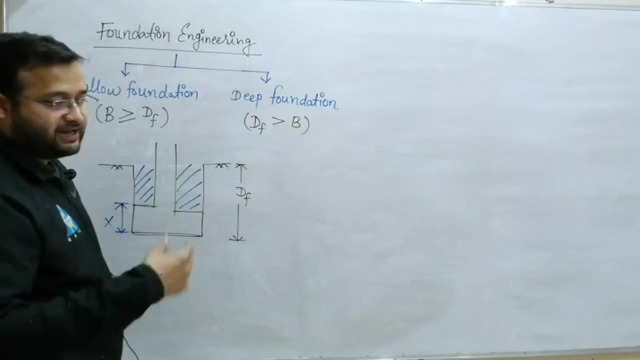 Clear Right now. I have nothing to do with thickness of footing, Because in thickness of footing I have to dig a hole, Because I design the thickness of footing in RCC. I have taught you the bending moment criteria. one way shear criteria. two way shear criteria. 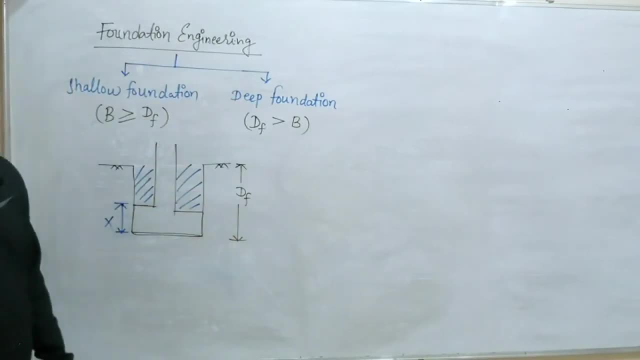 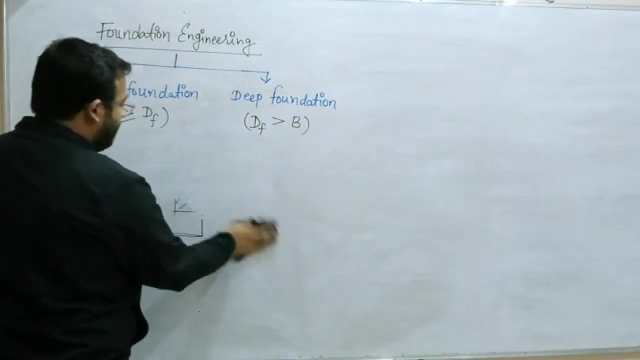 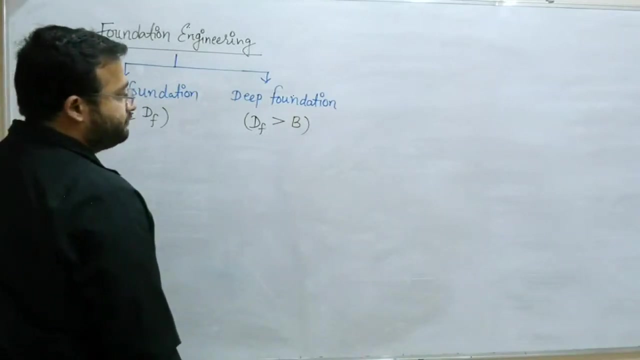 So we design the footing in RCC. Is it clear till now? So this will be my depth of footing, Depth of excavated part. Let's move ahead Here. I have to find the bearing capacity. On what basis do I have to find it? 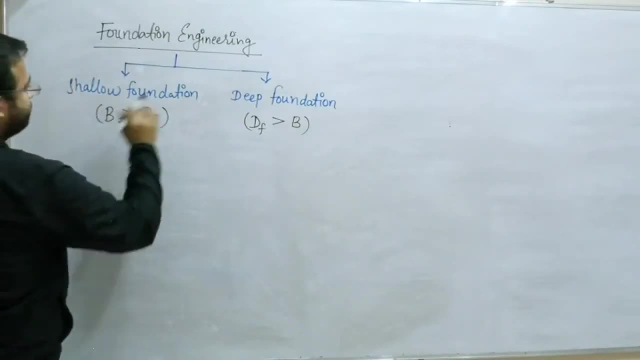 We will talk about that. So for now, we are going to take the shallow foundation. Our today's chapter, the first chapter that I am teaching here, will be your shallow foundation. First of all, we will see the shallow foundation. After that we will jump to the deep foundation. 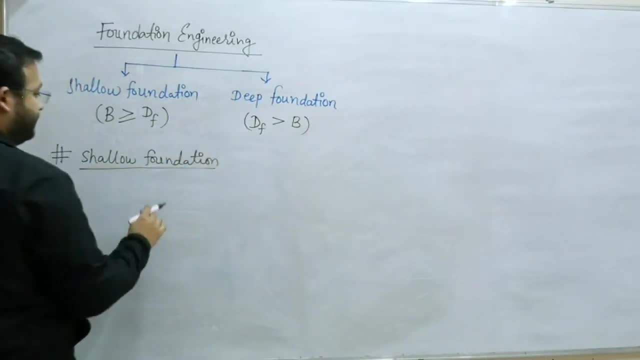 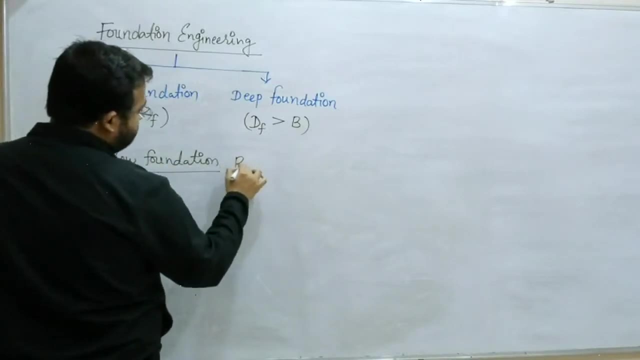 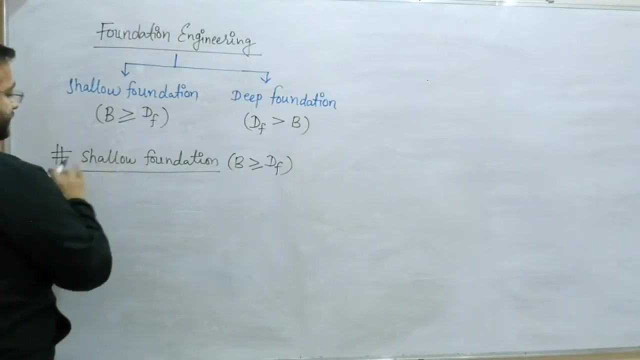 So you have understood the shallow foundation, Brother. shallow foundation means a foundation whose width is more than its depth, Or if it is equal, then also it will work. Now, in shallow foundation, I will tell you: If you have to find the bearing capacity, then I will have two criteria. 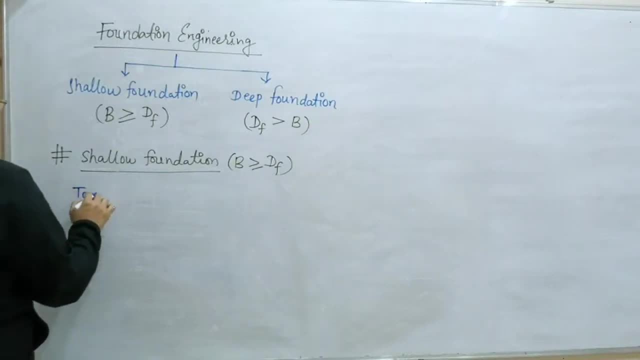 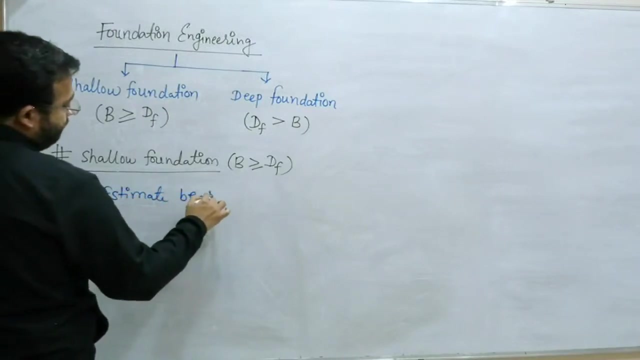 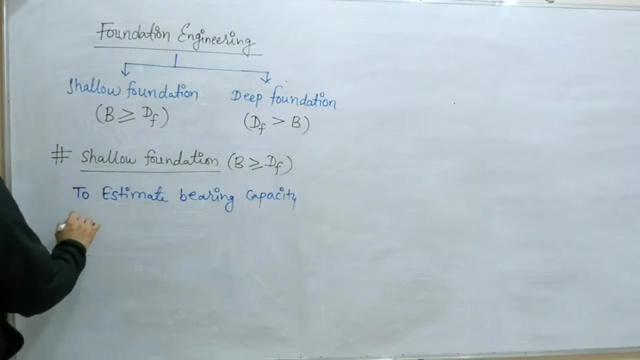 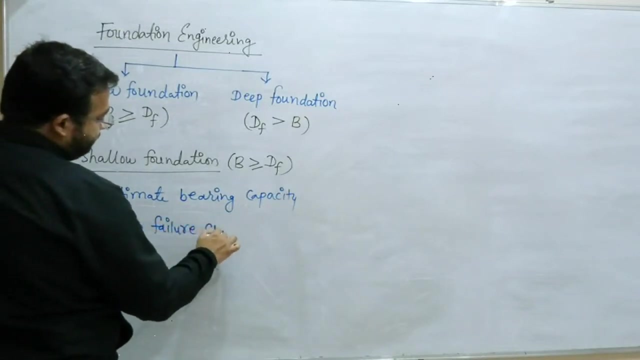 If I have to find the bearing capacity, then I will have two criteria. So I am looking here To estimate bearing capacity. I will have two criteria To estimate bearing capacity. What criteria will be there? We will have one criteria, That is, your shear failure criteria. 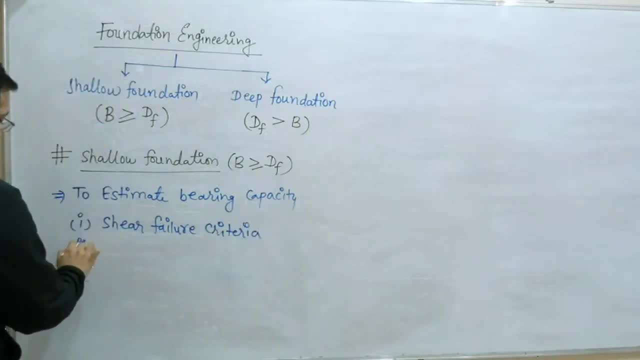 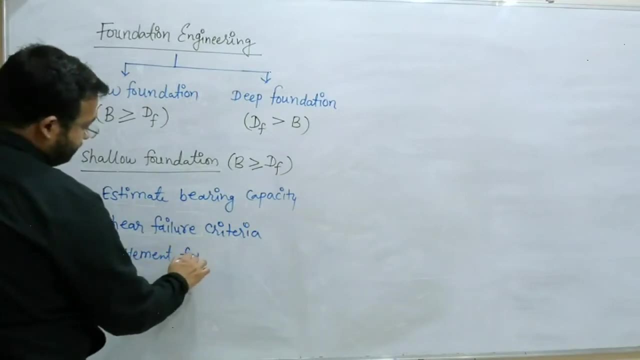 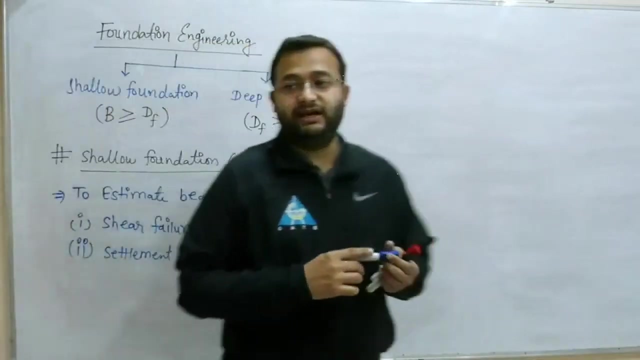 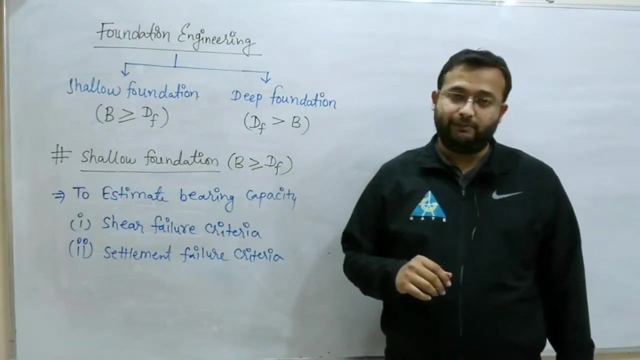 And your second criteria will be settlement failure criteria. What I am trying to say is that if you have to find the bearing capacity, You have to find the bearing capacity in the shallow foundation. So the bearing capacity of the soil can be found in two ways. 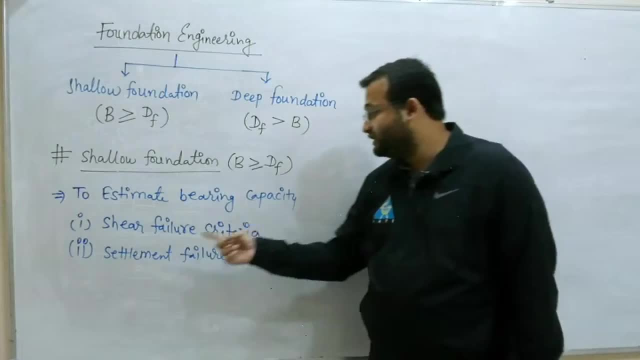 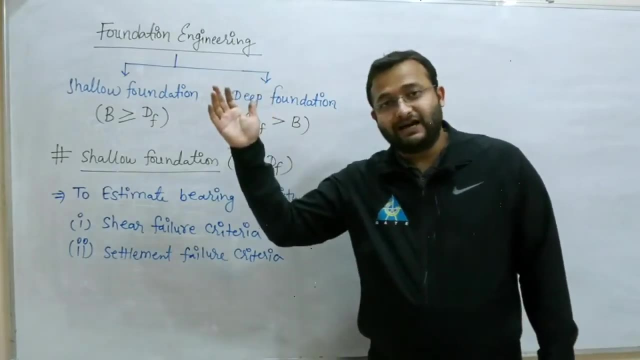 One way is your shear failure criteria. The other way is your settlement failure criteria. That means you keep on applying load, The load on which the soil gets shear. That will be your maximum load. What will be your corresponding Bearing capacity can be determined. 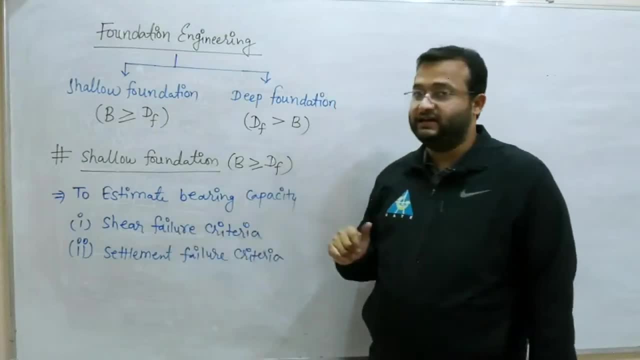 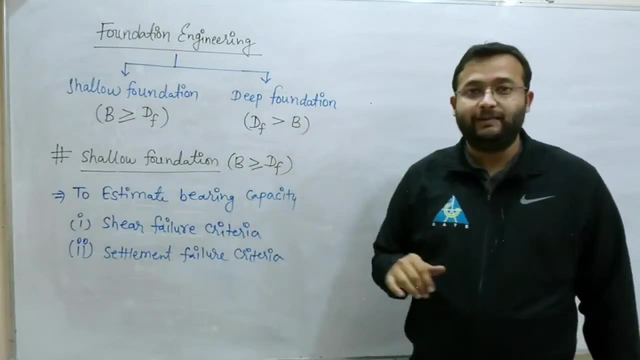 So what I have told you? This is your shear failure criteria. That soil may be sharing by going on some load. We have one: Settlement Failures Criteria, Settlement failure criteria. What does that mean? You keep on loading, keep on measuring the solution. 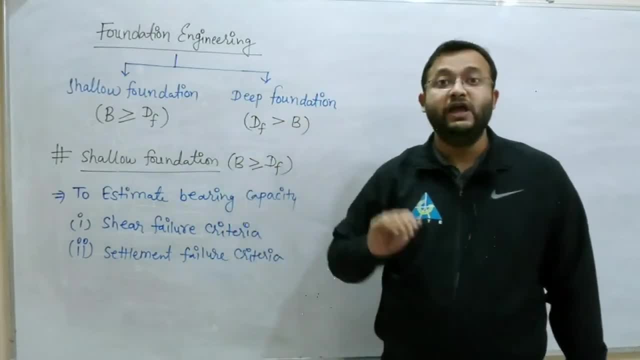 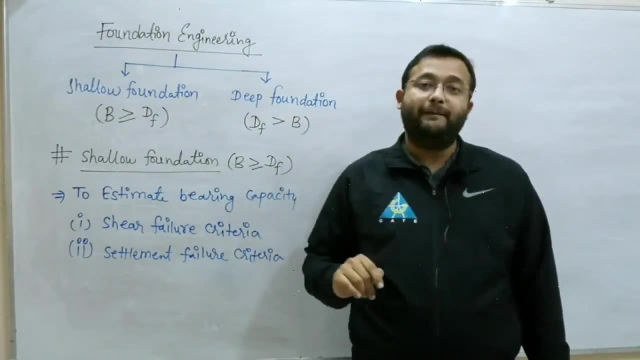 Keep on loading. keep on measuring the solution. Keep on loading. keep on measuring the solution. If, at some particular maximum settlement You are suddenly observe a large settlement Means on that load your soil is already shared. I am just applying load on the soil. 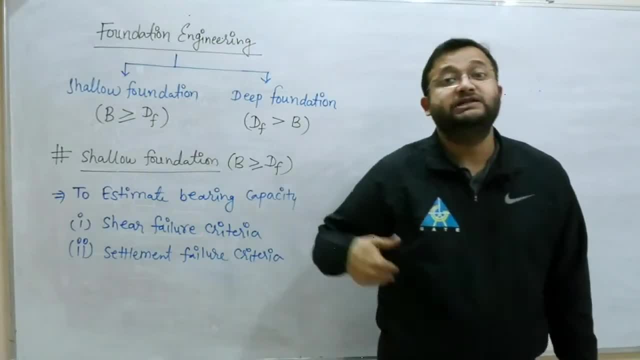 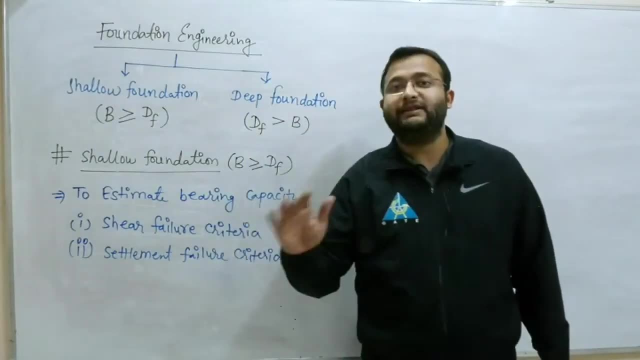 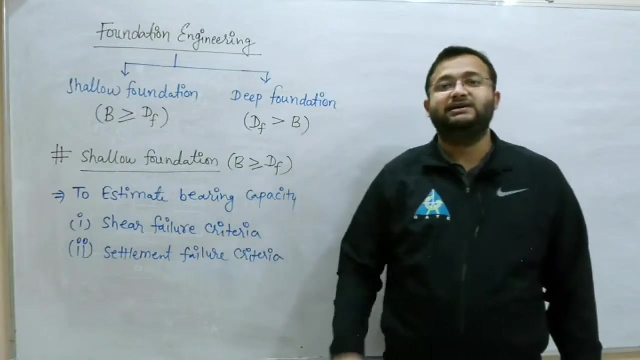 Apply it, apply it, apply it. The value of settlement is getting more and more in the soil. Suddenly you get a lot of settlement on. a load Means your ultimate bearing capacity has come. The sudden large settlement means that the soil has been shared there. 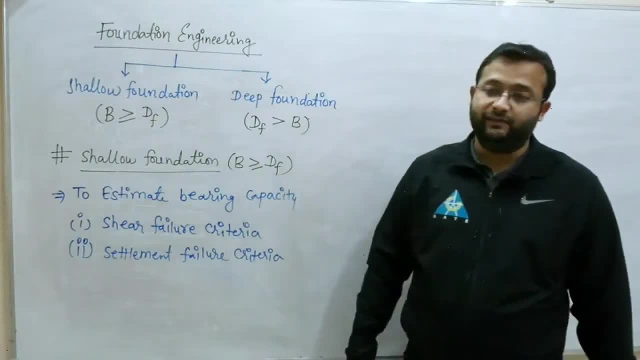 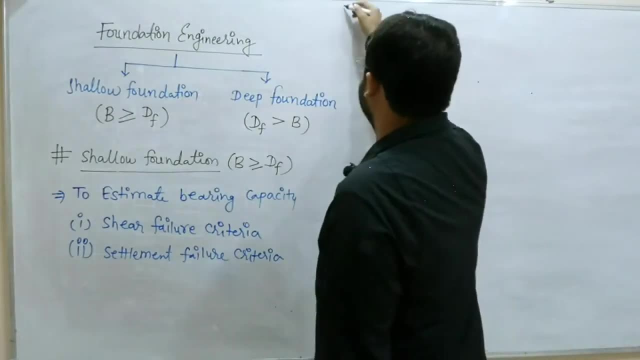 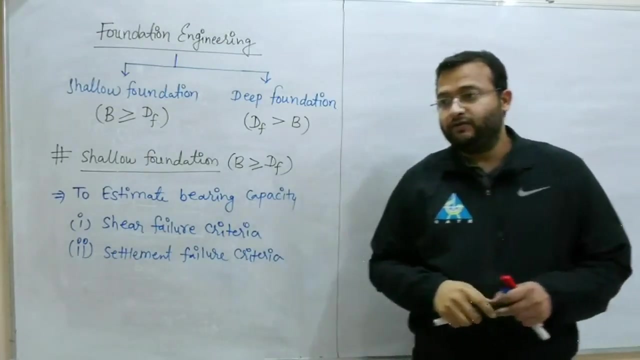 So that is based on settlement failure criteria. So we will talk about this here in the coming time. Right now, we are looking at how many types of bearing capacity can be determined. We will read that here. Right now we are looking at how many types of bearing capacity can be discussed. 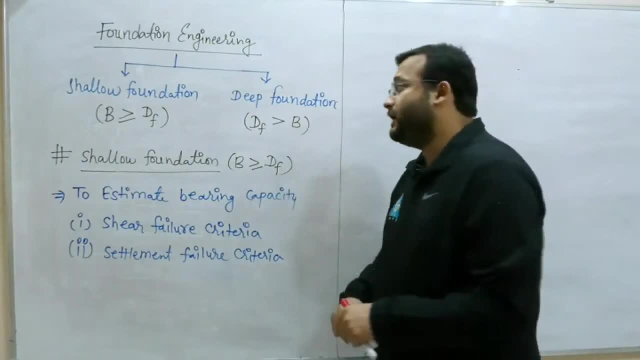 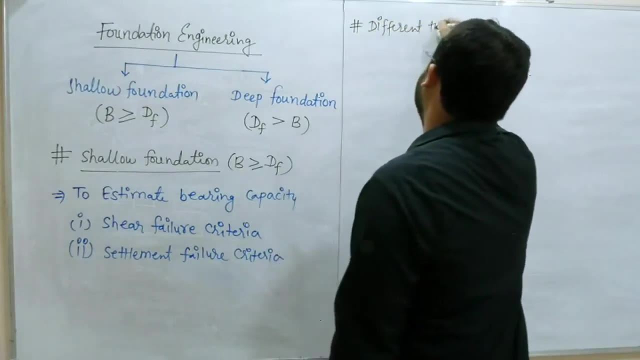 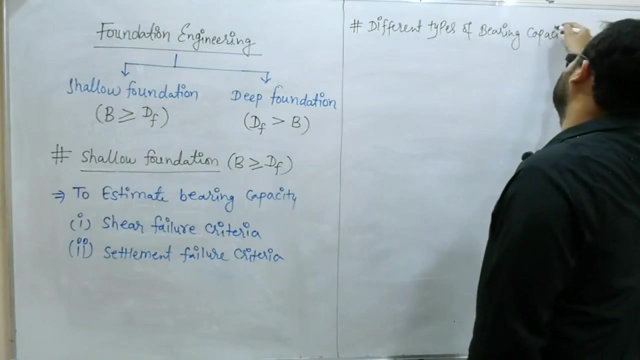 We will read that here. So first of all, I am writing the name of the topic here: Different types of bearing capacity. What am I writing? Different types of bearing capacity. Bearing capacity Now, in different types of bearing capacity. I am going to take the first type of bearing capacity. 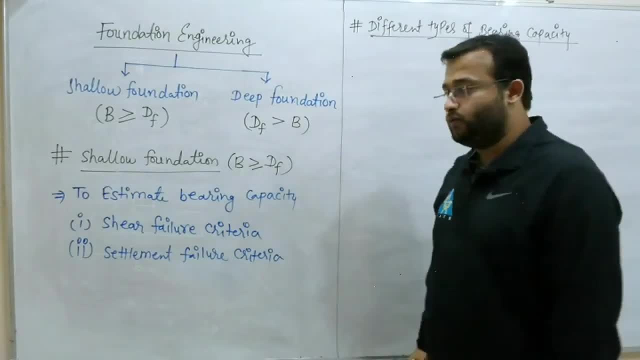 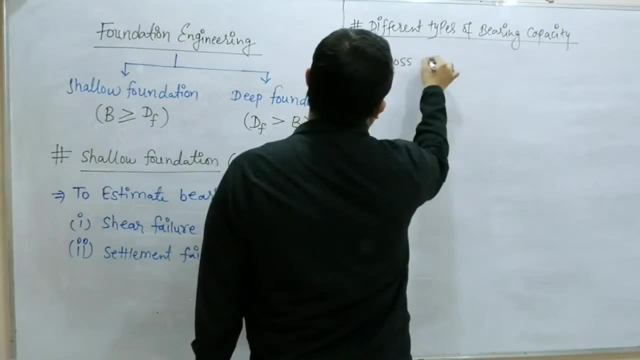 Which I will call here gross pressure. What will I call Gross pressure? So see what I have written here. I have written here gross pressure. Now let us understand what is this gross pressure. Right, Let us understand what is gross pressure. 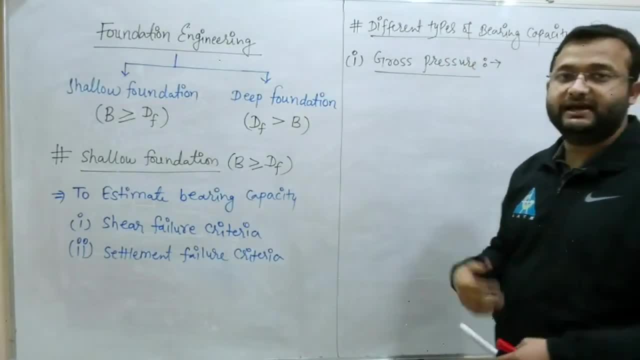 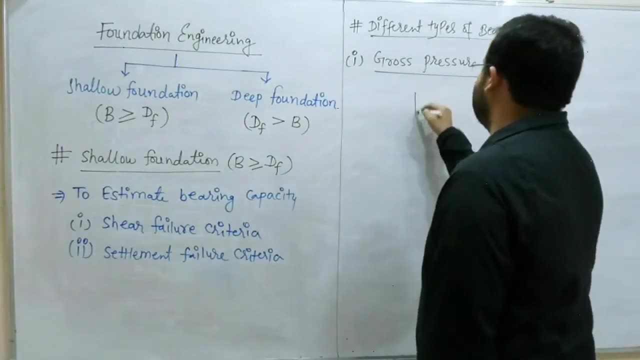 There are some definitions, There are some ways to understand it. Come, let us understand it. First comes your gross pressure. What is gross pressure? I will explain what is gross pressure? Suppose, let me assume that this is your footing. Let me assume that this is your footing. 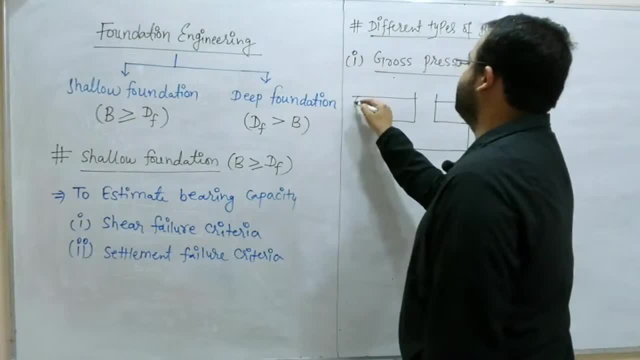 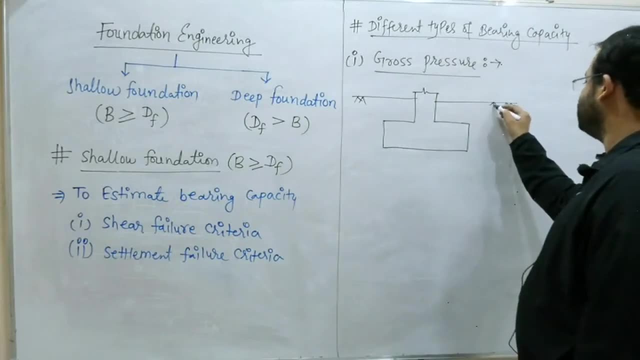 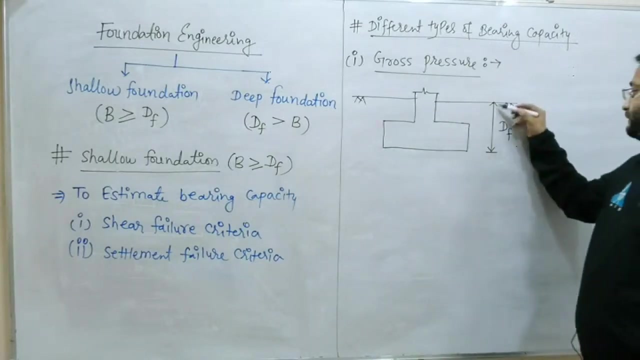 This is your ground surface, Something like this, And this column will be going upwards From this ground surface to this depth. What do we call this Depth of foundation Df? What do we call this Depth of foundation Df. 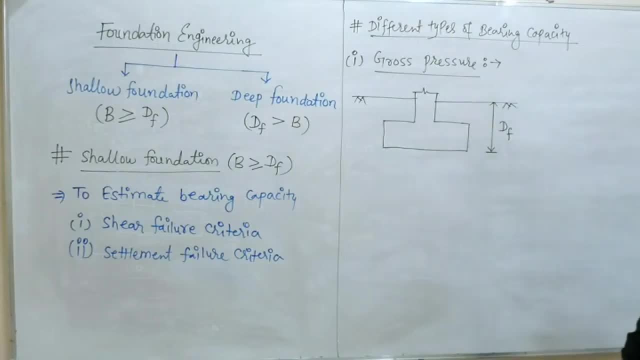 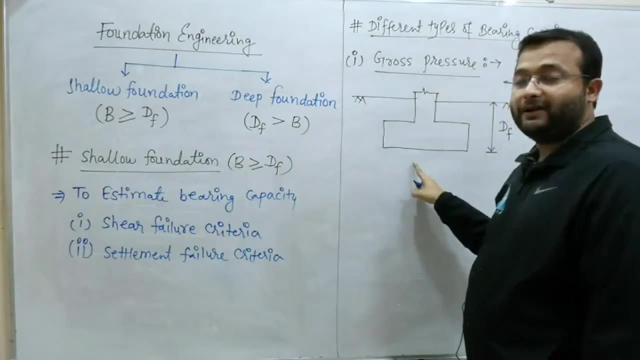 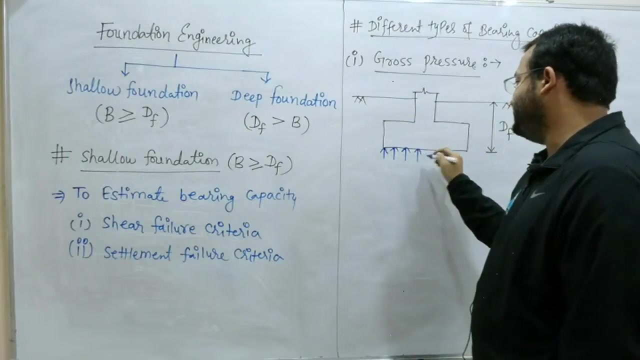 What do we call this Depth of foundation Df? This much of depth will be there. You will have made this footing in this Here. where will the gross pressure be applied? It will be applied at the base of the footing. So whatever pressure is there, we will measure at the base of the footing. 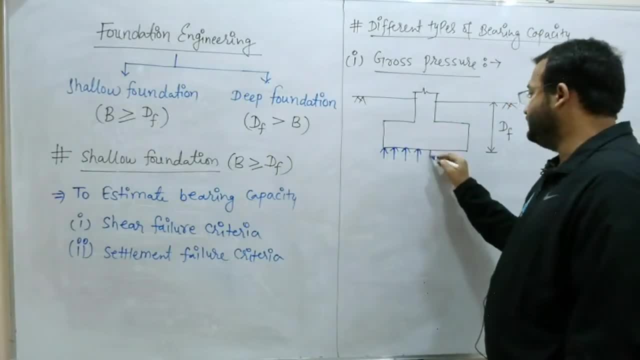 Because what is present at the base of the footing, Soil? So what is the soil applying? It is applying pressure upwards. Now, against to whom this pressure is applied? Now, it is not like that, just the soil feels like applying pressure. 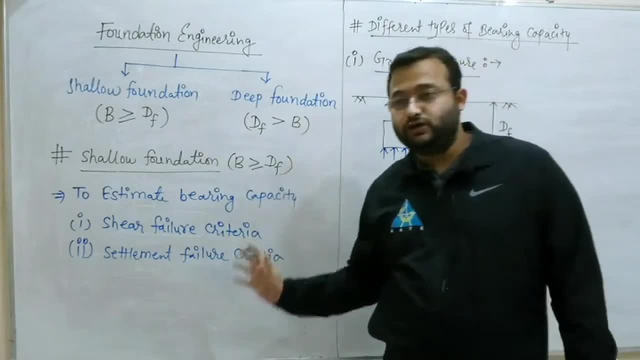 So this is how it is applied to the ground surface. It is not like that soil ka man kiya to usne, pressure lagana chalu kar diya. Issa nahi hoga. Yeh kisi cheech ke aggest lagega. 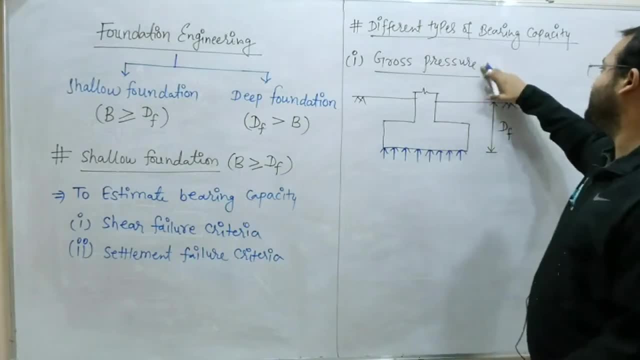 Kin cheech ke aggest lagega, wo samalna yaha par zaroori hai. Main baat aapko yaha par bata dhu ki gross pressure ko mai QG se denote kar raha hoon. 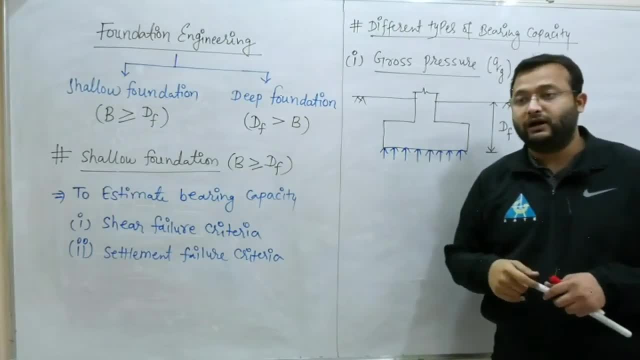 Gross pressure ko mai kisse denote kar raha hoon, QG se yaha par denote kar raha hoon, Sanway aadi meri baat. To yeh gross pressure, QG kis cheech ke aggest lagra hai? 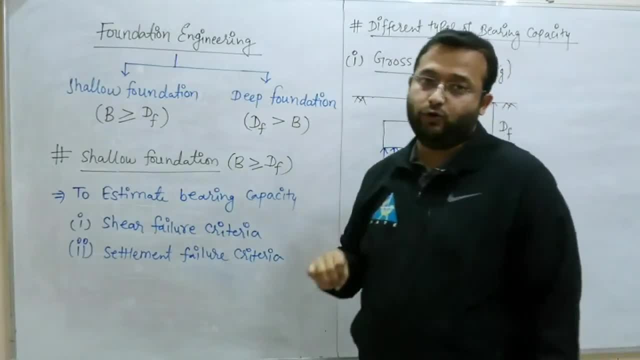 Wo janna sabse pehle zaroori hai To yeh teen cheech ke aggest lagraha hoga. Teen cheech kya hai? Woto mai yaha par batata hoon, ki gross pressure jo lagraha hai. 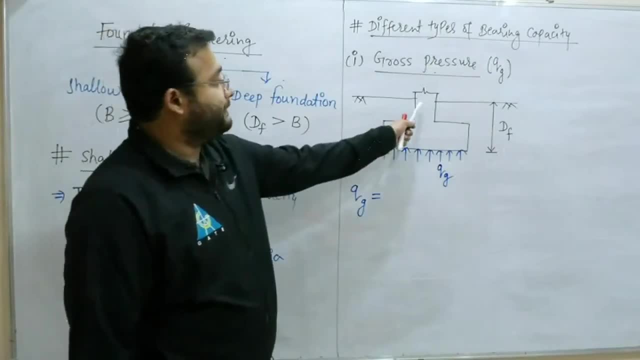 wo lagraha hai. pehla jo load aapke column se aara tha Slab ka load beam me aara tha beam ka load column me aara tha column ka khudka self weight tha wo kis me aara hai. 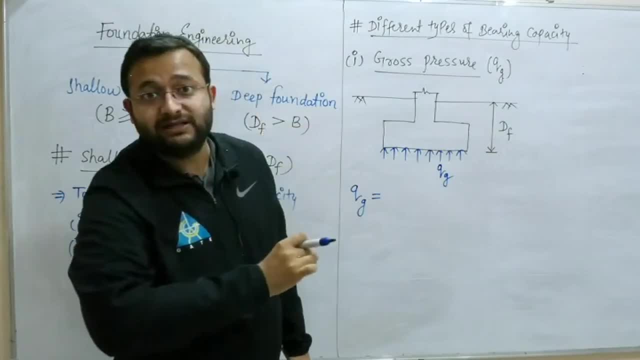 Footing me aara hai, To yeh jo total weight aara hai. no, upar se super structure, se yeh sab structure hai, wo jo super structure hai. to super structure se jo load aara hai, wo load ke aggest yeh pressure lagraha hai. 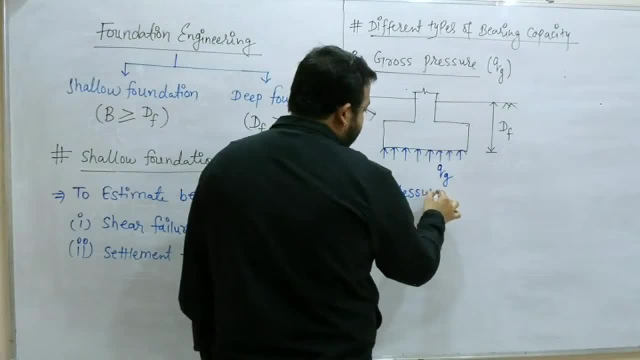 To mai likh raha hu. pressure, yeh gross pressure, kiske bana ban hai, Yeh hai pressure due to applied load. pressure due to applied load, plus yeh gross pressure, lagne ka ek karan, yeh hai. 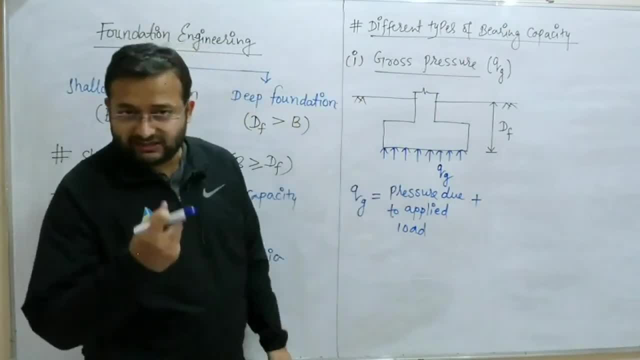 Doosra karan bhai. yeh jo footing hai. iska khudka self weight hai, uske aggest bhi lagraha hoga to gross pressure ka. jo doosra karan hai, wo hai pressure. 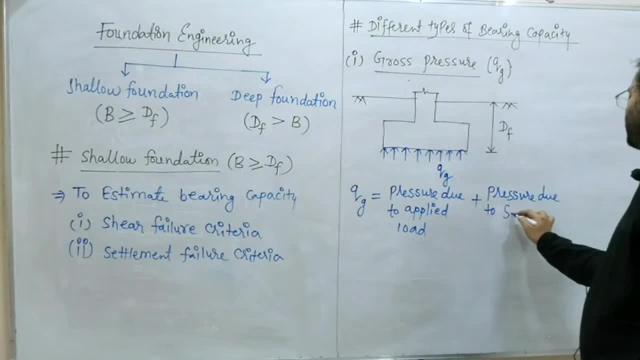 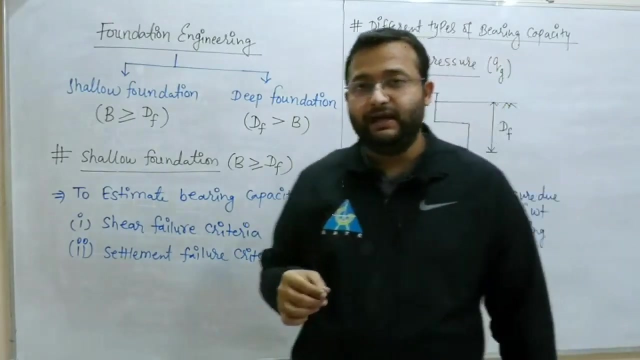 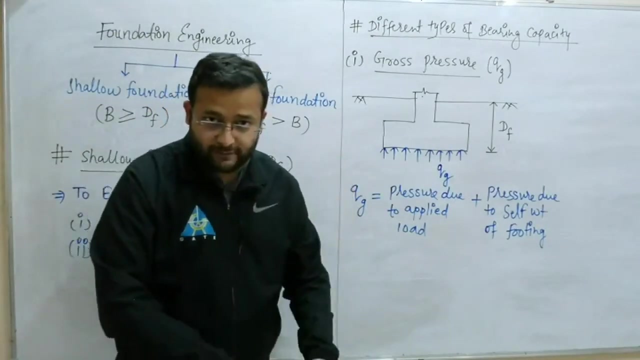 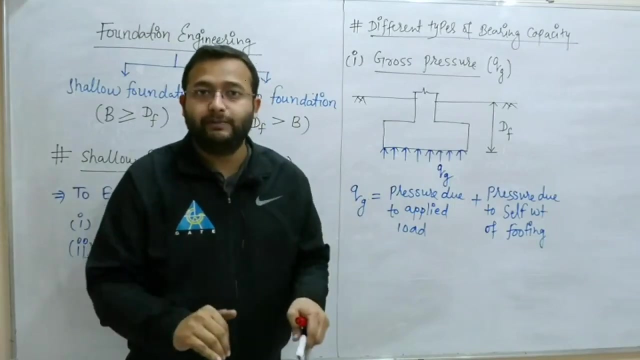 pressure due to self weight of footing. maine gaya theek hai sab self weight of footing ke karan lag gaya pressure, pressure of footing. so let any load as aound level five Excel. in physique, any physical workload would be at one time. 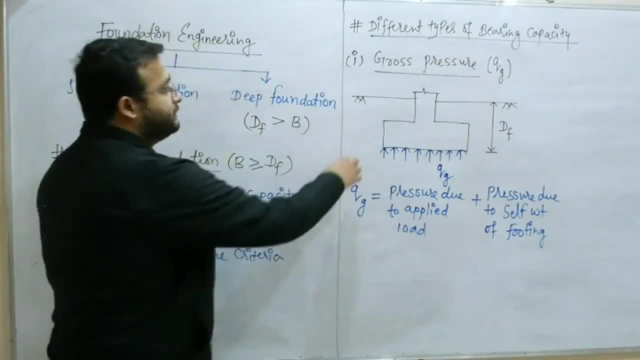 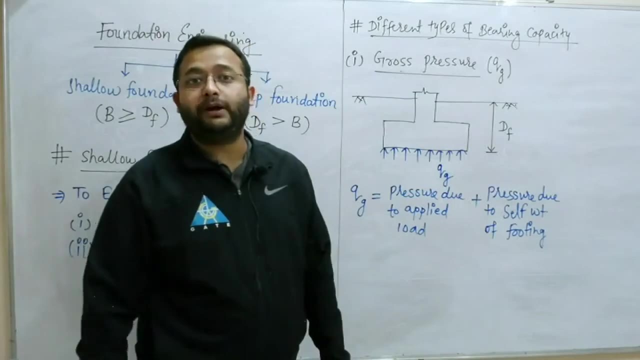 considering the way as to build foundation cost. this is basically the level. You have filled the soil again in this empty space. what will that soil also apply? It will apply pressure on the footing. do you understand? What I am trying to say is that you have filled the RCC again in the pit that you had dug. 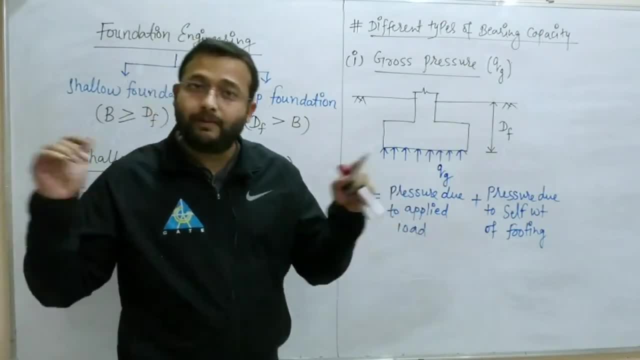 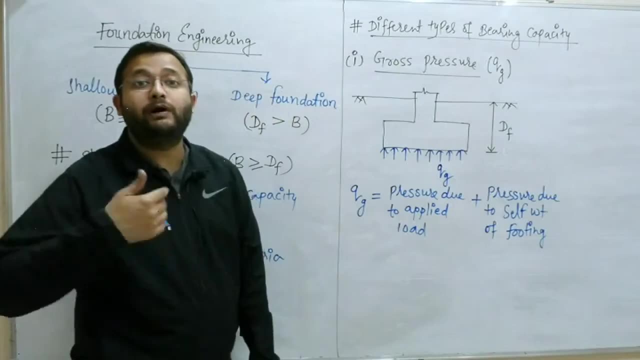 Now we will have to fill that pit again. so the soil that we had taken out, we put it back. What will this soil apply? on this footing It will apply pressure, which we will call overburden pressure. So here we are, applying plus pressure due to overburden. 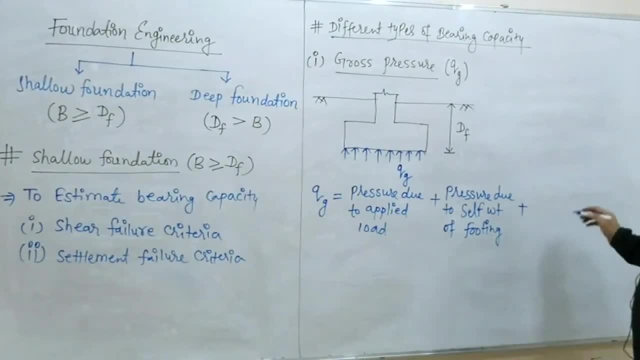 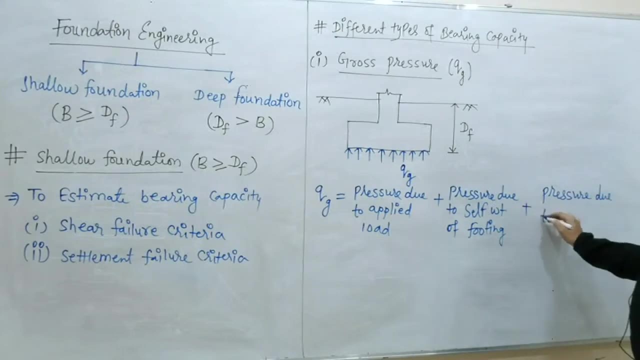 I am taking overburden here plus pressure due to overburden of soil. Ok, Pressure due to overburden of soil, So pressure is applied on this soil and the soil here on the footing If I add these three pressures. 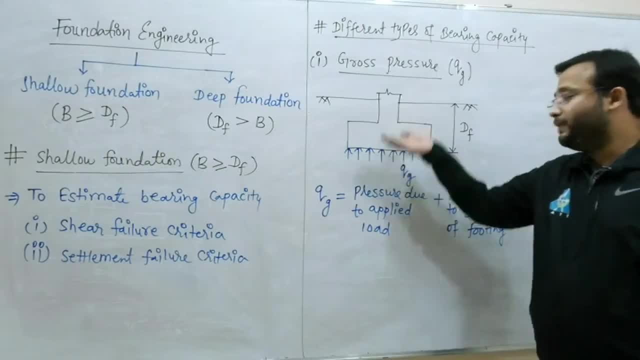 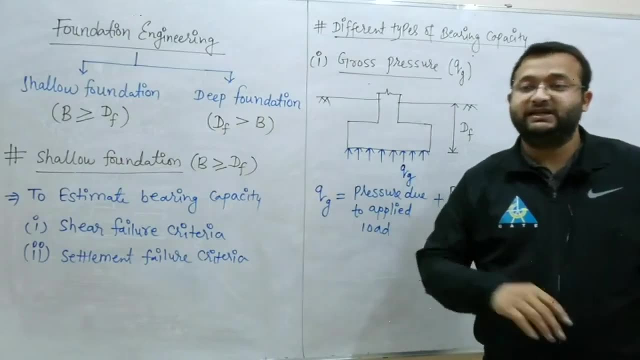 then in total the amount of pressure that soil will send is the same. So if I add these three pressures, then in total the amount of pressure that soil will send is the same. Oil will be applied on the base of the footing from the bottom to the top for an equilibrium condition, and this is called gross pressure. 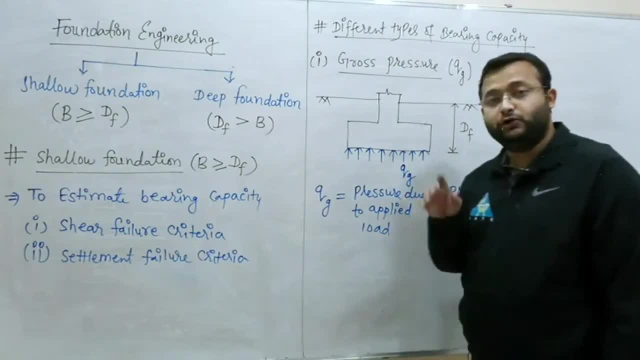 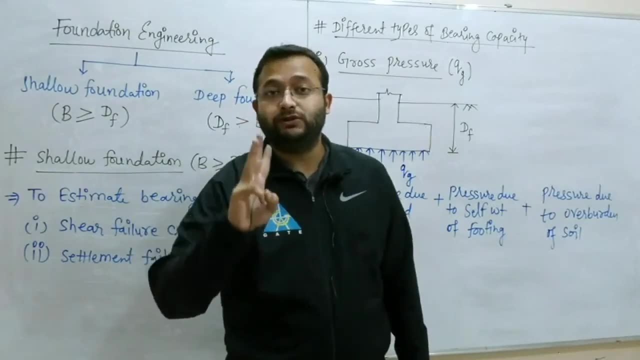 Do you understand what I am trying to say? So gross pressure is the total pressure, including all the types of loads, plus pressure due to self aid of footing, plus pressure due to overburden of soil. Is it clear so far? So this was your gross pressure. 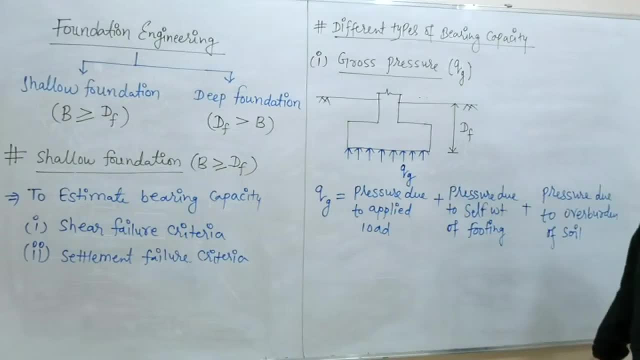 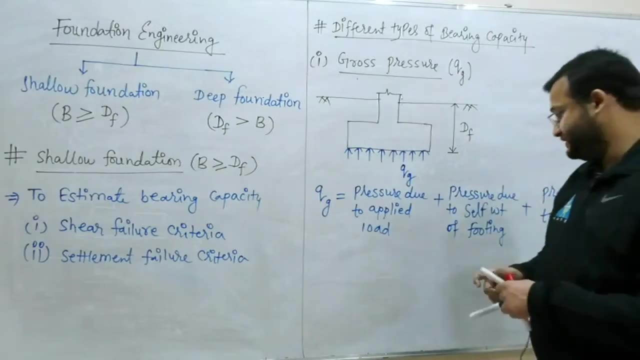 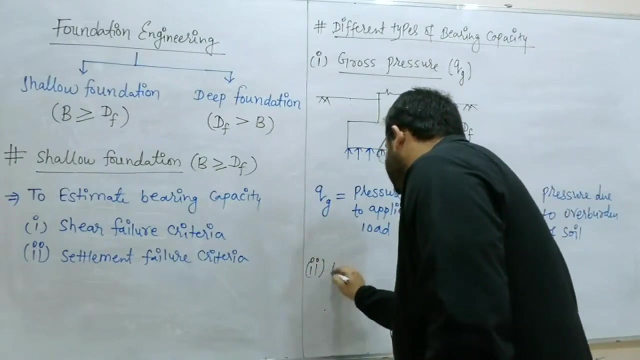 Do you understand what I am trying to say? Yes, sir, we are completely clear about this. I told you that. if this is clear, then I will tell you the next thing, and that is related to your net pressure. Here I am telling you that next, we have net pressure, net pressure, net pressure. 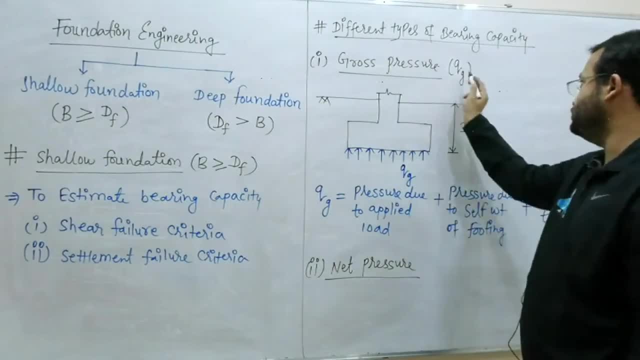 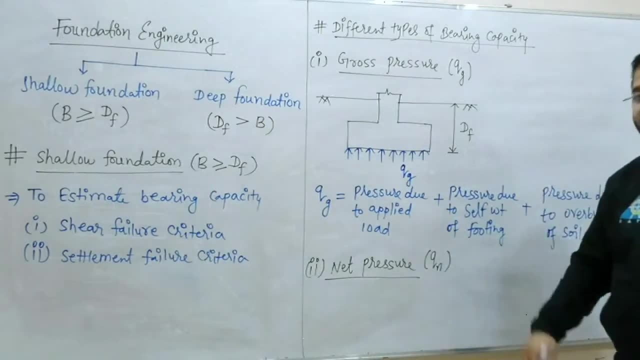 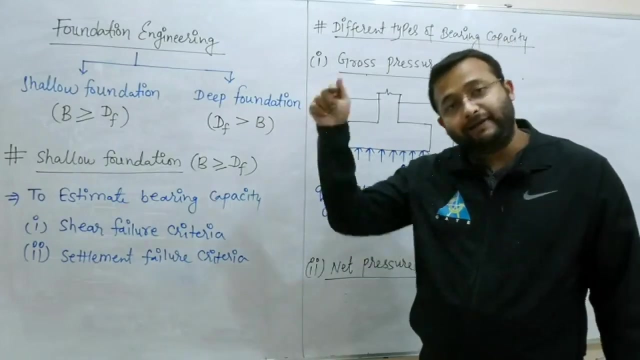 Just like I had gross pressure and I denoted it as Qg, so I denoted net pressure as Qn. Now, what is Qn? Qn is that pressure on the base of the footing in which we have considered pressure due to applied load and pressure due to self aid of footing. 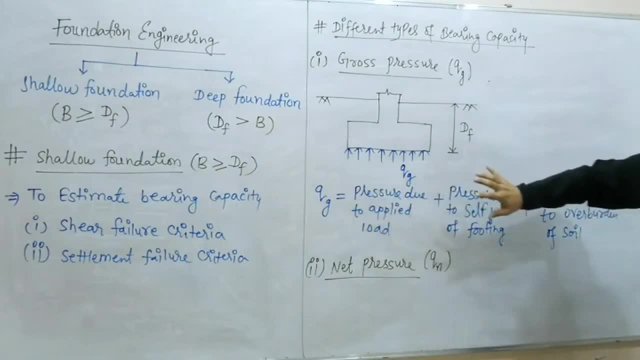 Means I have considered pressure due to this and pressure due to this. If I consider pressure due to these two, then we will call this pressure as net pressure. That means what we are doing with this pressure. We are not considering overburden pressure in estimating the net pressure. 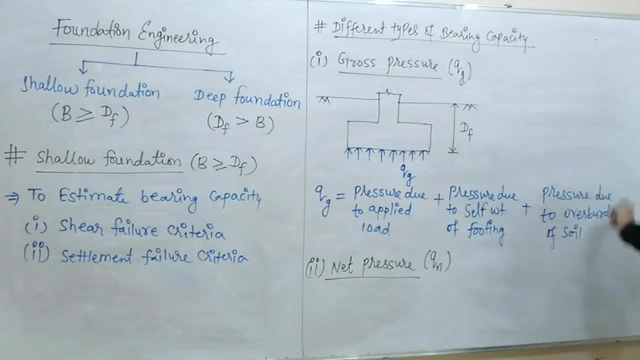 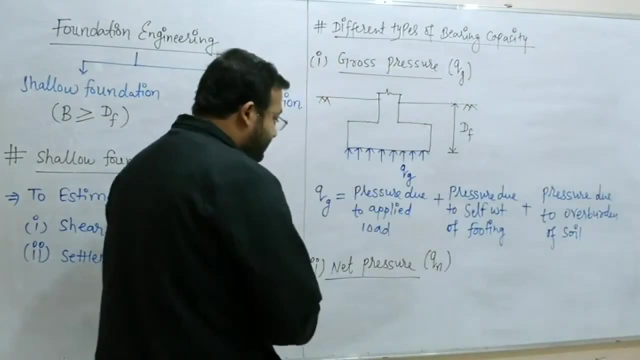 Are you getting my point? So we are not considering this overburden pressure in the net pressure. So what did we do here? We have written here: Okay, what did I say? The sum of these two will be net pressure. 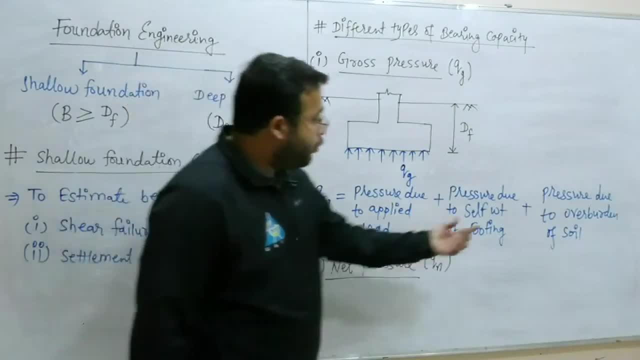 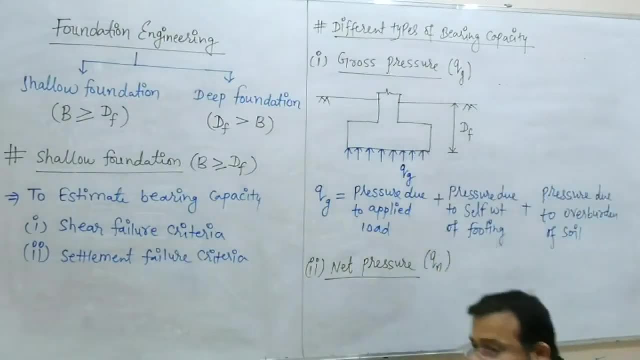 So can I write that if we minus overburden pressure from Qg, then we will get net pressure. So I will write it here. Brother, you do one thing, You do one thing. What will happen to your net pressure? 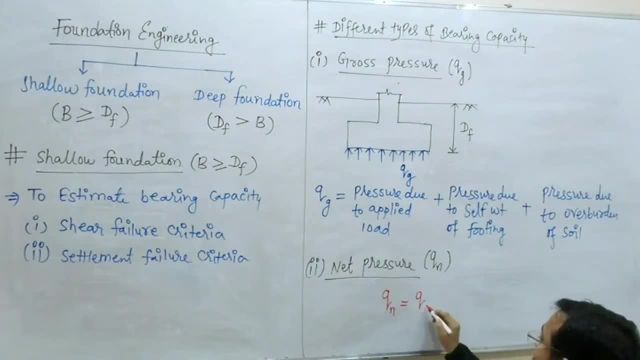 Your Qg which is coming: gross pressure. What is there in this gross pressure, In this gross pressure? pressure due to applied load, pressure due to self aid of footing and pressure due to overburden. We do not need overburden pressure in net pressure. 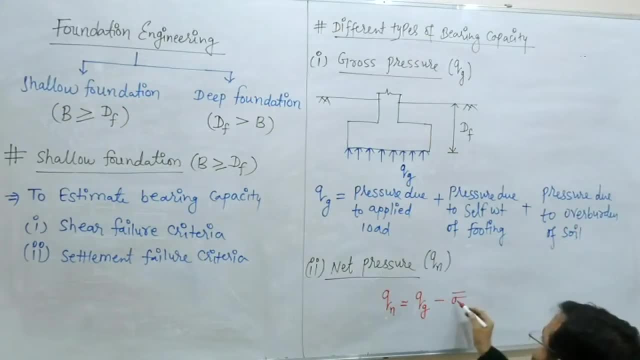 So what can I do? I will minus it here. and I am denoting the overburden pressure from sigma bar. What am I doing here? I am denoting it from sigma bar, So sigma bar is the overburden pressure. 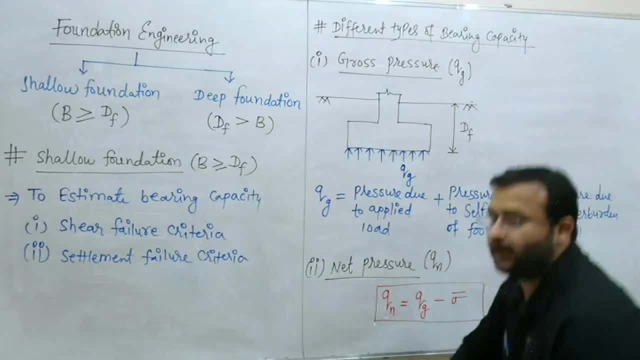 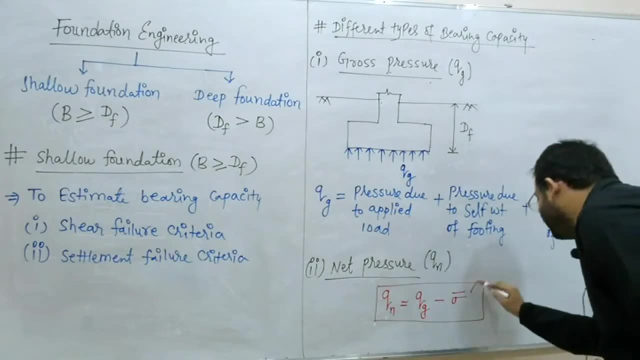 So if you minus overburden pressure from gross pressure, then what will you get? You will get net pressure. So, sir, what is the value of sigma bar? So what is this sigma bar? This is your overburden. 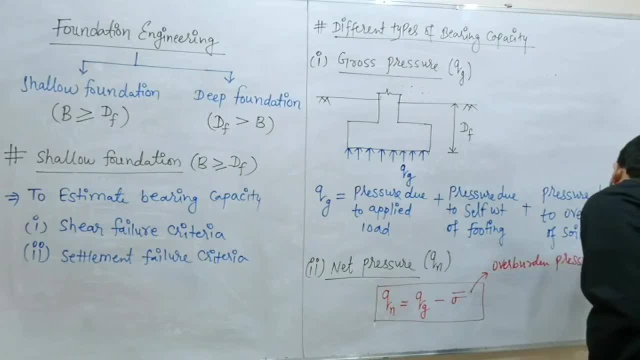 This is your overburden pressure. Now, if you ask me what is the value of this, then I will write: sigma bar is equal to effective stress. And brother, what is sigma bar? It is one type of effective stress. I will write the unit weight of this soil here as gamma. 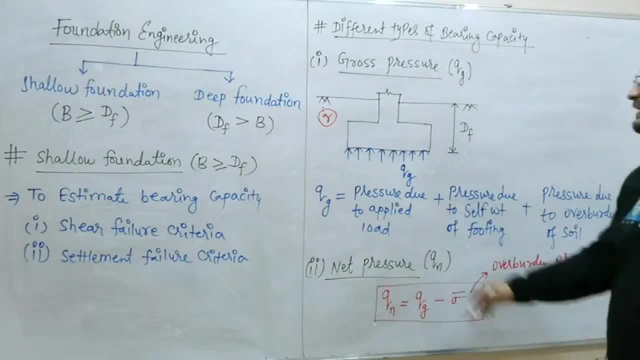 The unit weight of this soil here is gamma. So what will be the value of sigma? bar Gamma into Df? The discussion is over. So what did you get Gamma into Df? The discussion is over. When did this happen? 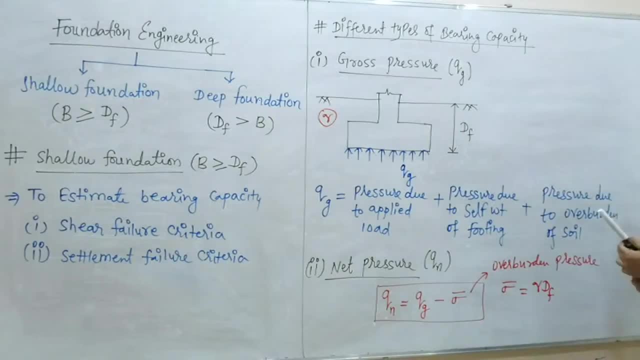 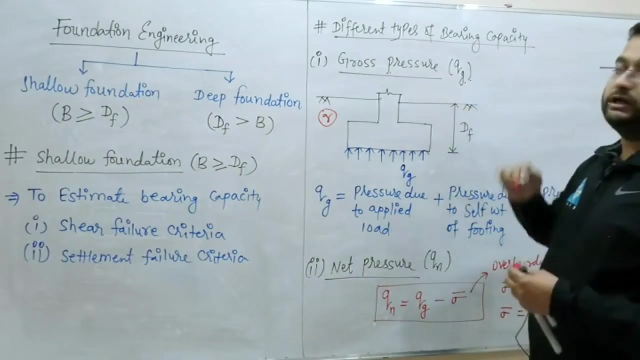 When there was no water table. You did not have a water table. So here you can write: no water table, No water table. Then you would have got this value If you have a water table on the ground surface. I assume that suppose there is a water table on this level. 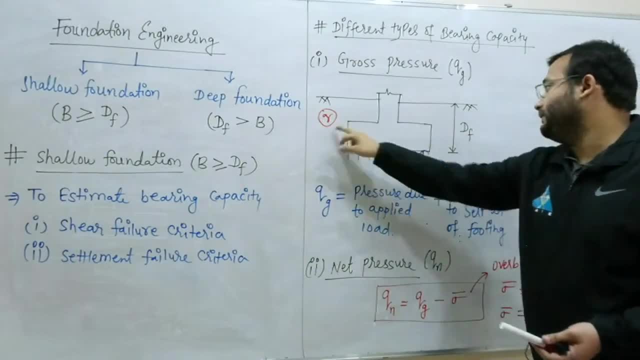 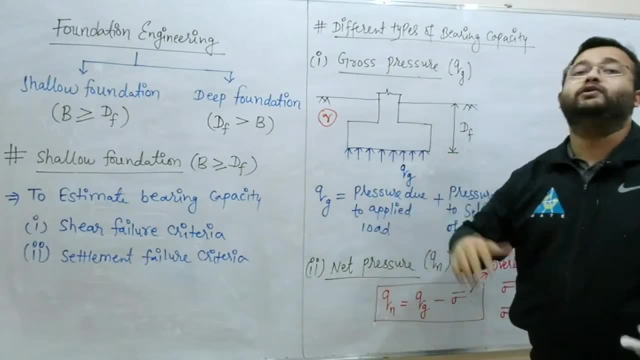 So what will become of this? gamma Gamma submerged, So total stress gamma into Df, Total stress minus gamma w into Df Poor water pressure, So total stress minus poor water pressure, Gamma saturated minus gamma w. What will become? 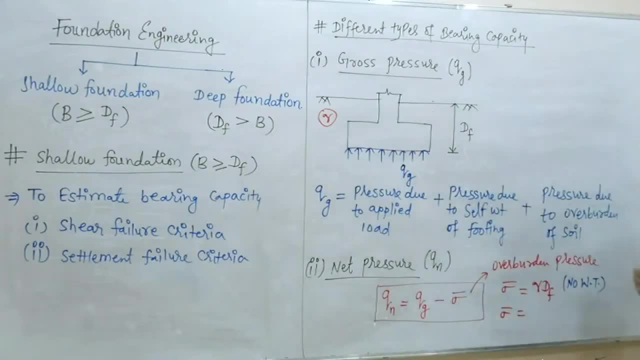 Gamma submerged. So gamma submerged Df will become when the water table will be present. So here I have written gamma submerged into Df. So what has become When you will have a water table present at that time? That means when the fully submerged condition is present. 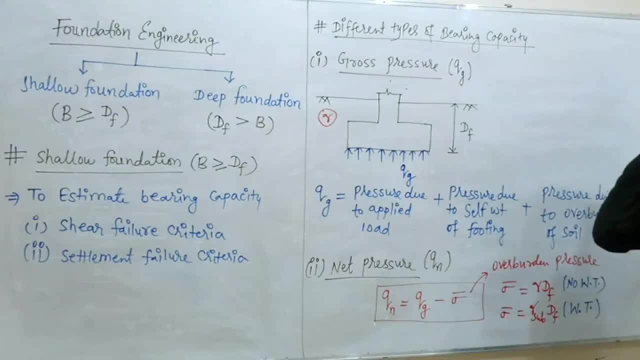 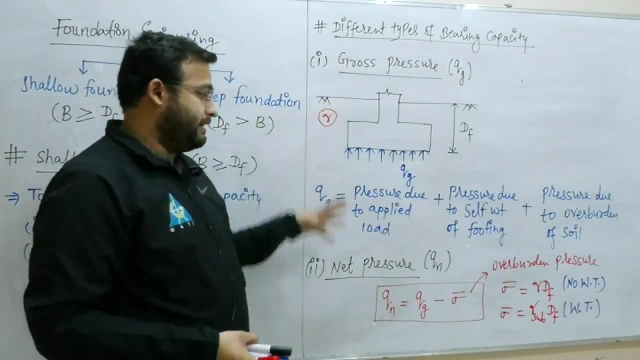 Then this one will become. So what types of bearing capacities have I told you till now? I have told you two types. One, I told you, is gross pressure. I told you, is net pressure. Are you listening to me? Are you listening to me? What am I saying? 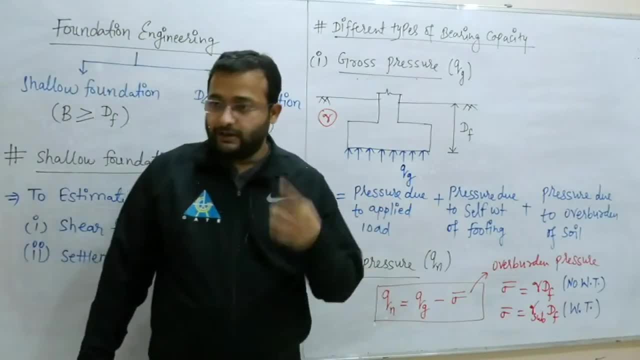 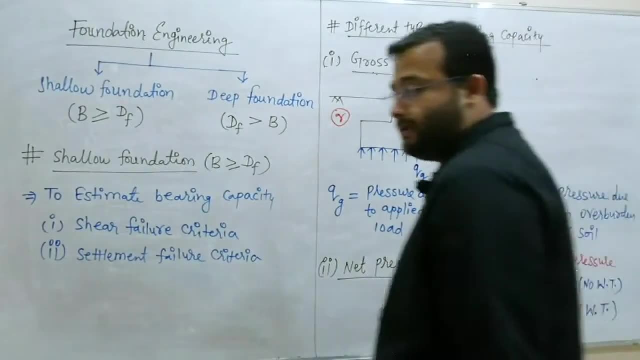 So one is your gross pressure, One is your net pressure. I am giving you to take a photo. I am moving away from the middle. Those of you who are going to take a screenshot Take a screenshot, And those who want to take a photo. 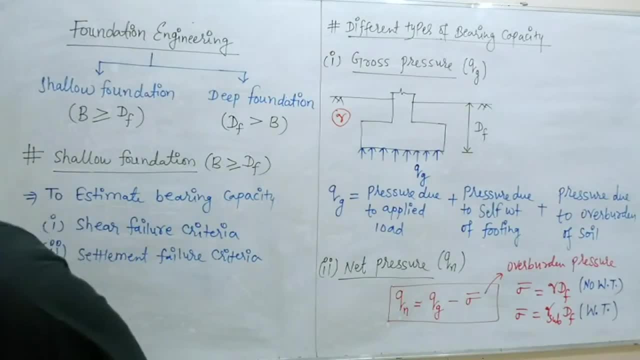 They will quickly take a photo And all of you will share it at once. Right, All of you will share it at once Because foundation engineering is an important topic. What is foundation engineering? It is a very important topic. Many times, 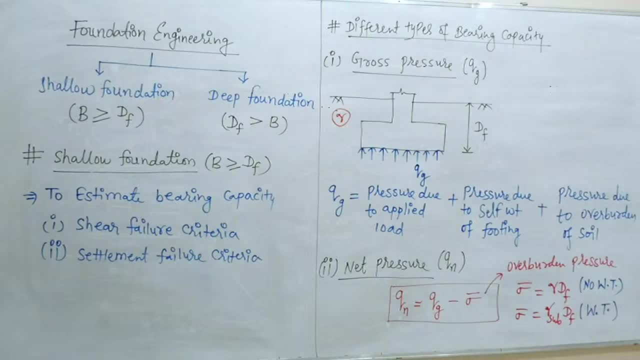 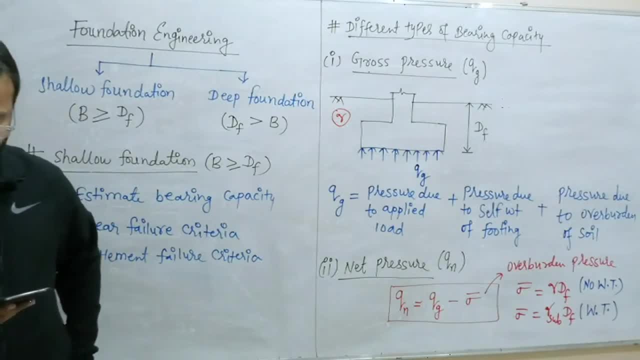 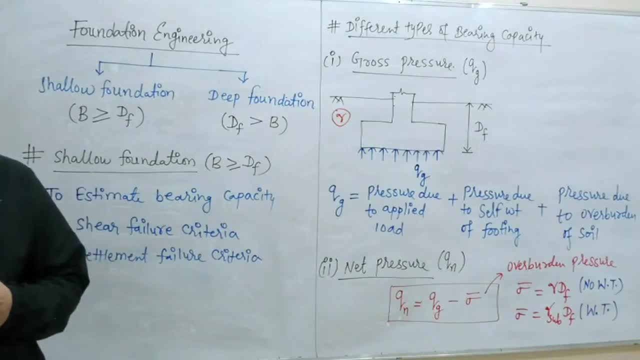 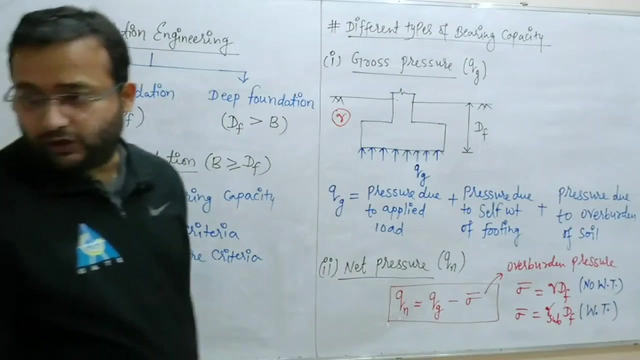 Chalo mene share kar diya hai. sabi ne photo le liya hai. sabi ne photo le liya hai, sabi ne screen shot le liya hai. jisko jo jo lena tha sab le chuka hai. chaliye aage badte hain. 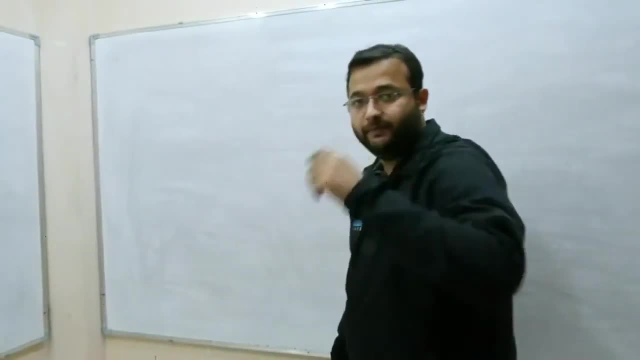 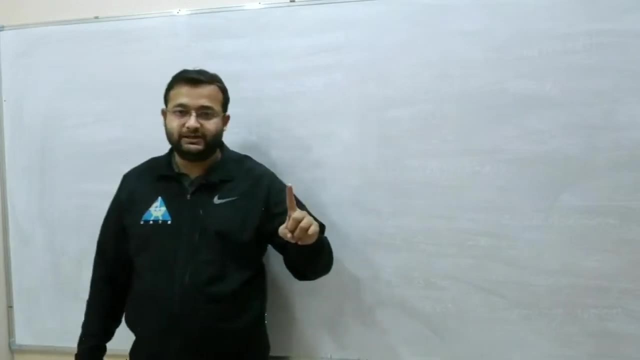 aage badte hain. hum log yaha par aaiye. mai aapko batata hu, iske aage ke bearing capacity is Abhi tak humne gross pressure dekh liya. Hai na Hum log ne gross pressure dekh liya. 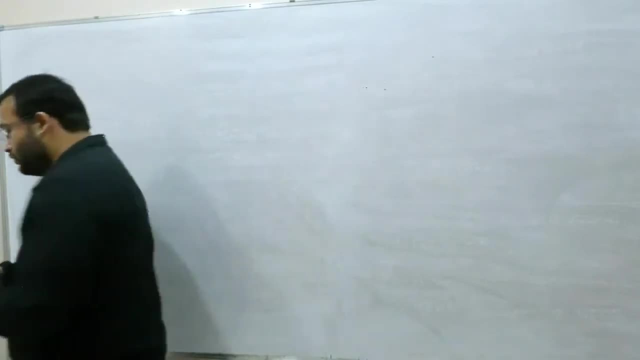 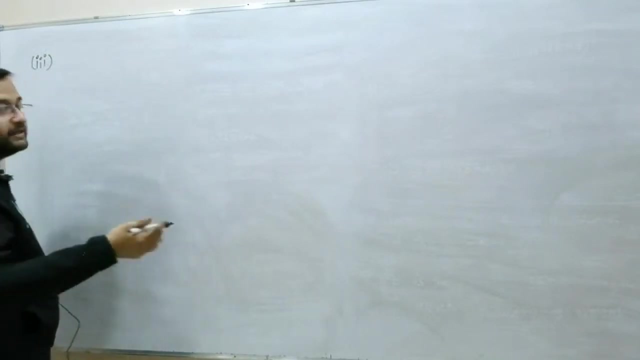 Hum log ne net pressure dekh liya. Next me aap log ko batata raha hu ultimate bearing capacity. Next me aap log ko batata raha hu: next type ka. jo humar apas bearing capacity hai, usko hum kahenge ultimate bearing capacity. 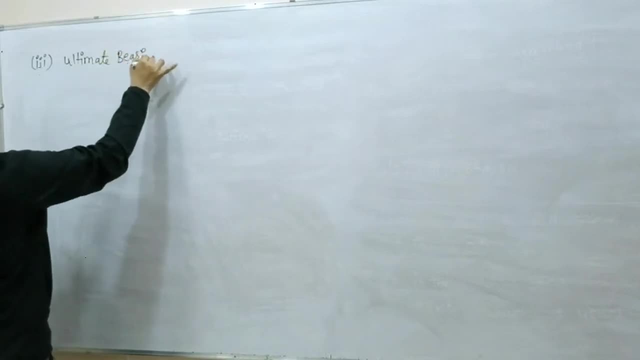 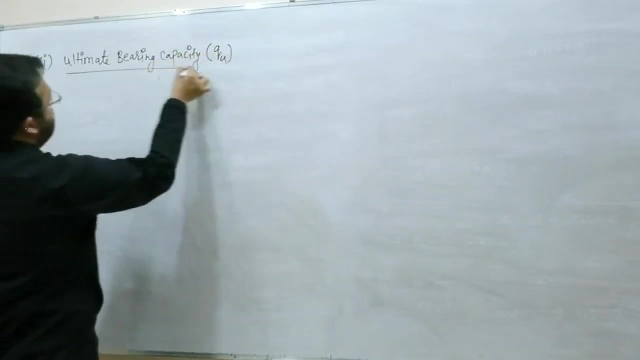 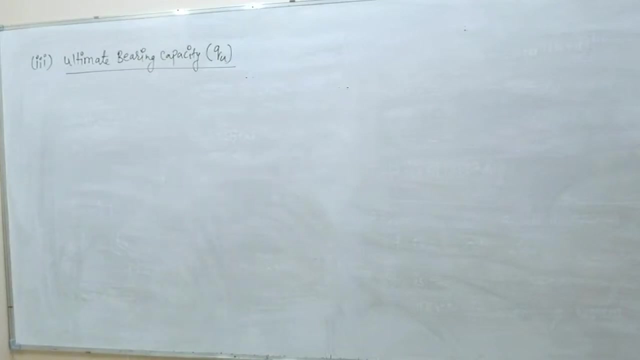 Ultimate bearing capacity. Theek hai Isko hum kise denote karenge. QU se denote karenge Abhi ultimate bearing capacity? kya cheez hai, sir, Main ka aaiye hum isko Samasta hai, What is ultimate bearing capacity? 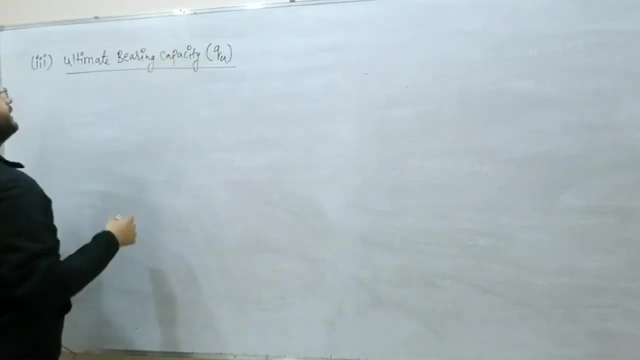 Toh main aap par aapko hi batata raha tha ultimate bearing capacity QU ke baara mein. Main ultimate bearing capacity QU ke baara mein batata raha tha, Pera mai iska chota sa definition likh deta hu. 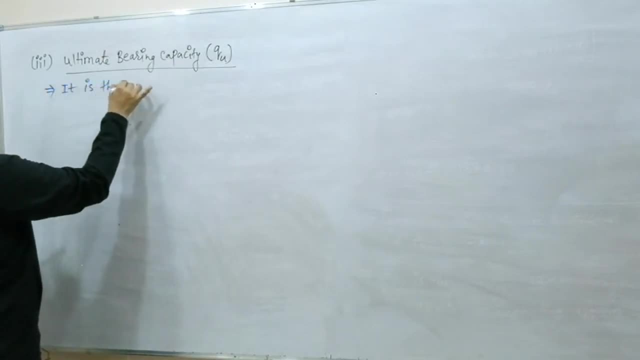 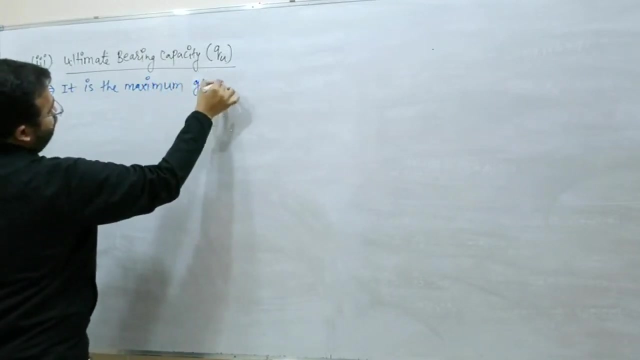 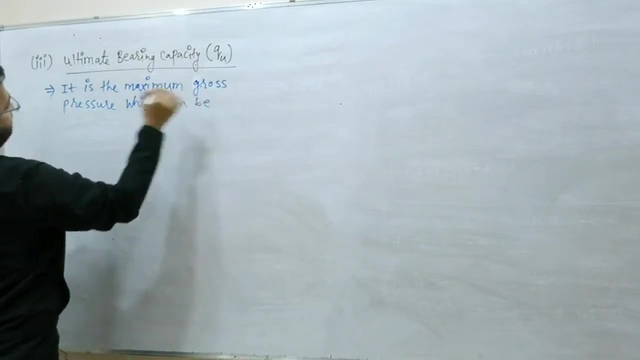 Ki. it is the maximum gross pressure. It is the maximum gross pressure, Maximum gross pressure Which can be applied, Which can be applied At the base of footing, At the base of footing, Without shear failure. Hai na At the base of footing. 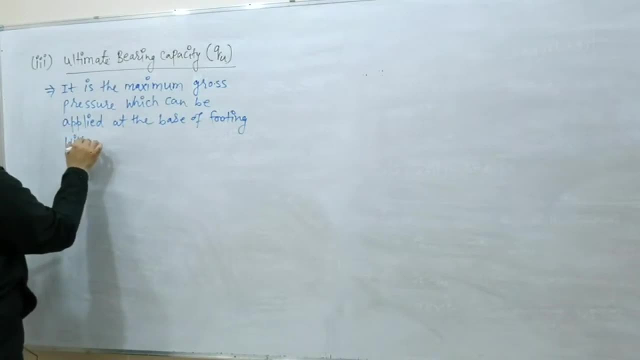 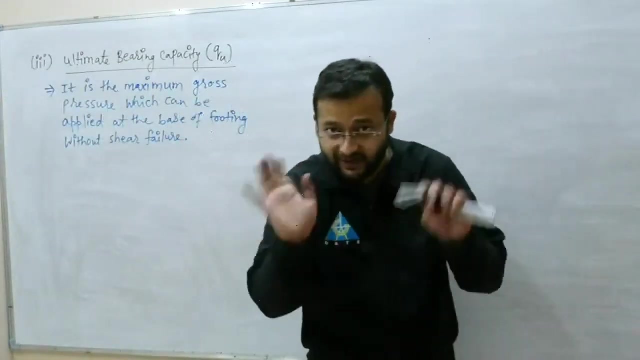 Without shear failure. Without shear failure, Sir, maari maari baat, kya bula cha raha hu main. So it is the maximum gross pressure Jo ki aap base of footing par laga sakte hai, Aur shear failure tab bhi nahi hoga. 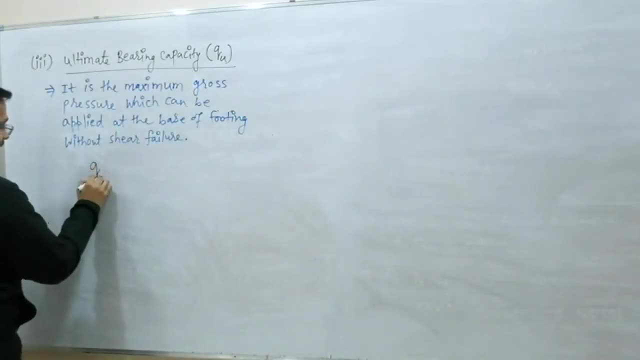 Kere ka matlab. ye hai ki dekho, Ye hai aapka ultimate bearing capacity, Which is your maximum gross pressure. Aur abhi thur day pehle hi mai aapko gross pressure padhaya hu. The maximum value of gross pressure is your ultimate capacity. 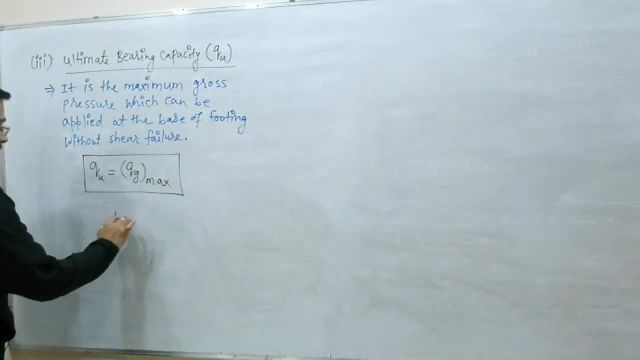 Abh, meri baat ko samalne ki koshish kariyega, mai kya batana chaara hu. Mene kaha ki mere paas ye kya hai footing hai. Mene kaha ki mere paas ye kya hai footing hai. 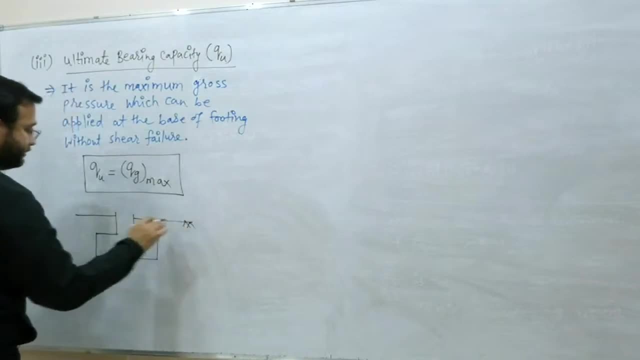 Mene kaha, ki meri paas ye kya hai footing hai. Yes, sir, footing hai. Abhis footing par yaha, par hamar paas kya hai Gross pressure lag raha hai. abhi gross pressure ke andar kya kya shamil hai. 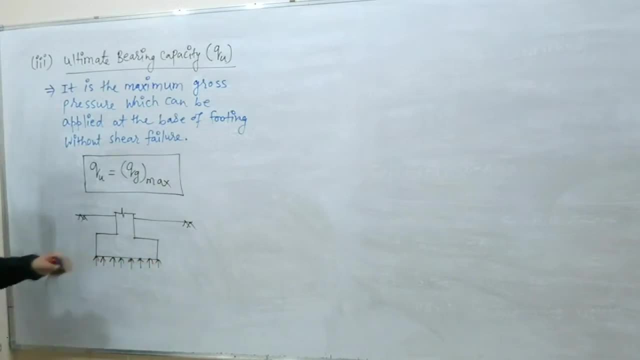 Bhai, yadi mai bol rahun ki yaha par gross pressure lag raha hai. To his gross pressure ke naiche kya, kya shamil hai His gross pressure mai apka self-fador footing shamil hai, Applied load shamil hai. 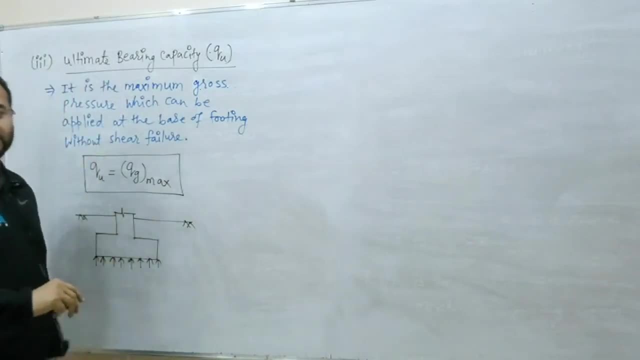 Aur over burden of soil. Tinu shamil hai his gross pressure me Abh kaha that how much pressure was coming due to your load. how much pressure was coming due to your self-fit of footing? how much pressure was coming due to your over-bodying of soil? 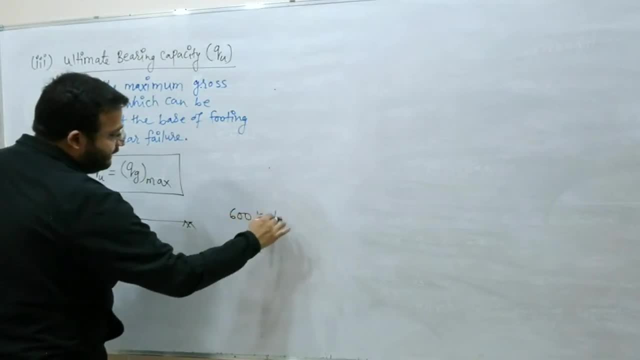 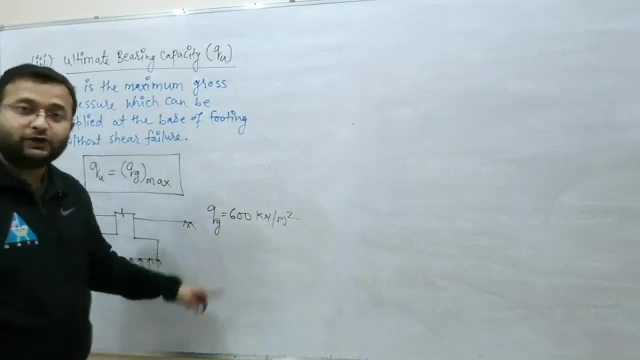 then I came to know that the total gross pressure that is coming, that is coming QG, equal to 600 kt per m2.. This gross pressure is coming in total. Can my soil take this much pressure or not? I don't care how much gross pressure is coming. 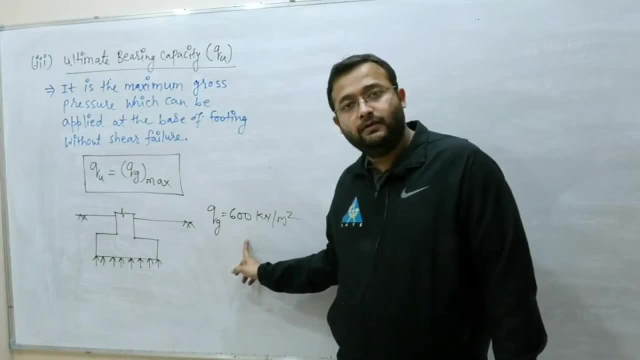 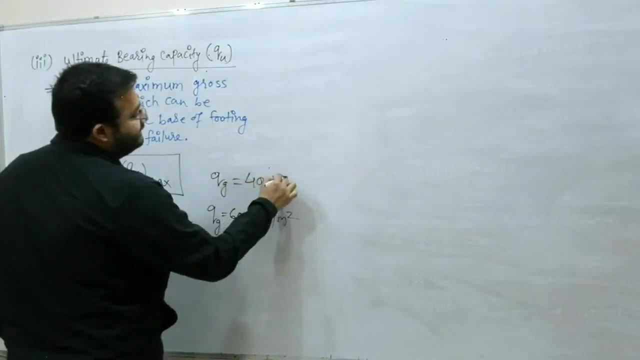 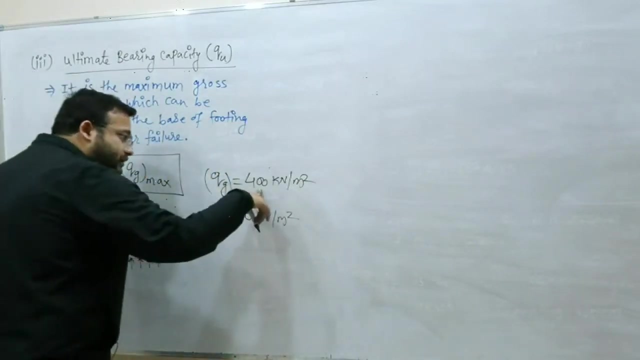 Can my soil take this much pressure or not? So I saw that no, my soil is not taking this much pressure. The maximum gross that my soil can take is 400 kt per m2 only, So this maximum value of gross pressure on which soil is safe. 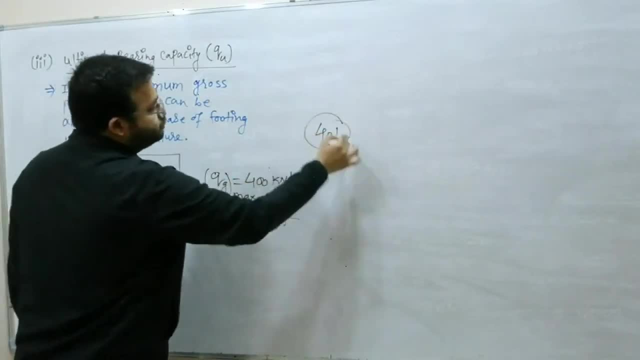 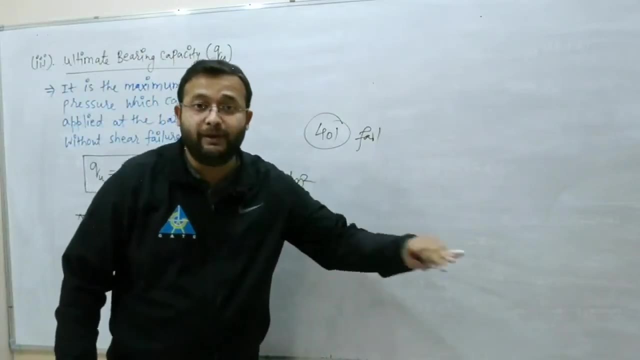 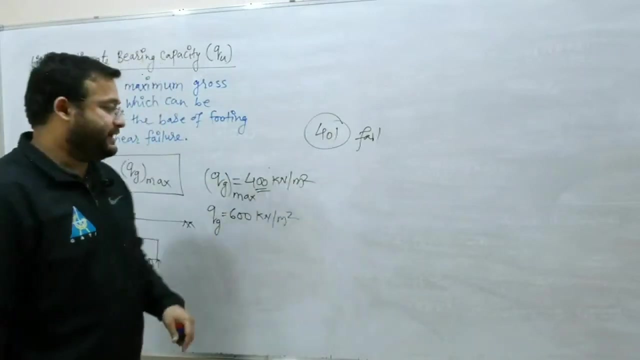 your soil is safe till 400,. you applied 401, soil came here and failed. means 400. is that value? that maximum gross pressure is there till where your soil will remain safe? There will be no shearing in the soil. So what will be your maximum gross pressure? 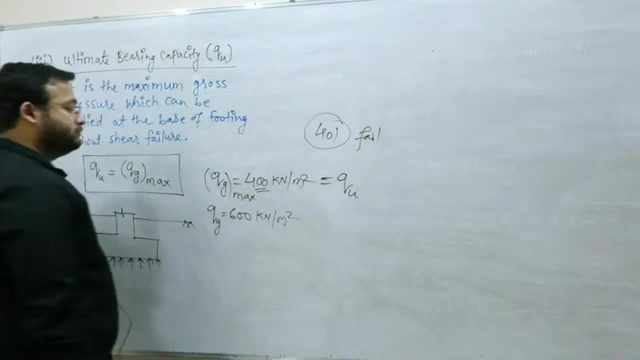 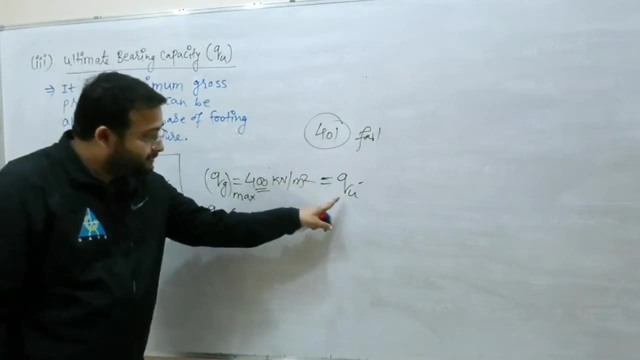 Ultimate bearing capacity will be called QU. So you are understanding the difference between QU and QG. Both are gross pressures. Ultimate bearing capacity is also one type of gross pressure and gross pressure is also gross pressure. This also considers your self-fit of footing. 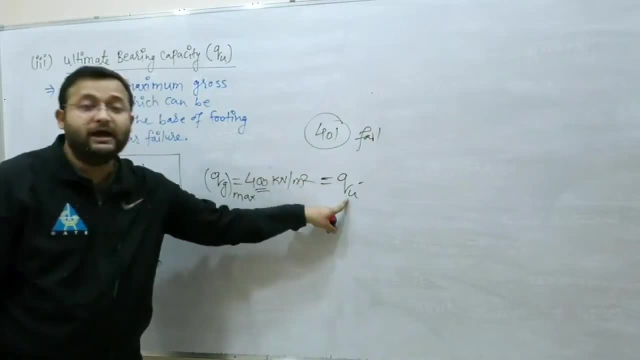 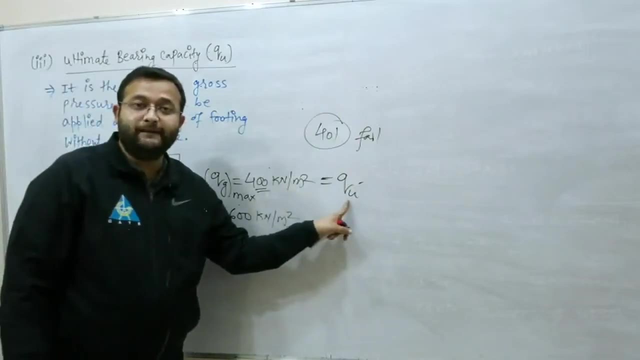 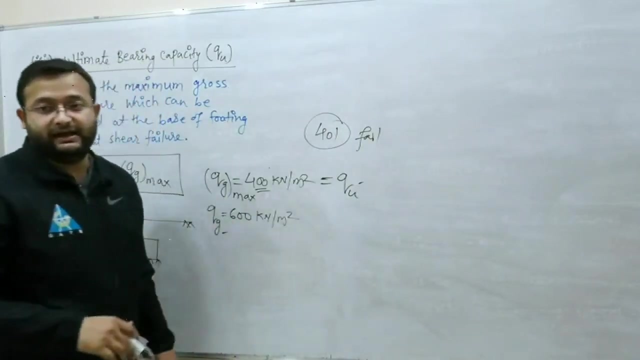 this also considers your total applied load coming from columns. this also considers your over-bodying pressure. But what is the difference between these two? The difference between these two is that this is the gross pressure till where the soil can remain safe, And this is the gross pressure which is telling your total value. 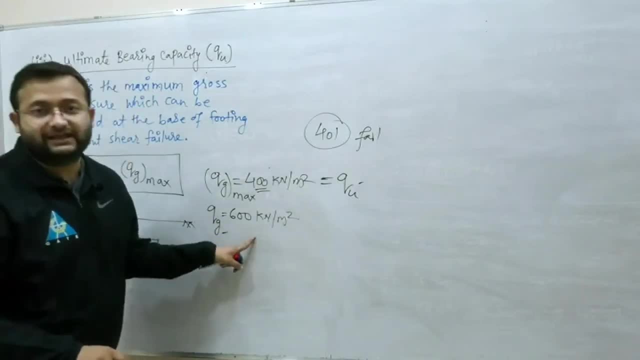 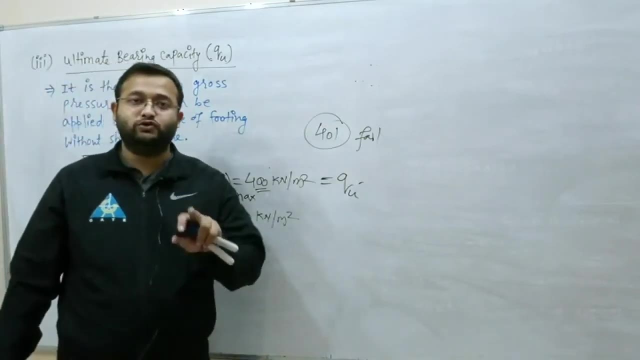 Now here. it is possible that the soil is safe or not. I will not be able to understand that. Do you understand what I am saying? So ultimate capacity is that maximum gross pressure till where your soil is not shearing. I have clearly written this here and I have also told it here. 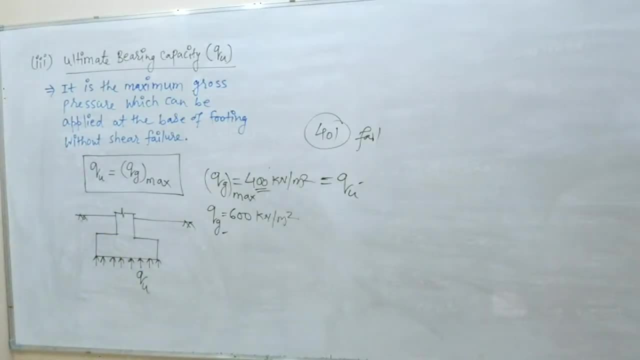 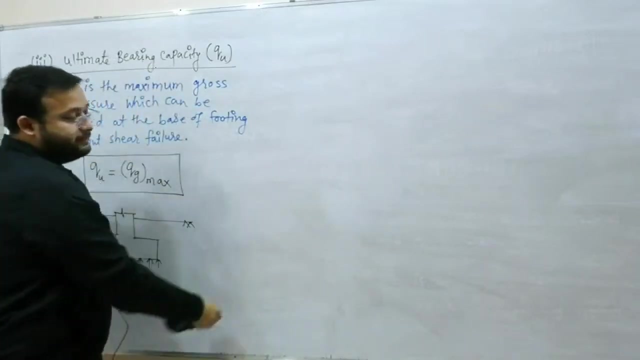 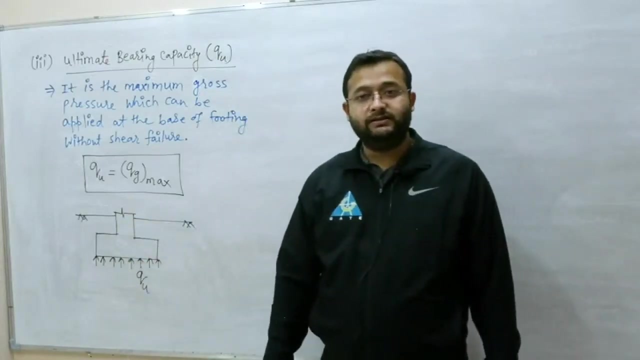 So what will be your maximum gross pressure bearing capacity? Definitely, this bearing capacity, this bearing capacity of yours, where is it being applied? This bearing capacity of yours is being applied on the base of the footing. Please listen to my third point. 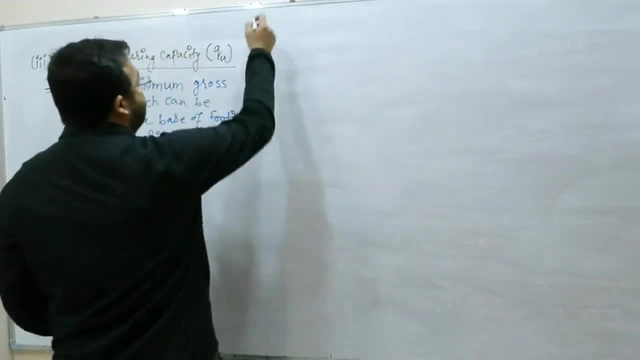 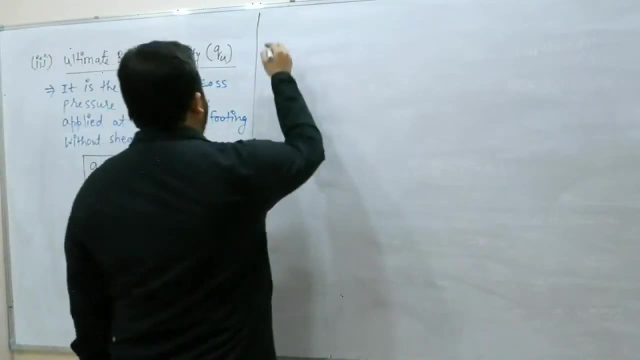 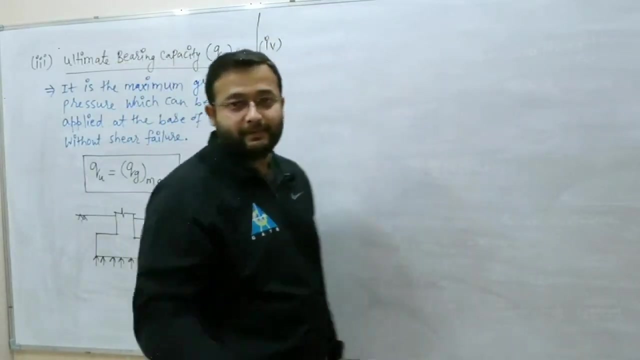 on the base of the footing. Let us move ahead. This was my third type of bearing capacity. Let us see the fourth type of bearing capacity. I am looking at the fourth type of bearing capacity here. What am I looking at? the fourth type of bearing capacity. 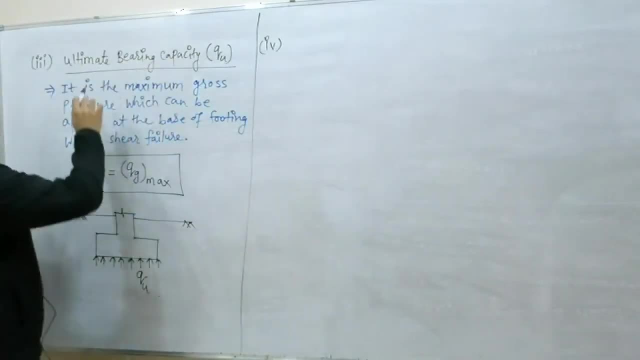 Its name is like I had gross pressure, like I had gross pressure. so what did I get out of gross pressure? I got out the net pressure. Now what do I have? Ultimate bearing capacity. So what can I get out? Net ultimate bearing capacity. 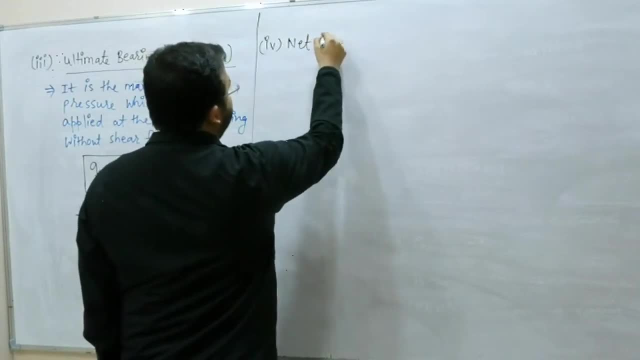 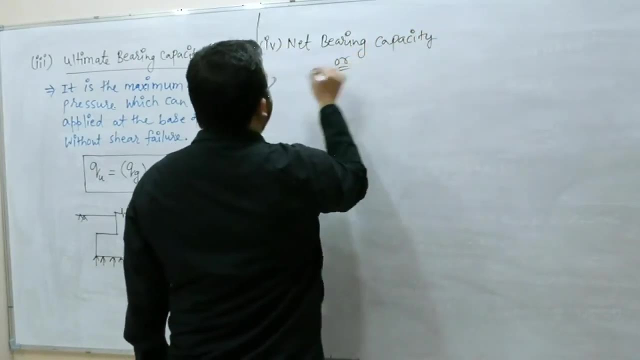 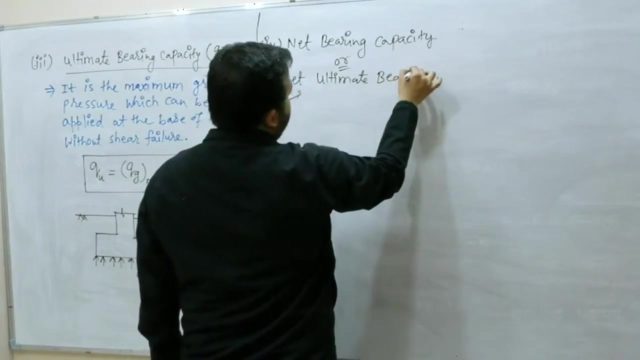 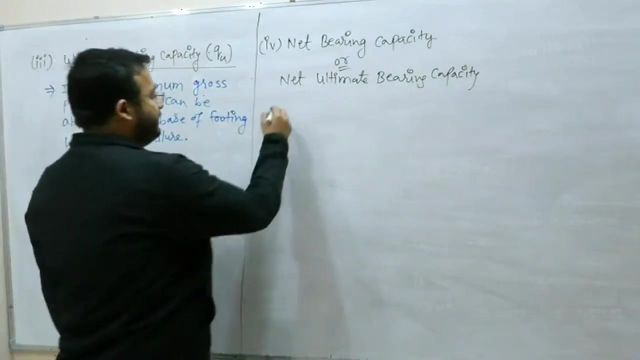 So what am I getting out here? Net bearing capacity- You write net bearing capacity, Or you can write net ultimate bearing capacity, Net ultimate bearing capacity. If you want, you can write it, No problem. We will denote this by QNU. 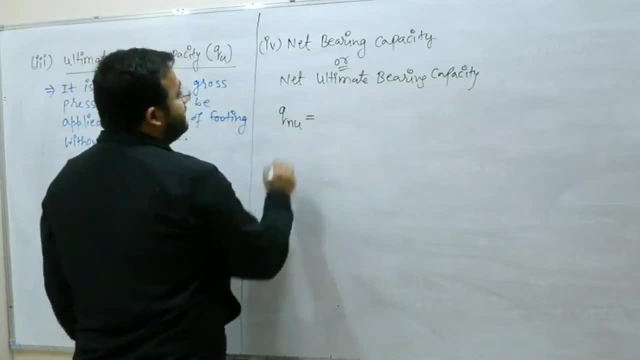 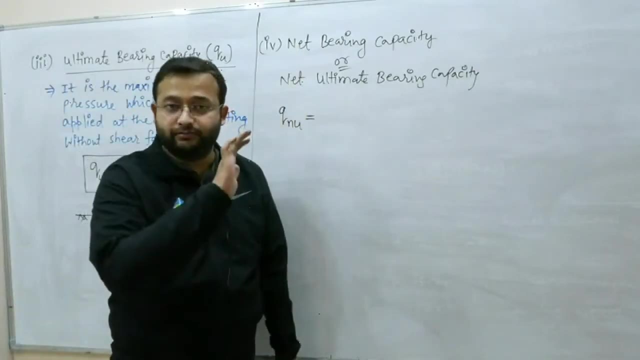 Now, what is QNU Net? Ultimate Bearing Capacity? Whenever the word comes net, remember whenever the word comes net, it means that here you do not have to consider overburden pressure, You do not need to consider overburden pressure. 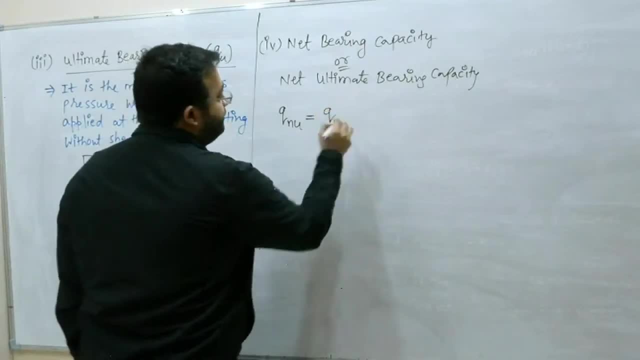 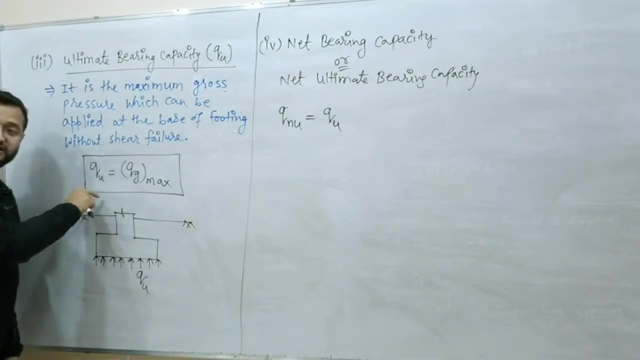 So what will be the net ultimate here? Your ultimate, which is coming. what has been included in this ultimate? Self-fit of footing, applied load and overburden is included, So I do not have to take overburden, So minus overburden from this ultimate. 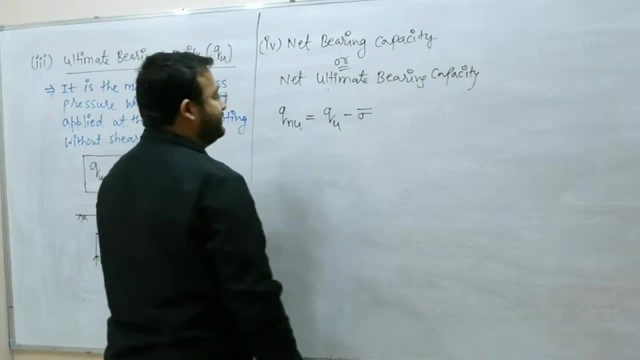 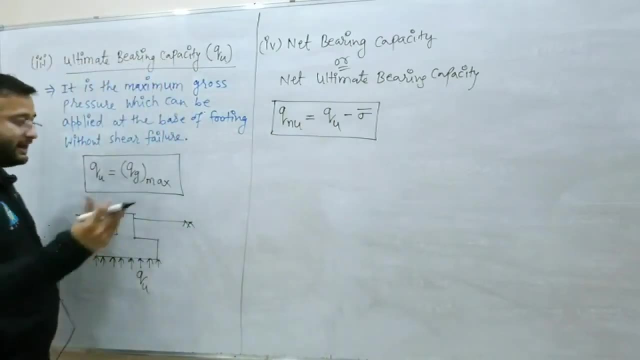 So what did I do with this ultimate Minus overburden? So what have I got here? I have got this value of net ultimate here. Okay, what will be the unit of all this, Brother? this is a type of pressure. 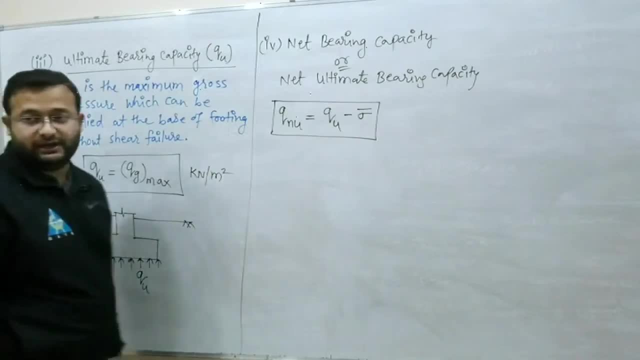 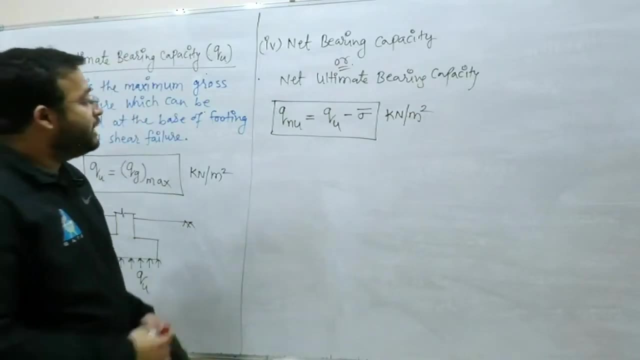 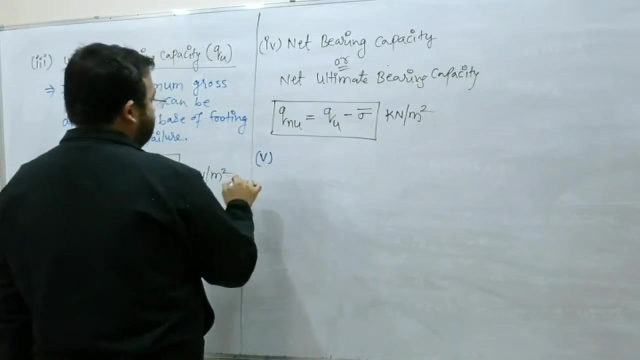 bearing capacity. All these units will remain in kN per m2 only. What will be the values? It will remain in kN per m2 only. Do you understand what I am saying? So this was your net ultimate bearing capacity. The fifth type of bearing capacity of the next type. 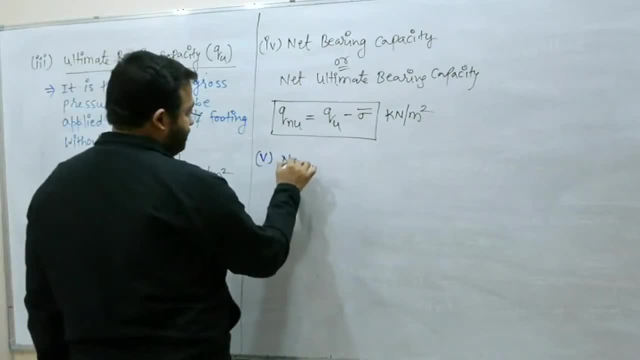 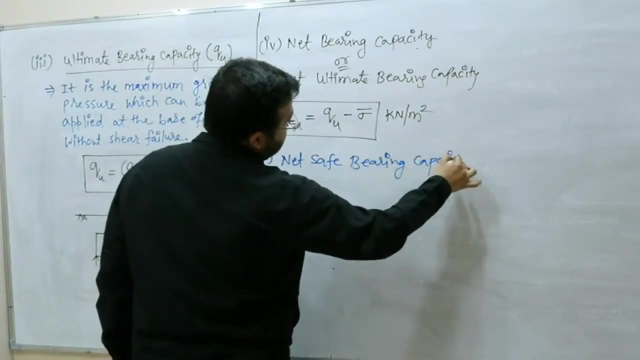 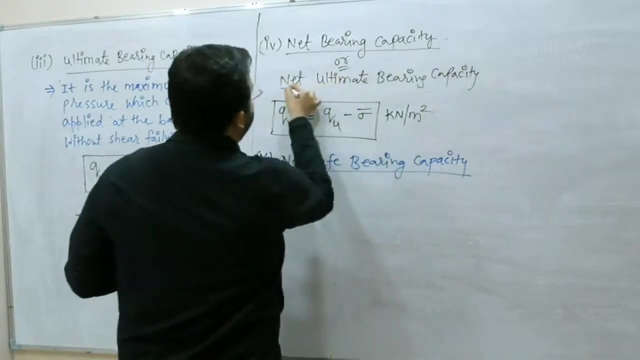 I am telling you: Net Safe Bearing Capacity, Net Safe Bearing Capacity. Now, what is this Net Safe Bearing Capacity? So, this Net Safe Bearing Capacity, Right, This Net Safe Bearing Capacity of yours, your net, like the term is telling, net. 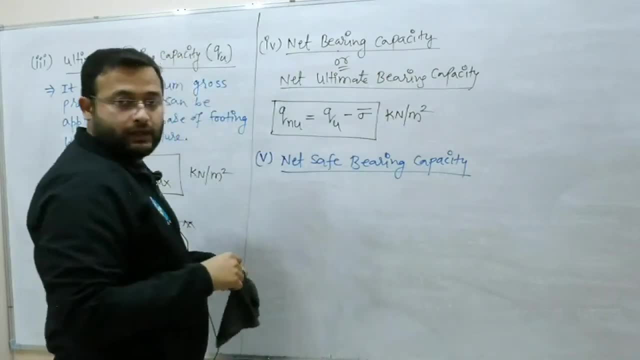 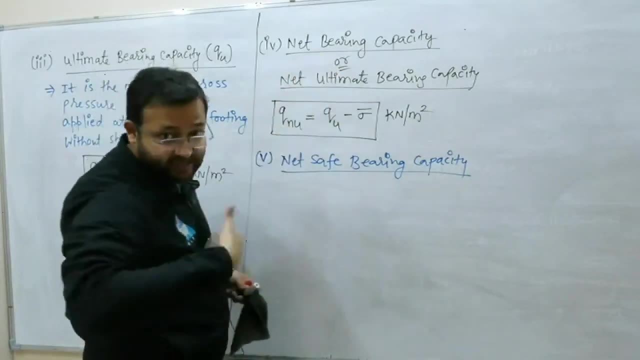 So net bearing capacity is written here. It has to be made safe. Brother, this net bearing capacity of yours, I have to convert it to net safe Means. I have to make this bearing capacity safe. So do one thing: Divide it with factor of safety. 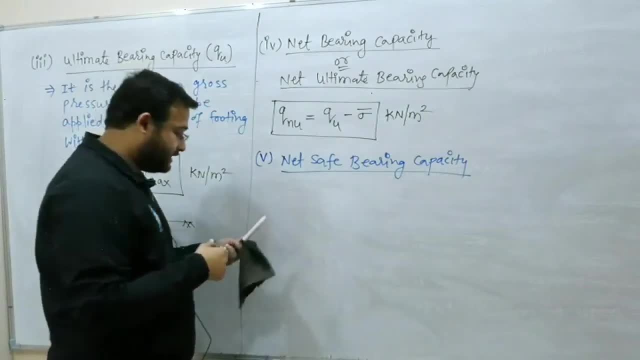 So your net bearing capacity will be converted to net safe bearing capacity. So what did we do? How will we denote net safe? We denote it with QNS. What will we read it? Net Safe Bearing Capacity. So I said, Okay. 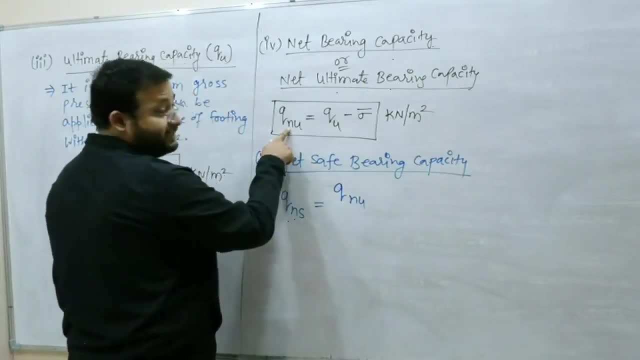 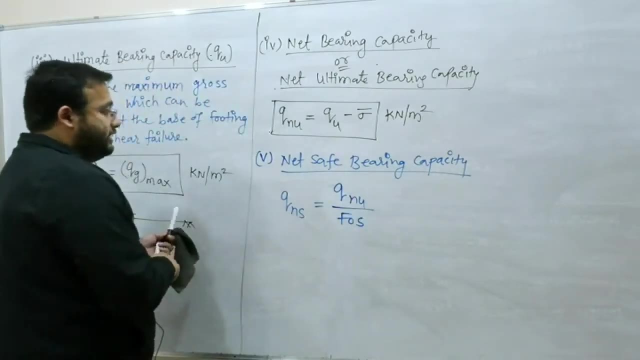 What did we write here? Net Ultimate, which I had taken out from here. Net Ultimate, Who did we divide it with? We divided it with factor of safety. So in which it was converted, It was converted to net safe bearing capacity. 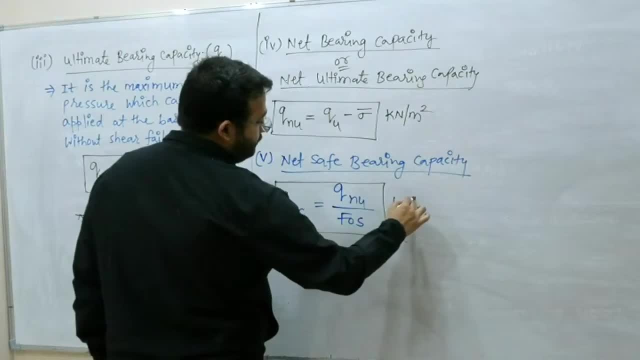 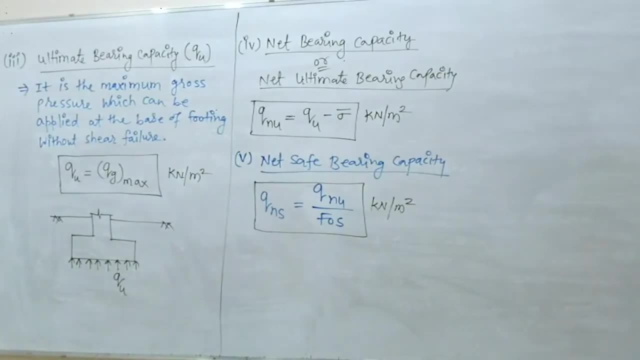 What will be its unit? Of course, It will be in Kilo Newton per meter square. Okay, Is everything clear? Yes, sir, Everything is clear to us. Next, Fifth, This is done. Sixth, bearing capacity, which I am telling you. 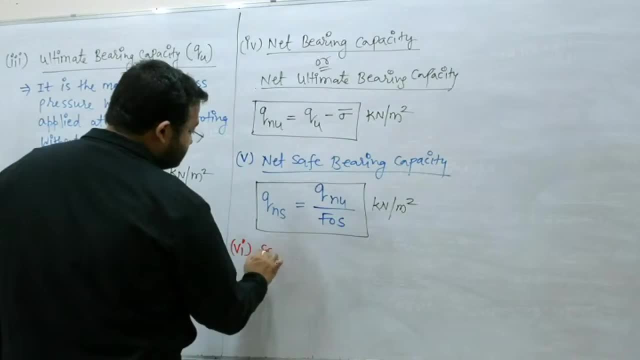 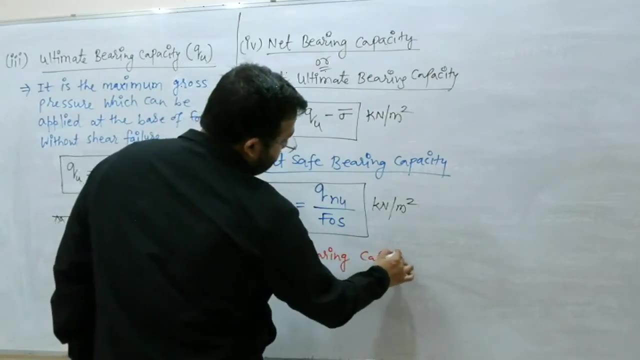 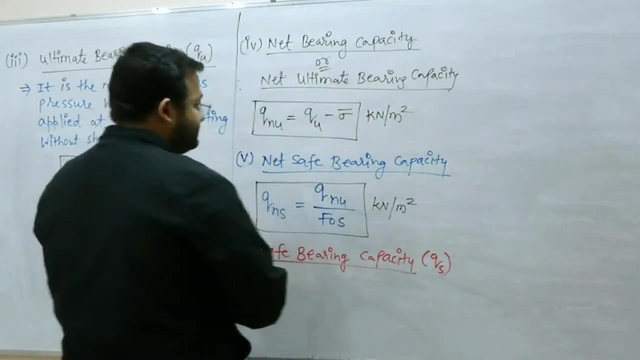 That sixth bearing capacity. I am telling you Safe bearing capacity, Safe Bearing Capacity, Now safe bearing capacity. We can denote it with QS here, And we can denote net safe with QNS here. Okay, Now what I am telling you here. 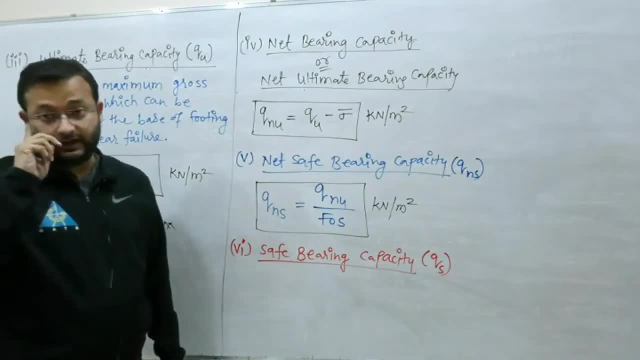 In safe bearing capacity. Listen to me carefully, Look, Listen carefully. First of all, What did I tell you? Ultimate bearing capacity QU. If this QU had to be converted to net ultimate, Then what did I do to sigma bar? 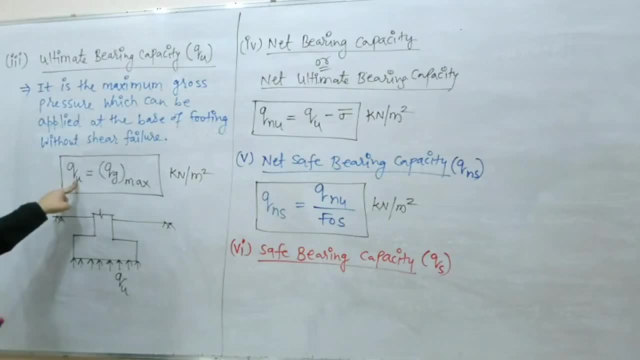 Minus Overburden pressure. What can be the value of this overburden pressure? It can be Gamma Df. When the water temperature is high, It will be negative. So What is the value of this overburden pressure? 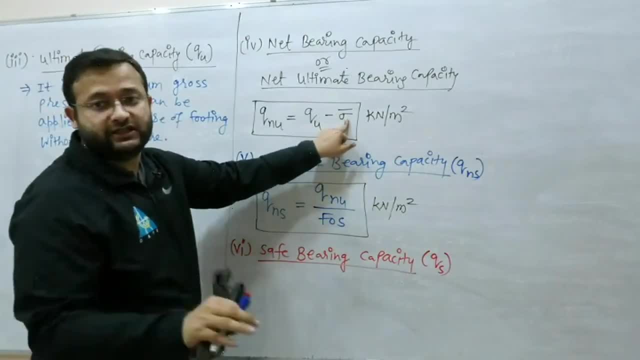 It will be negative. So What is the value of this overburden pressure? It can be Df When the water temperature is low. What can be the value of this sigma bar? This sigma bar's value is Effective stress. 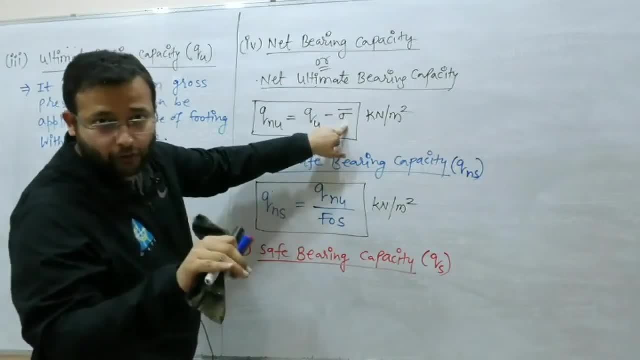 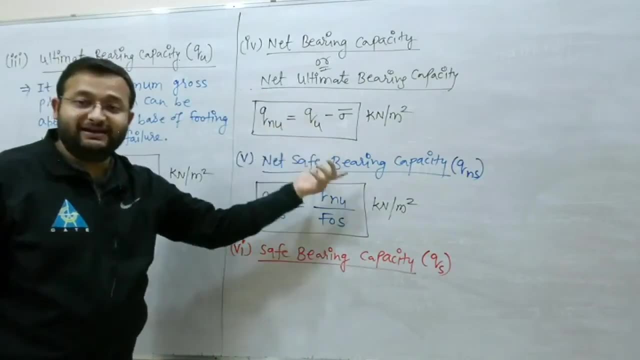 Effective stress. So Gamma Df can also be the Df When water temperature is low. I told you this earlier, So I am telling you That when I had to go from ultimate to net ultimate, Then I reduced sigma bar. 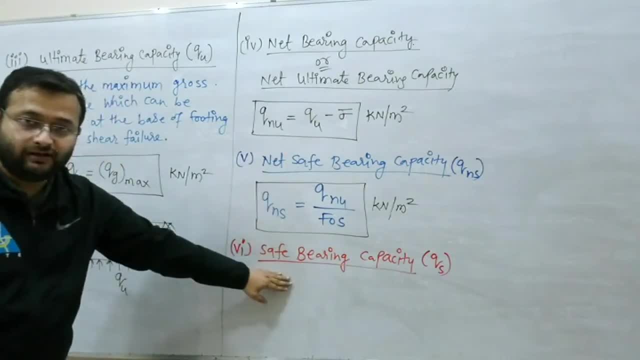 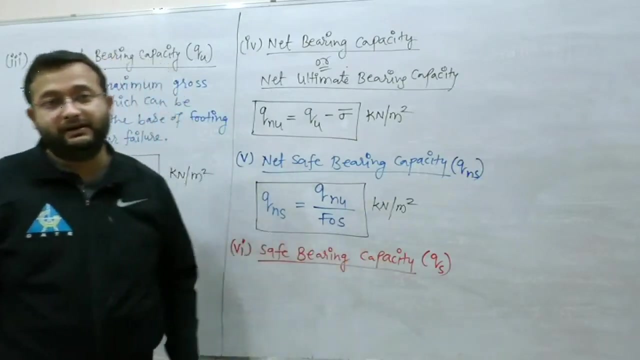 Now I have to move from net safe to safe. I want to remove the net word. Earlier I wanted to add net word, So I had to reduce sigma bar. Now I want to go from net safe to safe, So What will I have to do here? I have to remove the net, so I have to add the sigma bar here. 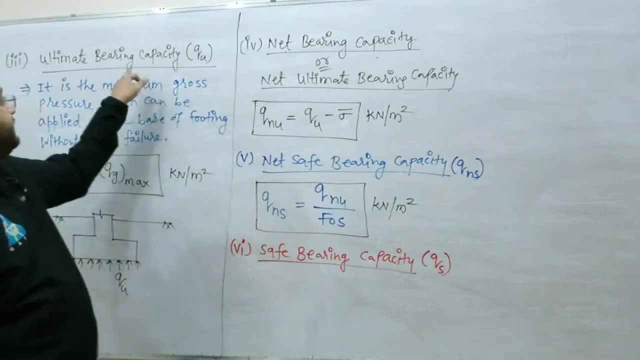 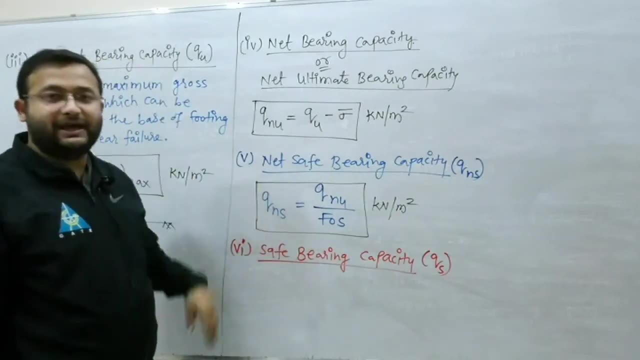 Do you understand what I am saying, Brother? first I had to go from the ultimate to the net ultimate, so I did sigma bar minus. Now I have to come from the net safe to the safe, so add the sigma bar, So the net term will be removed. 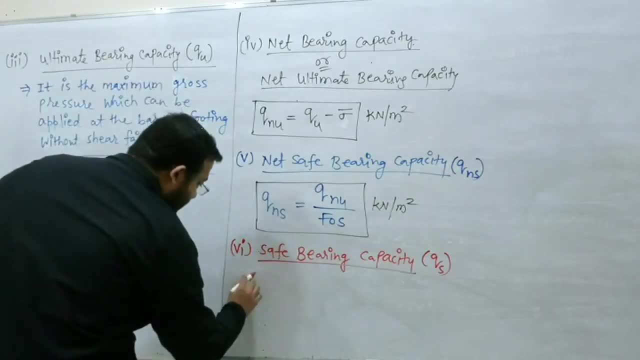 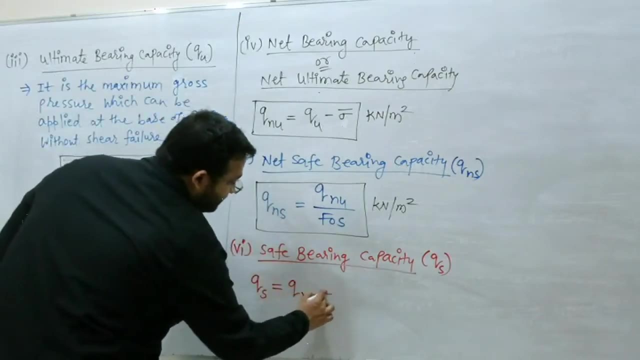 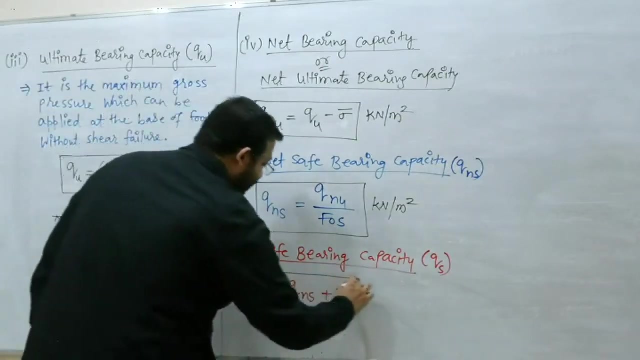 So what we did here? we made the safe from the net safe. So what will be your safe bearing capacity? The net safe that you had removed from here. you add, overburden pressure to this net safe. This will be your safe bearing capacity here. 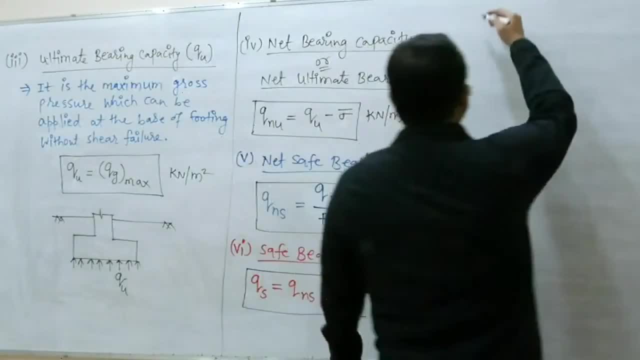 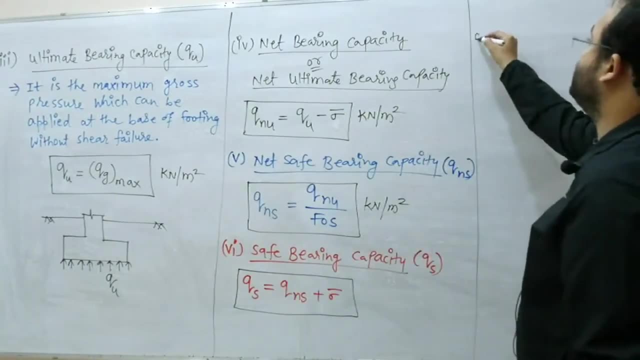 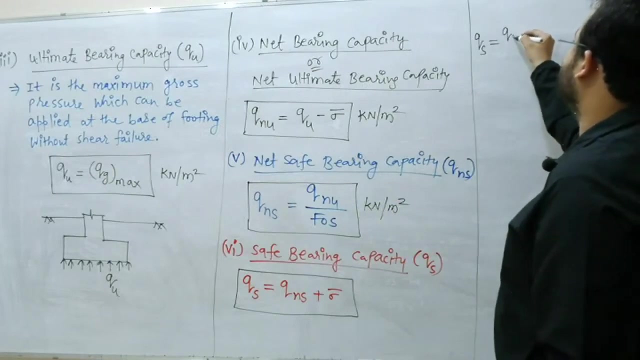 Now see here what is the picture? The picture is that safe bearing capacity Qs will be equal to What is net safe? Net safe is yours. I have just taught you that net ultimate is the factor of safety. Divide it with the factor of safety. 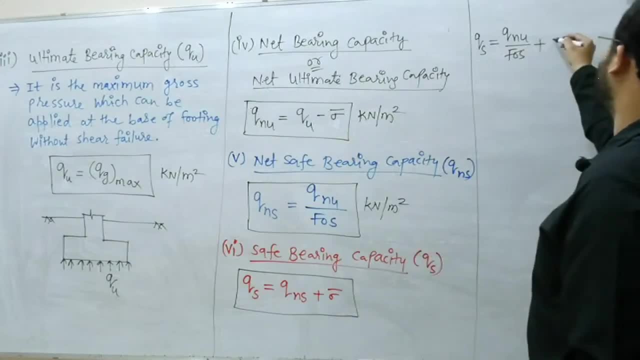 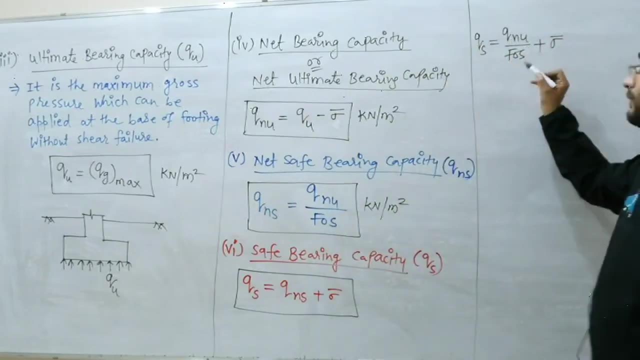 This is your net safe And this overburden sigma bar. I have written here. So see, instead of net safe, I have written net ultimate divided by the factor of safety. here Now I am saying Qs is equal to. 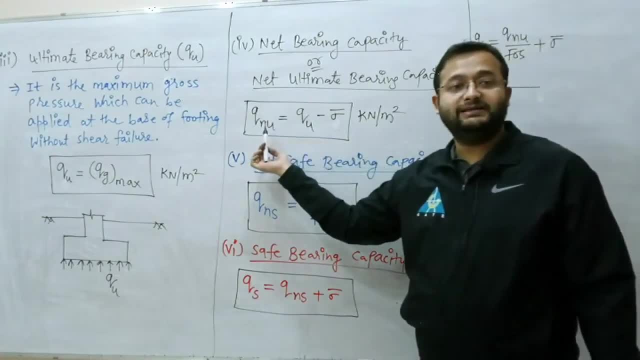 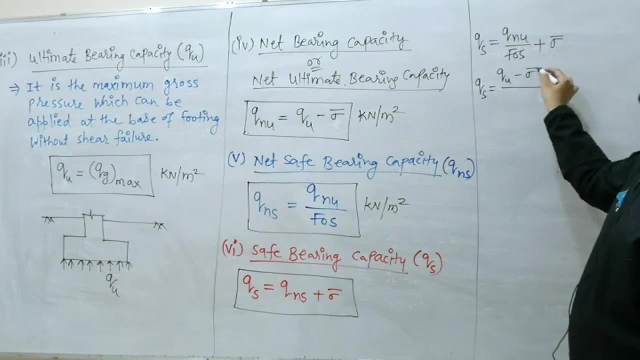 What can we see with this net ultimate? Where did this net ultimate come from? I had minused the sigma bar from your ultimate, So what should I write here? Whatever your ultimate will be, you minus the sigma bar from it. divide it by the factor of safety plus the sigma bar. 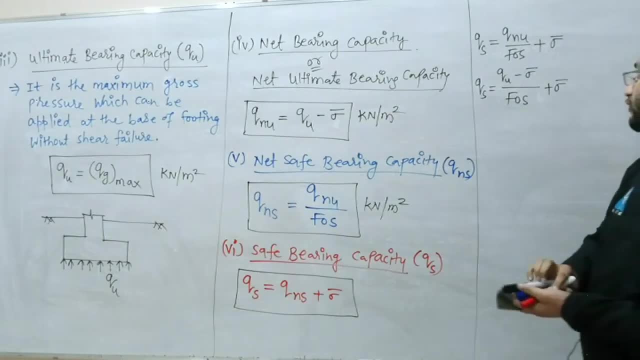 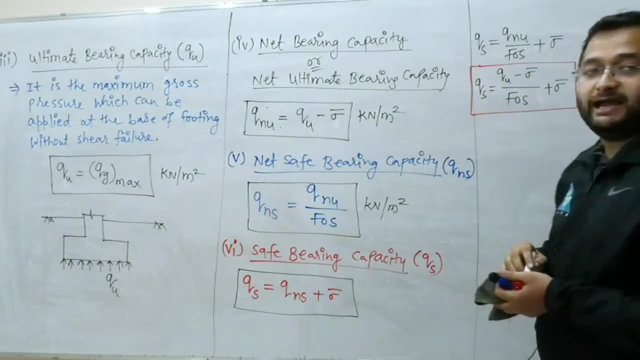 So this is mine here. So this is my formula for finding the safe bearing capacity. It is an important formula. Sometimes questions are asked here in different exams, Whether it is your RRB exam, your GATE exam, your SSC exam, your engineering services exam. 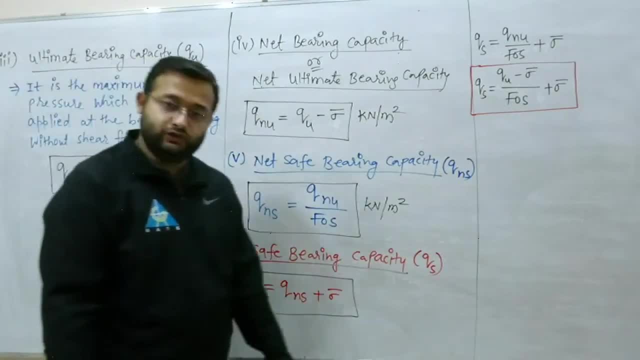 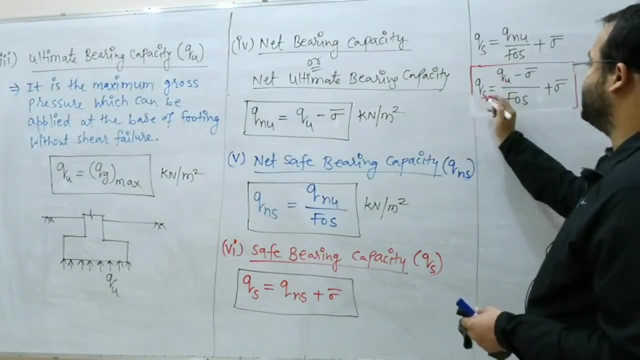 To find the safe bearing capacity. a few questions are asked for 1-2 marks, So you should know how to find it. You should notice one thing here: I have told you about these 6 types of bearing capacity. Why am I making you study in circles? 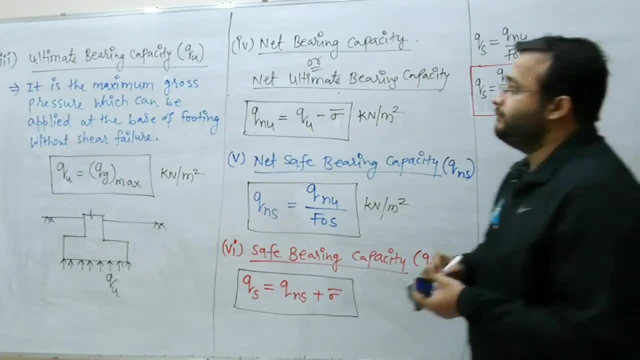 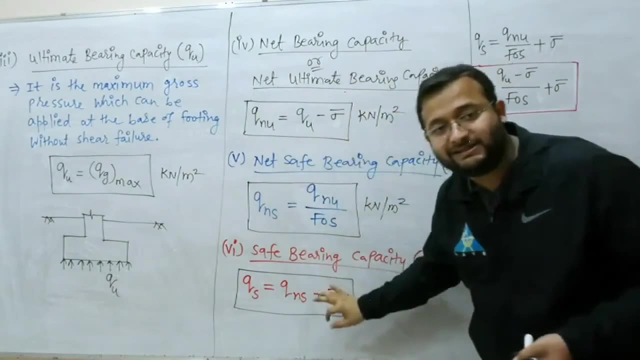 Why did I teach you to find the ultimate first? Then I found the net ultimate from the ultimate, From the net ultimate. I found the net safe From the net safe. I found the safe again When you had to come back. why did you get so confused? 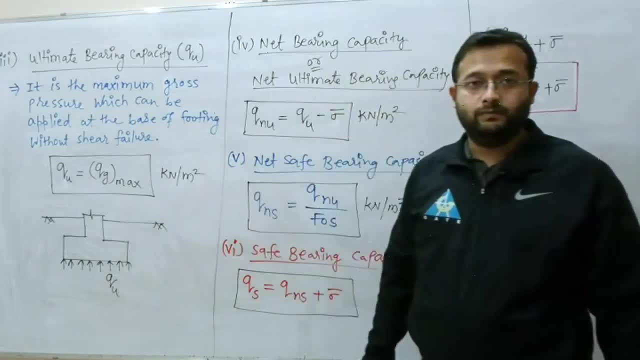 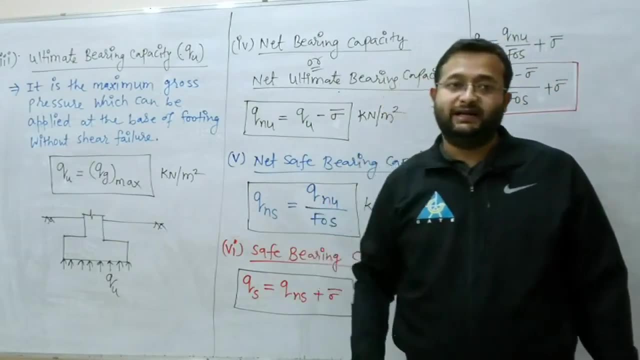 Directly in the ultimate, we divide it by the factor of safety. When you had to make it safe, what do we want to do? We want to make our bearing capacity safe. Understand my point, Understand that point, Understand what I want to tell you. 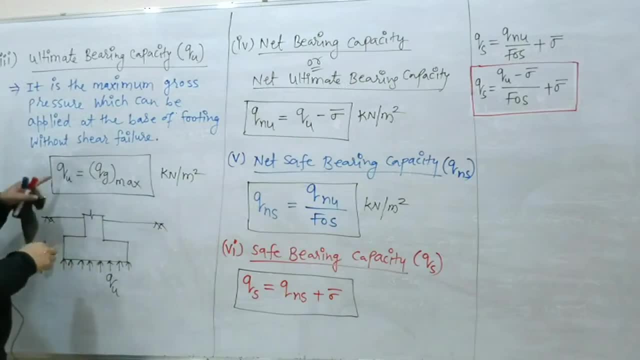 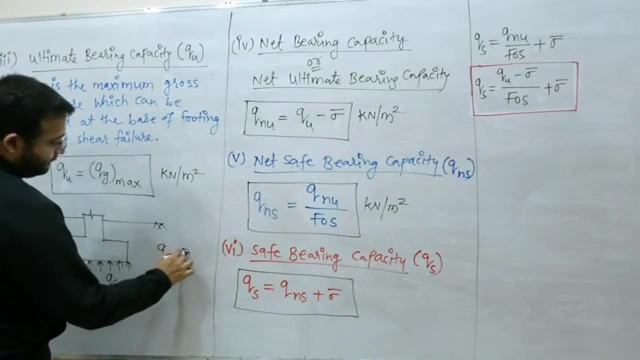 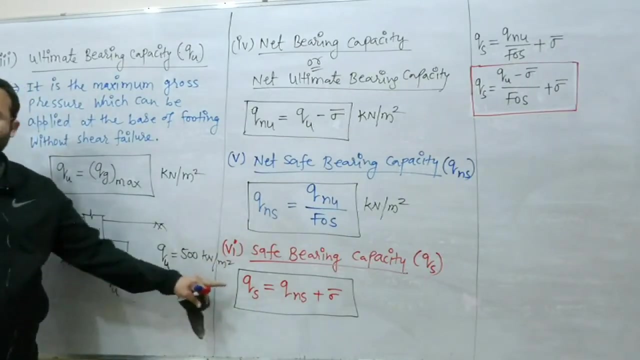 For example, how much ultimate bearing capacity did I get here? Here the ultimate bearing capacity that I got: I got, for example, 500 kN per m2.. For example, the ultimate bearing capacity that I got: I got 500 kN per m2.. 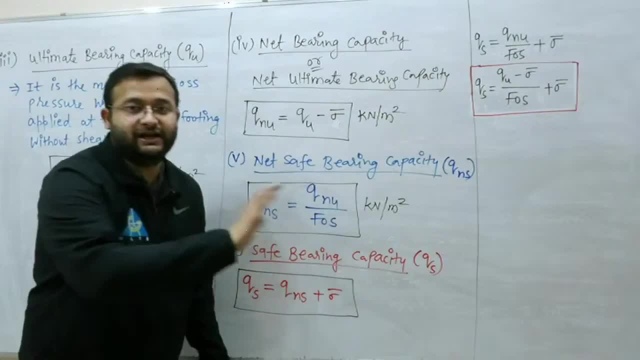 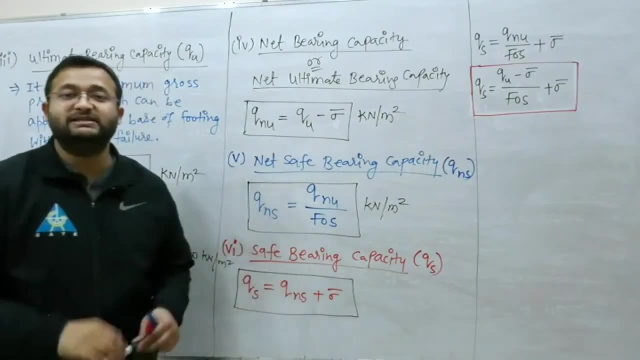 This means that you apply 500 kN per m2 pressure on your soil On the base of the footing. On the base of the footing Your soil will be safe. It will not be shear. But as soon as you increase the value a little- 501,- then the soil will become shear. 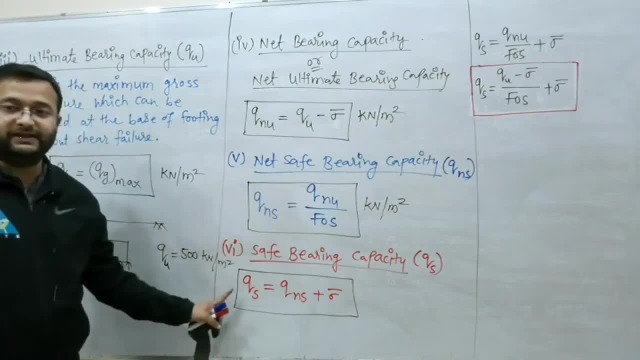 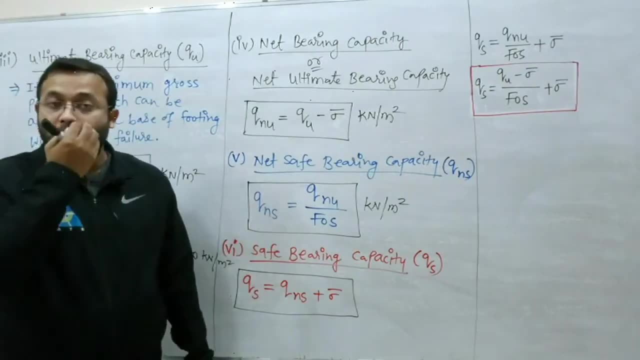 Did you understand my point? This is your ultimate bearing capacity. I am saying that we will never apply 500 kN, We will apply less than 500 kN. So I said: do one thing: apply the factor of safety here. 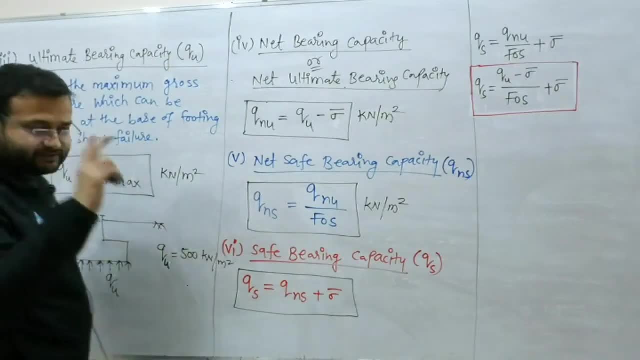 So I said we want two factor of safety. How much factor of safety do we want Two? So I am saying that you convert the ultimate capacity here into safe. We want to make it safe. What do we want to do? We want to make it safe. 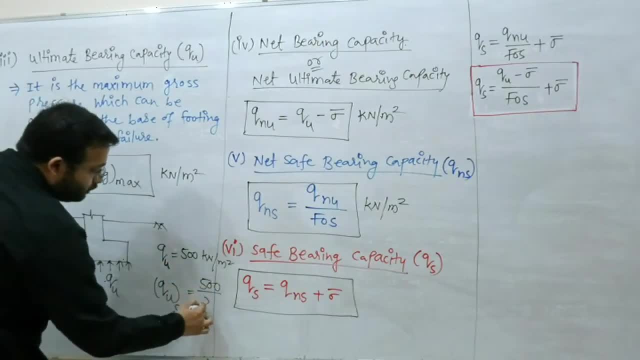 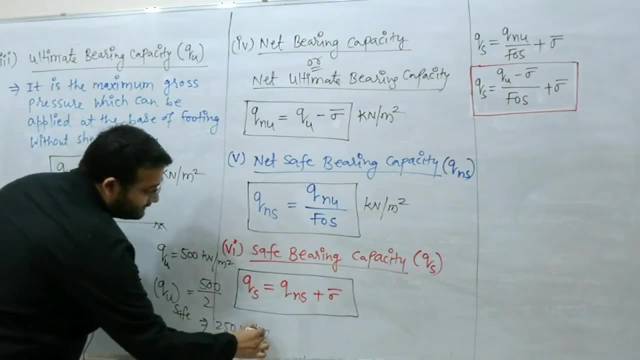 So what did we do? 500 divided by 2.. What was 2?? Factor of safety. That means: how much can I apply? now? I can apply 250 kN per m2.. This is the meaning of it. If you are following this approach, then this is absolutely wrong. 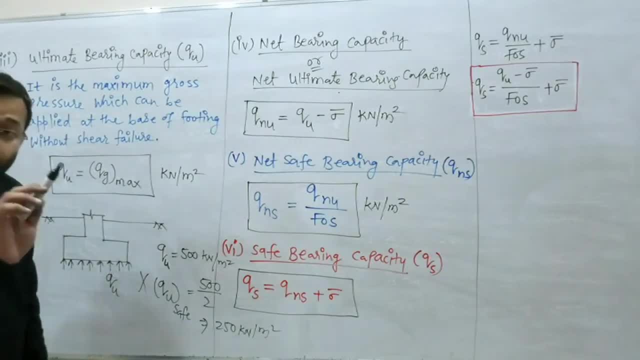 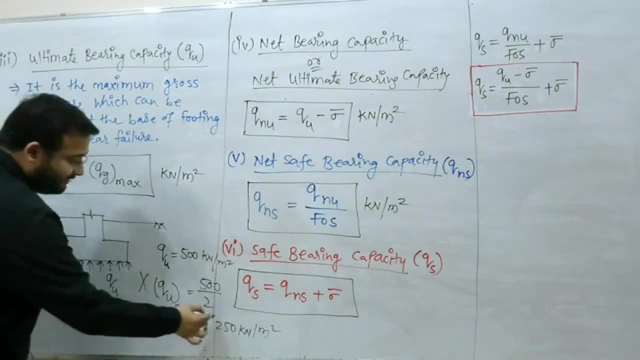 It will be considered as an approach. Why, sir? Because you have to listen to me. If you are applying such an approach that you are directly dividing the factor of safety in the ultimate bearing capacity, then you are adopting a wrong method. 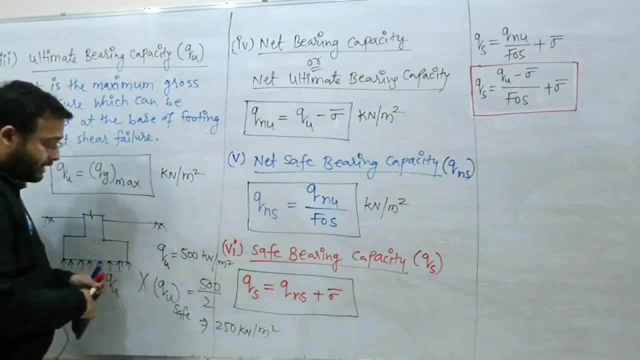 Why, sir? What is the reason behind this? Understand that I have applied the factor of safety directly in the ultimate bearing capacity here, which is wrong. Why? Because where did this ultimate bearing capacity, 500 kN per m2, come from? 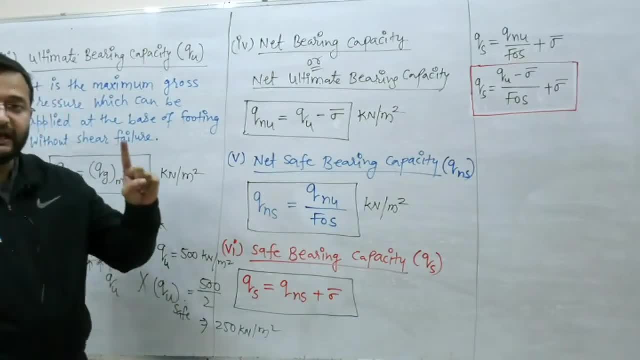 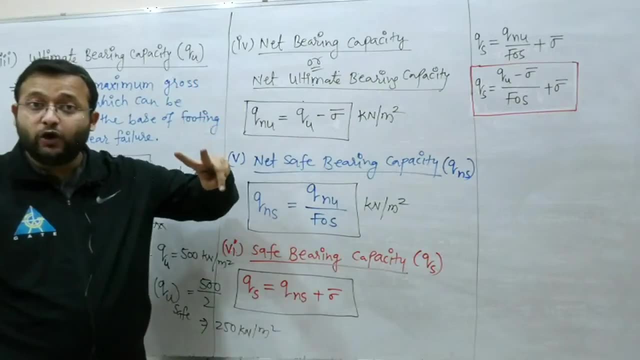 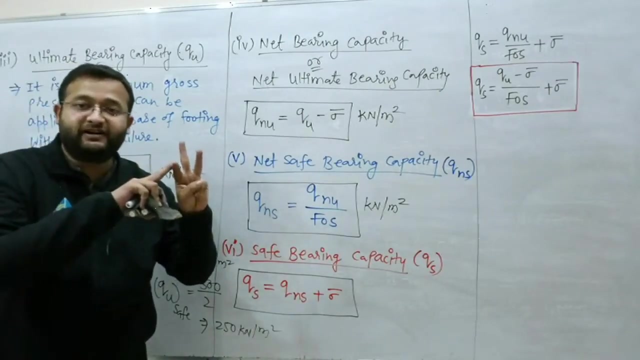 This 500 kN per m2 came from, first because of the applied load, second because of the self-weight of footing and third because of the overburden pressure, If you apply the factor of safety in the applied load. 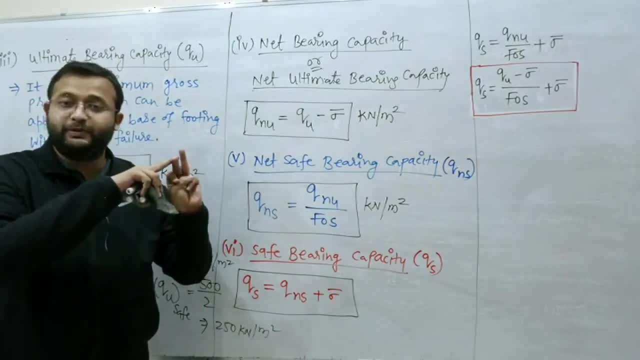 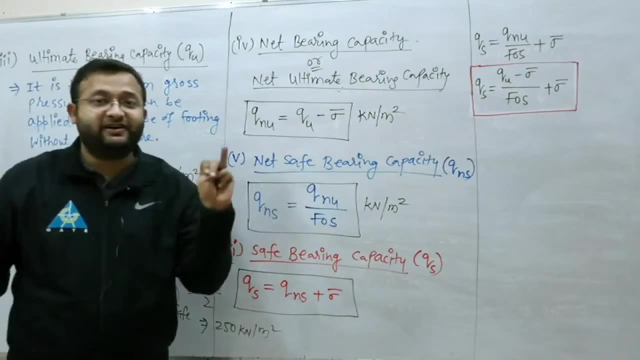 then there is no problem. If you apply the factor of safety in the pressure coming due to the self-weight of footing, then there is no problem. But you cannot apply the factor of safety in the overburden pressure. You do not need to apply it. 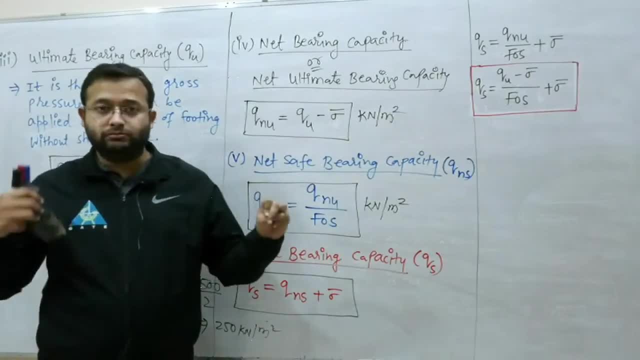 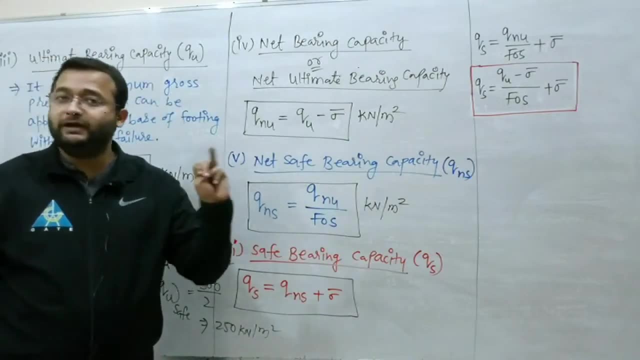 I do not mean that the government will come and put you in jail. There is no need. There is no need to apply the factor of safety in the overburden pressure. Why, sir? There is no need? Because what is the overburden pressure? 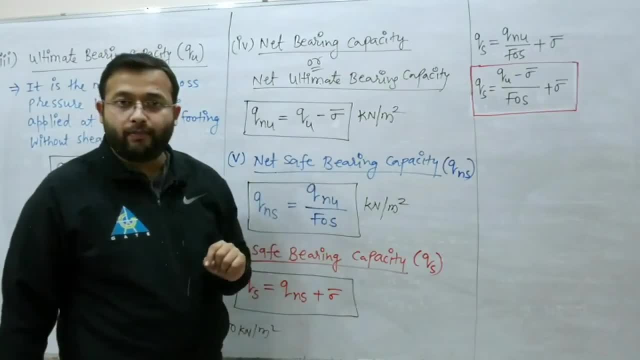 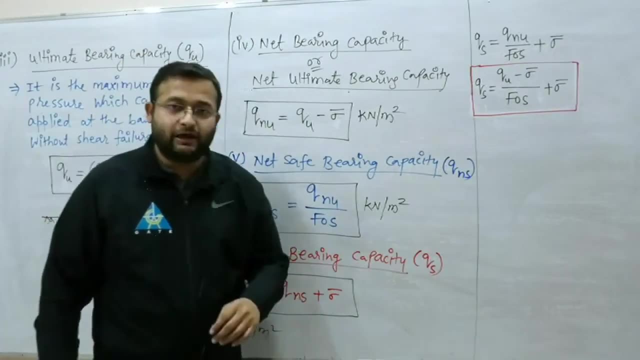 The overburden pressure is the self-weight of the soil itself. Sigma, bar, Gamma, df. The overburden pressure of the soil itself is the self-weight. Tell me one thing: When I was not making the foundation there, even then that soil was present there. 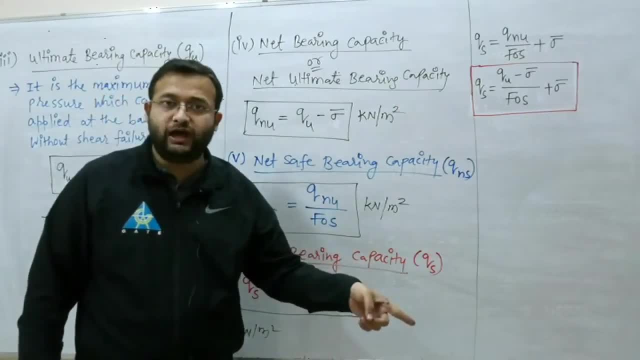 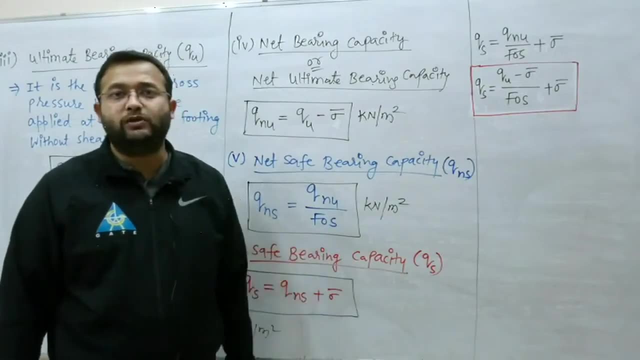 When I was not making the foundation. even then that soil was present there. Was there any deformation in the soil? Brother? that soil is present there since 10 years. The soil is present there since 20 years. The soil is present there since 100 years. 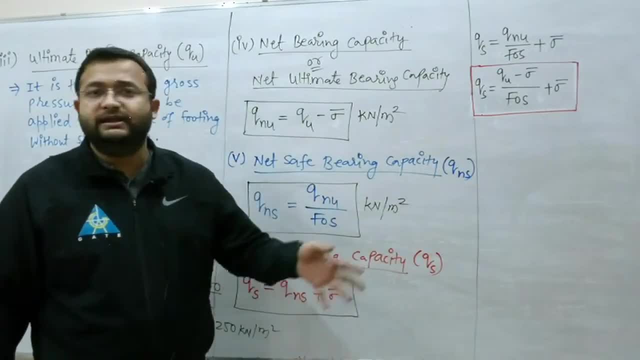 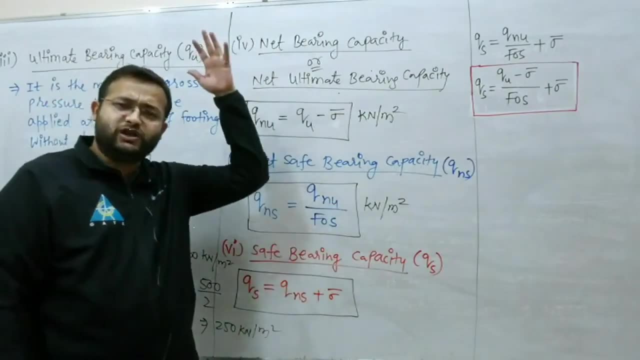 The soil is present there since 500 years, Then there is no deformation Means due to the self-weight of the soil itself. it is looking like history That pressure is coming on from many generations, So due to that, I am not getting any deformation. 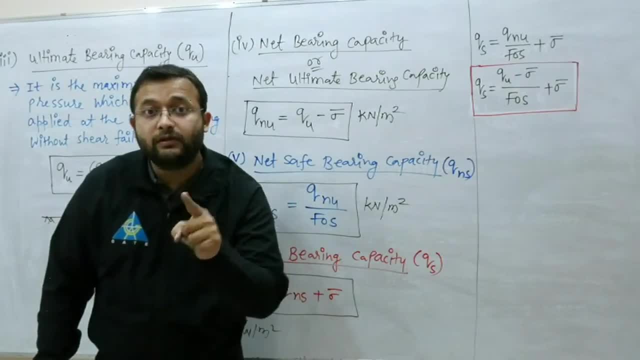 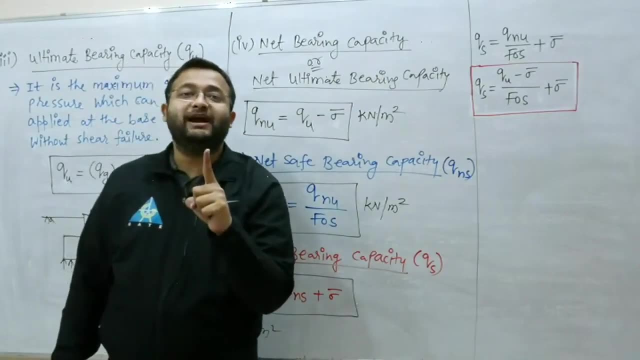 What is the deformation? Due to applied load, Due to the structure which I have made, Due to self-weight of footing, So in which you should apply the factor of safety, You should apply it in both: Apply it in applied load, in self-weight of footing. 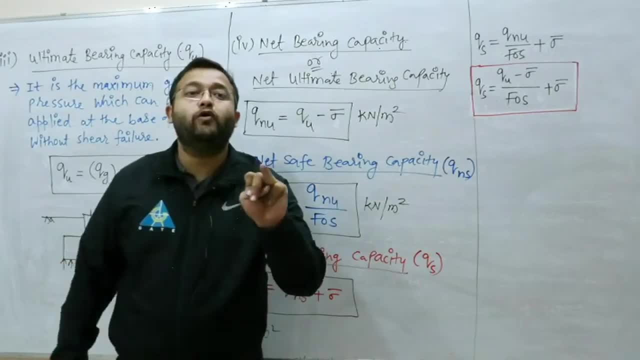 In these it is necessary to apply the factor of safety. This third reason, the overburden one, it does not need the factor of safety. So if you directly in 500, means if you directly apply the factor of safety in the ultimate bearing capacity. 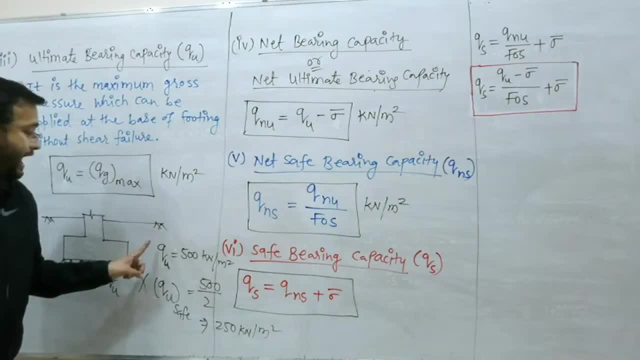 then it is wrong, Because it means that you have to apply the factor of safety in the ultimate bearing capacity. If you are dividing the ultimate bearing capacity with the factor of safety, then it means that you have also divided the overburden pressure with the factor of safety. 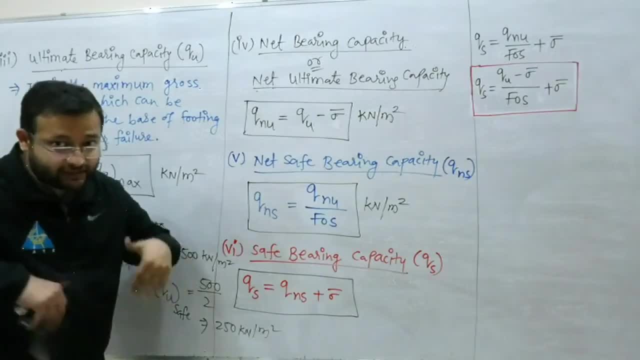 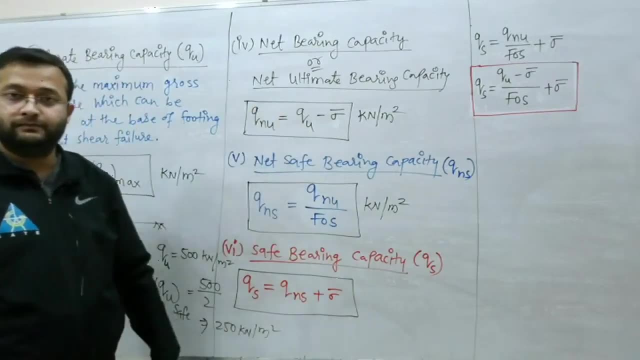 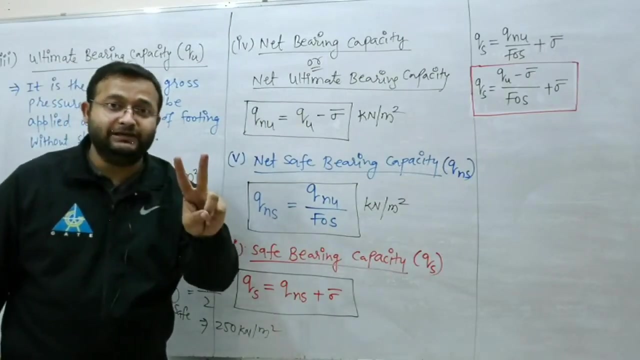 Which I never want. So see how I turned the picture. How did I turn the picture? That in this ultimate first of all, I have minused the overburden pressure. So now what is actually left? here, Only applied load and self-weight of footing is left. 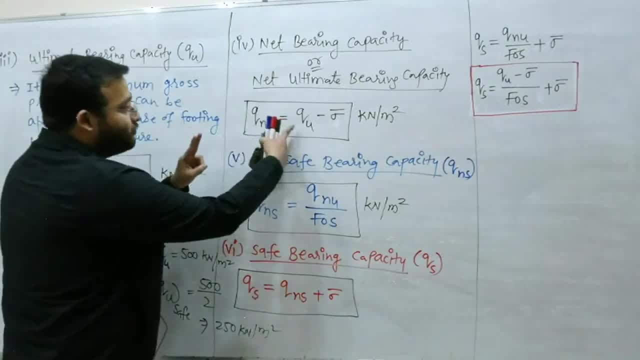 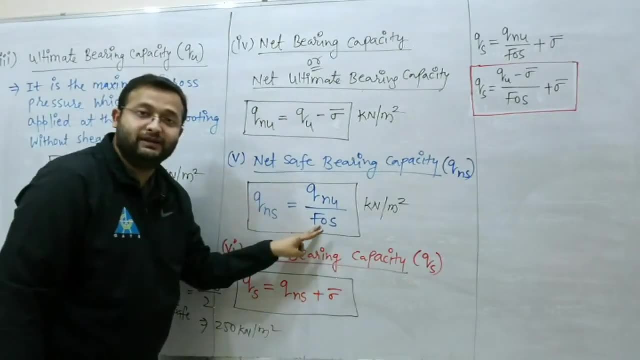 Because of them, only the pressure is left. So now this much is left, In that I have applied the factor of safety. Net ultimate means only these two things are left. Now I have applied the factor of safety in it. Now the overburden pressure which I had minused, 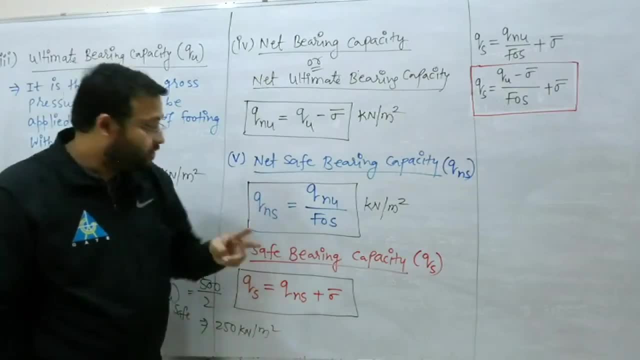 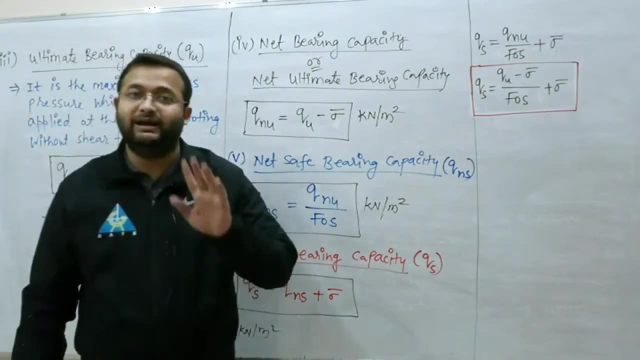 I want to consider it again without the factor of safety. So I have brought it back and added it. So this is my safe bearing capacity. Apply this much pressure on your footing to design. So when I had taught you RCC, when I had taught you RCC, 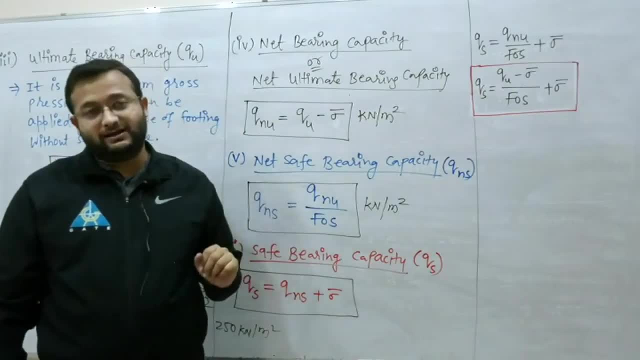 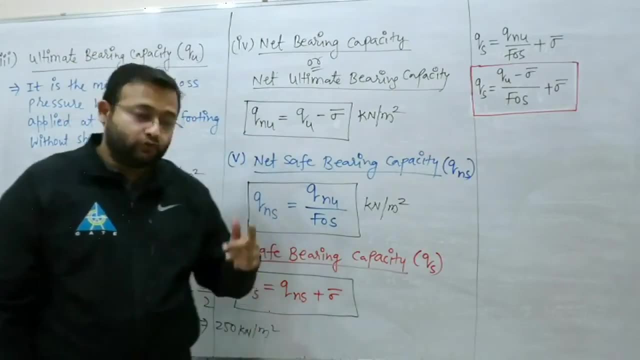 reinforced cement concrete. then you will remember what we used to do. We used to write SBC in load divide. We used to write safe bearing capacity. So this is your SBC Short name: S, B and C: Safe bearing capacity. 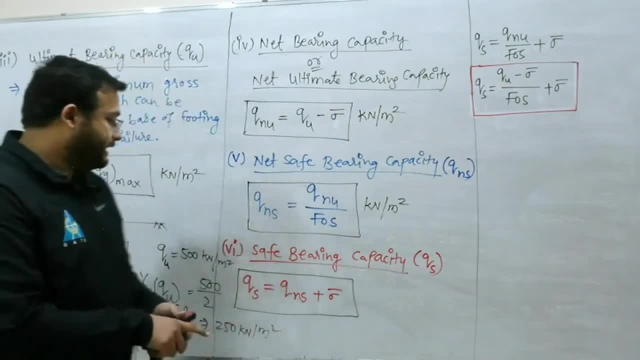 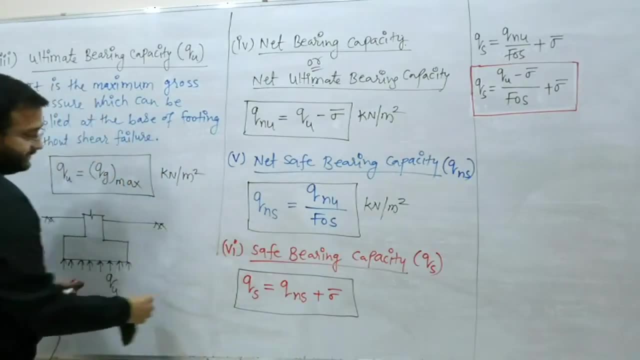 Do you understand what I am saying? So in this way we used to proceed there. So you must have understood very well why we have proceeded like this, step by step. I hope it will be clear to you, The concept will be clear to you. 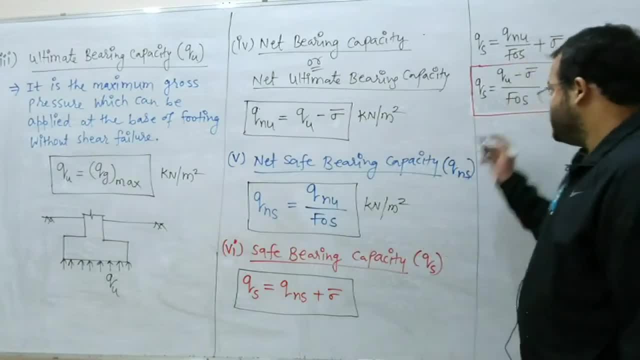 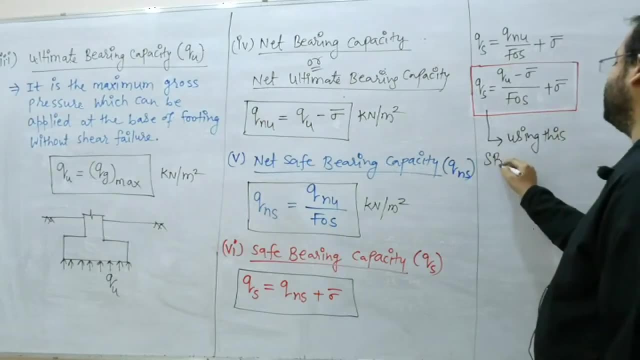 Okay, So you will note this much. I will write about this: safe bearing capacity. Using this SBC. using this SBC, plan area of the footing is designed Right. Plan area of the footing is designed. Plan area of the footing is designed. 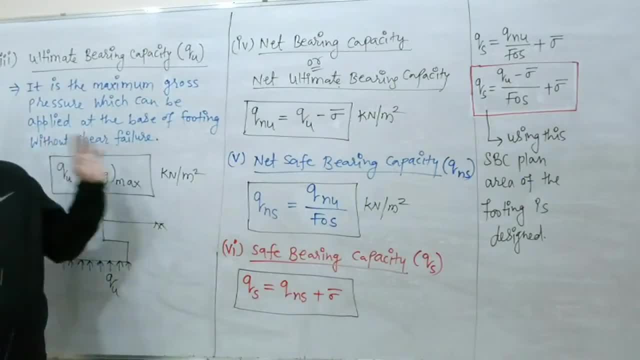 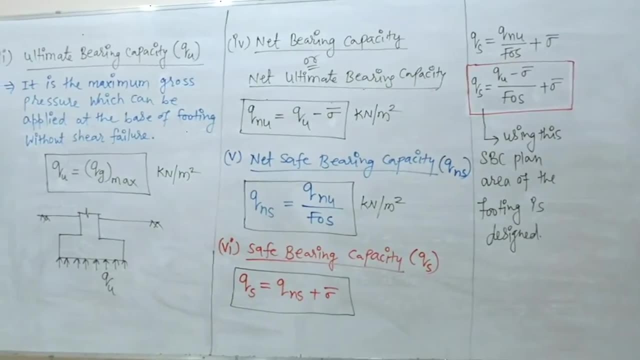 Clear. So we will take a photo. so quickly We will take a photo. So here till now, see once I turn the camera and tell you what I have taught you till now. Till now I have taught you, See, Till now. 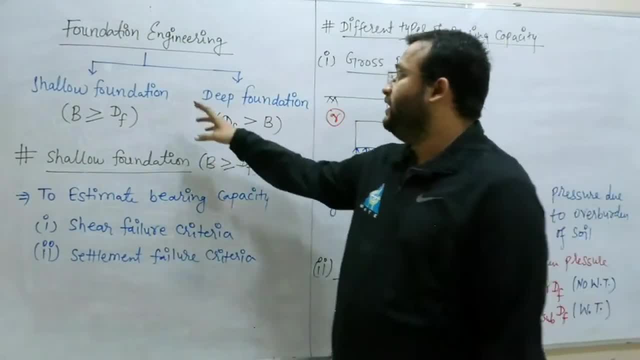 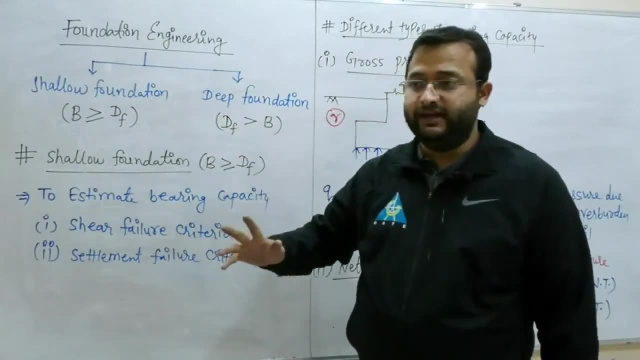 first of all, what we have seen till now. we will see that We have started foundation engineering. I told you what is shallow foundation, what is deep foundation. We started today's chapter shallow foundation and bearing capacity. So in shallow foundation. 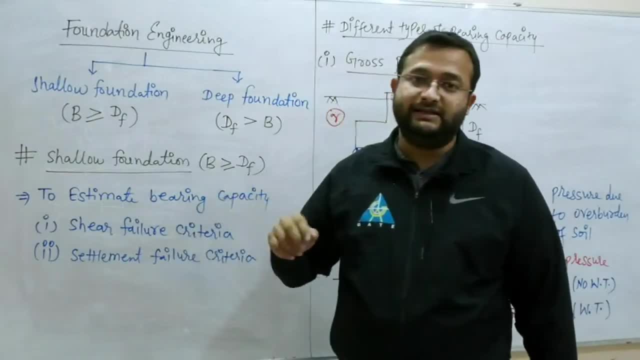 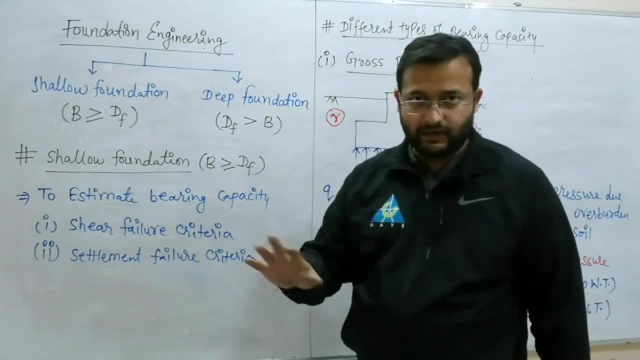 I told you that if you want to estimate bearing capacity, then you can have two criteria: One can be your settlement failure criteria and the other can be your shear failure criteria. We will see about this in the coming time. If you apply shear failure criteria, 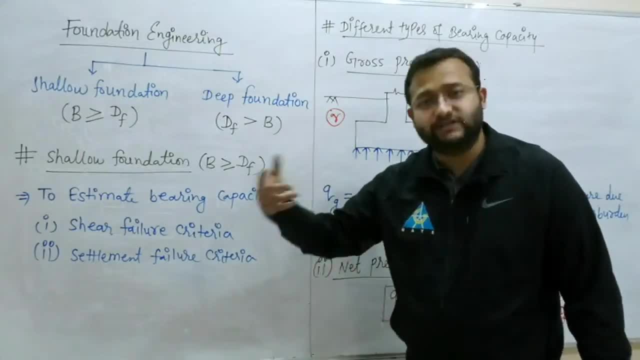 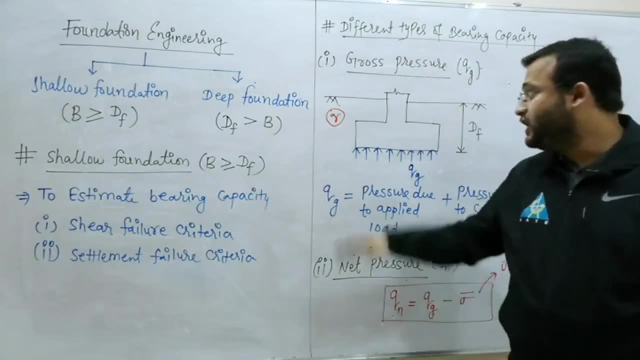 then how bearing capacity comes out. If you apply settlement failure criteria, then how bearing capacity will come out. We will discuss about that now. I told you that we can determine which type of bearing capacity, So I gave you information of gross pressure. 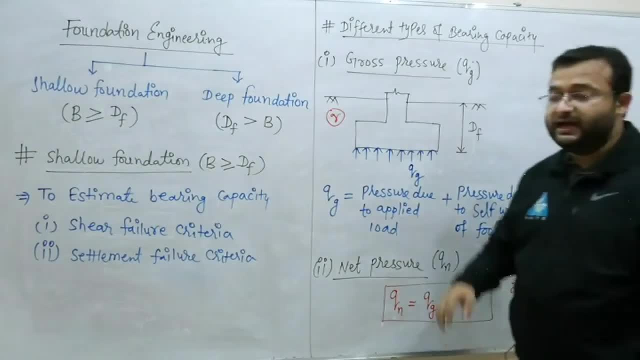 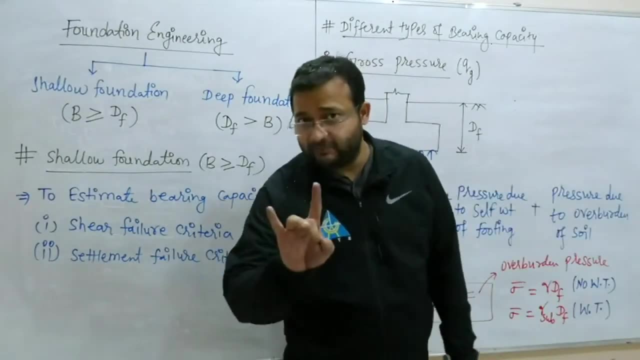 I gave you information about net pressure. Whenever net word comes means you have to consider overburden there You don't have to consider overburden. Why you don't have to consider overburden? I have just told you that we don't want to divide it with factor of safety. 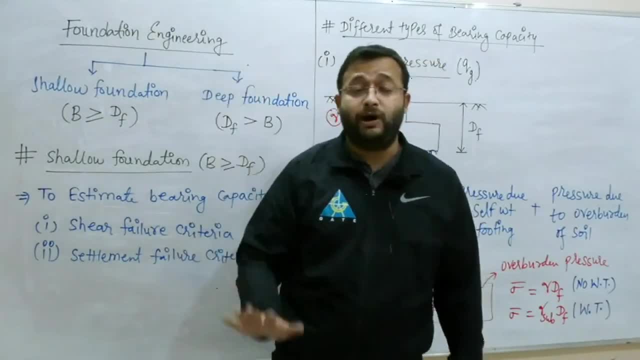 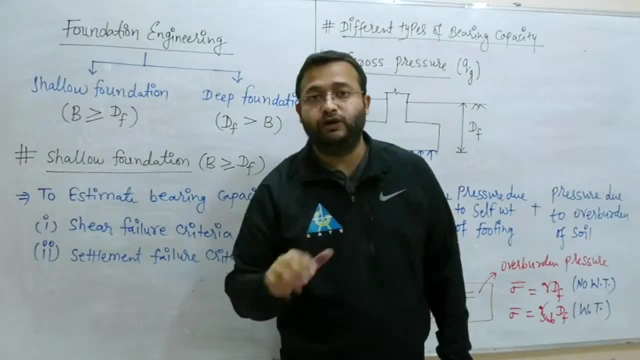 Because it is coming from many ages, from many years, from many times, So it doesn't need factor of safety. Who needs factor of safety? The one who just applied applied load? the one who just applied self-adapted footing? 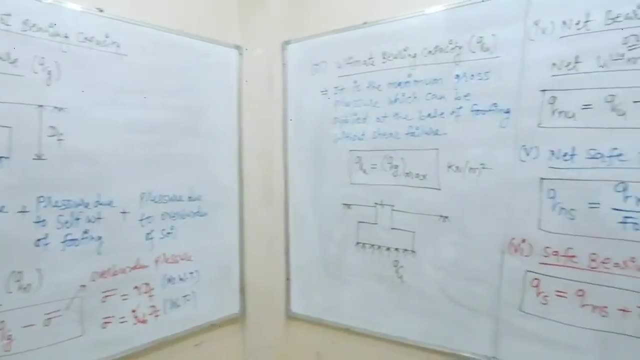 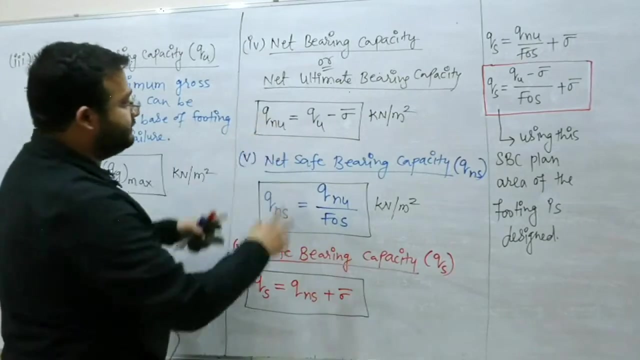 he needs factor of safety. Am I saying it correctly? Now, after that, now, after that, right After that, we will move forward. And I gave you information about ultimate bearing capacity, information about net bearing, information about net shear. information about net shear. 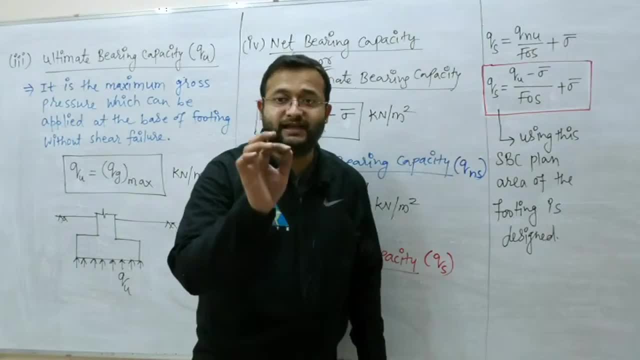 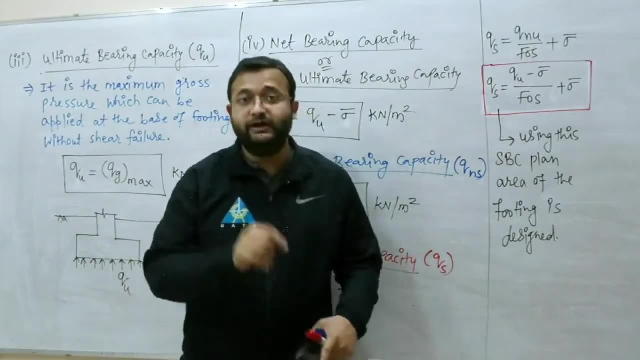 and information about safe bearing capacity. That safe bearing capacity is your bearing capacity, which you design. plan. area of the footing in reinforcement. concrete subject: while using it. Okay, We will take this much photo. Those who want to take photo, take photo. Those who want to take screenshot. 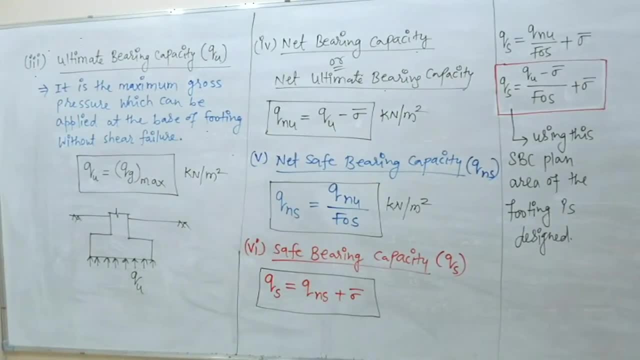 take screenshot And those who want to share, share it Now, you should be fine. All right, Okay, Let's go. Yeah, sure, Let's go. Okay, Okay, Hello, Thank you, Thank you, Thank you. 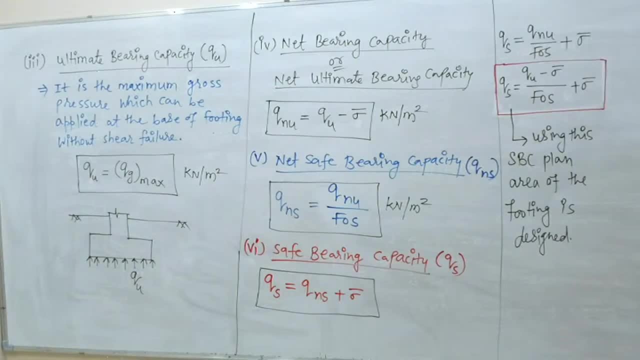 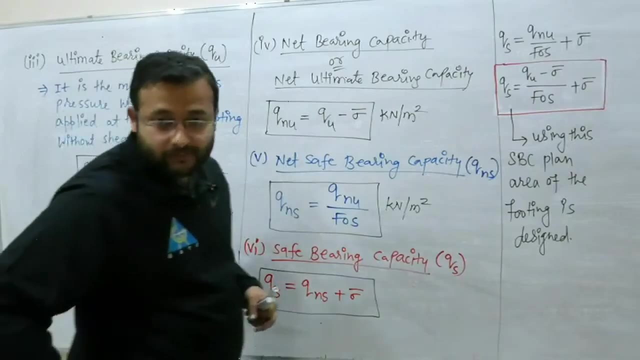 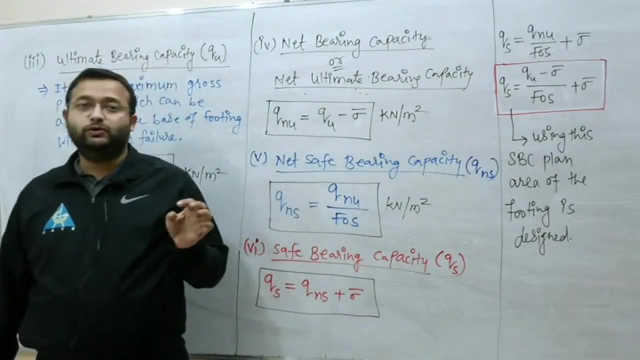 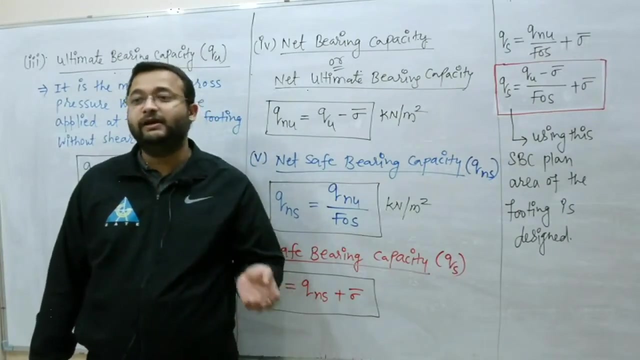 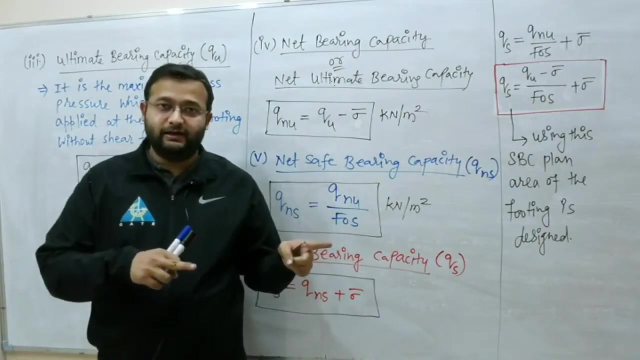 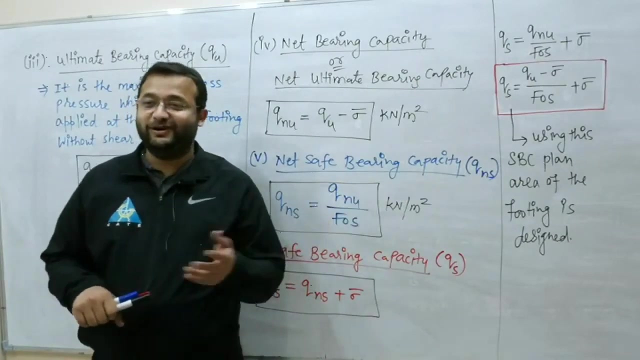 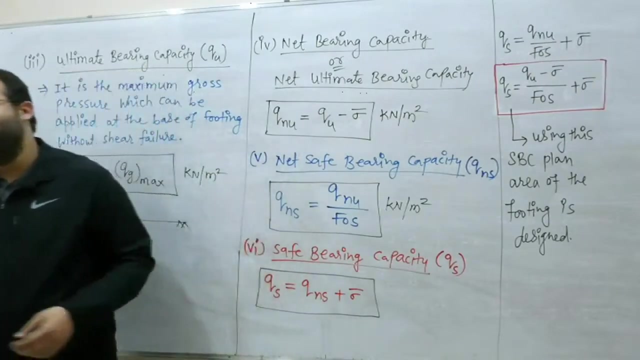 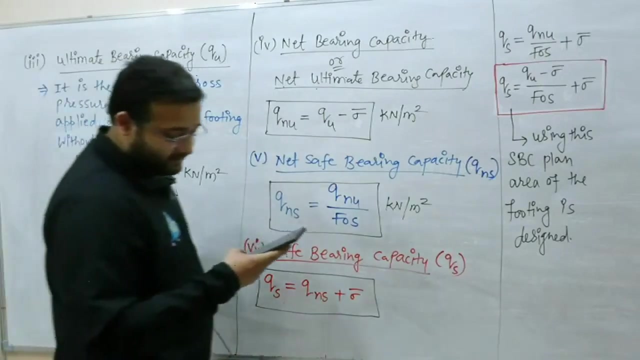 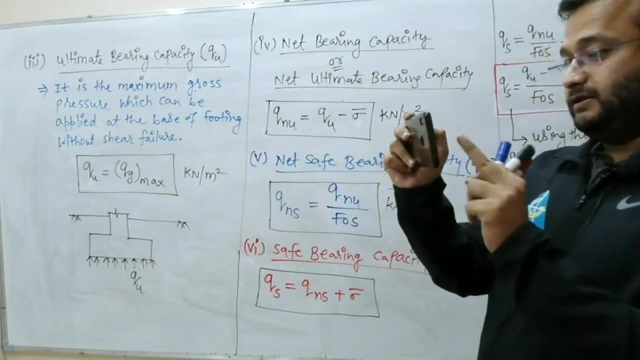 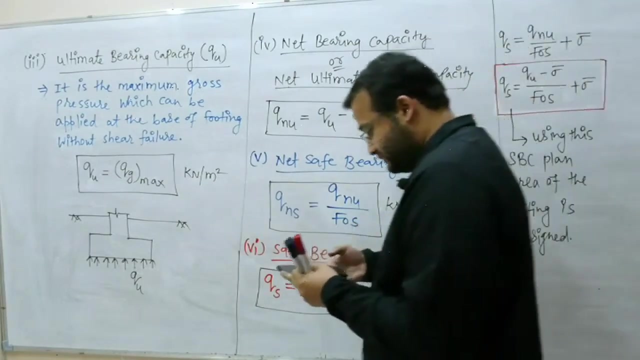 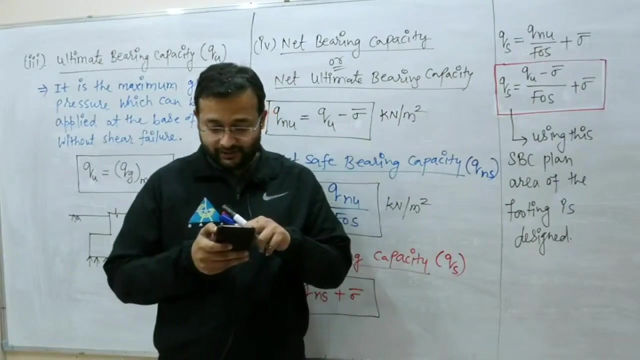 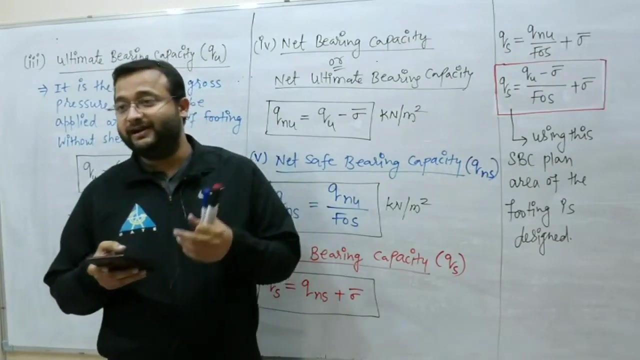 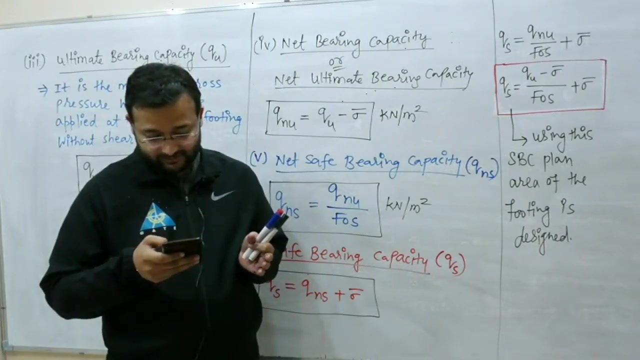 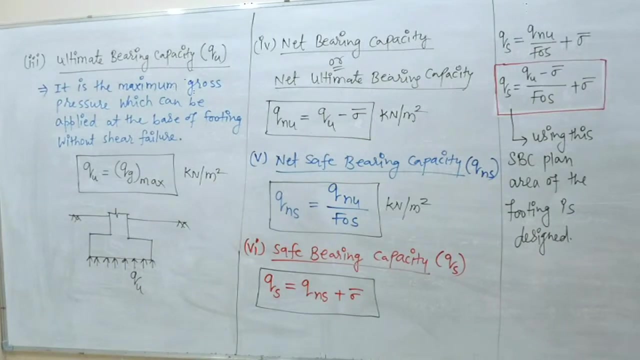 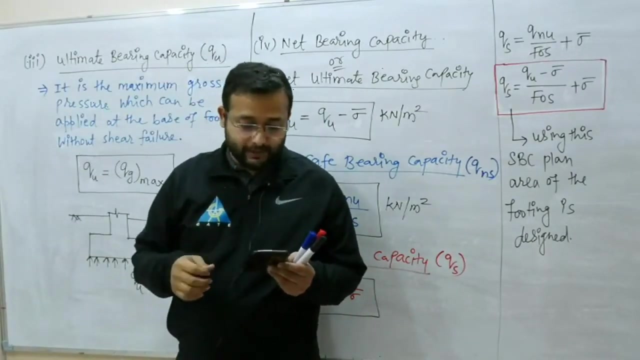 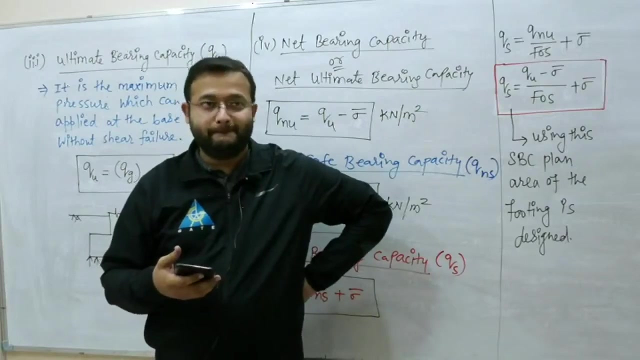 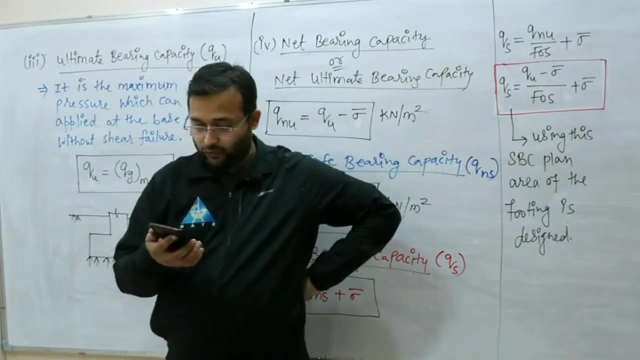 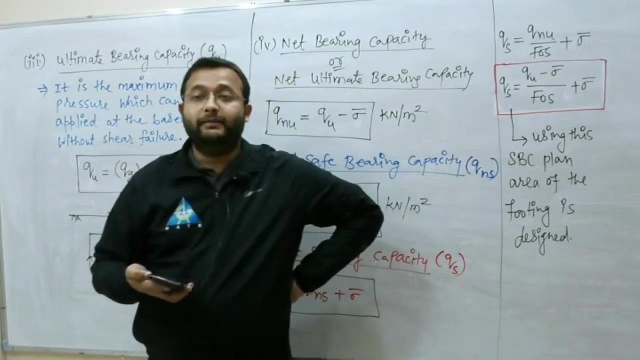 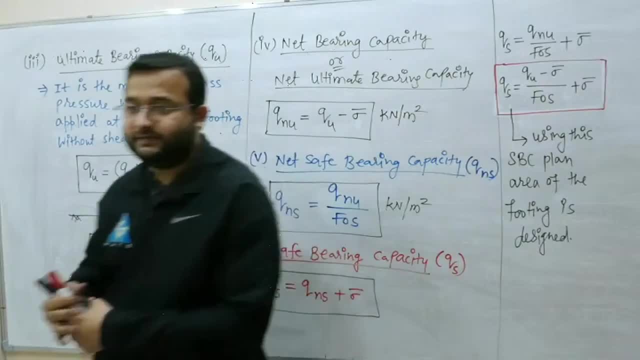 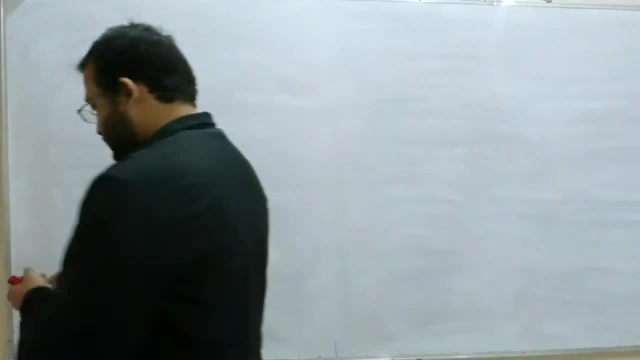 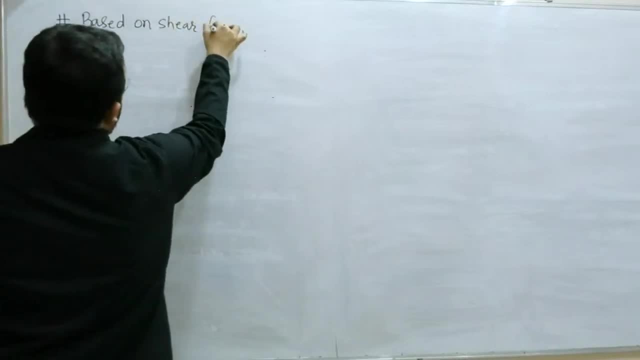 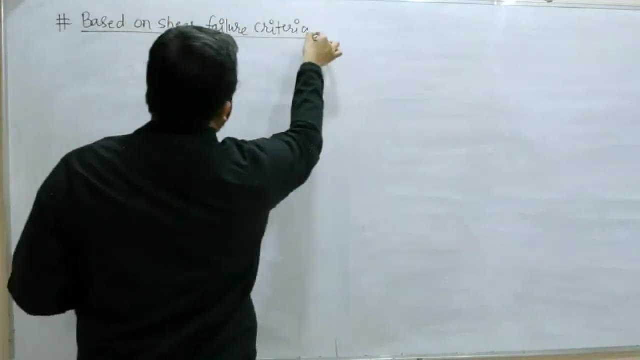 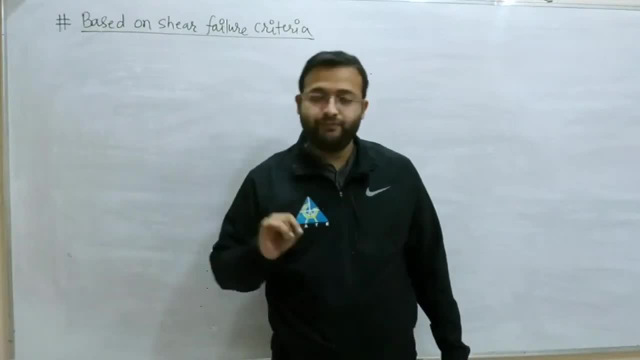 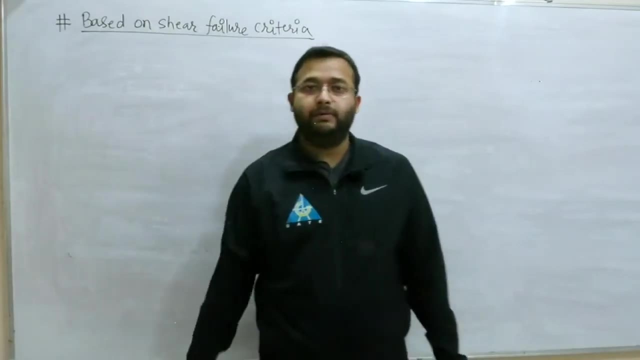 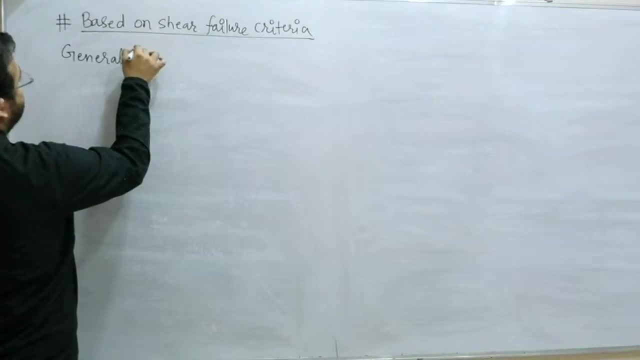 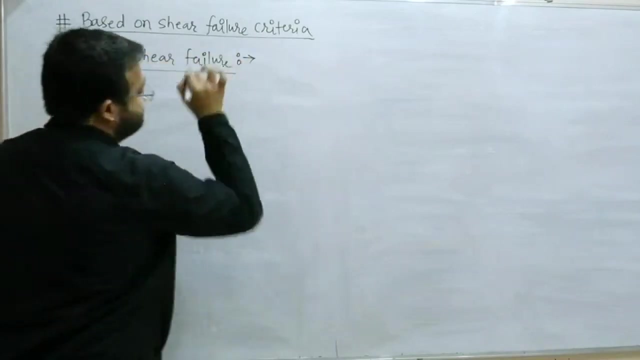 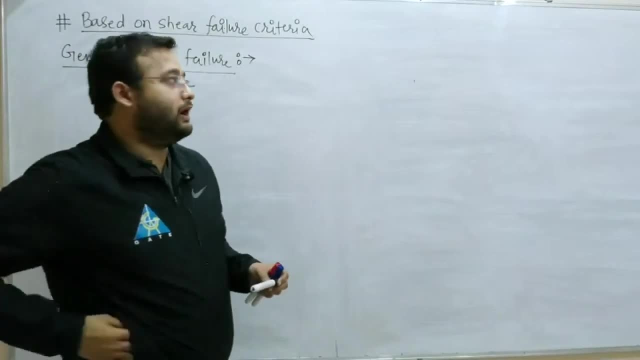 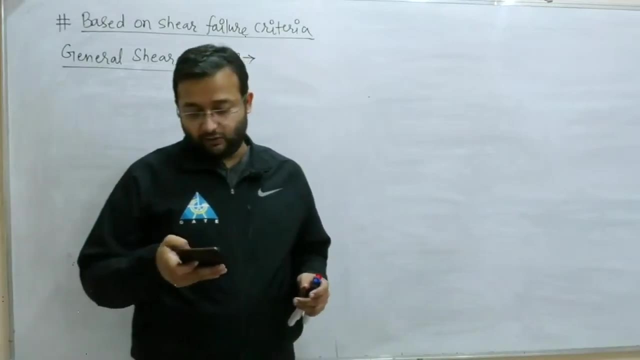 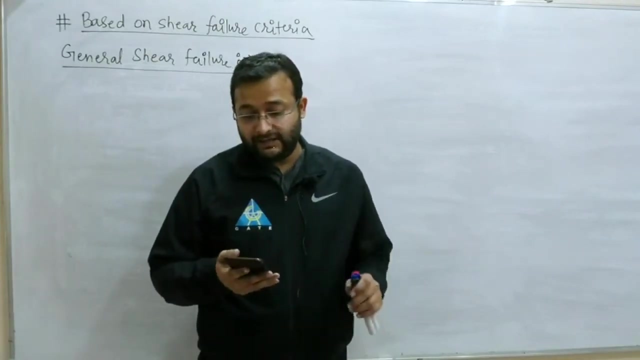 So, as I told you about General Shear Failure, I am telling you that when will you get to see this General Shear Failure? I am telling you that you will get to see this General Shear Failure in highly dense soil, Whenever you will have highly dense soil. 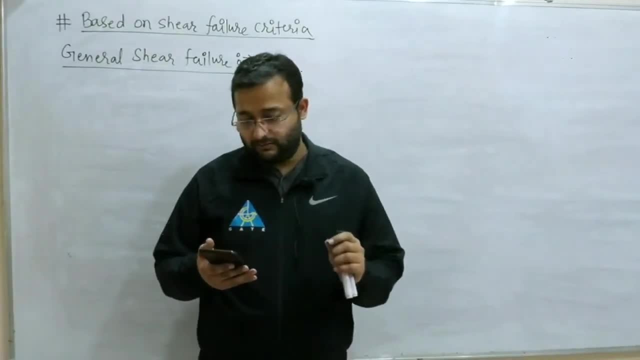 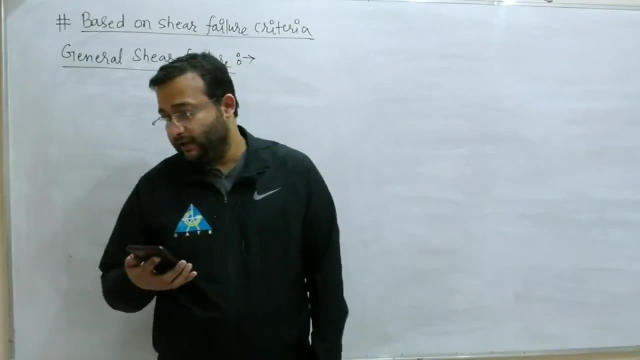 For a minute. the net is off, not net. the light is off. So if the net is off, just give me 10 seconds. it will be covered again. By the way, the class is going on. there will be no problem. 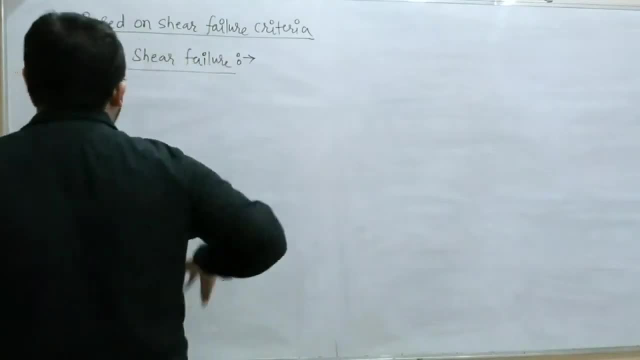 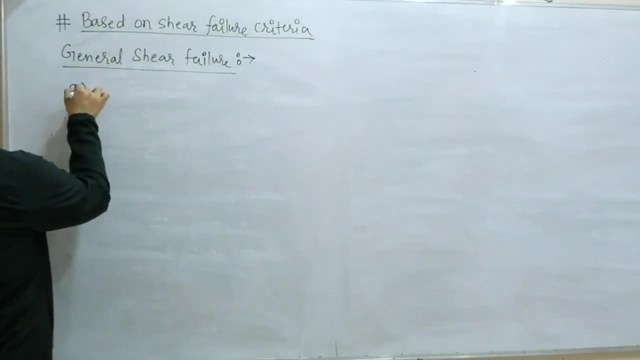 No, the net is not gone. Okay, the class is going on. So I was telling you about General Shear Failure, About this General Shear Failure. I will write some points. Those points are very important. You should note them. 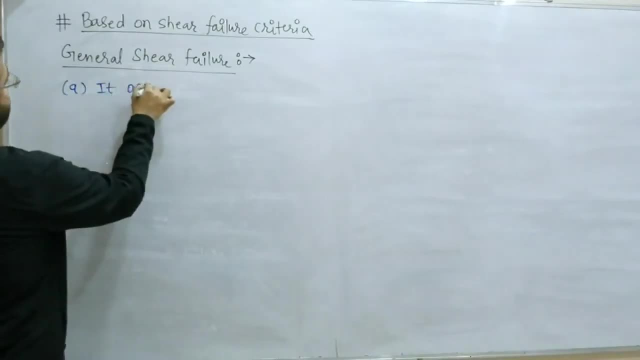 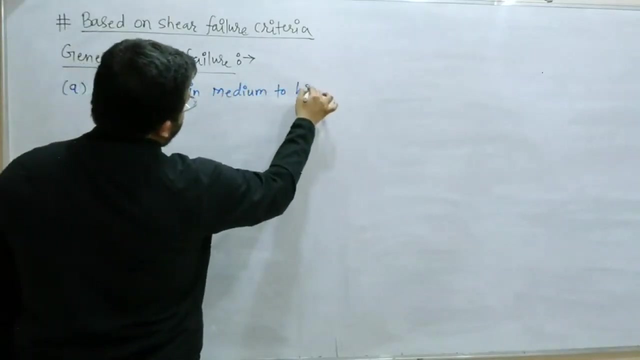 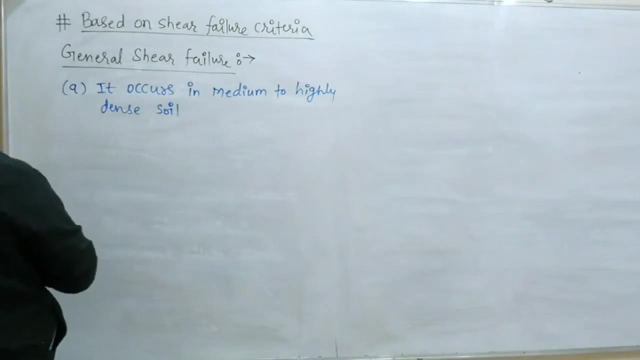 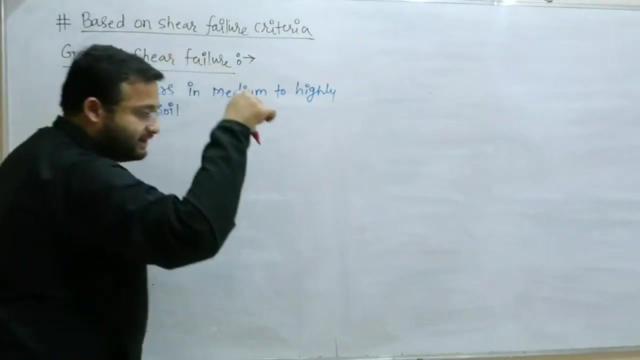 The first point is that it occurs in medium to highly dense soil, In that we will generally see this failure. The second point I am writing is that during failure, when failure is happening, you keep applying the load, keep applying, keep applying. 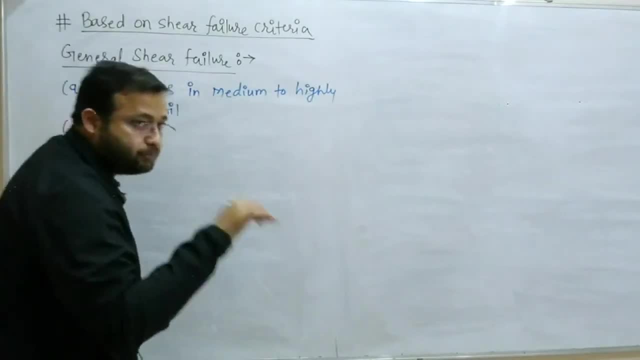 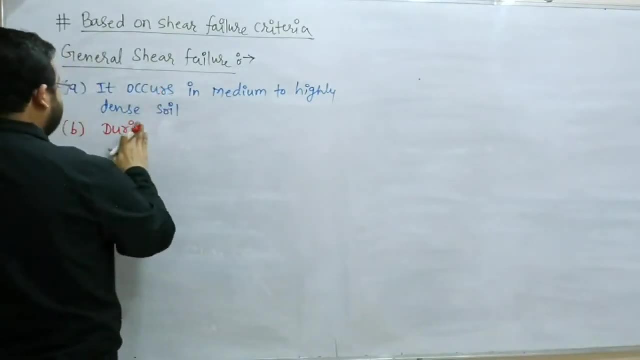 the soil is getting sheared on some load. So, at that time, what will we get to see? During, during failure, during or at the time of failure? I will write this. I will write this At the time of failure. 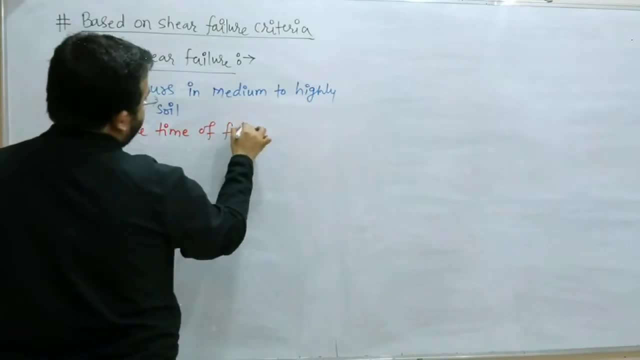 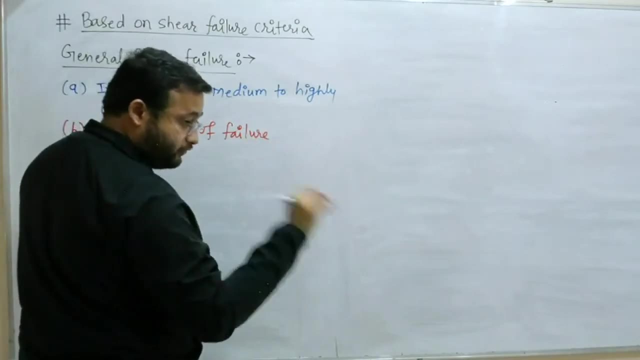 at the time of failure. what will we have to do At the time of failure? we we will get at the time of failure. what will we get? We will get high bulging. We will get bulging At the time of failure. 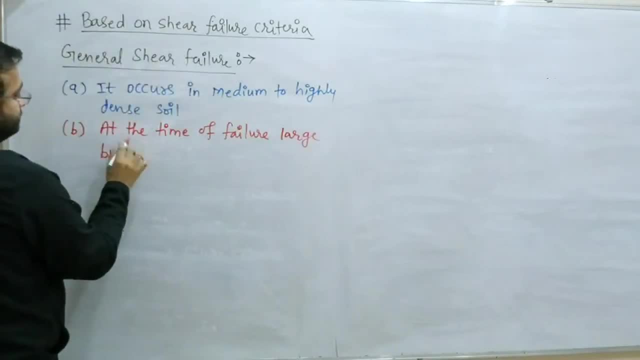 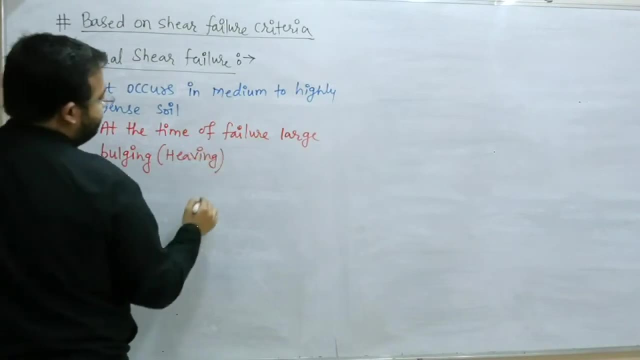 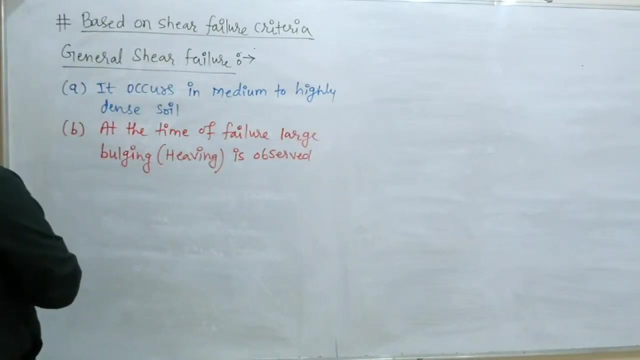 large bulging, large bulging. I will tell you the meaning of bulging now. You can also call it heaving, Large bulging, or heaving is observed. Okay, What is the meaning of this? I am telling you that now. 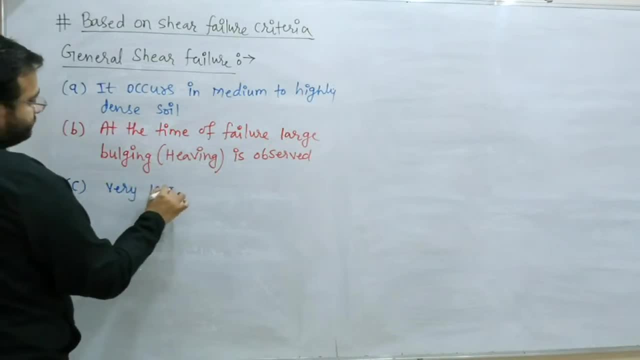 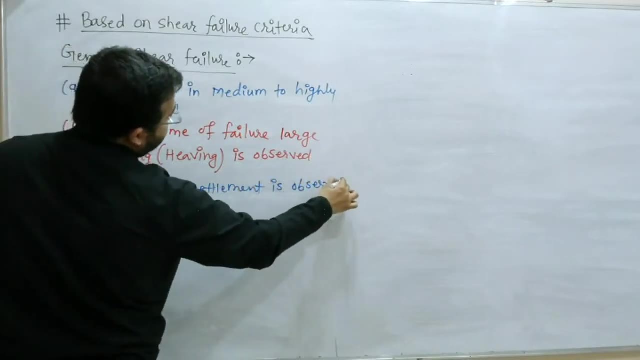 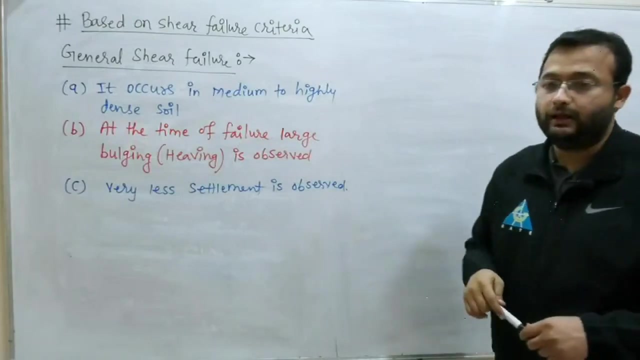 And very less settlement is observed. Very less settlement. less settlement is observed. We will get to see very less settlement here. What is the meaning of all these statements? Let's see. I said here, I said one thing here. I told you here: 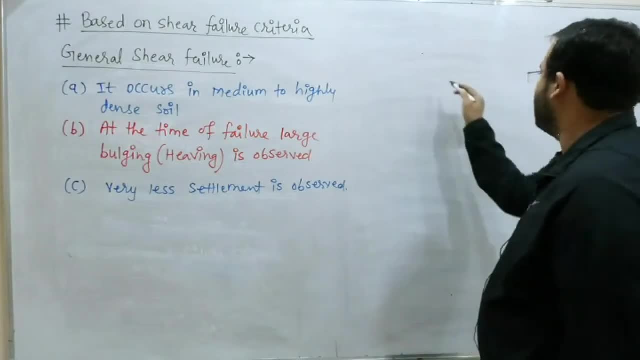 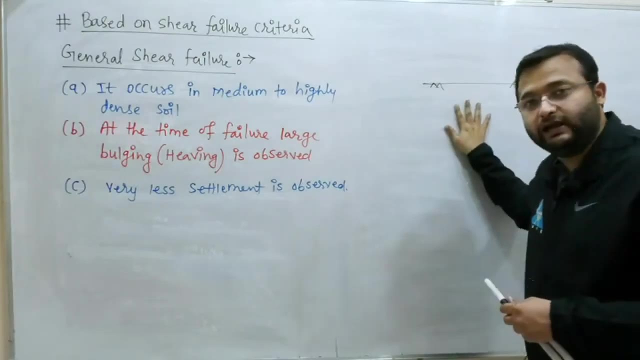 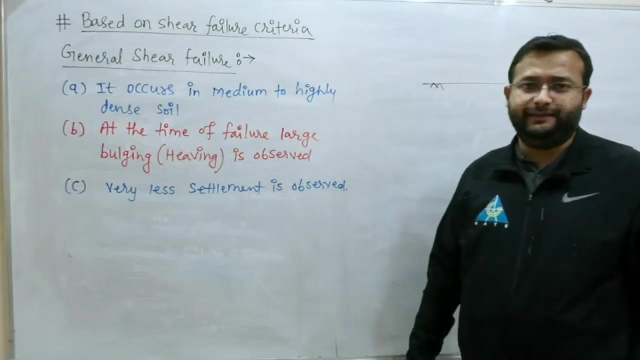 that, brother. brother, I told you that this is your ground surface. What is yours Ground surface? The soil here is very compacted. The soil here is very compacted. The soil here is very compacted. It is very dense. 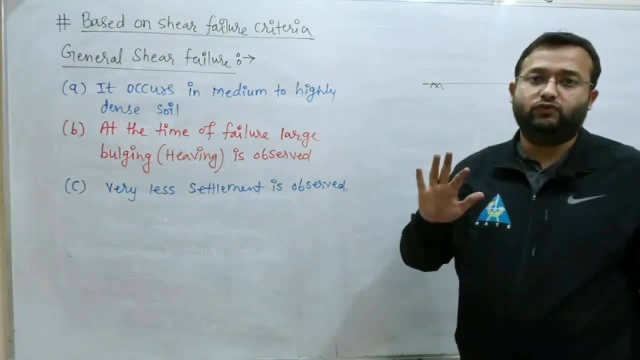 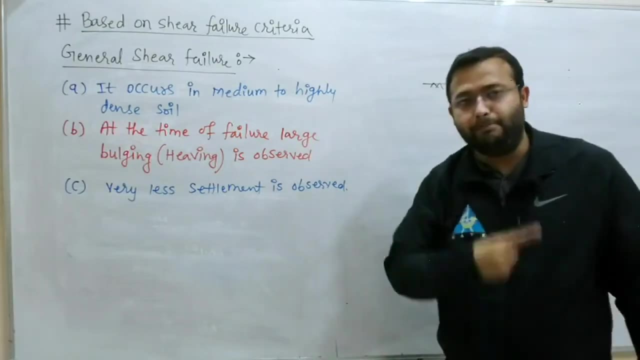 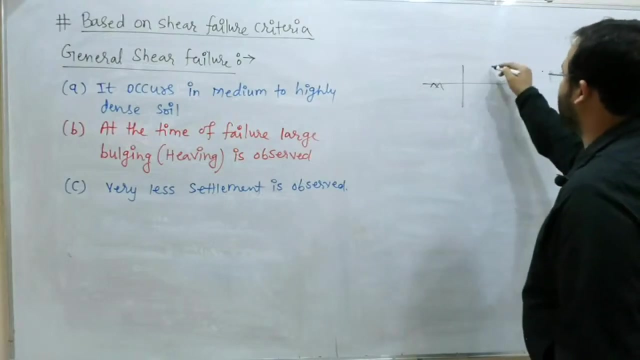 Even I can say that it is well consolidated. It must have been over consolidated in some time, So it is very highly dense. What is the void ratio in this? Very low, There is very low void ratio. Okay, Now, if I get a chance to put footing in this, 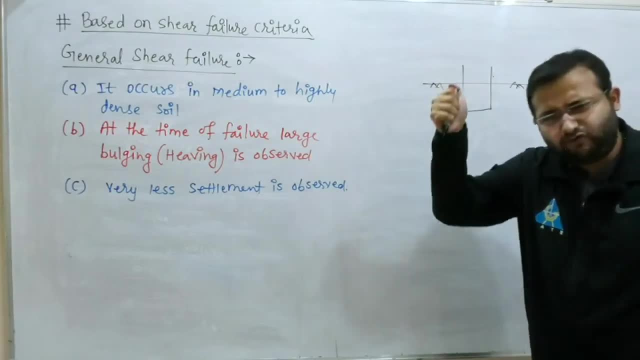 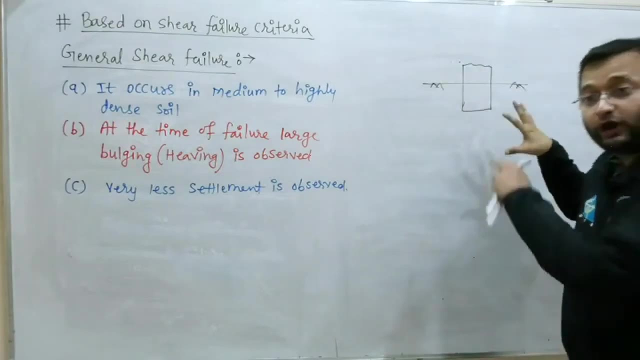 first of all, there is no space in this soil of voids. Still, there is no space in this soil of voids. So what will happen If I am putting footing in this now? the soil was highly dense. then what will happen to the soil? 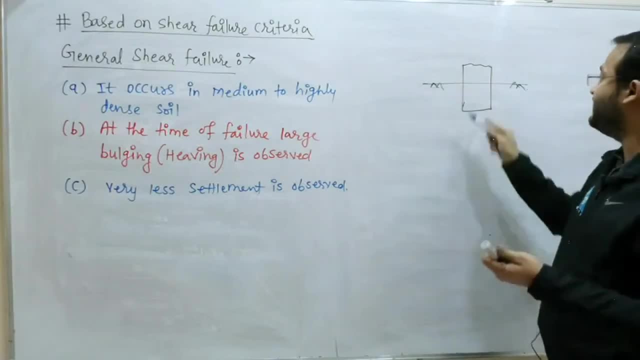 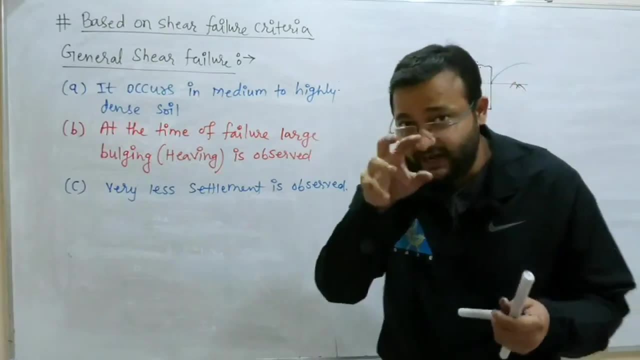 Will it try to come out of here? What will the soil do from here? Will this soil try to come out of here? This is called bulging. Whenever the soil is dense, and if you are putting footing in it, then the surrounding soil comes out. 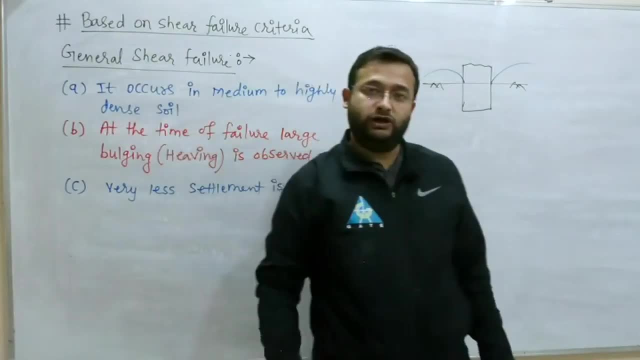 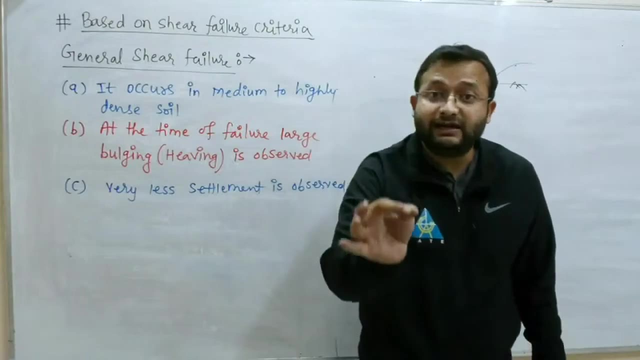 It swells. We call it bulging. So at the time of failure, you keep on loading, keep on loading, keep on putting footing in, keep on putting footing in. at the time of failure, you will get to see a large bulging. 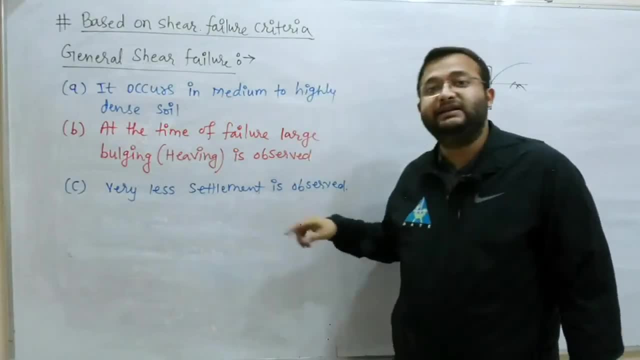 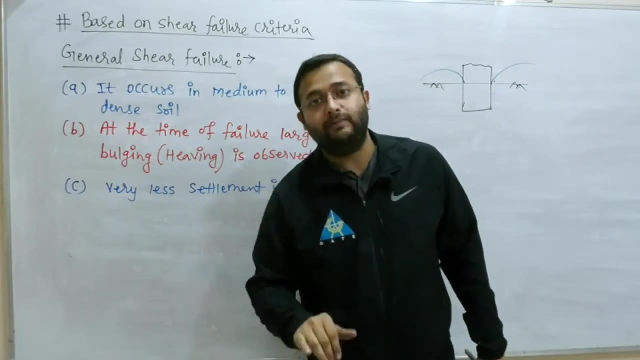 Because you will not get to see any settlement, Or you will get to see very less settlement Because there is no void ratio in the soil. What I mean to say is that it is very low. There will be void ratio, but it will be very low. 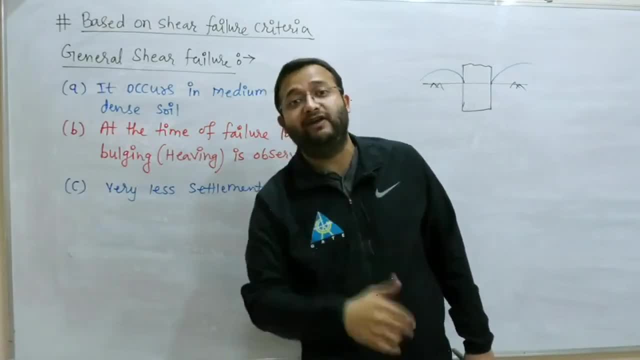 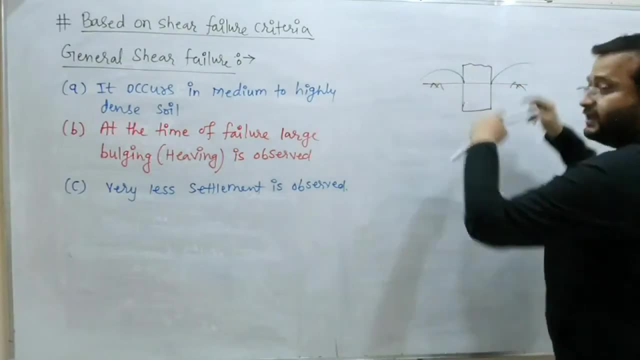 Because the soil is already well compacted, already well dense, already well consolidated. Do you understand? So, at this time, the failure that I am getting to see that the soil is bulging, we are calling it shear failure. What will the soil do here? 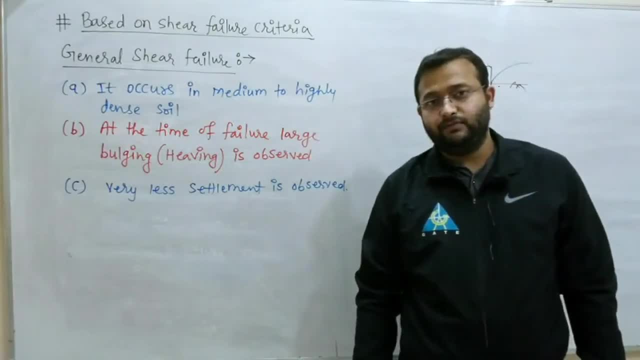 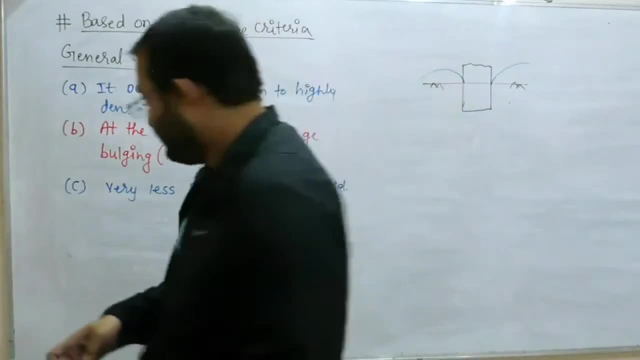 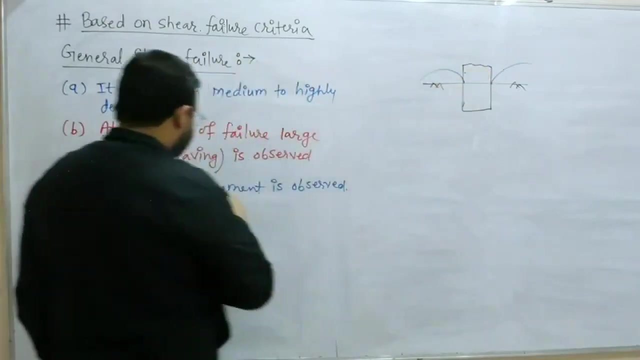 The soil below it can suddenly shear. So that is our shear failure, Or we will call it general shear failure. Notice one more thing in this. I have understood these three statements, These three We will also call this heaving, That the soil coming out is known as heaving or bulging. 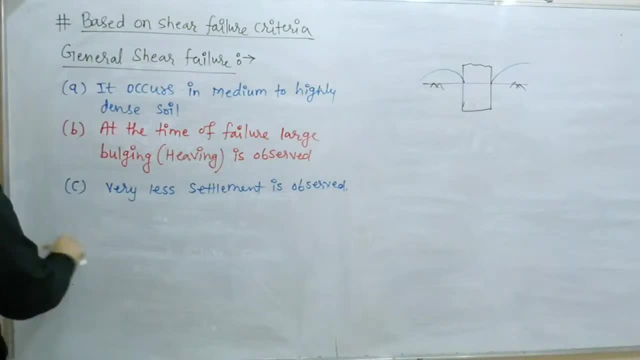 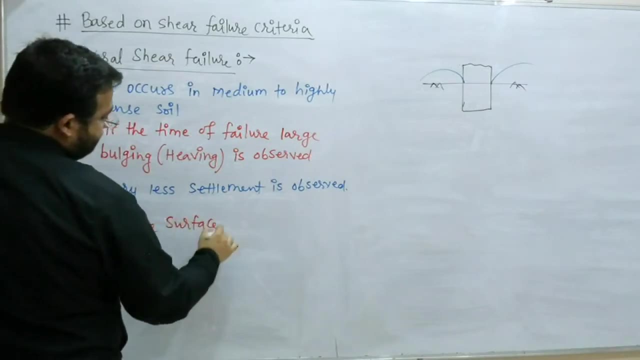 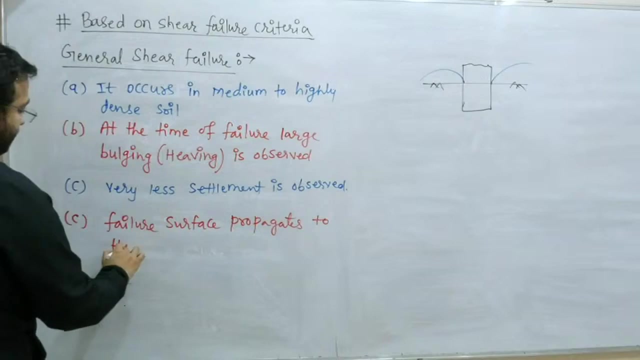 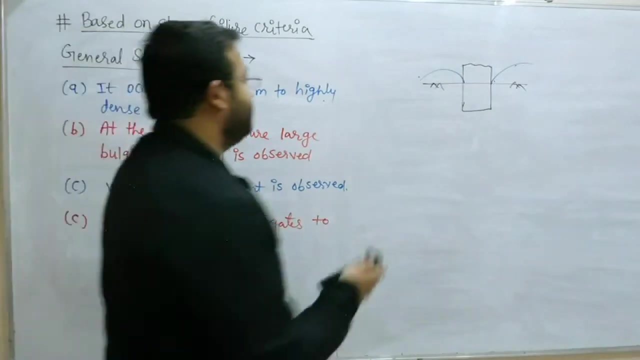 I am adding one more point in this. What is that point? This point is: failure surface reaches to the ground surface. Failure surface propagates to the ground surface. What does this mean, sir? The meaning of this here is that let me assume that I have made a shallow foundation here. 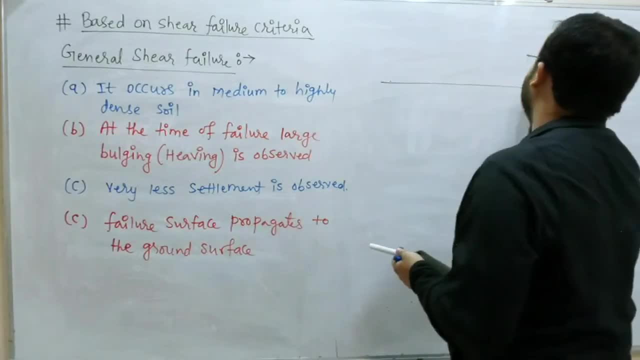 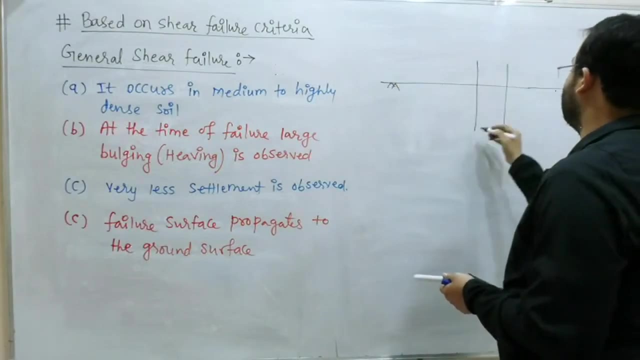 As I say, what do I have? I am saying that I have a ground surface like this And in this ground surface, what have we made? We have made a footing. What kind of footing is this? This is shallow footing. This is shallow foundation. 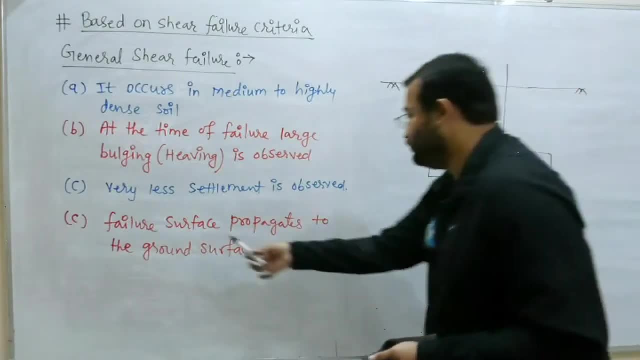 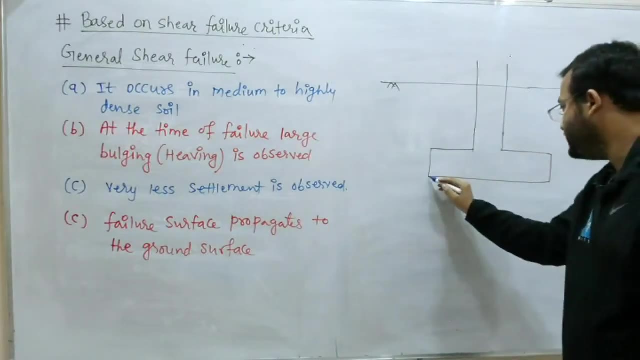 Clear. Here I am saying that your failure surface propagates to the ground surface. Where does failure surface start to meet? Failure surface starts to meet with ground surface. So it comes like this: This is first linear Right. Like this Before some extent. 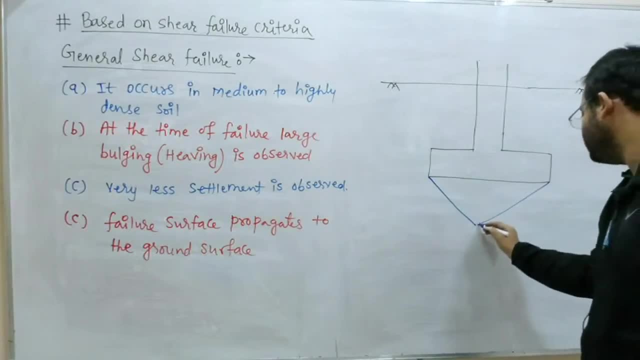 what happens? It is linear: From here to here, And after that it fails, Like this line comes of failure surface. So from here it propagates to the ground surface, From here it propagates to the ground surface. 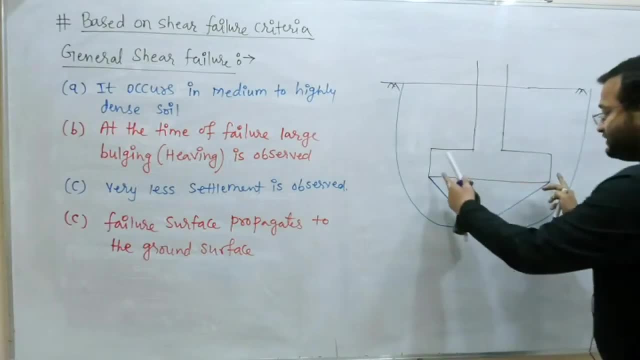 So if you continue to apply load, first you get this much zone of failure. First you see this triangular, you get this much zone. But if you continue to apply load, then this failure surface propagates slowly. And where does it go? 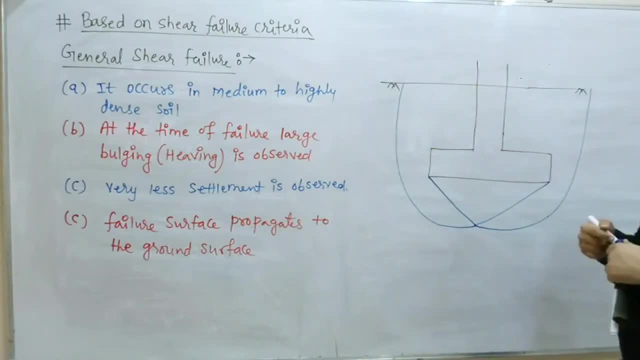 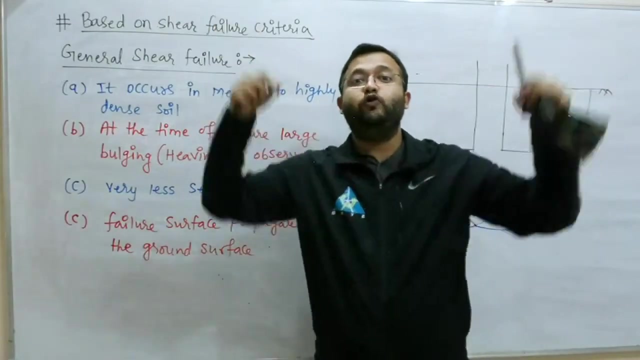 It goes up to the ground surface. Why did it reach the ground surface so easily? Because the depth of foundation was less. What is the depth of foundation here? Less, Because we are falling into this, Falling into the shallow foundation. That is why your failure surface comes to the ground. 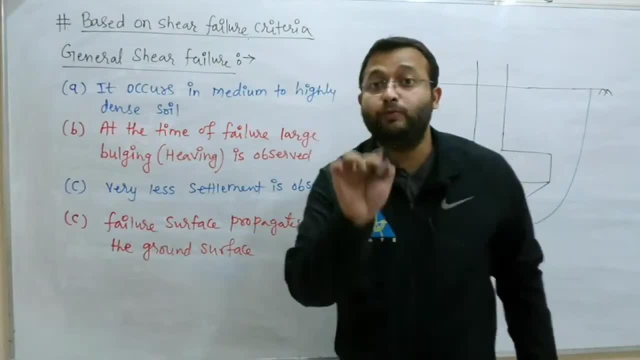 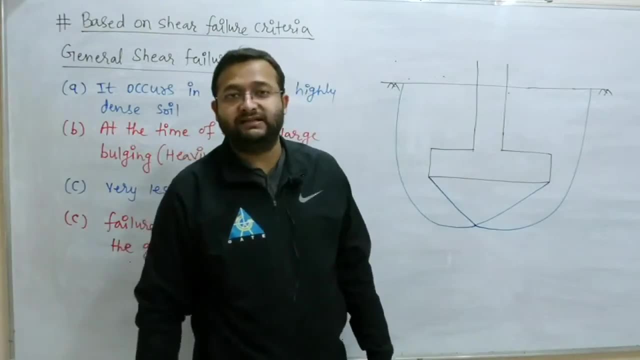 You can see cracks around the footing on the ground. This means that the failure surface has come to the ground. Can I see this Absolutely? You can see it. You can see it 100%, Wherever this failure is happening. wherever this failure is happening. 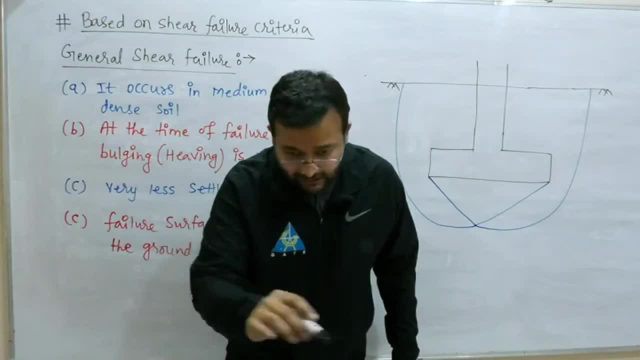 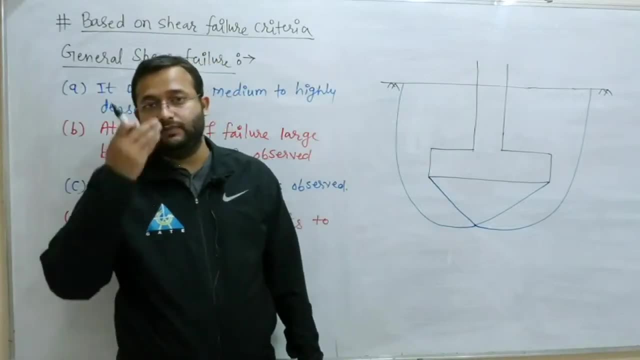 around that ground in the soil to see these little cracks, I will understand that the failure surface has come up. It has reached the ground surface. I will get to see this. Do you understand what I am saying? So this is your general shear failure. 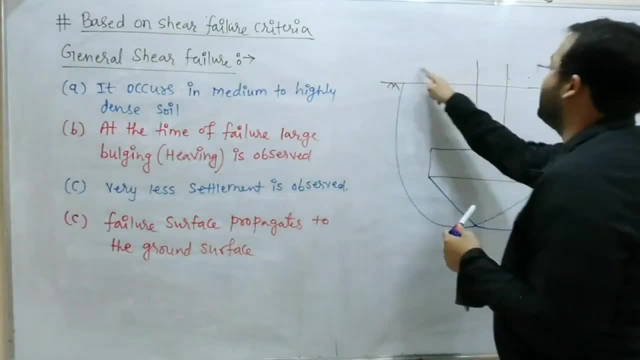 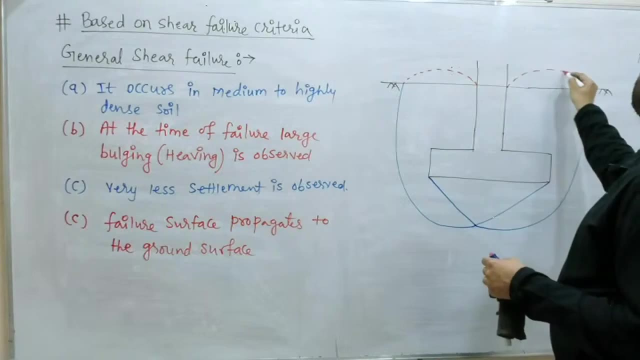 which reaches the ground surface. Okay, What will you get to see at this place? Heaving. What will we call this? What is this? The soil here has come out Heaving. What do we call this? Heaving, If we call this heaving. 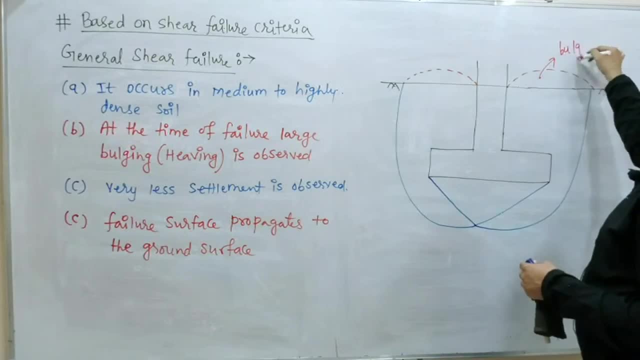 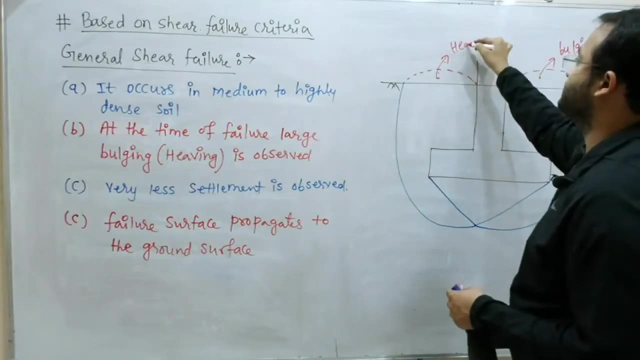 it is called bulging. You can call this bulging or you can call this heaving in its bracket. So I will write heaving here. Both are same things. Heaving or bulging, both are same. Okay, So this was my general shear failure. 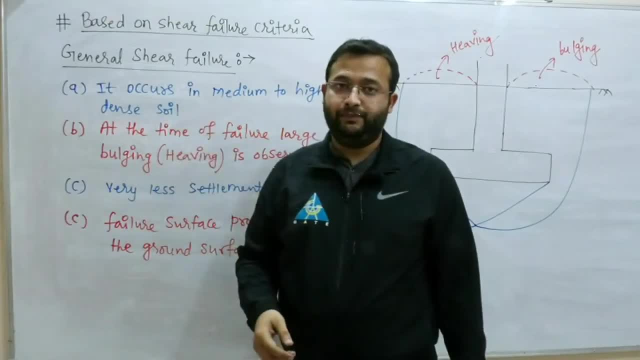 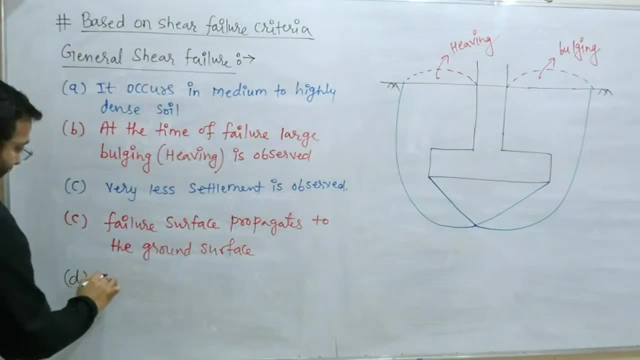 So I told you that this is seen in medium to high dense soil. What soil will we get to see? I am telling you, You can see this in those soils where your angle of internal force is high, Where your angle of internal friction is greater than 36 degrees. 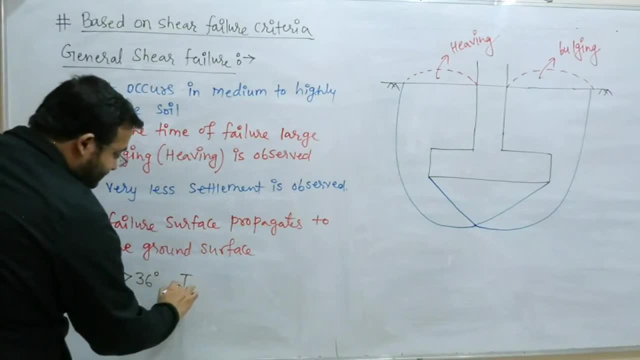 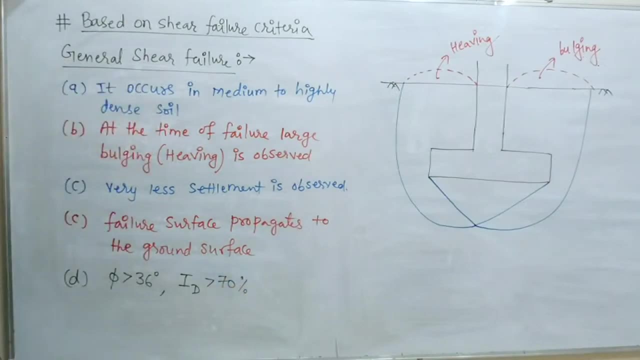 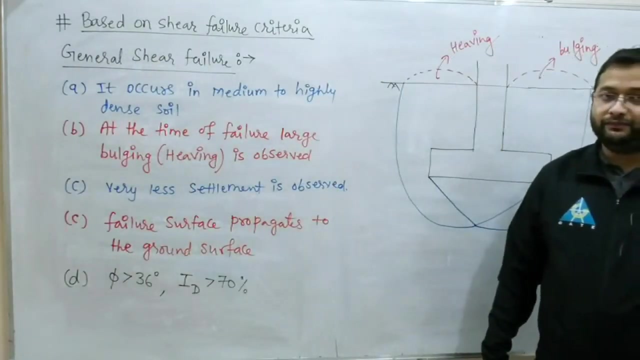 You can see this there. You can see this in those soils where your density index is greater than 70%. You can see this there, Do you understand? So these soils will come in your highly dense soil category and there we will be able to see it easily. 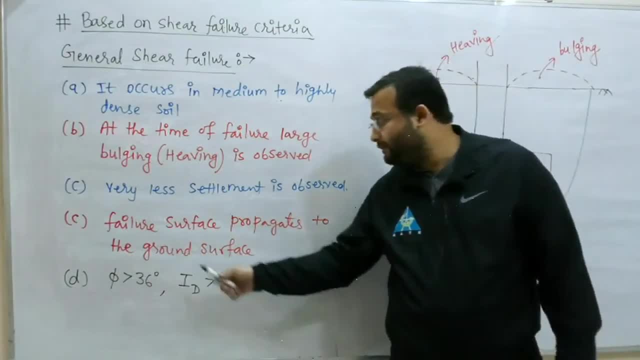 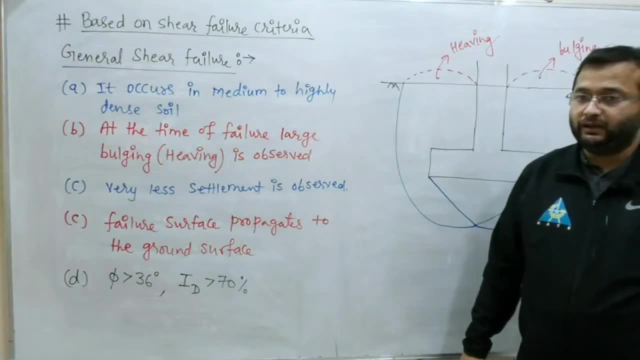 Your void ratio where it is less than 0.5, there also you will get to see general shear failure. But this is not a fixed parameter. But, yes, we have complete information about this Clear. So this was your general shear failure. 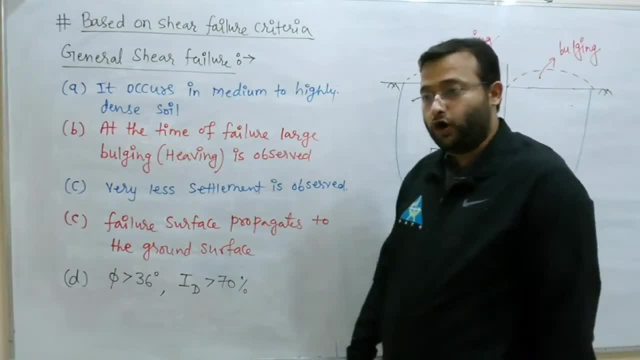 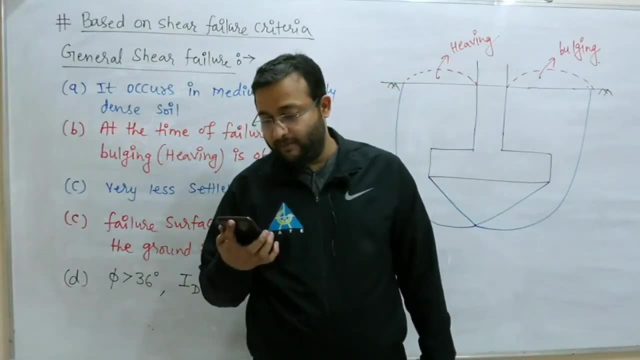 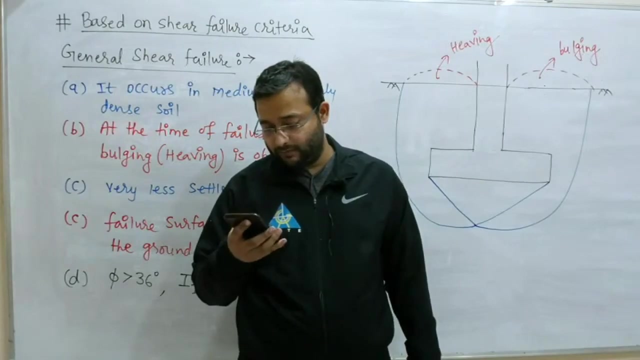 So whenever I have to make footing, or whenever I have to make footing and I am getting to see that my soil is present in a highly dense place, then what will I do there? Then? if highly dense is present there, right, If there is soil there and if it is present there. 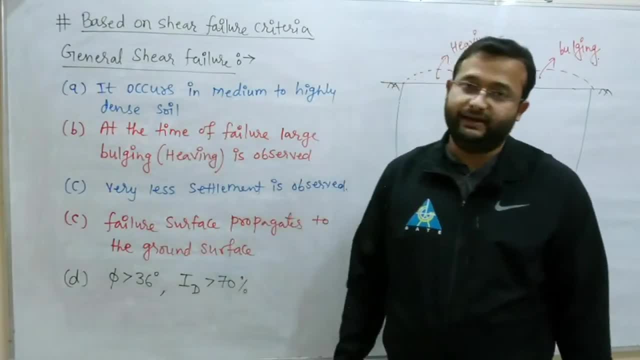 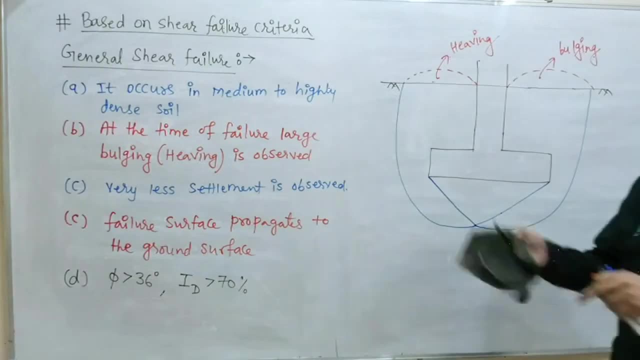 then you will be able to see general shear failure there. Do you understand what I am saying? So we have got everything clear. Come, let us move ahead. You can take a picture of this. I will rub the board number 2.. 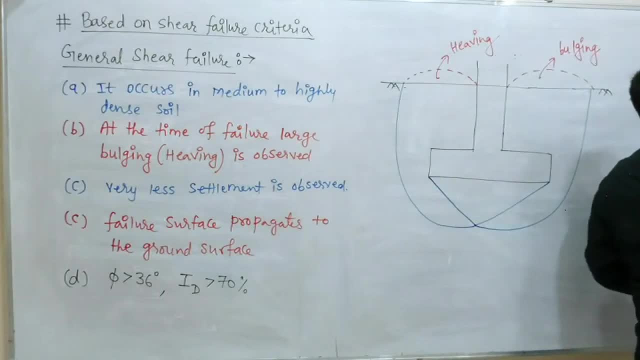 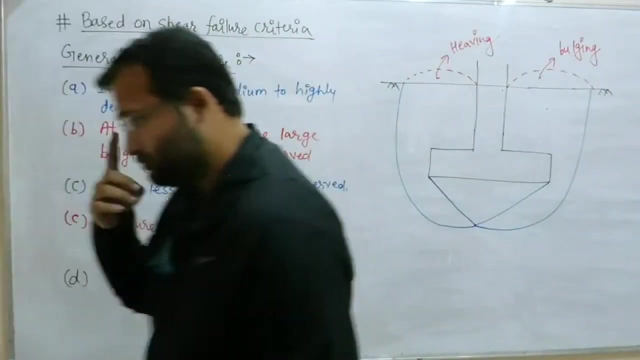 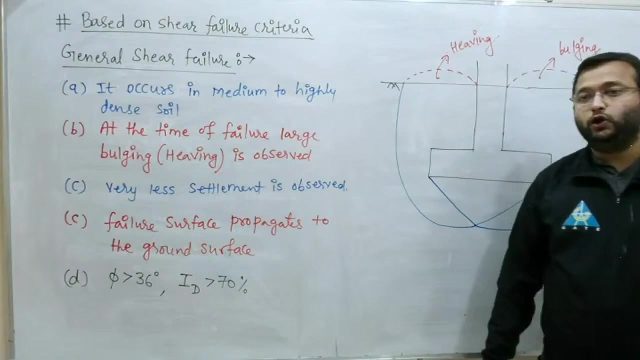 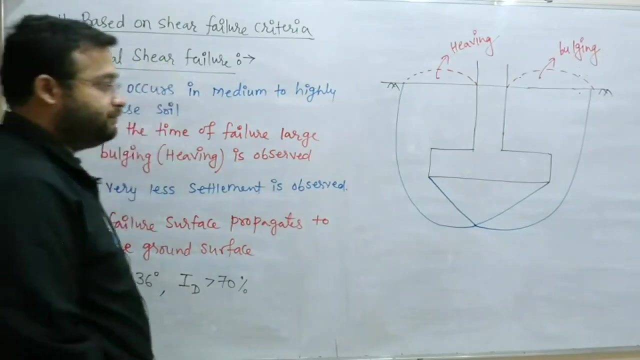 Okay, I will rub the board number 2.. You guys must have taken a picture or screenshot. Next type of failure that I have is called Local Shear Failure. I will write this as first number. Right, I will write first number: general share failure. next, what I have is local share failure. 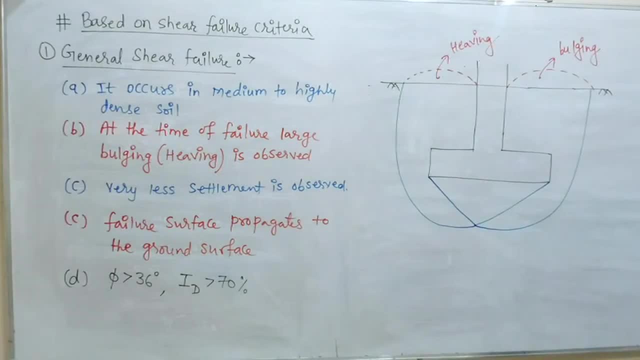 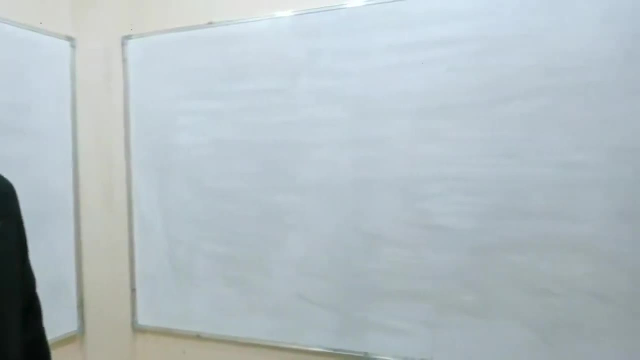 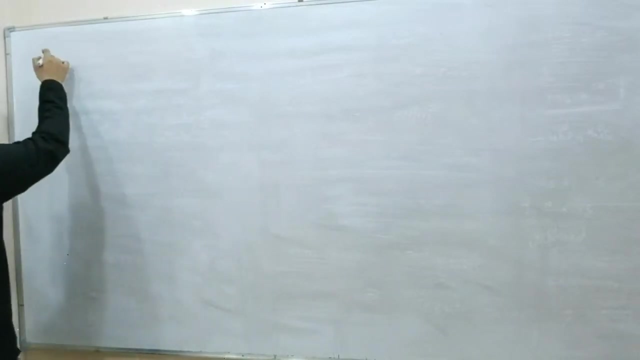 Should I remove it? Okay, you must have taken the photo, you must have taken the screenshot. Come, let's talk about the next type. I will move ahead. next I am talking, and that is your local share failure. Local share failure. 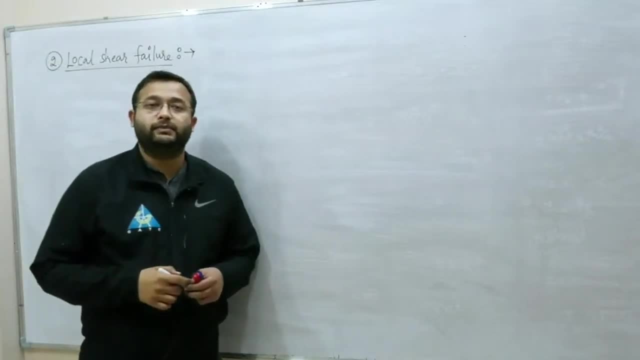 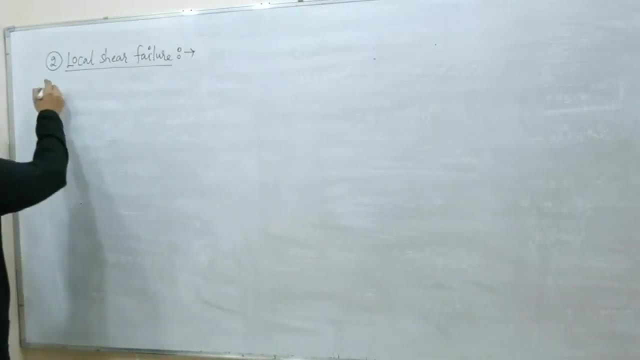 Right, If we are talking about local share failure. if we are talking about local share failure, then let me tell you which soil it will be on. So local share failure is on loose soil. Okay, so I have written a point here. 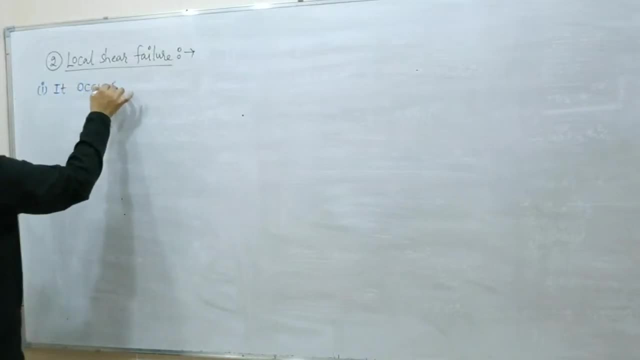 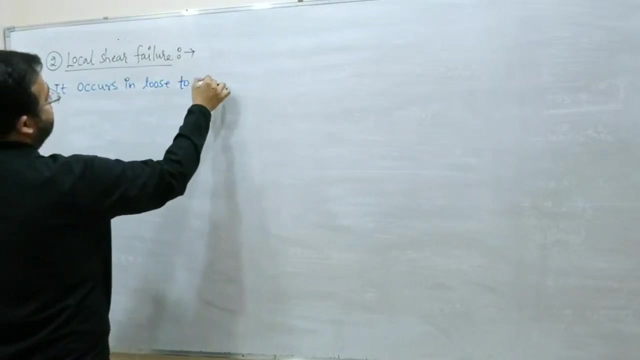 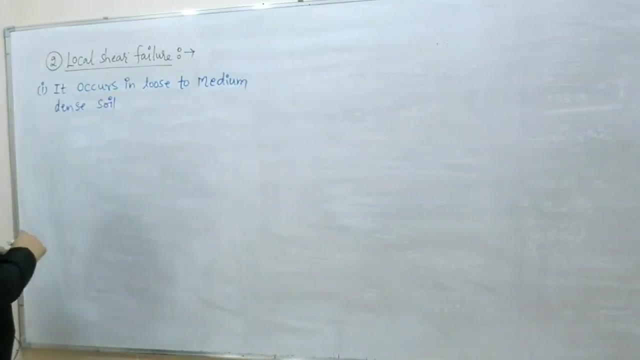 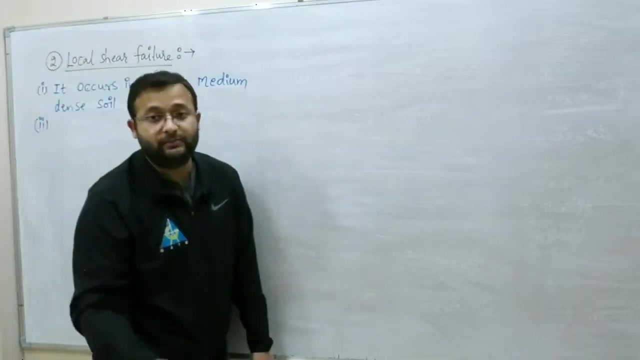 Okay, It occurs. it occurs in loose to. it occurs in loose to medium dense soil. We get to see this in medium dense soil only Now. here we will get to see large settlement at the time of failure, but we will not get to see bulging or we will get to see very less bulging. 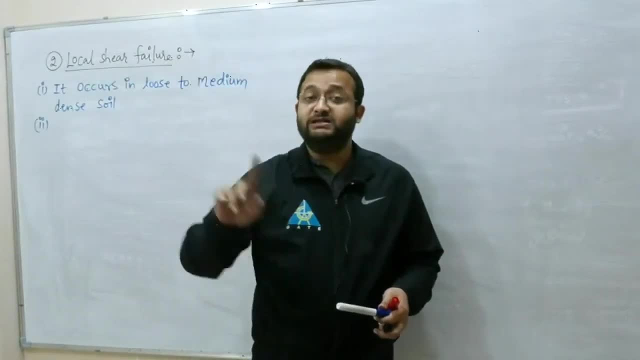 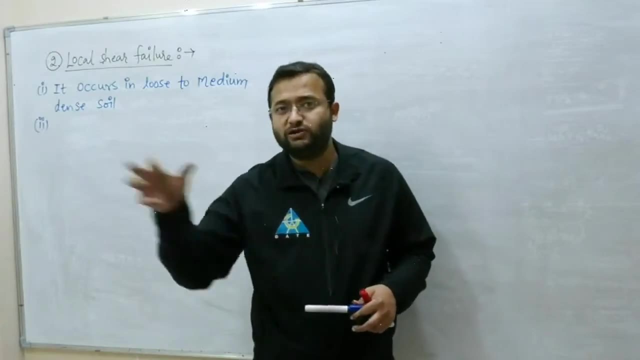 So in general share failure, just opposite condition is showing What was happening in general share failure: That I was having large bulging and less settlement was coming Because the soil was highly dense. What is the soil here? It is loose. 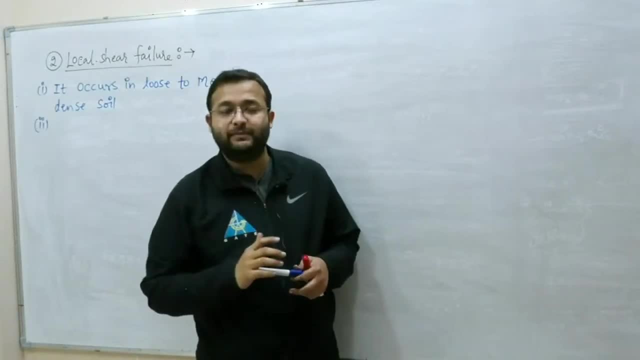 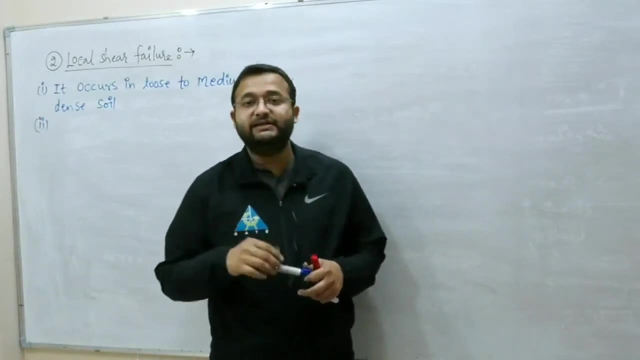 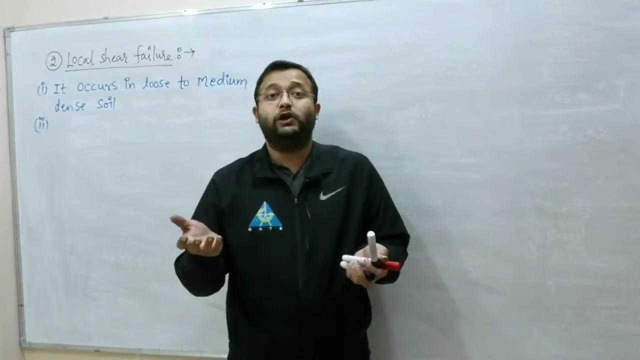 Or it is medium dense, I can say, Or it is loose, I can say. So. in such conditions, in such conditions, what will be happening In such conditions? it will be happening that, brother, you will get to see large settlement, as the soil is loose. 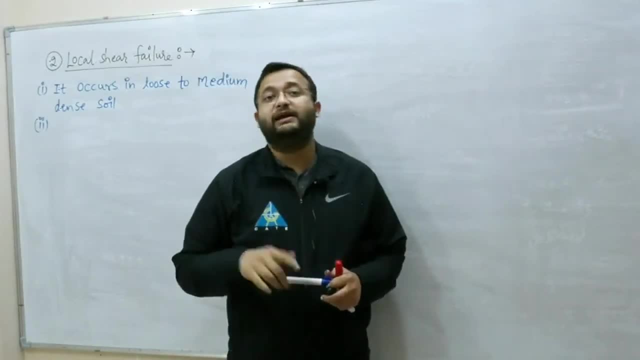 You are adding loads, So the settlement is coming continuously. But if the settlement area is coming, then the soil is settling. Then from where will the heaving happen? From where will the bulging happen? It will not happen. 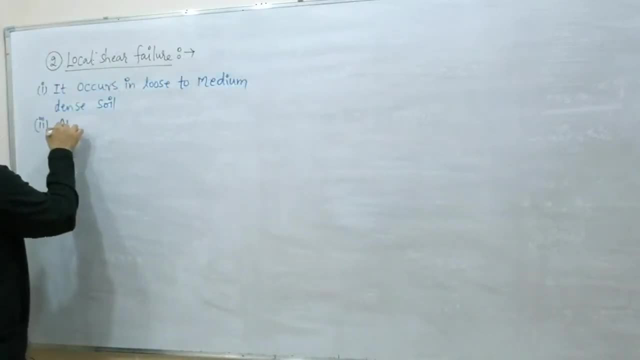 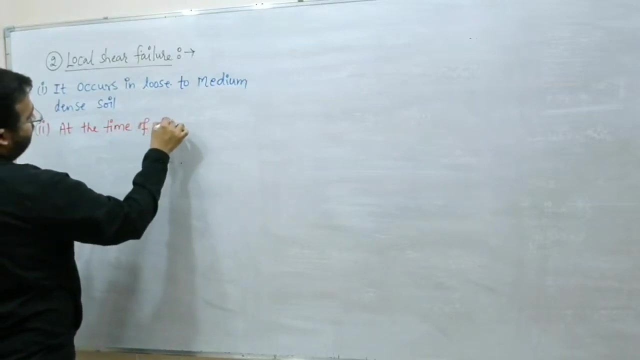 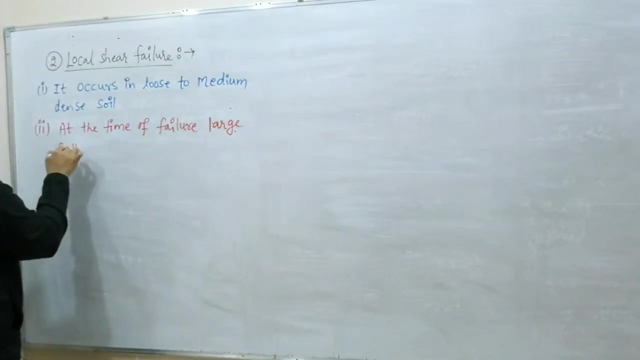 So here I am writing at the time of failure. we have written here what we have written here at the time of failure. at the time of failure, time of failure, large settlement is observed. third point: no bulging or very less bulging. 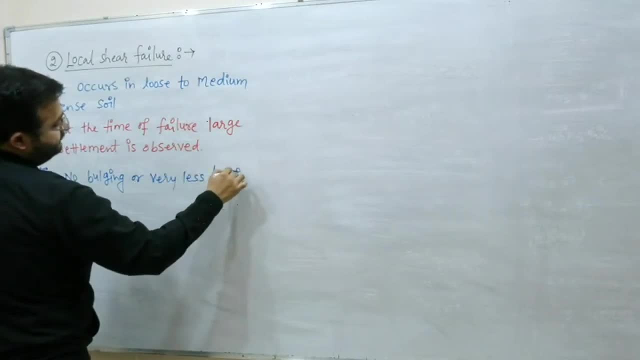 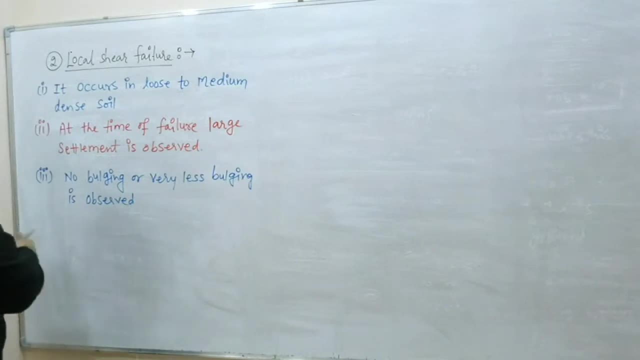 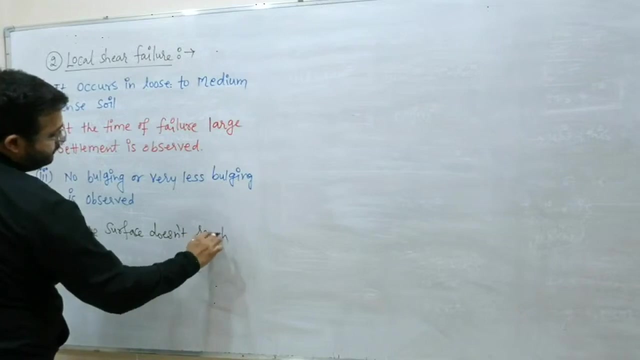 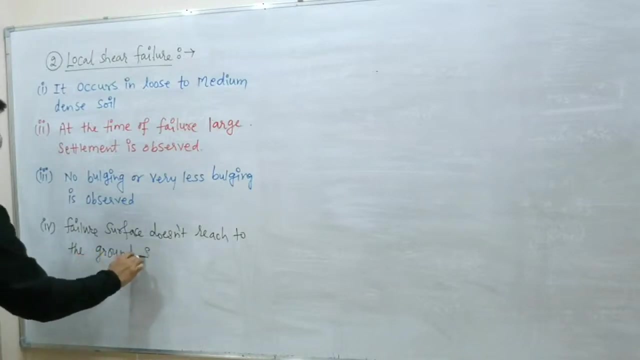 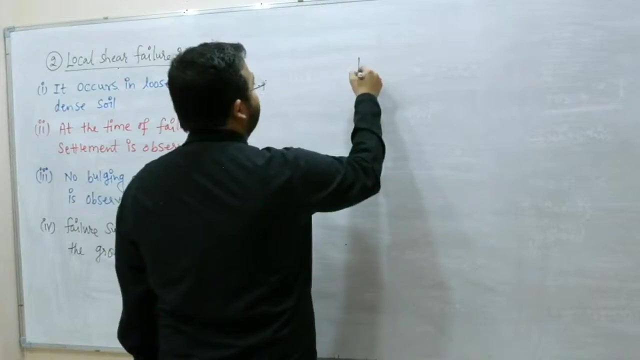 is observed Clear. Next point: I am writing that your failure surface does not reach the ground surface. Here, failure surface, failure surface does not reach the ground surface. It means failure surface does not reach to the ground surface. Now, what is the meaning? is this, like I told you that, what do we have? we have a shallow foundation. This we has. 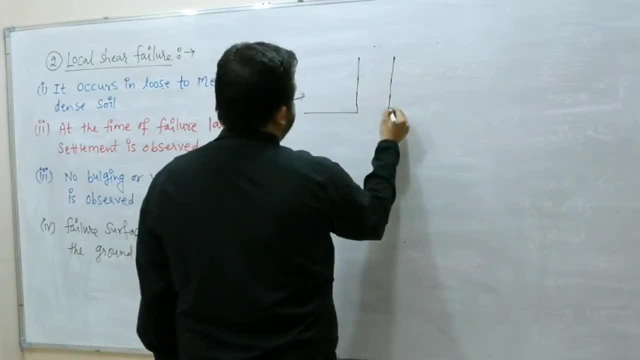 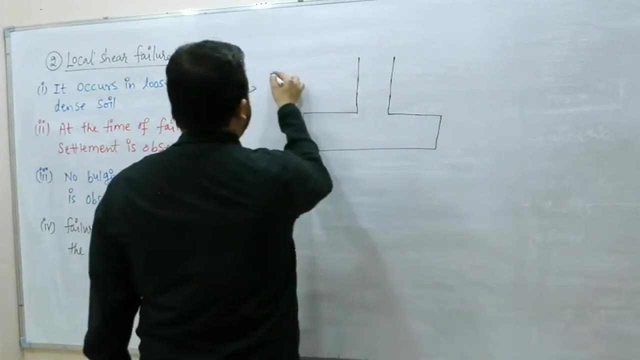 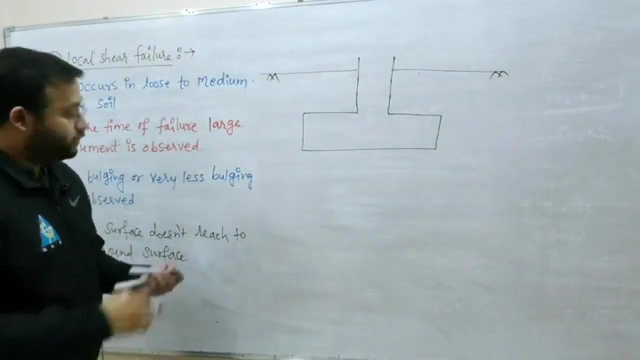 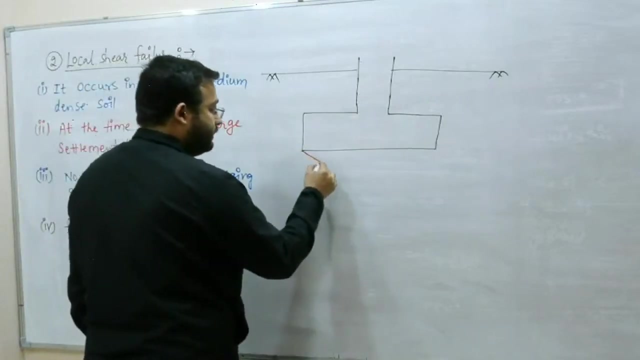 foundation here. We have made a shallow foundation here. What have we done? We have made a shallow foundation here. I assume that this must have been your ground surface in some way. Am I saying it correctly? So the failure surface here cannot reach the ground surface? Why? 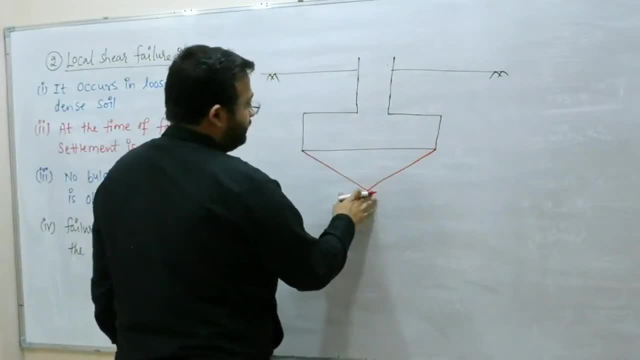 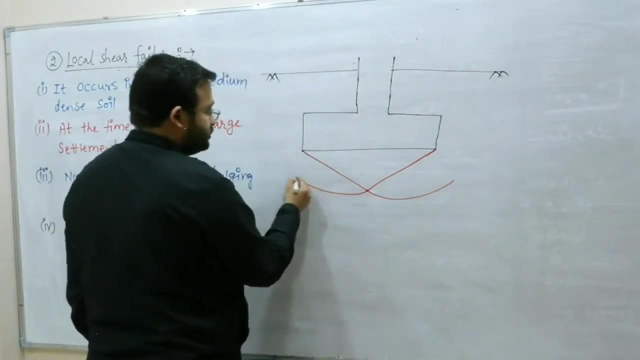 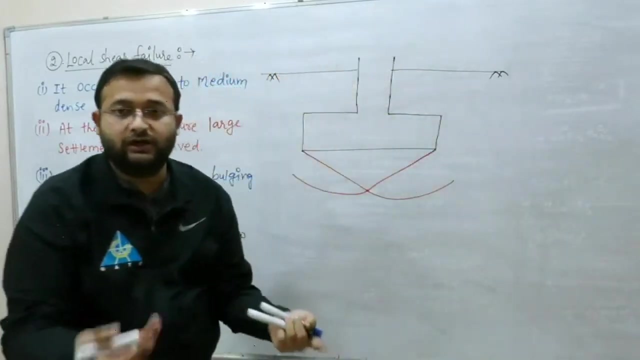 cannot reach. I will explain it to you. This is your failure surface. This failure surface came from here. It tried to reach to the surface but could not. Why? Because continuously the footings are settling, So the failure surface is not reaching to the ground surface. What 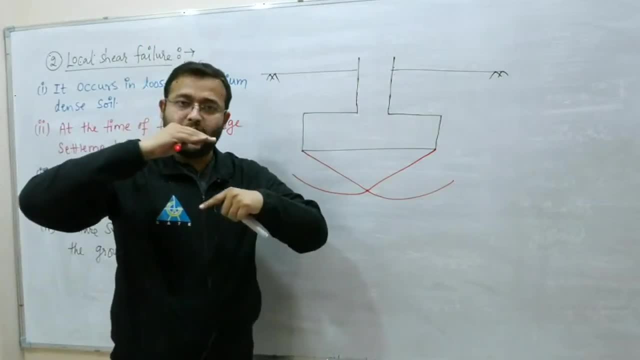 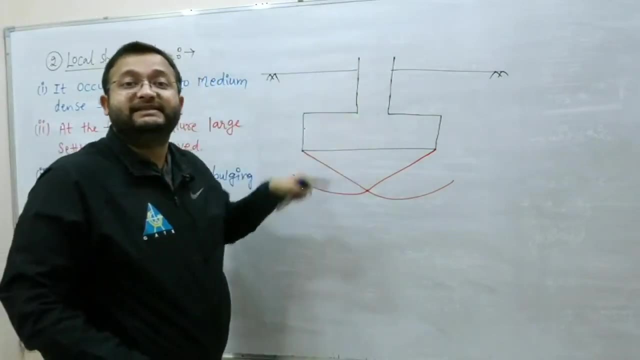 was happening there in the general shear, failure Settlement was not happening. Even then the load was continuous. So the failure surface reached the surface. Here also the load is continuous, Settlement occurs, The load is continuous and the failure surface is also. 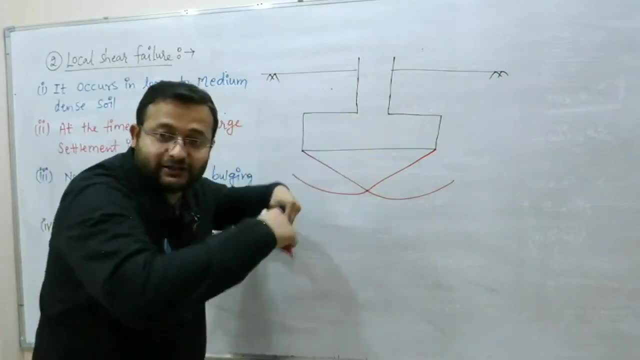 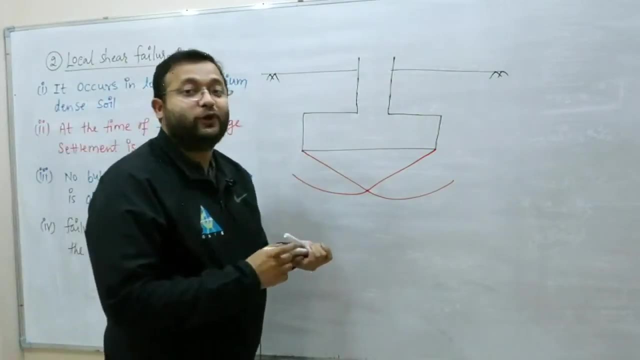 Because the soil was loose, the filler surface is not able to come up because the footing is going down. Do you understand what I am saying? So, due to this reason, because the soil is continuously settling here, there were a lot of voids. the soil was loose. 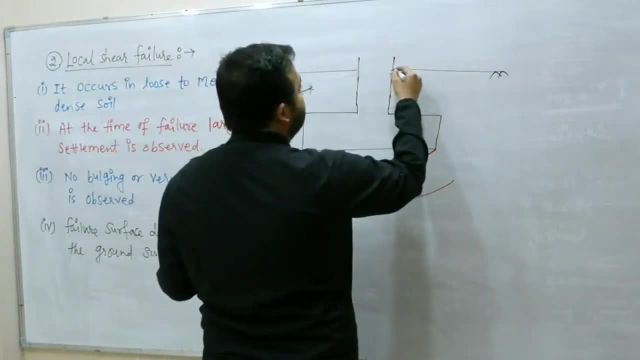 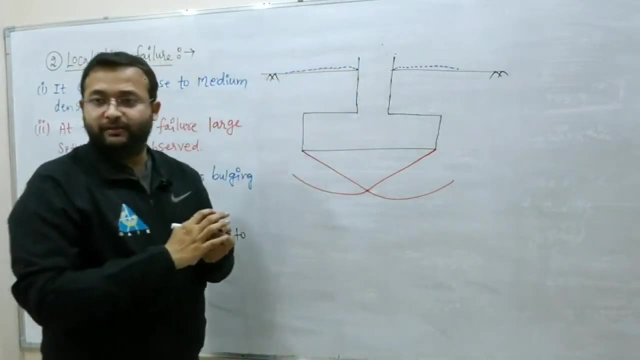 So here we will not get to see bulging, And if we are getting it, then we will get very less bulging. Right, We are getting very less bulging, So you can write no bulging or very less bulging. 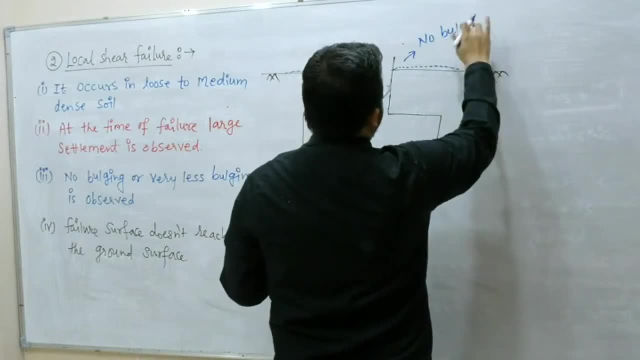 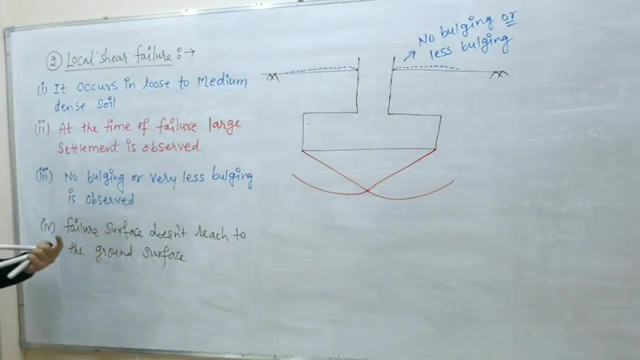 Here I have written no bulging, no bulging or less bulging. I can write like this: here Is my answer clear. Yes, sir, your answer is clear. In which type of soils can we get to see this? So we can say this: 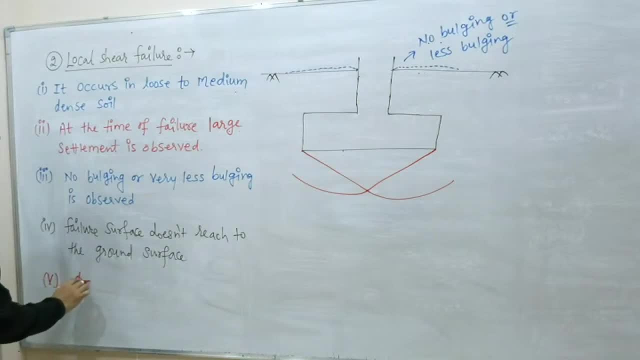 we can say this, that when your angle of internal friction comes to less than 28 degrees. and density index. I had taught you this density index in the beginning lectures when I was teaching in chapter number 1.. Then we had told you about density index. 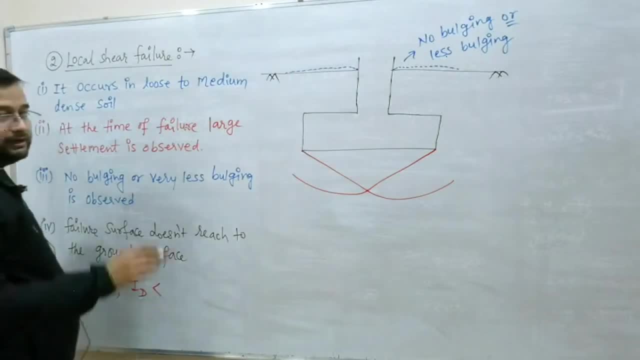 that? what is density index? E max minus E, divided by E max minus E minimum? I had taught you this, So we also know density index as relative density. When density index comes to less than 20%, then we have local shear failure in our soil. 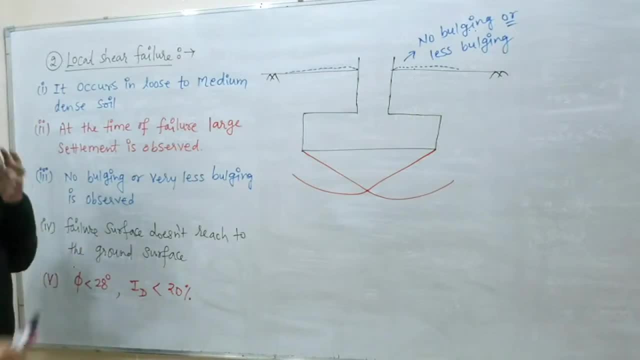 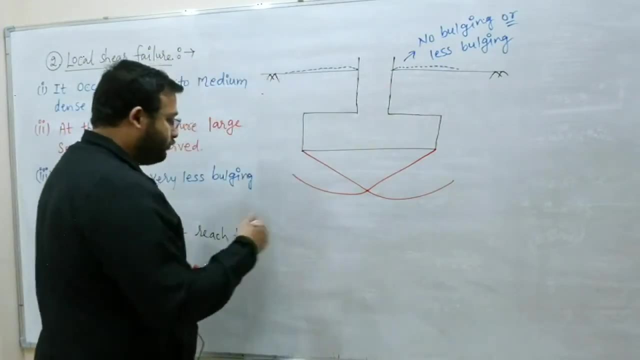 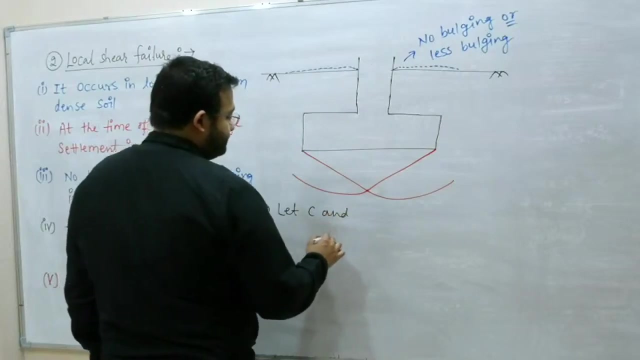 We can see this in our soil. Okay, So this was about our local shear failure. I am introducing one thing here and I am saying that let I have written something here- let C and phi. let C and phi are the. 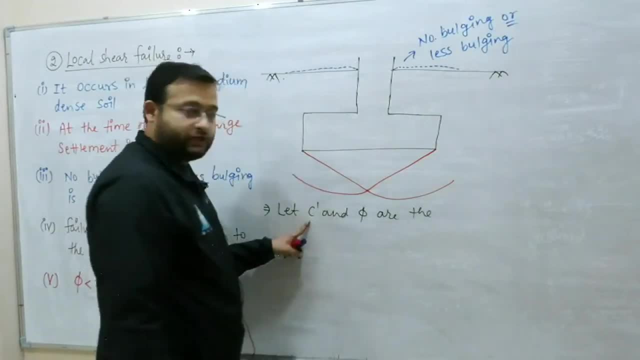 or I will write C? dash- effective shear strain parameters. C means cohesion, phi means angle of internal friction. It has one more name: angle of shearing resistance. So I was telling you C? dash and phi dash are the effective shear strain parameters. 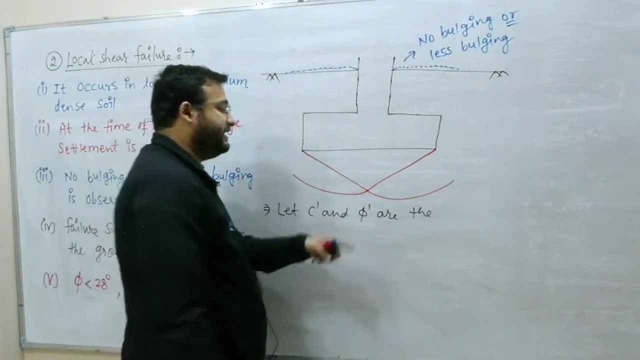 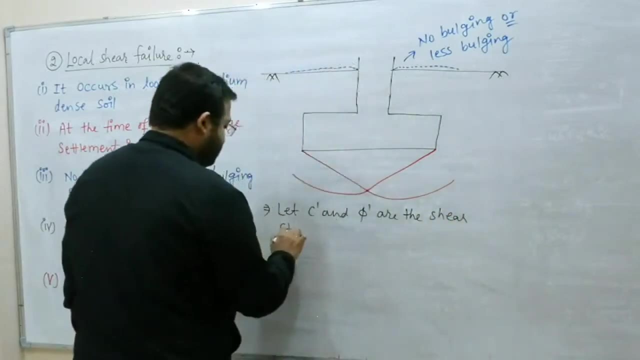 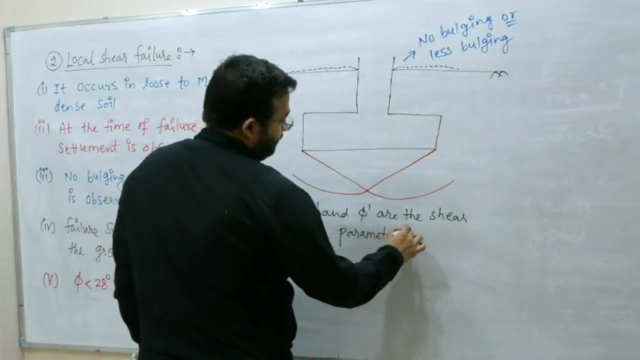 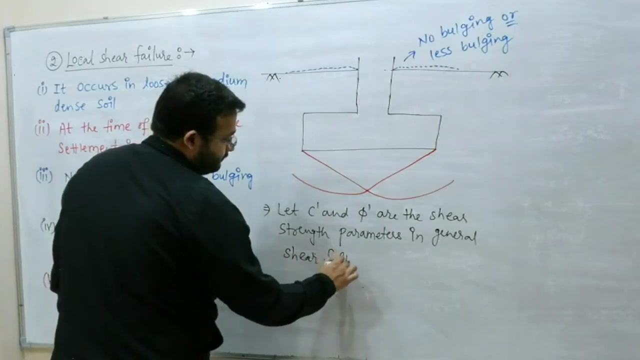 In which case, In general shear failure. So let C dash and phi dash are the. are the shear strength, shear strength parameters, shear strength parameters in general: shear failure, general shear failure. Then you know, general shear failure. 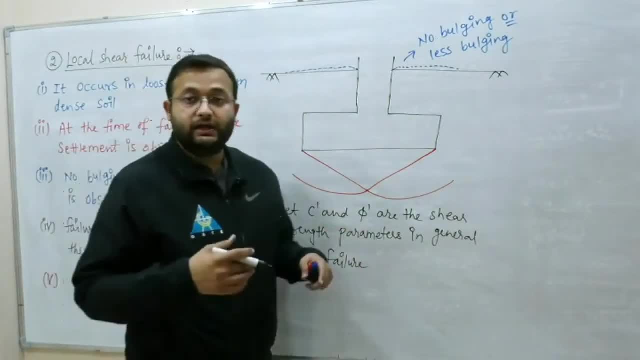 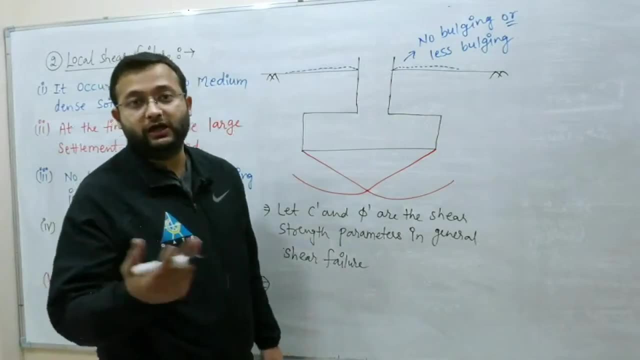 What did we say? We agreed that C dash and phi dash. what are they? They are shear strength parameters in general, shear failure. What will be their values in local shear failure? So I am saying that in local shear failure. 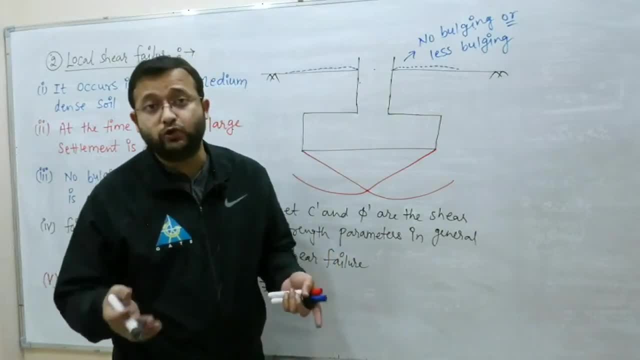 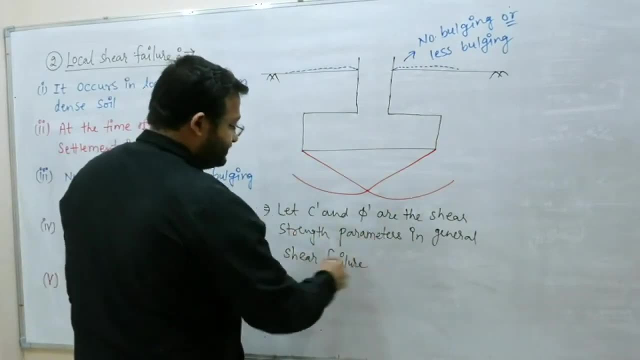 these values will be slightly modified. They will be reduced because the soil gets loose in local shear failure. So we will reduce the values. So let C dash and phi dash are the shear strength parameters in general. shear failure Then. 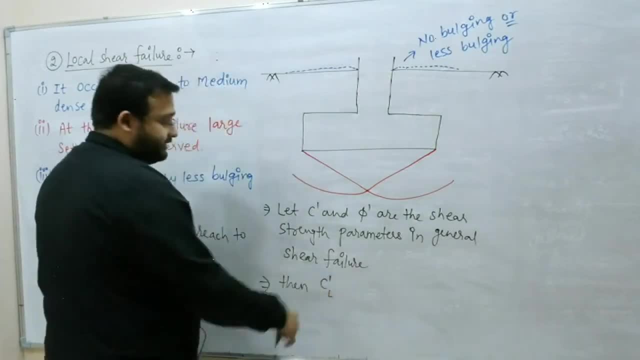 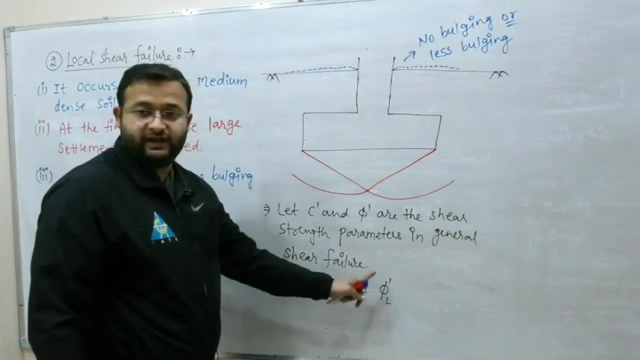 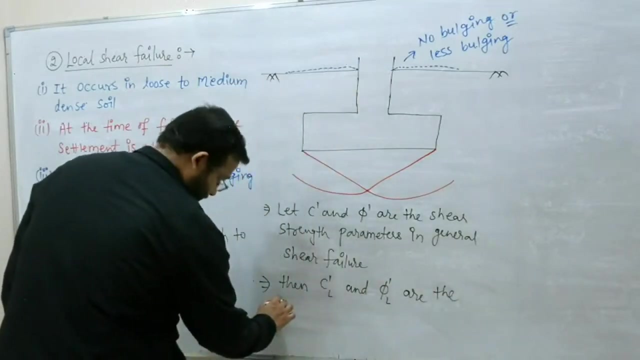 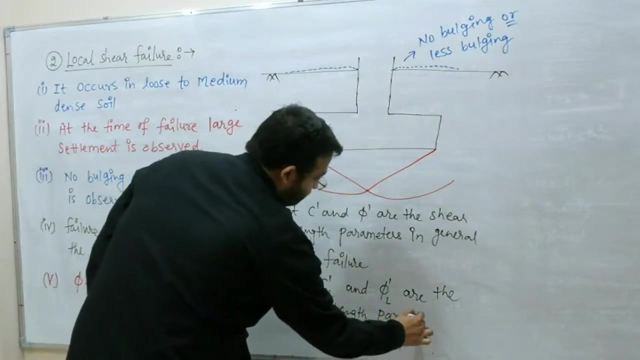 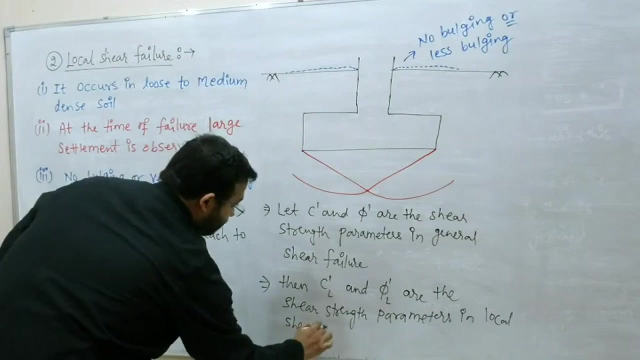 C? L means in local shear failure, effective cohesion and your phi local in local shear failure, phi dash. are the shear strength parameters in local shear failure? Are the? are the shear strength parameters? are the shear strength parameters in local shear failure? 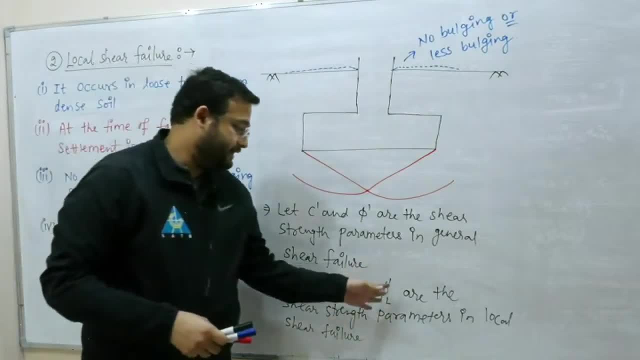 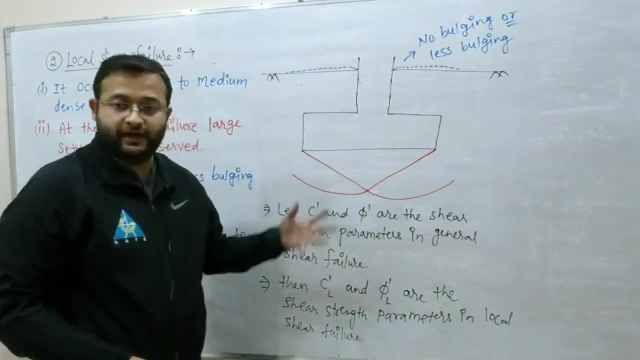 Are the? are the then C dash and phi dash? are the L, L are the shear strength parameters in local shear failure, So in general shear failure and in local shear failure. So what will be the difference between the two? 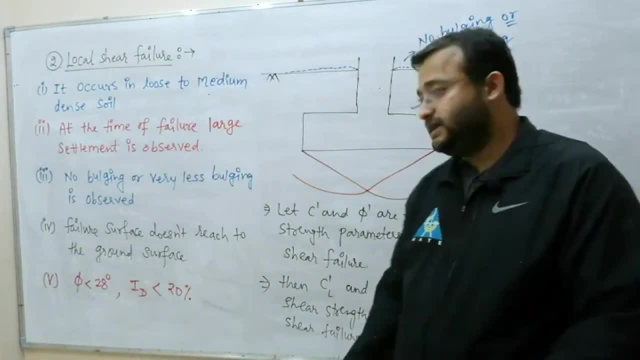 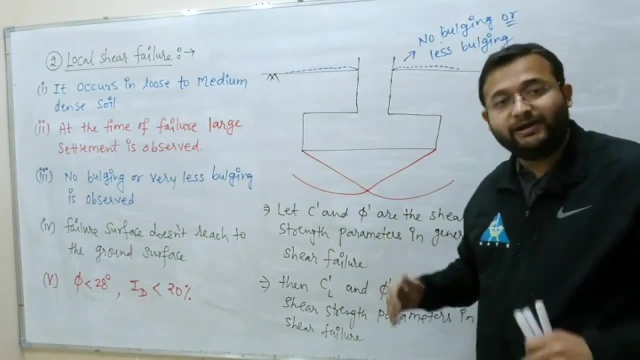 Will there be any difference? Definitely there will be a difference here, And the difference will be that the ratio of the- actually, when I talk about theiez Roman, it will be like this: The ratio, this is the ratio of the moisture. 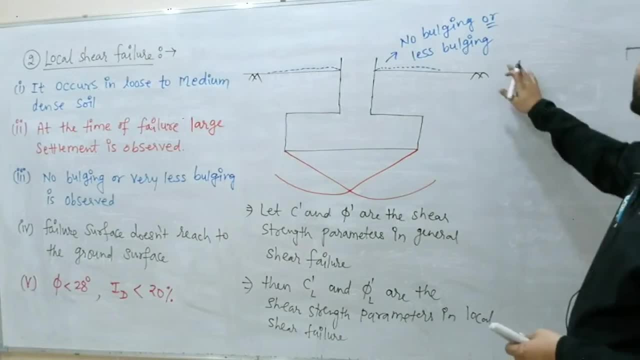 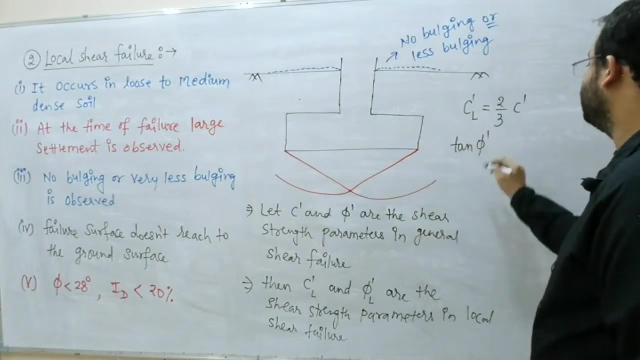 and the ratio of the it will be equal to an большification. It is a flat period of 실 on coverage but if I talk about it and if we talk about angle of internal friction, then 10 phi dash of local shear failure will. 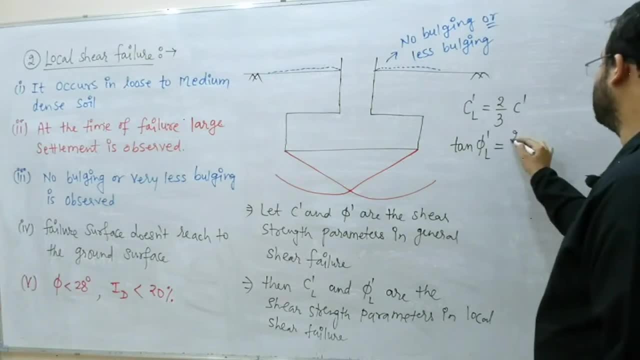 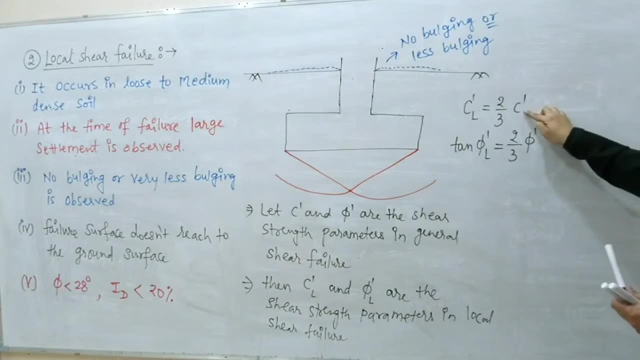 be taken as two-third will be taken as two-third of phi dash, of general shear failure. so see here, and it is correct if you write C' L equal to two-third of C dash and phi dash, these are in general shear failure. so it will be converted in local and phi dash is in general. 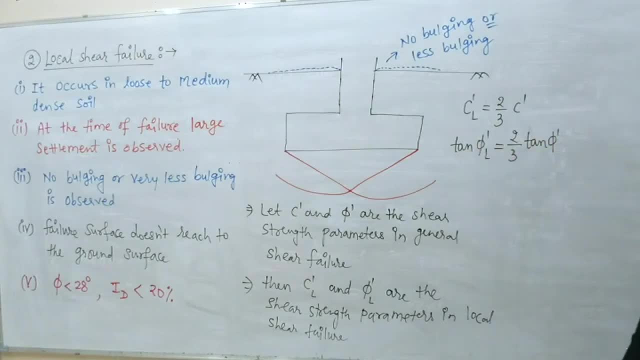 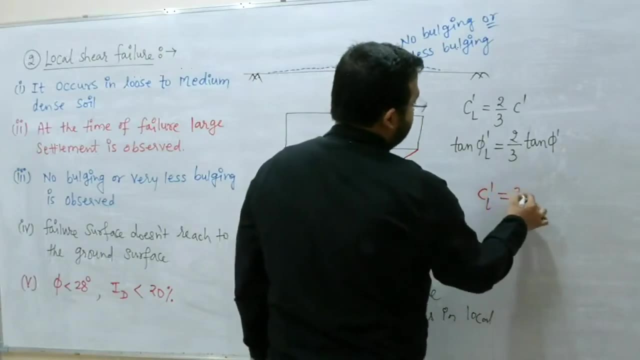 shear failure. so where is the fault here? often children make mistake. they write it correctly: C dash L is equal to two-third of C dash. phi dash will be converted in local of general share failure. They write it correctly. They make a mistake in writing 5.. What mistake. 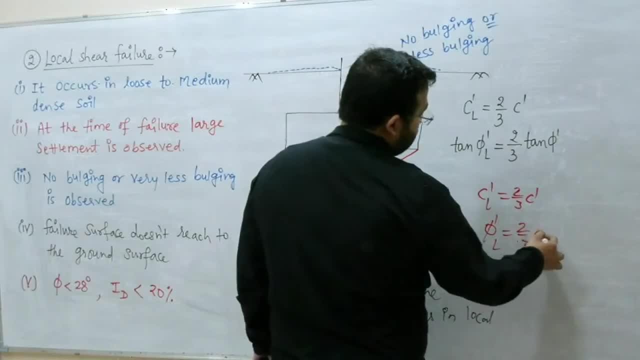 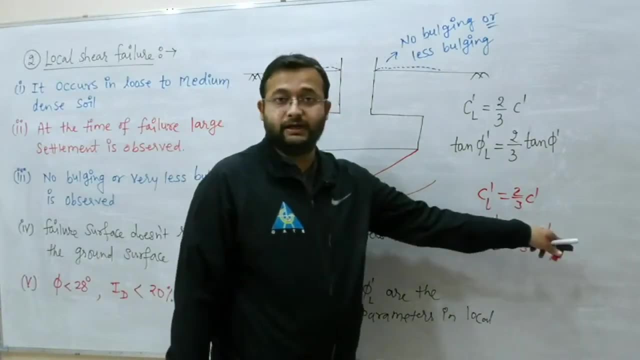 they make. They write 5-L like this: Two-third of 5-. They make a mistake. Local share failure is not directly two-third of 5-. You have to use 10-5-L, equal to two-third of 10-5-. 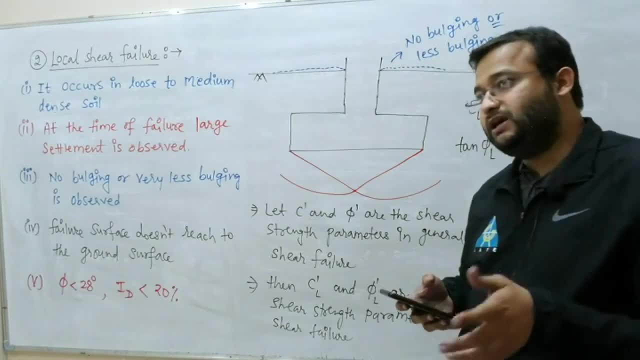 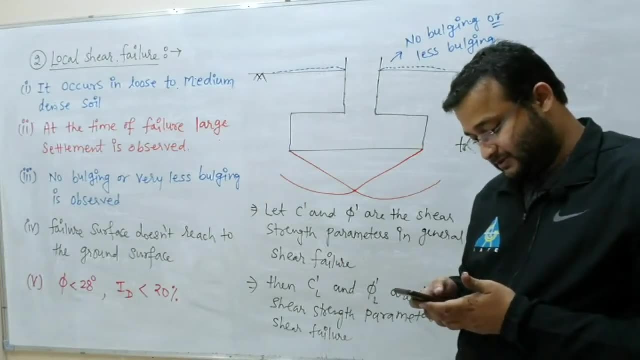 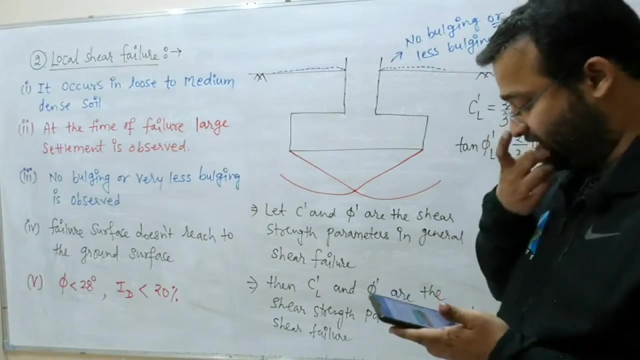 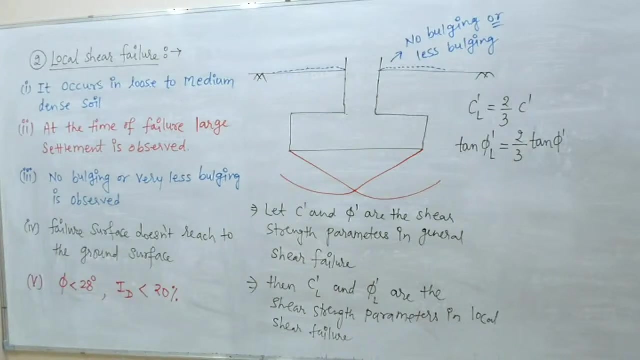 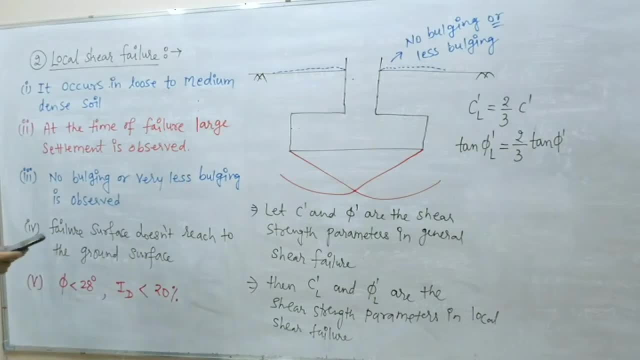 They will be able to see it later in live form. What's the matter? They send kids before me. Very good, Look, this is a kid. What's his name? He is making notes. There is a student named Onkar. 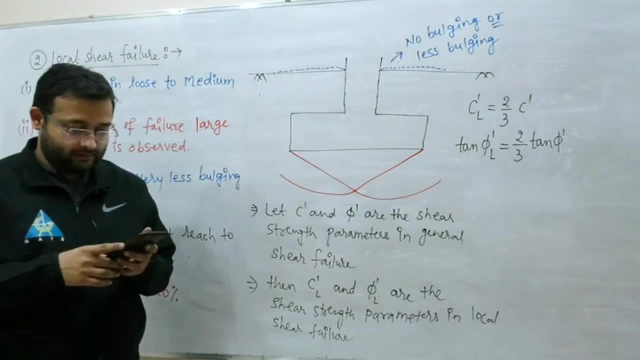 He has sent it on my telegram. There is a student named Onkar. He has sent the notes that I am getting written on my telegram. He has done it very cleanly. He has sent it on telegram. I have also sent the photos of my board. 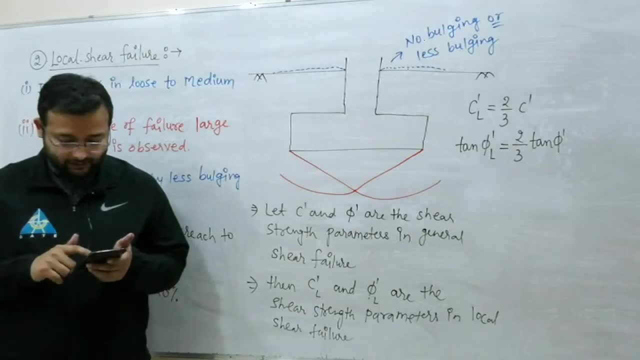 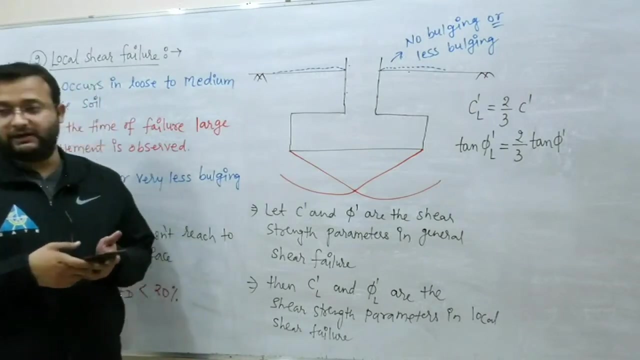 Everything is available. How can I tell you: Don't do that, Don't do heart-wrenching things. I am trying my best from my side, From where I can give you something, From where I can make you do something. I will bring a new face in front of you very soon. 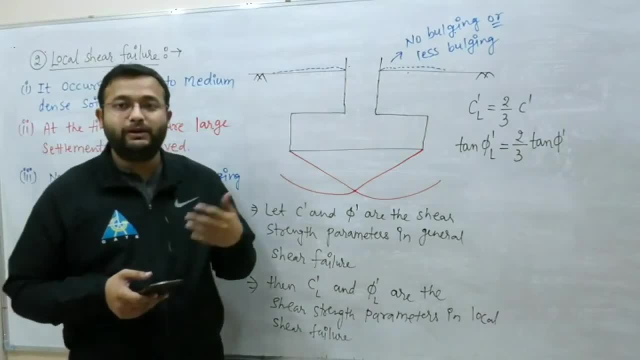 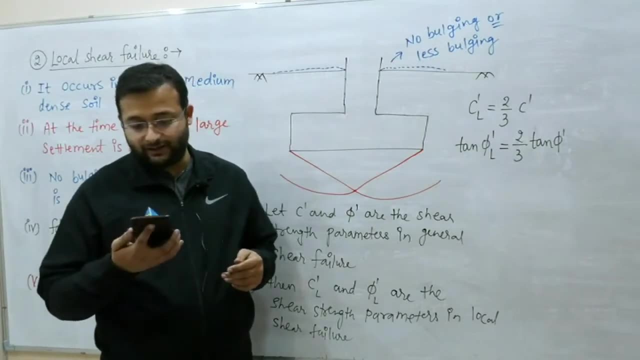 Very soon Where we will talk better. I will make you do all that. I will plan for you all the day. You will do weird things here, Do you like it? We will always help each other. Ok, I will deal with the issues of begged. 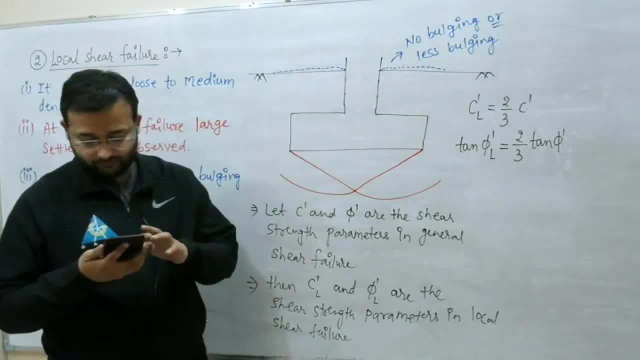 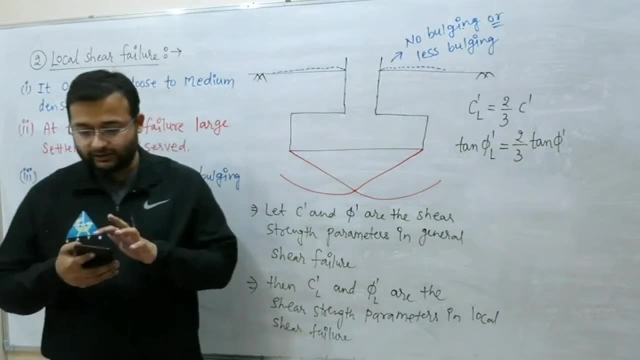 Ok, Ok, Now we will talk. all thenikks, Let us know this message: Let's do it or else you will die. Come here, How are you feeling? How are you feeling? Best wishes, dear friends. I am enjoying your lovely conversation with you. 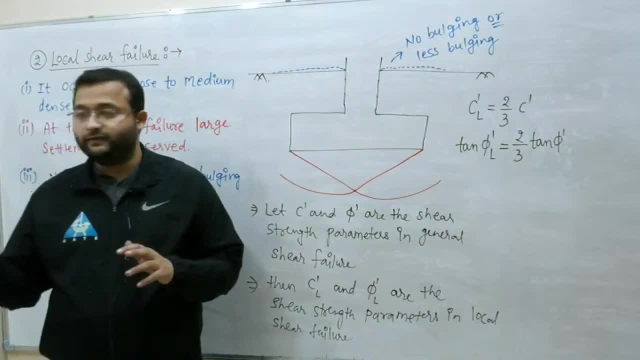 very much, So please message. Hey, Dr Pramod. I want his doctor's residence number. My name is Pramod Kulkarni. It is your first employment in the hospital. In order to find out how he works, I have contacted these people. 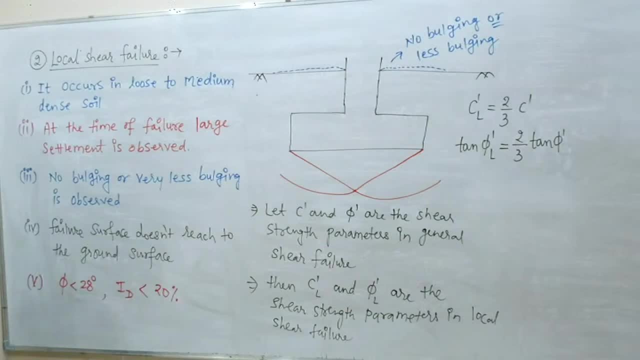 and they also decided to trust me to speak for the next round of the issues of begged. Yes, Papa Donna, who I'm talking about? they will also give it to me, etc. Be itsبد, and you too, Let's move forward. I will rub board number 1 and what we are missing is punching shear. 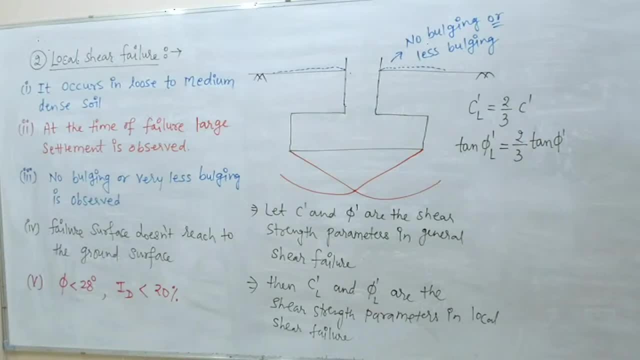 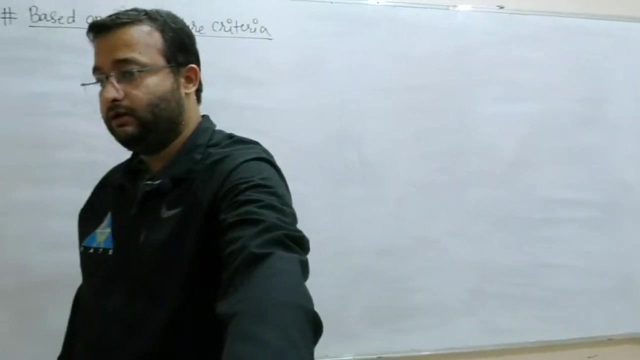 failure. I am telling you that here, See punching shear. failure occurs in structure also, although we are not talking about structural designing. but where does this failure occur? it occurs in structure also. punching occurs. Okay, For example, as I bring you here next our, I am making you write. let's see here next. 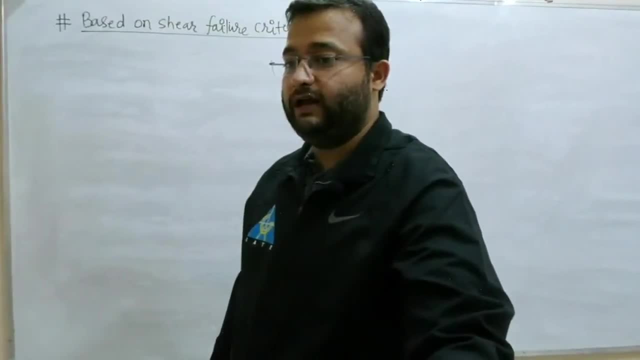 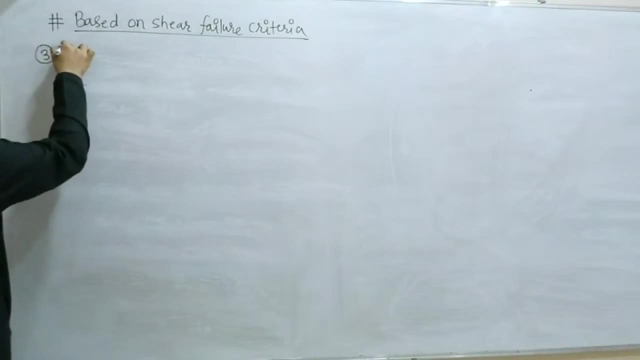 type of failure that we have: Punching shear failure. Okay, There is no need to write much information in this, but still it is okay. let's see a little bit about this too, about punching shear failure. What is this punching shear failure? 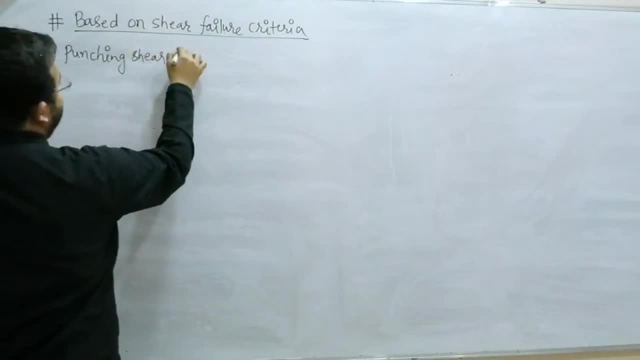 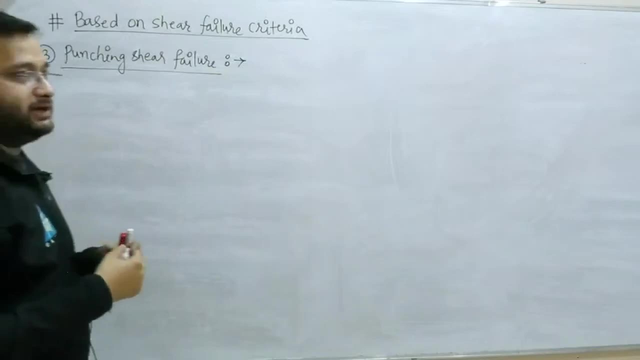 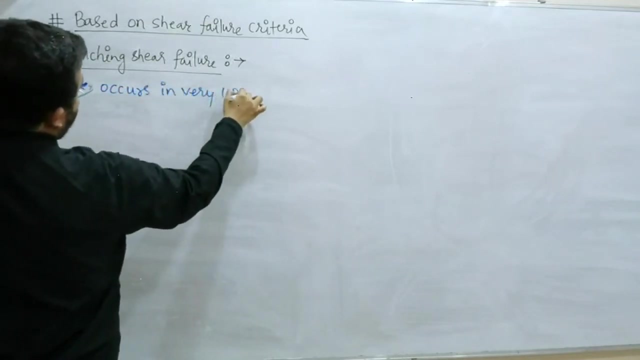 What is punching shear failure? Come, let's understand this. this will be the last topic of today. So punching shear failure, I am telling you that here it occurs in structure also. it occurs in structure also. Here it occurs in very loose soil. it occurs in very, very loose soil. it is very, very loose. 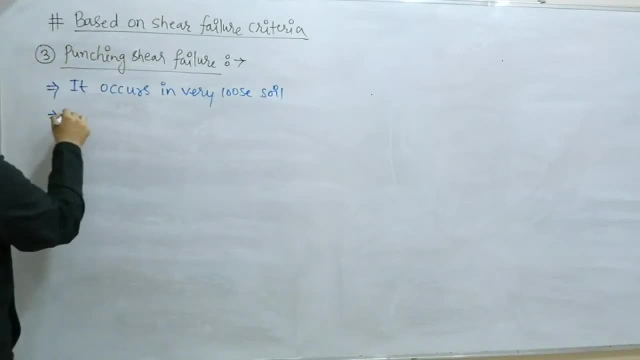 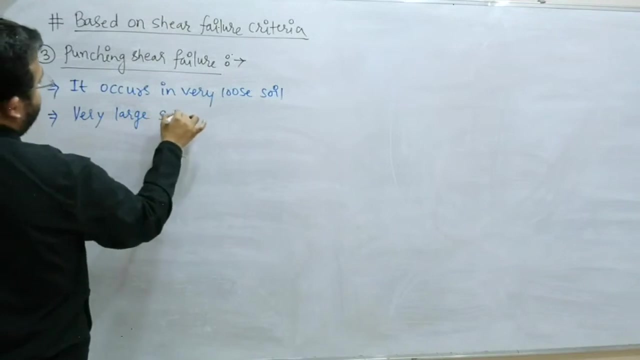 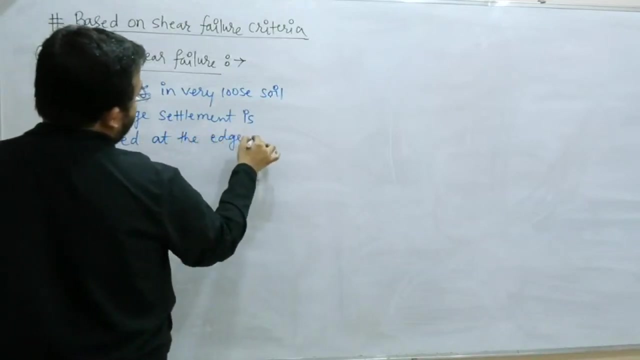 soil. very loose soil means loose sand usually generally means this occurs in that Here large, very large settlement is very large settlement, very large settlement is observed, observed near the edges of the footing or at the edges of the footing, at the edges of the footing. 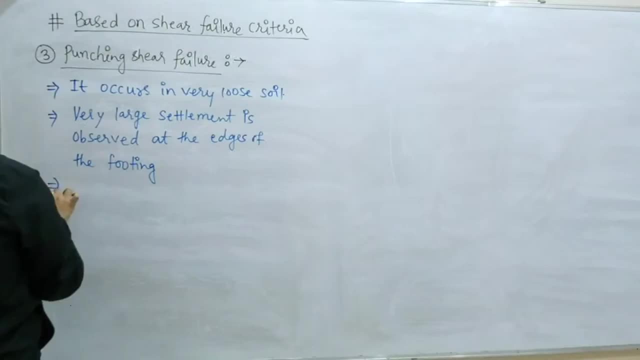 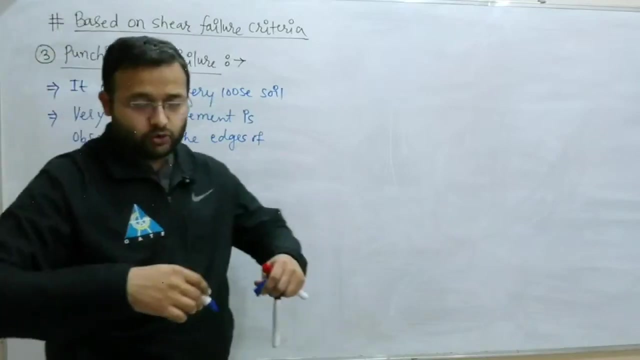 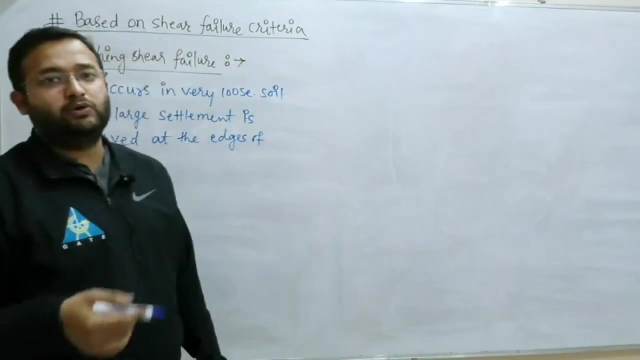 this is your punching shear failure. definitely it will not reach the ground surface because you are smart: when the settlement is high, failure surface cannot reach the ground surface. failure surface reaches the ground level only when the settlement is low. when the settlement is high, failure surface will not reach the ground level. 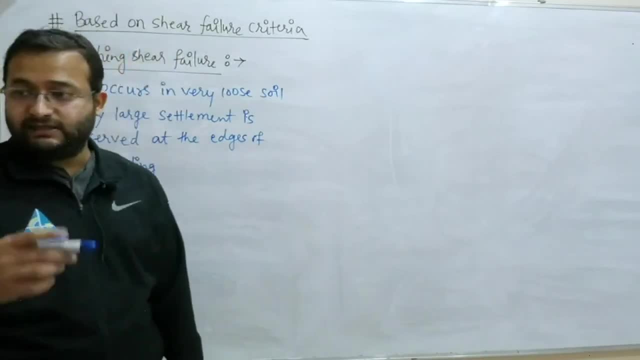 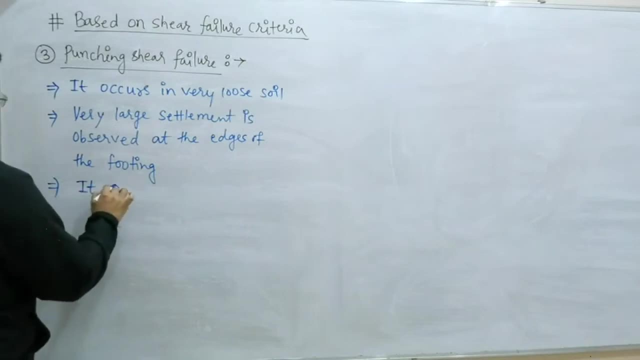 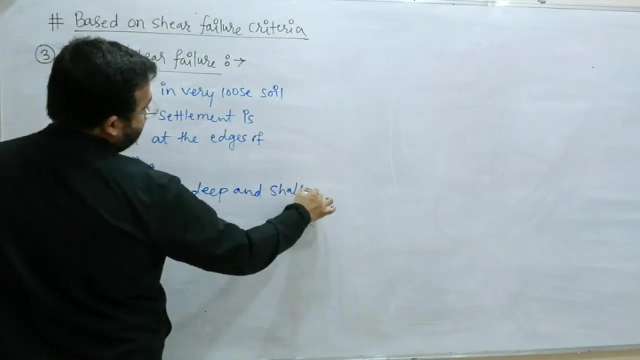 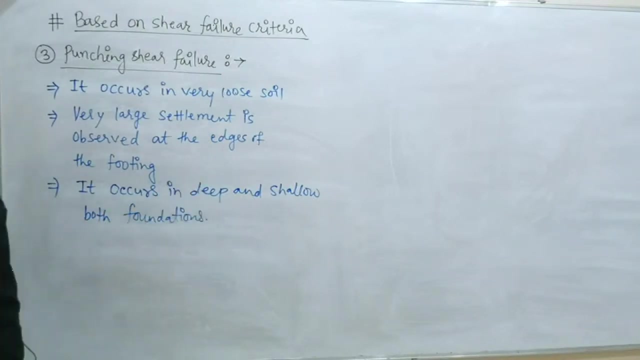 secondly, I was telling you this punching shear failure does not only occur in shallow foundation, it also occurs in deep foundation. so it occurs in deep and shallow both. it occurs in deep and shallow, both foundations, deep and shallow, both. we will get to see this. is it clear? 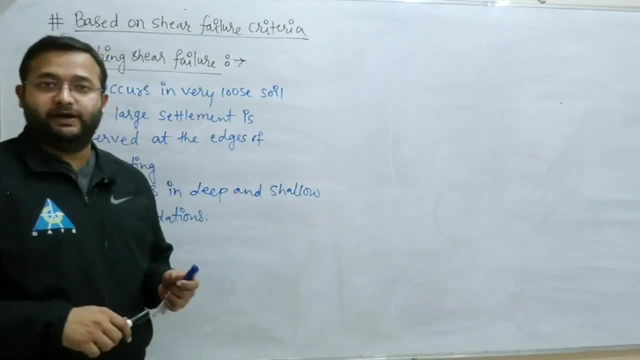 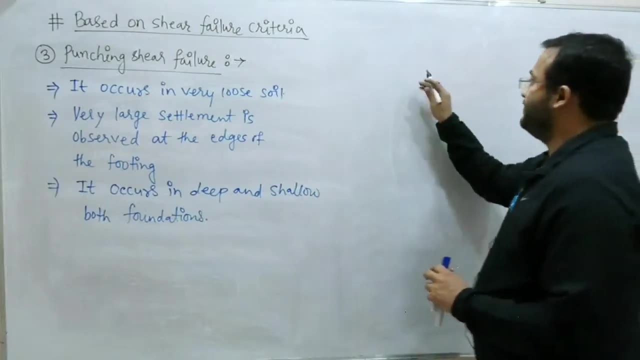 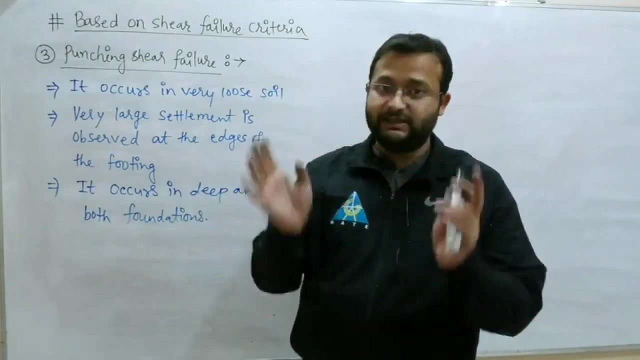 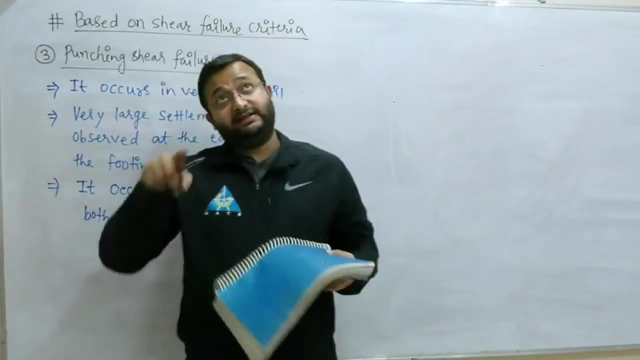 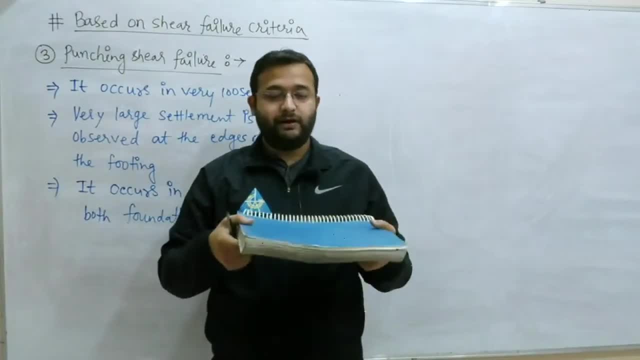 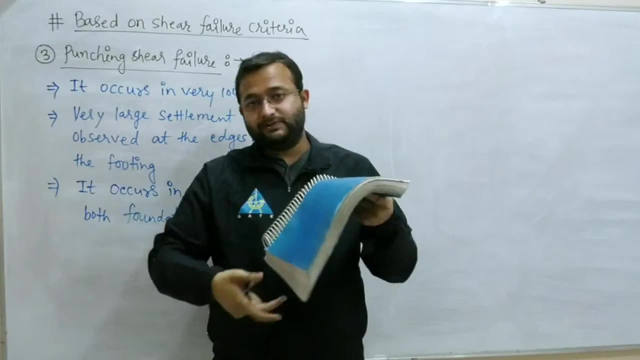 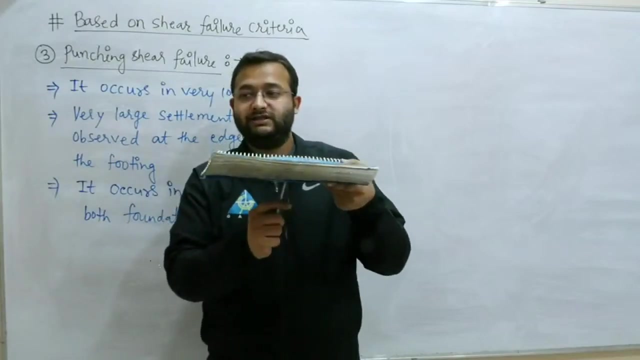 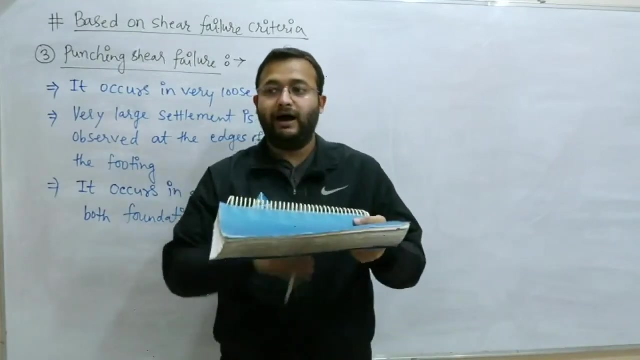 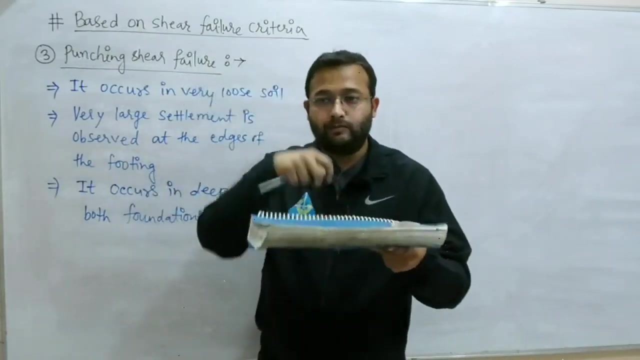 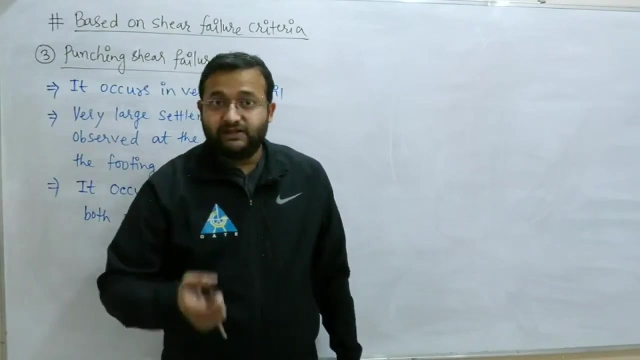 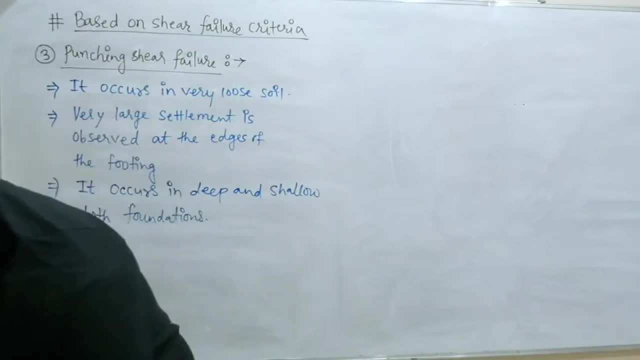 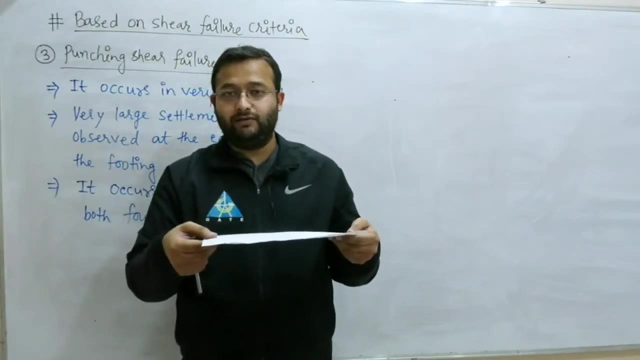 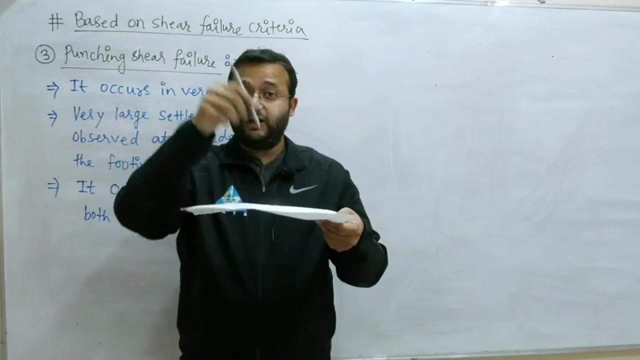 When will it occur in footing? When you will not keep sufficient thickness in footing, Like I am saying. this is my footing Now. see, I have kept very less thickness in footing, Very less thickness, In the same condition if you have kept a column on it and the weight of the column is very high. 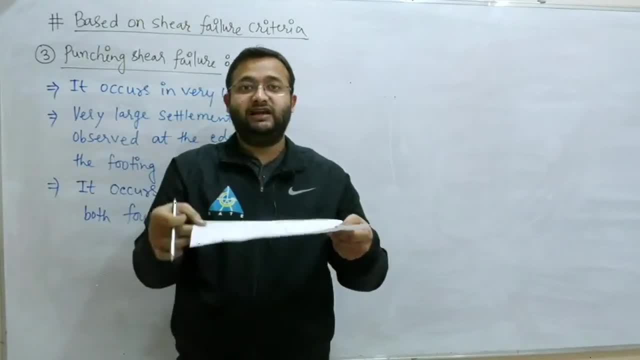 there is a lot of load coming from the column. there is a lot of cross-section of the column, but the thickness of footing is very less. then, in the same condition, what will happen? It will punch it like this and it will go down. 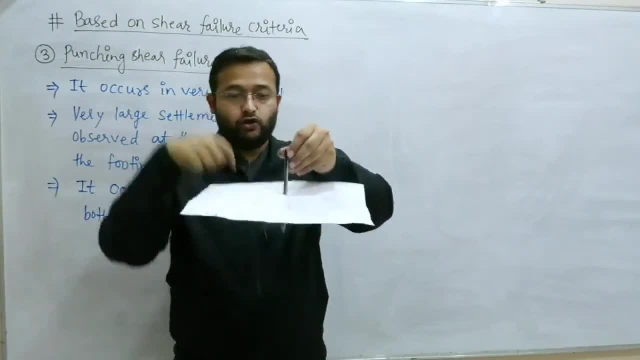 Means what will happen- See, the column is visible- when it comes out. So what will happen to the area around the footing? It will be punched with high load and it will come down When, When the thickness of footing is less. 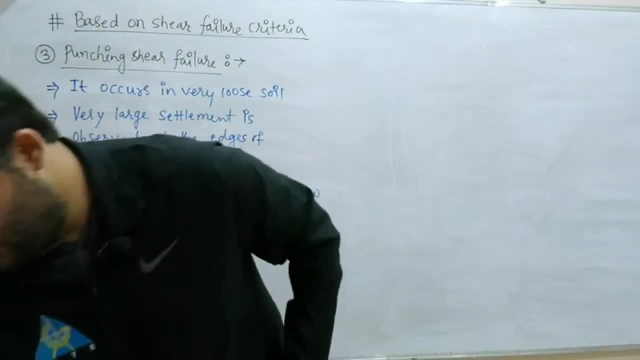 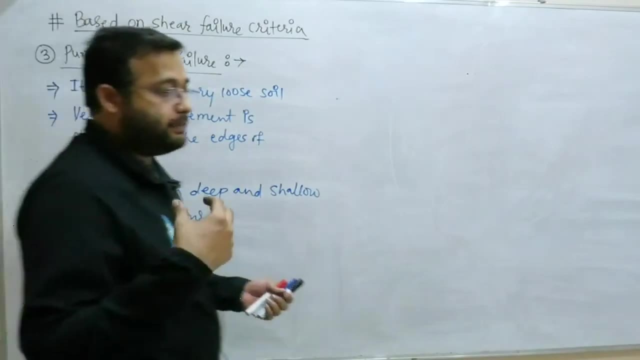 So the same thing was happening here, The same condition was being formed here. What condition was being formed? That the load was more here, But the thickness of the soil was very loose, So we got to see continuous settlement in our footing. 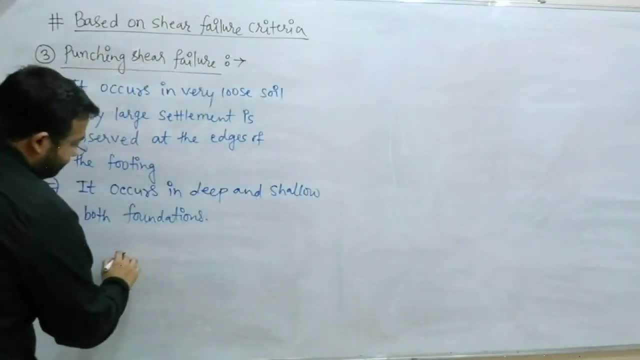 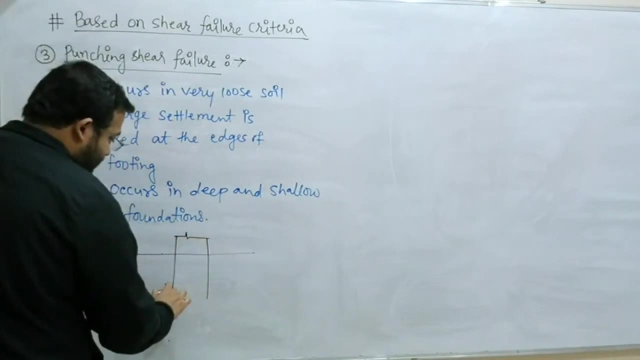 Okay, As I make it here and tell you Like this also occurs in deep foundation. So, as I say, this type of foundation must be working with me. Okay, So, in this way, if we see continuously in it, then here on its edges, on all these edges, 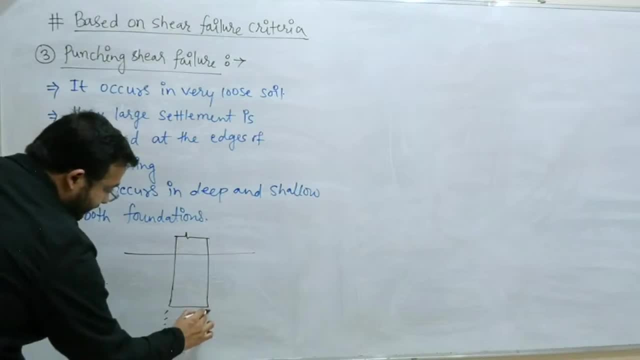 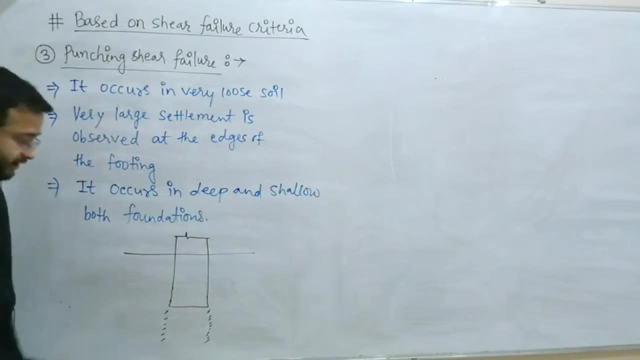 we will get to see continuous large settlement, A lot of settlement, So it will be going continuously down, Okay. Otherwise the failure surface will never come up. It will remain there only, Okay. So we will get to see this there. 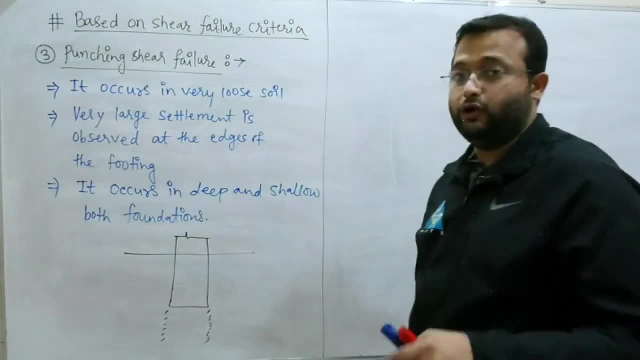 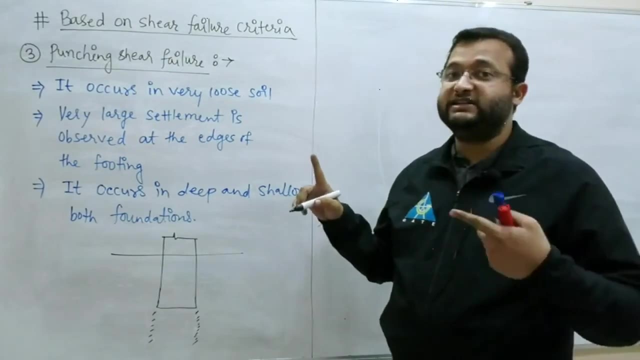 Now, if I see the comparative study in all three, that is, in terms of load versus settlement curve, then here in which the least settlement will be found In general shear failure And the ability to take load will also be more in general shear failure than in soil. 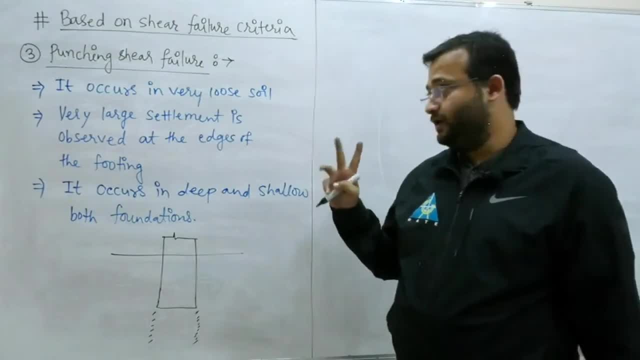 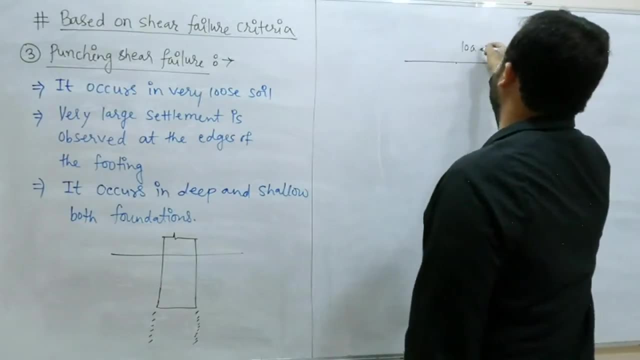 After that local shear failure. After that in the last punching, shear failure. So see, I am writing here. Here we see load versus settlement curve. Here I have taken load. Now this load can also be taken in terms of pressure. 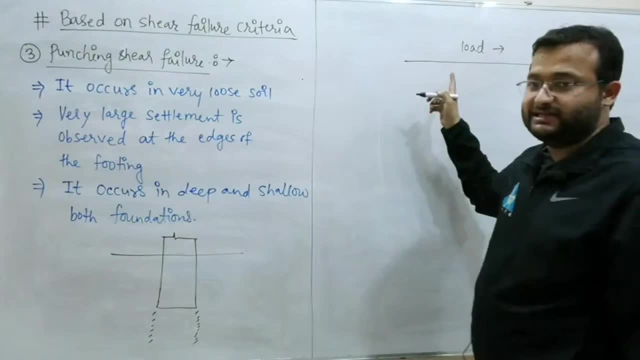 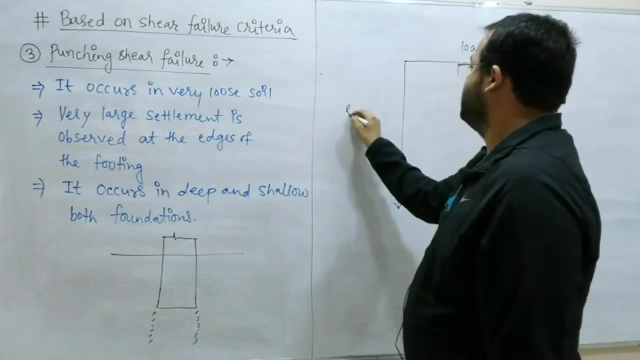 This load can also be taken in terms of pressure. You will have to divide it by area of footing here. Here we have taken your settlement. What have we taken here? Your settlement will be taken. Sorry, The settlement is increasing in this direction. 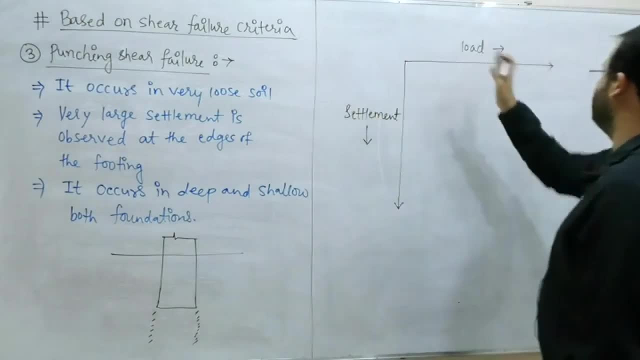 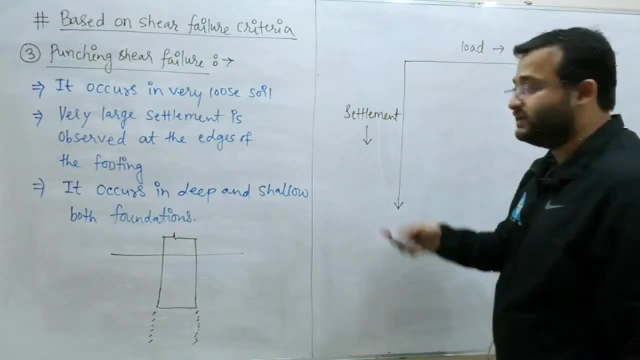 In downward direction. So see here, the load is increasing in this direction, The settlement is increasing in this direction. First of all, I am making a curve here for you all. Okay, This is the curve of general shear failure. This curve will be like this: 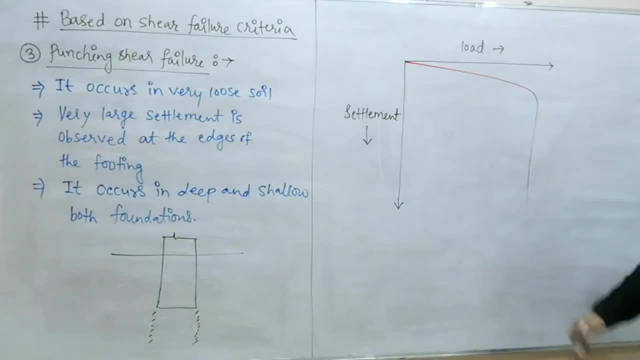 This load is increasing, The settlement is increasing. You will get to see sudden large settlement, So here. you will get to see sudden large settlement, So here the soil has been shared. So see, you have taken a lot of load. 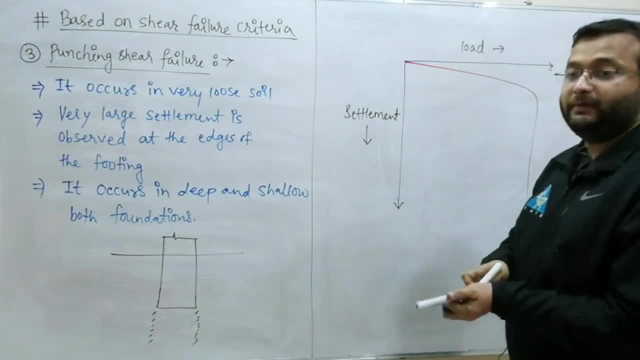 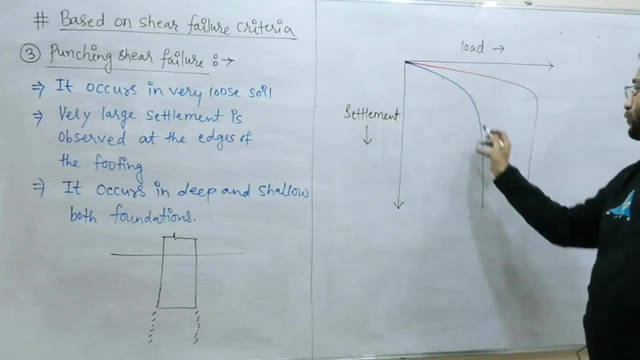 And your settlement was also very less. Second, here we are getting to see punching shear failure. Second, we will get this for local shear failure. You will get this for local shear failure. That means we will get a continuously progressive curve in local shear failure. 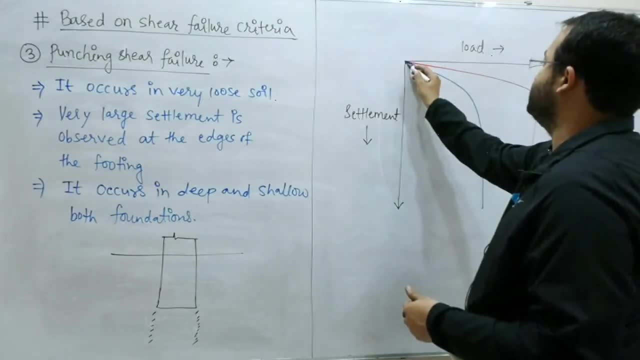 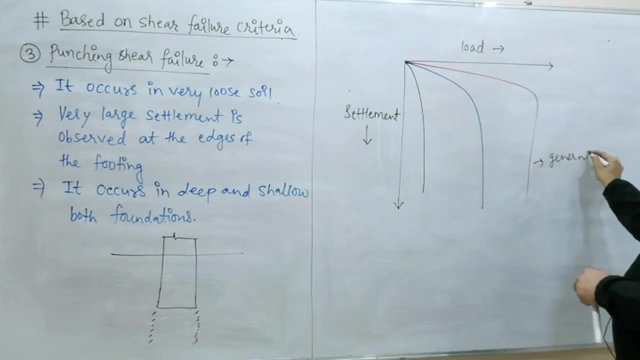 Okay, Similarly, here we will get in punching shear failure in this way. So see all three curves carefully. I will write about it. What is this? This is your general shear failure. This is your general shear failure. Okay, This is your local shear failure. 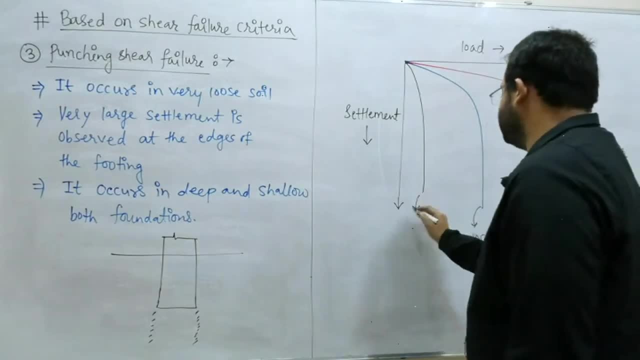 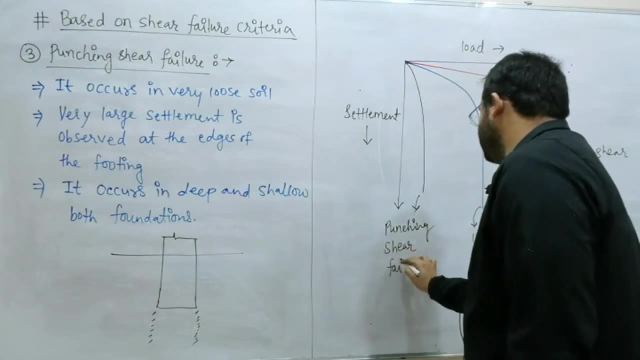 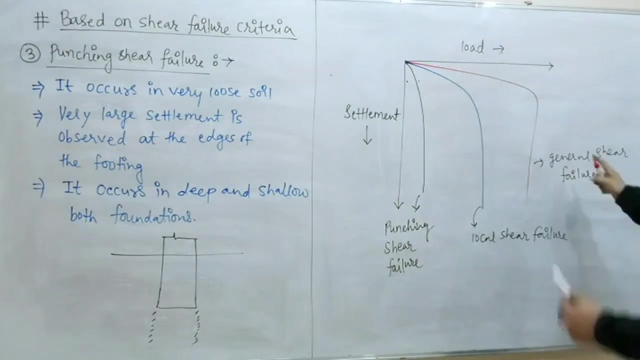 And this is your punching shear failure. Punching shear failure is your condition. Did you understand my third point? Yes, sir, I understood. The thing is, which soil will we get to see this general shear failure? Highly dense soil. It may be your dense sand. 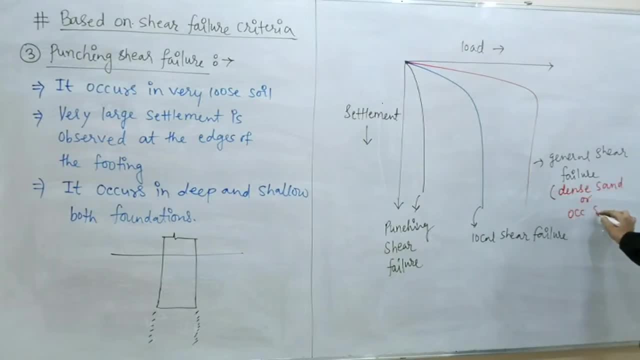 Or you can write OCC soil if you have Over consolidated clay soil. I had taught you OCC soil, Chapter number 3, where I had taught you compressibility Consolidation. There I had taught you OCC soil Over consolidated clay soil, Which has taken a lot of stress in the past. 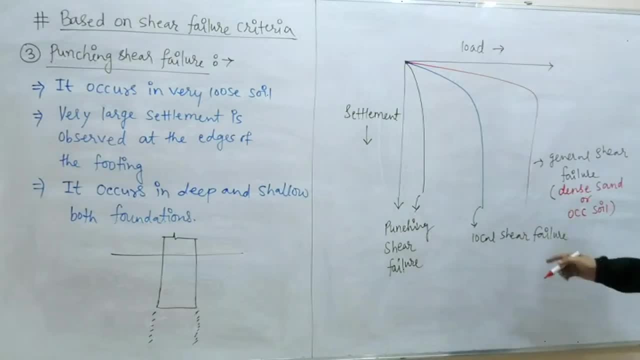 But is taking less stress in present If I talk about local shear failure. So where can we see local shear failure? In loose soil. Or I can write it, You can see it in loose sand, Or you can see this local shear failure in NCC soil. 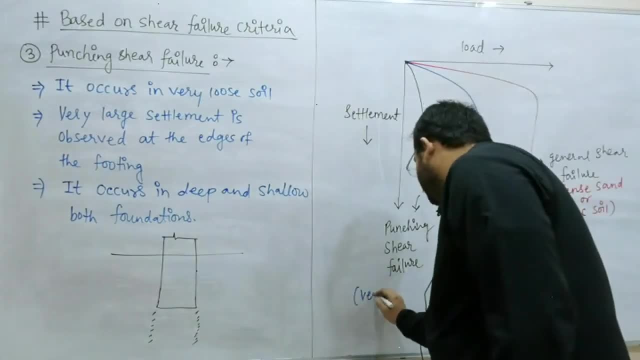 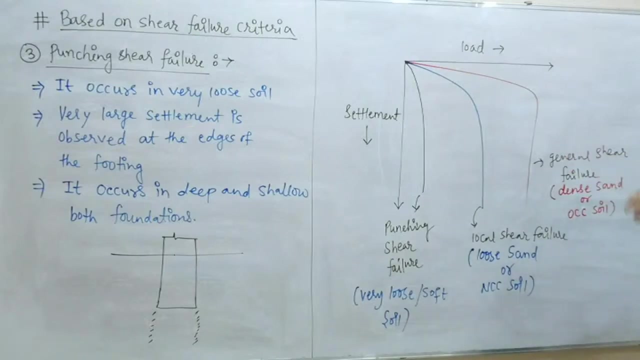 And the punching shear failure. You can see it in very loose or soft. So there we can see this type of failure: Punching shear failure. Do you understand? So these are the three types of failure. So what is the comparison between these three? 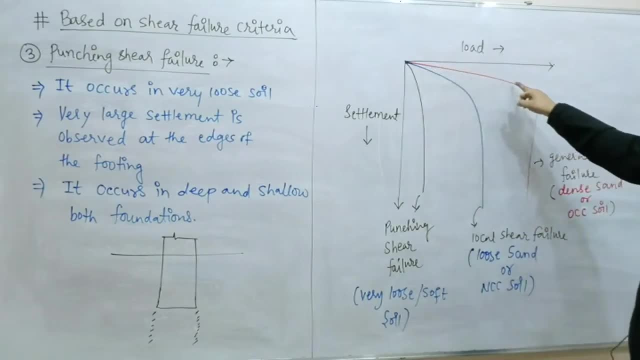 See here: load. This is the general shear failure. How much load is it taking And how less is the settlement After that it is shear. What is it doing? It is taking load and also giving a lot of settlement. But if we talk about this, 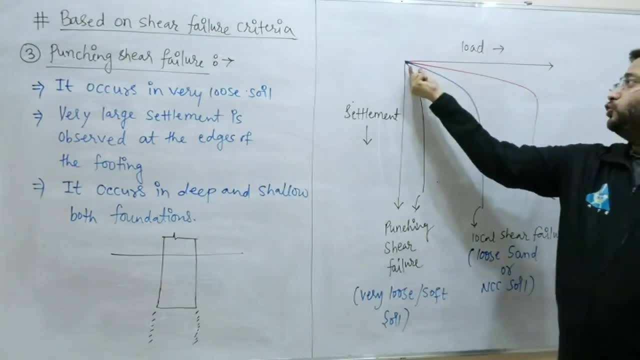 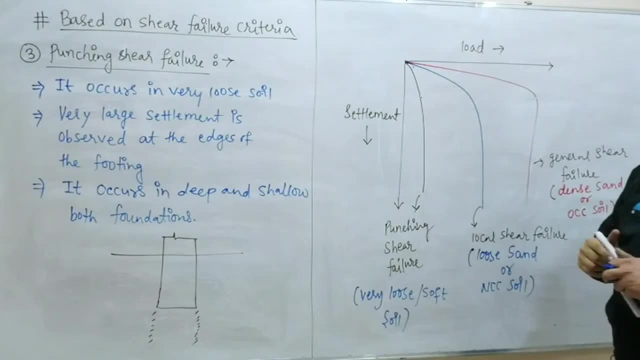 Then this load. The value of load is very less. The value of load is very less, But it is giving a lot of settlement. Okay, Now, here you observe clear failure. One more thing I am telling you: Where are you observing clear failure in these three? 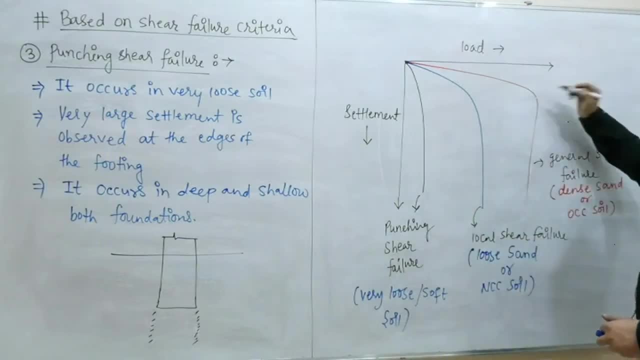 Where did the soil fail? Where is this clear failure observed In the general shear failure? Because what curve gave? suddenly, It gave large settlement, So it came to this place. Your soil was shared at this place, So you will get the ultimate point corresponding to this point. 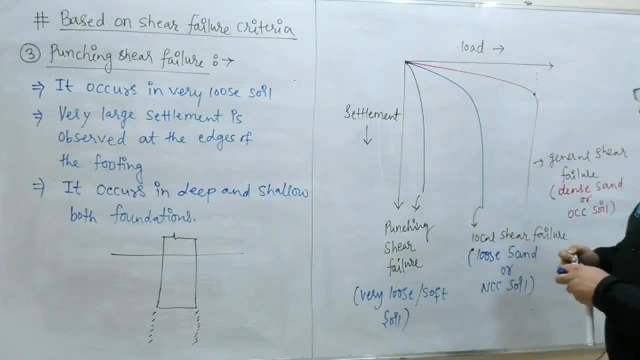 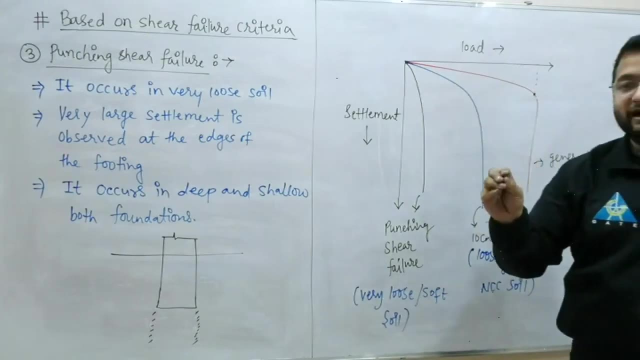 You will get the ultimate load carrying capacity. But if I talk about local shear failure or punching shear failure, Then there is no clear observation here. Here as we get the sharp point, So here we are not getting any sharp point anywhere. 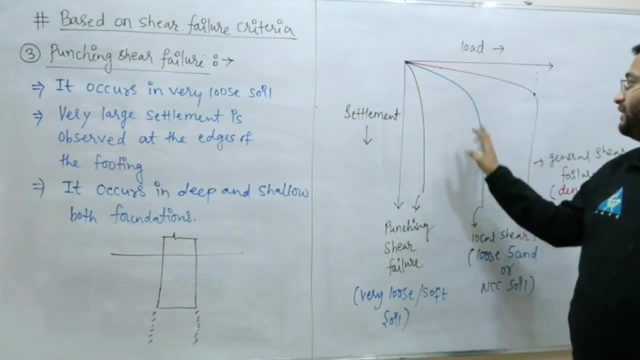 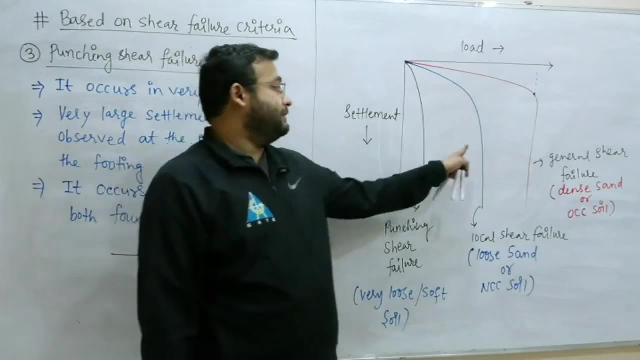 Here also, we are not getting any sharp point. So in this condition, where can we make these two curves? We can make it on the log log scale. Now, I have made all three on the arithmetic scale, But what can you do with the local shear failure? 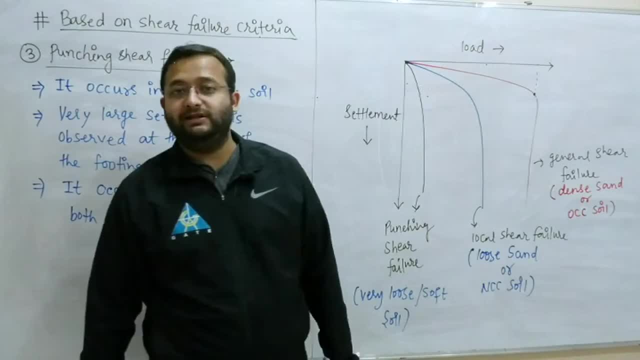 You can also make it on the log log scale. Then you will get the sharp point And you will get to know Where the failure is happening. If you make it on the log log scale, Then you will get the curve like this: 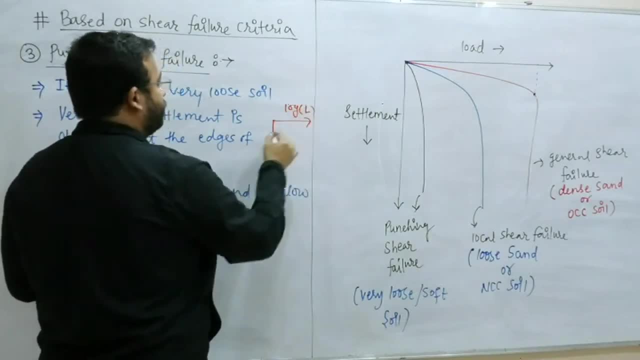 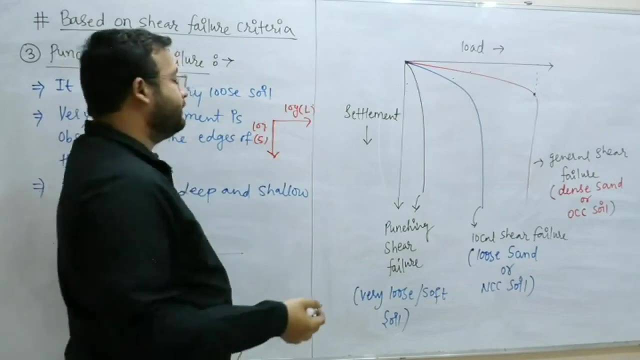 Here we have taken the log load, Log load And here log settlement. Log log curve means: Okay, Here also there is load, Here also there is settlement. But the curve is like log log. So in this condition there is a log on both the axes. 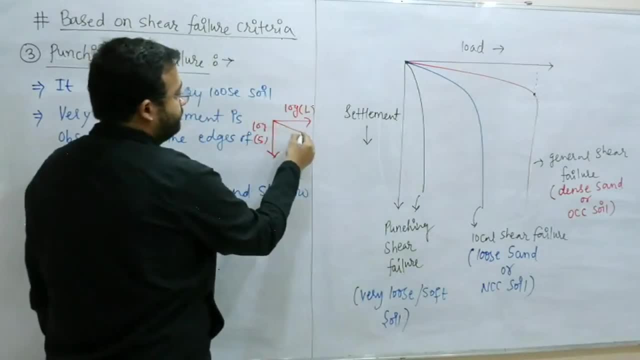 So if you make it on the local shear failure, Then you will get the curve like this, Like this, Like this, You will get the linear curve First. it will be like this And it will change the sign Means you will get the sharp point. 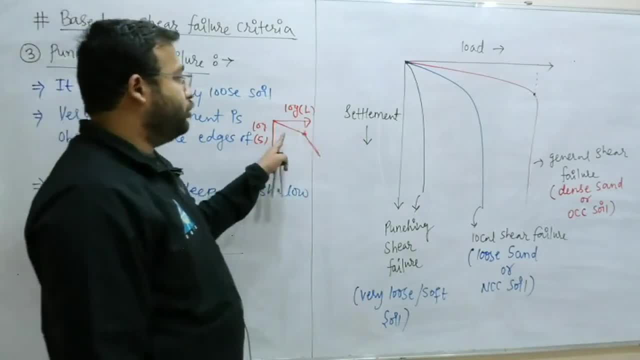 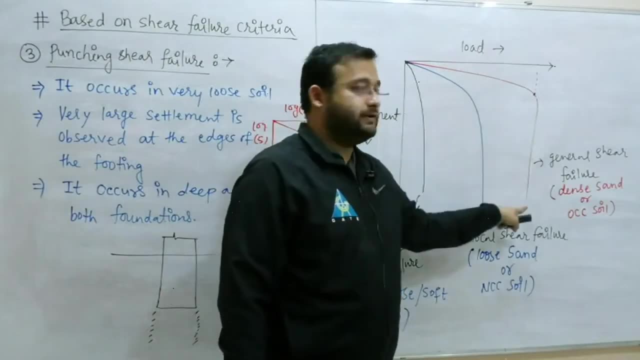 Here your soil is getting shear, So when will you make it on the log log scale When you are not observing clear failure in that condition? Here clear failure is being observed, So it is not necessary to make it on the log log. 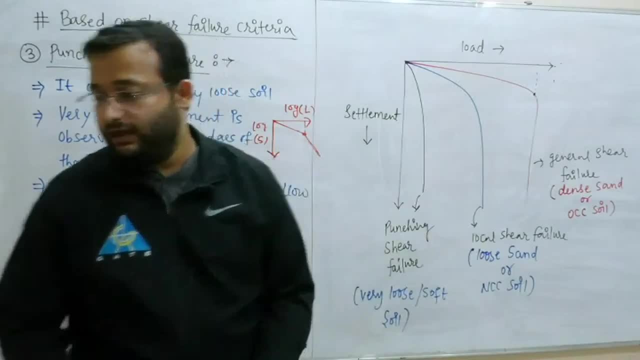 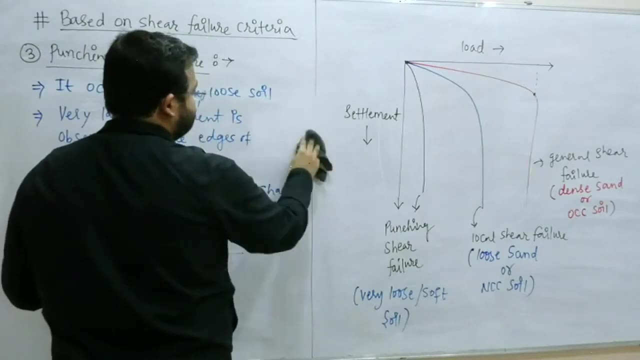 But yes, it can definitely be made on the log log Or it can also be made. Okay, Till here. So I have mentioned it here, You can note it. So this was our last topic for today's discussion, You note it. 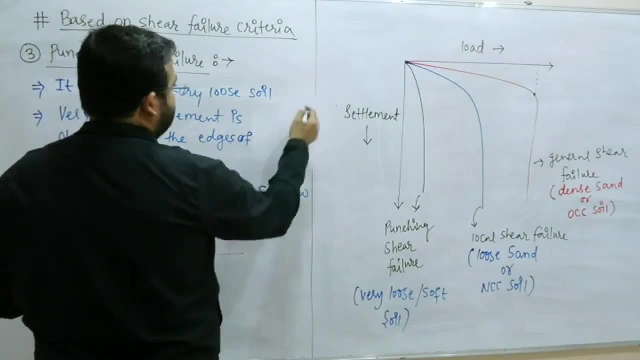 Do not forget to click on the like button And do not forget to subscribe to our channel. So till here. We will meet again in the next class. Thank you very much. Bye, Thank you very much. Take care, Take care. 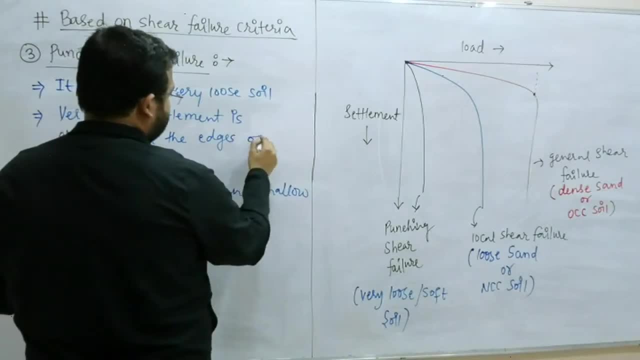 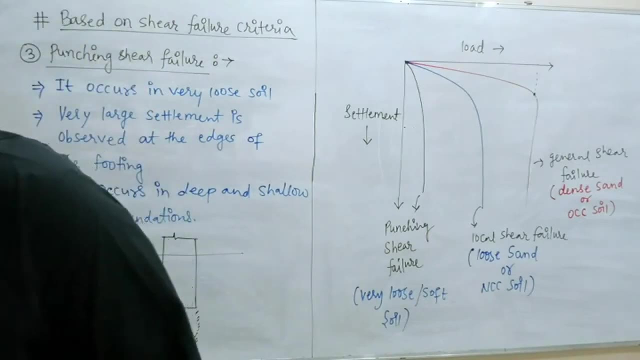 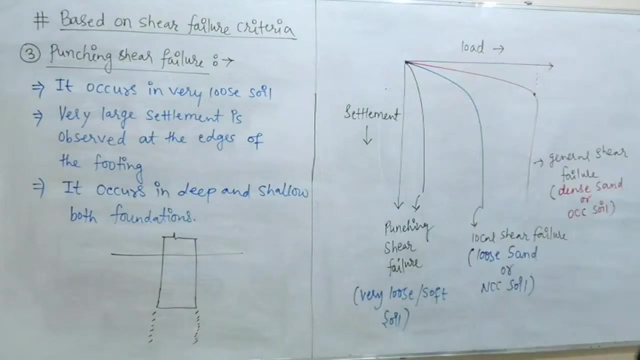 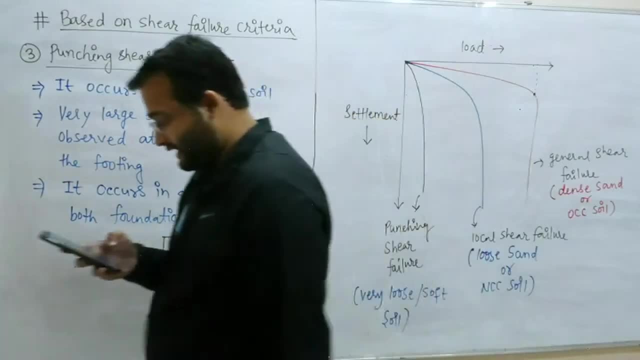 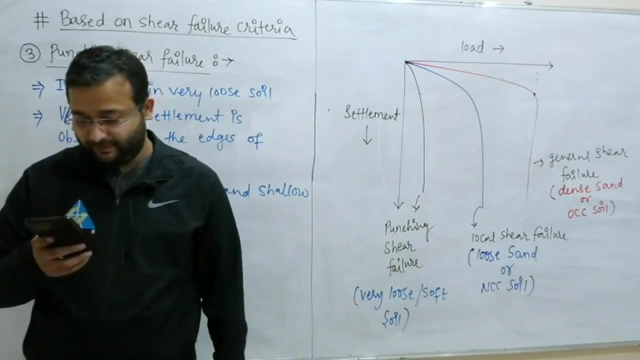 I have sent you on telegram. What is the matter? You have sent it before me. Who was the sender? Shivam Divedi. You have sent it before me. very good, Ok. Ankar ji's photo is also in the group. Everyone is sending it honestly. 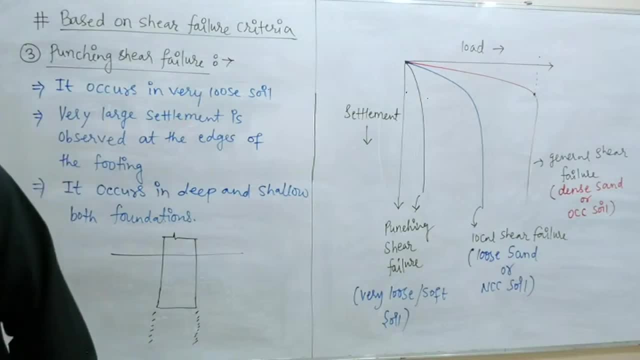 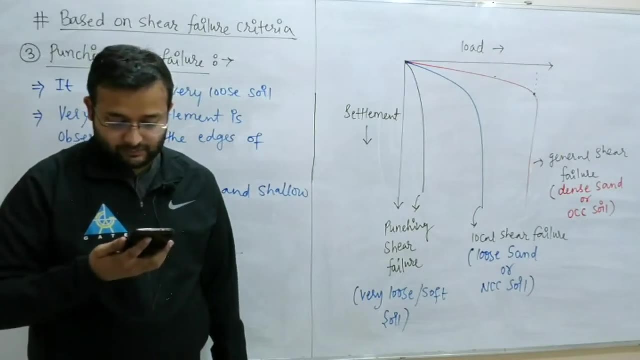 They are reading it. it means that you are good. Sometimes it hurts my heart, So my mind gets out. Don't do this, You won't believe it. I haven't eaten anything since morning. What time is it going to be? It is going to be 2.30 in the morning. 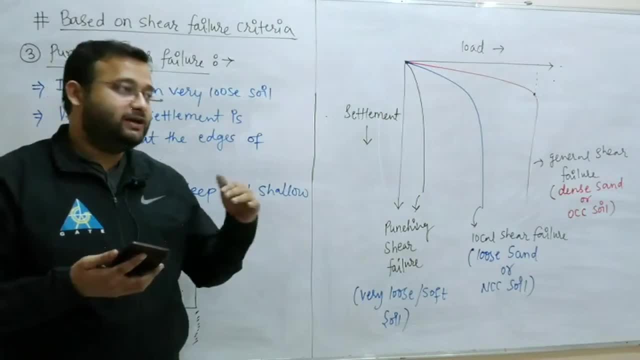 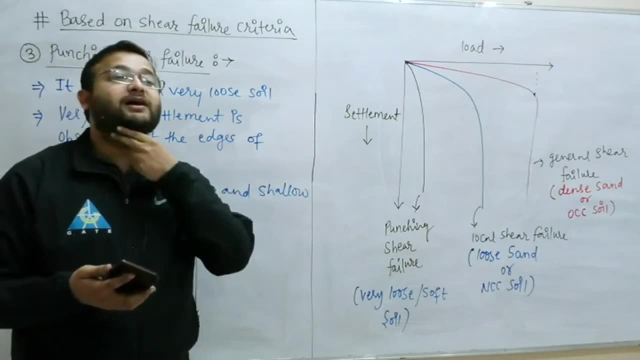 I haven't eaten anything since morning Because I have been studying since morning And in the meantime. if you will play such drama, If you will write such nonsense, Won't the other person's mind get spoiled? On top of that, his health is also bad. 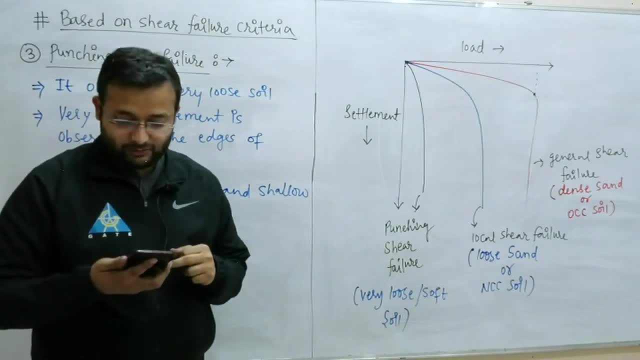 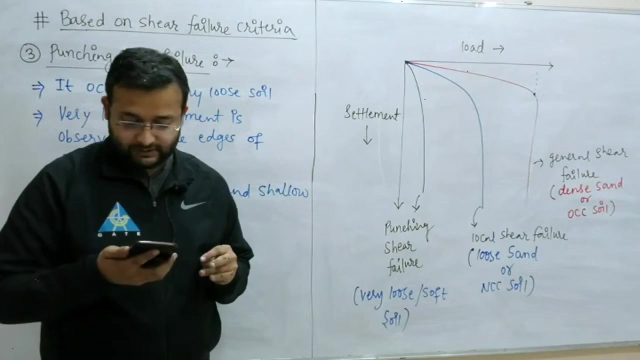 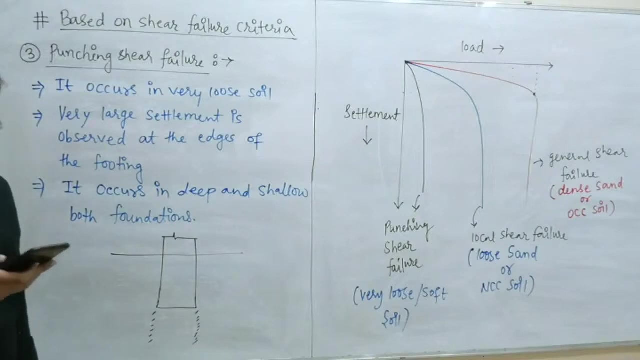 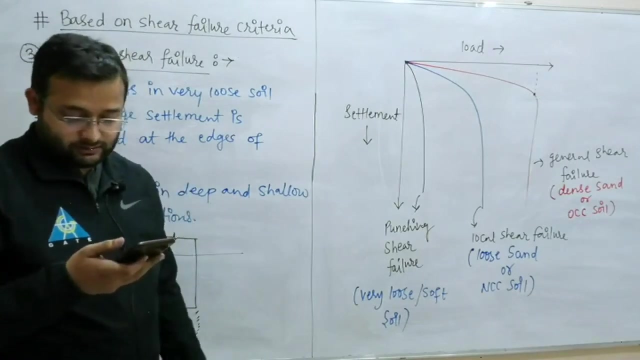 My whole neck is swollen. If you will write like this, It will hurt. I don't feel good. Ok, Come on, You people who are taking photos. I am stopping today's session here, So Thank you. thank you everyone. Ayush is right, Sometimes it hurts my heart. 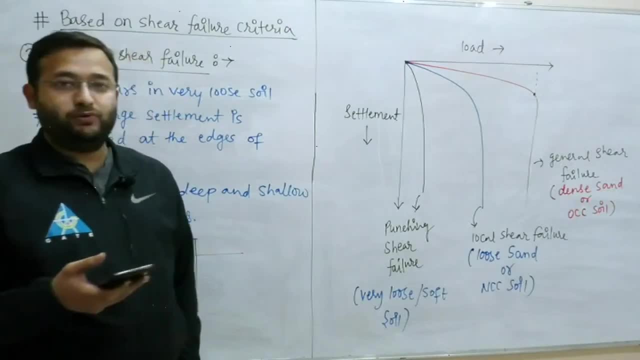 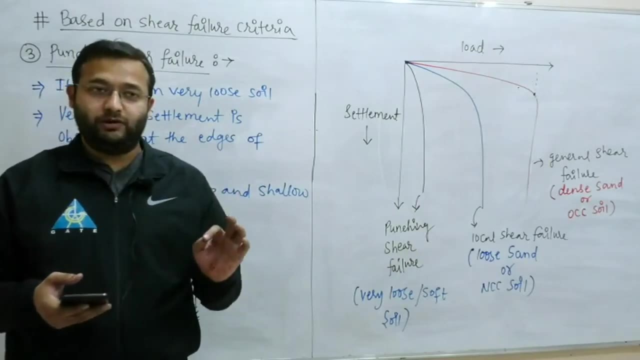 It is not like I don't want to teach you. If I don't want to teach you, then why should I come? Think for a minute. Those who are talking nonsense, right? That's why I am saying: I know that many of you are competitors. 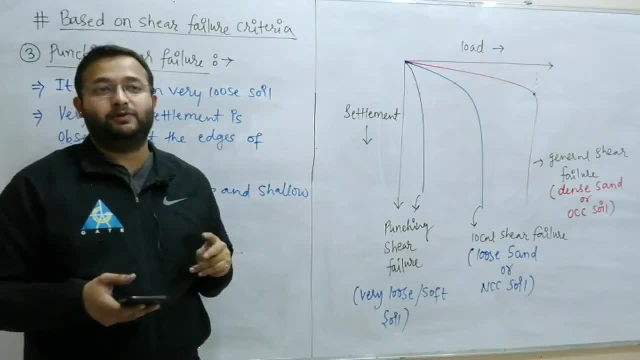 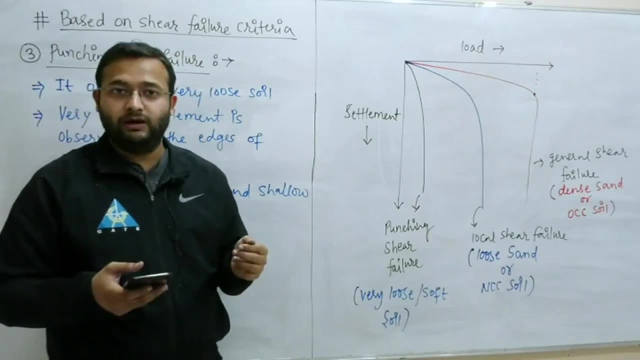 Of us and XYZ, Whatever it is. But I am telling you one thing: If I don't want to teach, Then why will I come here live? Why will I come live? Am I getting any income by taking live? Nothing is happening. zero, zero income. 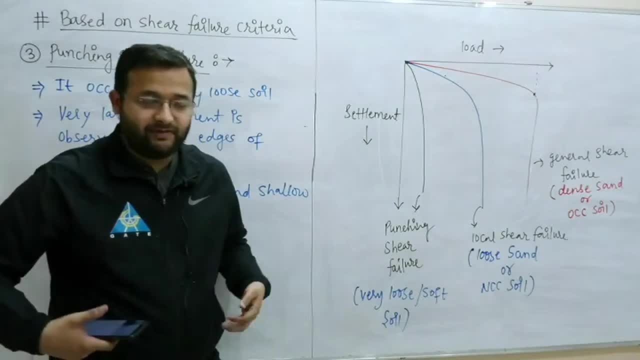 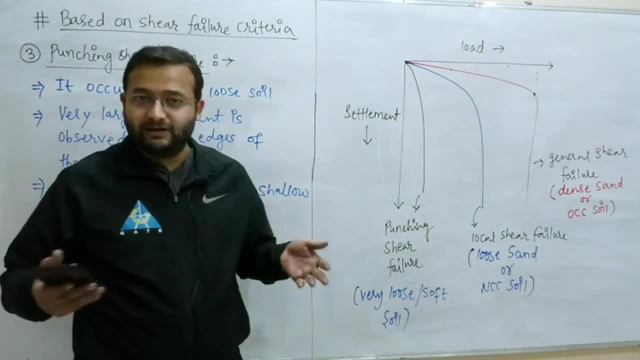 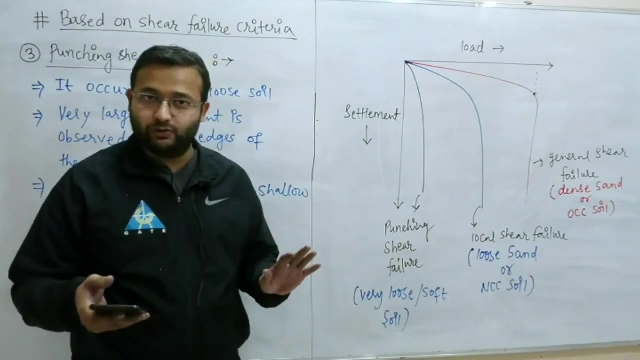 Why will I come? Why will I spoil my time? Why will I stand? My weight is also very high. Tell me, My throat is shaking. I haven't eaten anything since morning. Then why will I come to teach? And it is not like I get a separate salary to teach.